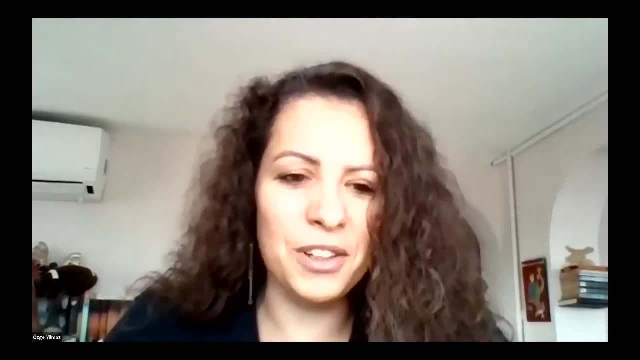 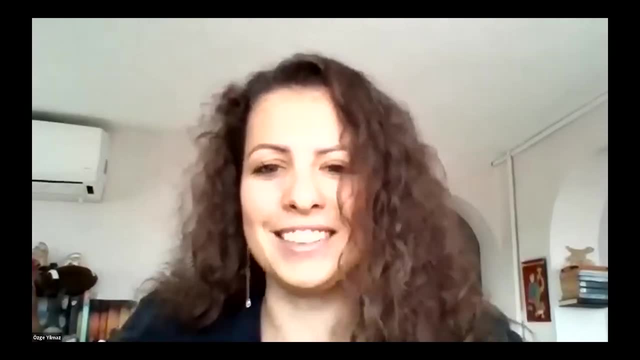 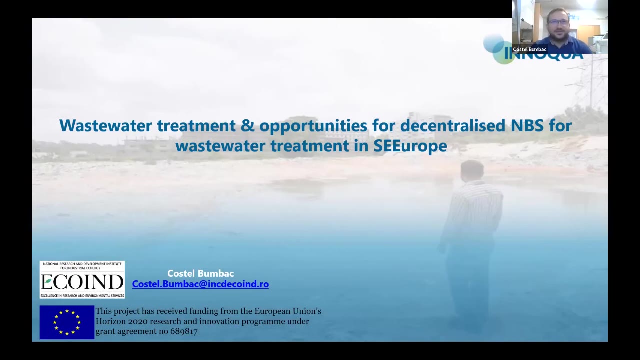 Manager of the INOKOA Project. He will give the introductory talk on the Inokoa Project, talk on wastewater treatment in region: opportunities for decentralized, nature-based solutions for wastewater treatment. because that, the floor is yours, thank you. good morning everybody. i am a coastal boomback. i'm a research scientist, as i said, within the environmental technology. 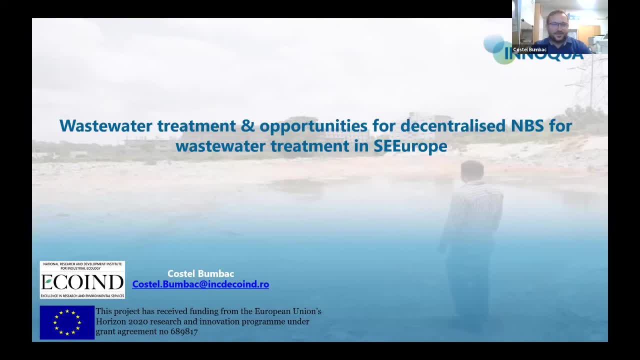 and technology transfer department of echoing romania and demonstration manager for the innova project. echoing dominates a national research and development organization dedicated to environmental research and services, providing services in the field of pollution control, environmental monitoring, impact assessment, ecotoxicity studies, air, water, wastewater and soil treatment and waste management. i will give a short introduction. uh, i'm afraid it. 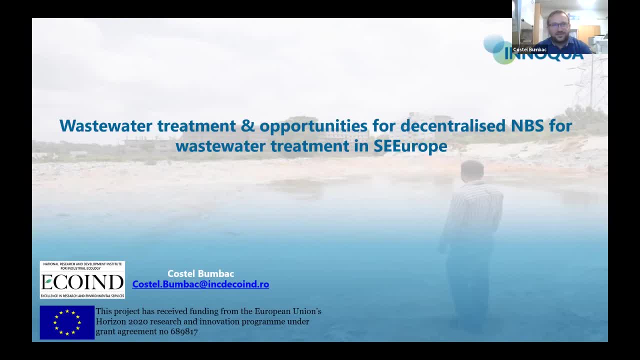 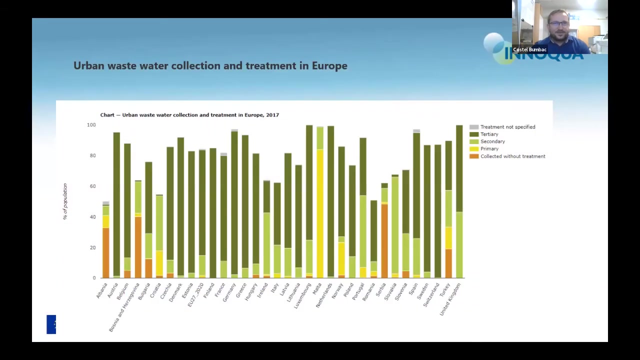 will be a little boring with fact and facts and figure figures on the status of wastewater treatment at european level, with a slight focus on of eastern european countries, aiming to identify the opportunities for decentralized wastewater treatment and, moreover, suitability of adopting nature-based solutions to address this matter. 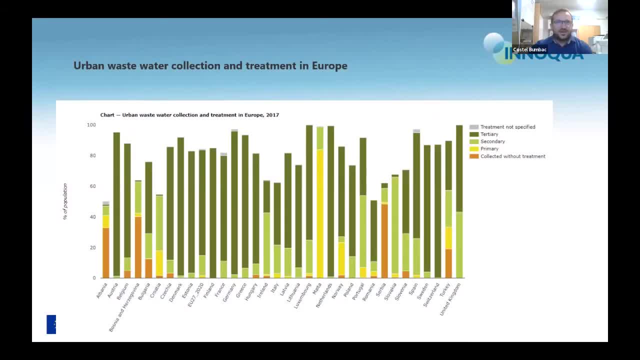 this is the overall image provided by eurostat for 2017, describing the urban wastewater collected and the level of treatment applied as a percentage of the population. orange bars represent the sewage collected but not rated before discharge. yellow bars represent primary treatments, such as settling, for example, light green bars represent secondary. 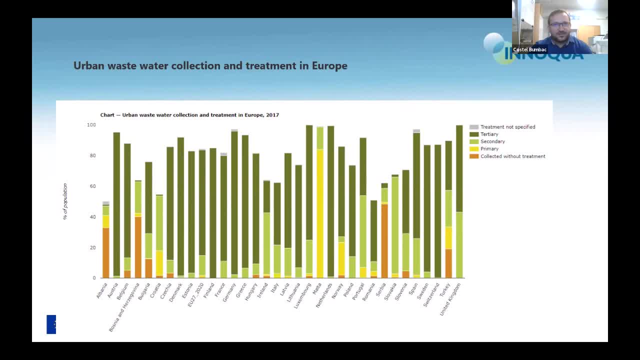 treatment to reduce dissolved and suspended organic compounds, such as those using biological methods, while dark green bars represents more stringent tertiary treatment, mainly to reduce nutrients. the treatment of urban wastewater from our homes and workplaces is fundamental to ensuring public health and environmental quality. so the main objective of the urban wastewater treatment directive and equivalent. 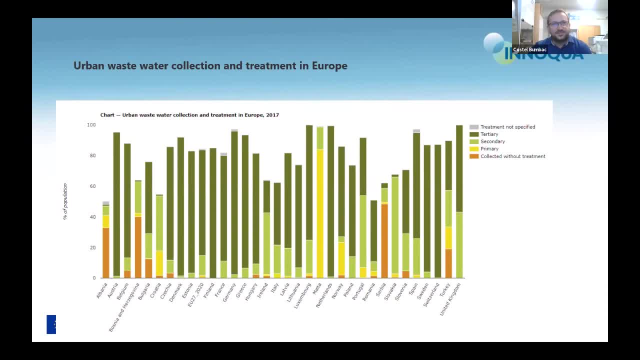 national legislation from non-european countries is to protect the environment, specifically surface waters, from the adverse effects of water discharges. the urban wastewater treatment directive covers agglomerations over 2000 people equivalent. in most cases, it stipulates that the wastewater must be subjected to biological treatment- secondary treatment, but engagements with. the particularly sensitive areas, such as those suffering from deodorization, more stringent tertiary wastewater treatment may be required to substantially reduce nitrogen and phosphorus pollution impacts, the irradiation of community buildings and situations like drought or school cataracts, such as bladder cramps or kidney issues. 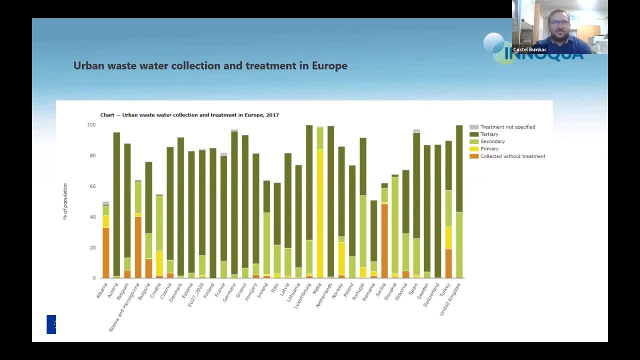 Texas, American Rwanda and the Netherlands, Florida and slovenia. between 71 to 76 percent of the total population are connected to urban wastewater treatment. there are several countries where more than 40 percent of the population were served by treatment below tertiary level in 2017, such as albania, bosnia herzegovina, ireland, malta, portugal. 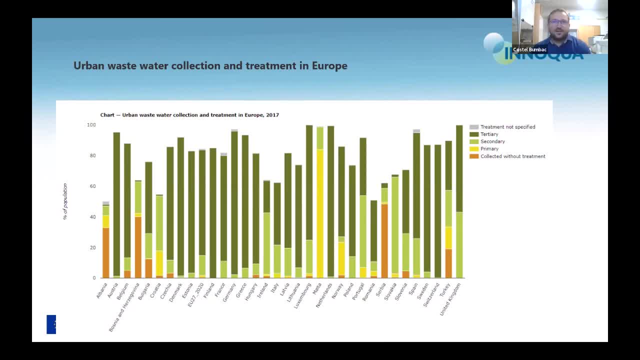 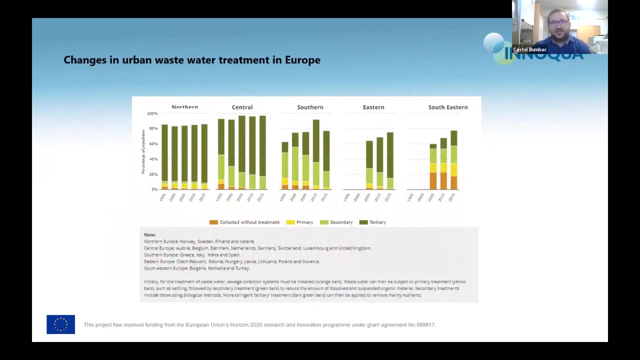 serbia, slovakia, turkey and the uk. some of these countries are islands which have long coastlines and have designated only fractions of their territory as sensitive areas, while others are candidates countries and potential candidates of the european union. wastewater to a tertiary level, for example, to remove nitrogen and phosphorus, which otherwise can. 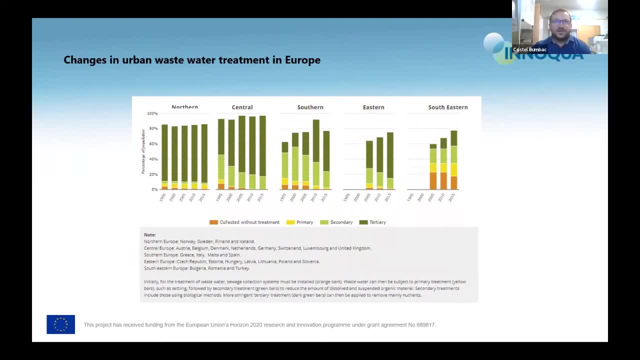 cause nutrient pollution. in 27 countries, almost 70 percent of the total population were connected to tertiary treatment facilities. tertiary treatment was widespread, already in place in a few countries by the 1990s in countries such as england, germany, sweden and switzerland. in several older your member states, significant effort to improve levels of treatment were 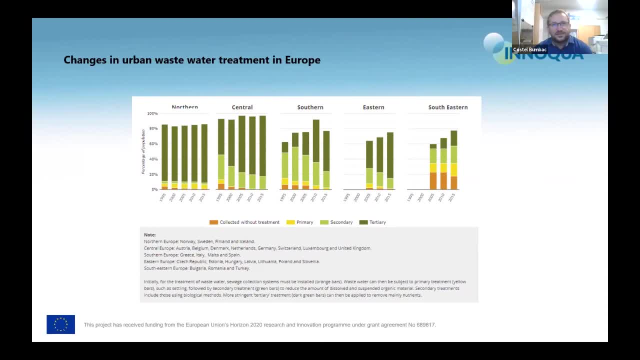 undertaking during the 1990s and 2000s in countries such as austria, belgium, denmark, greece, netherlands, portugal or spain, while in recent years, investment in the treatment of urban wastewater, particularly in the newer new member states, has been directing higher level treatment. 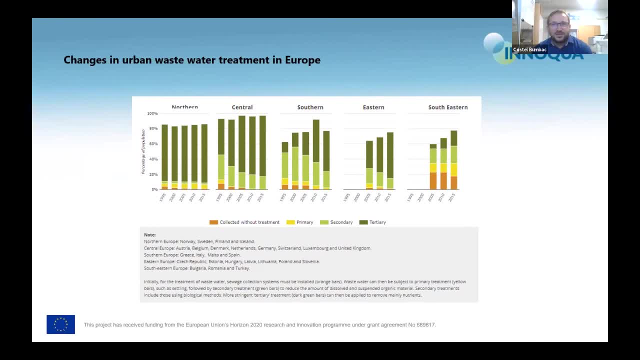 in countries like baltimore and ucsp and other countries with a habitat management management like Bulgaria, Czech Republic, Estonia, Hungary, Latvia, Lithuania, Poland, Romania and Slovenia. This may reflect that these countries have designated their entire territory or most. 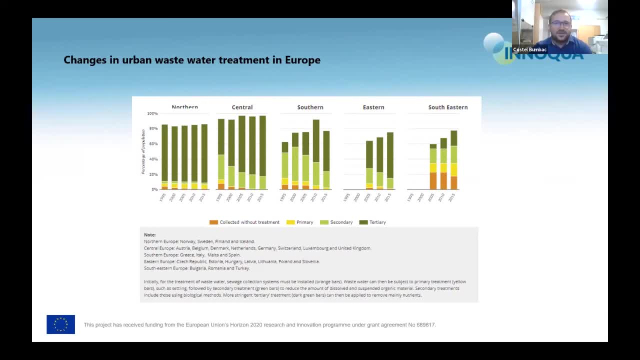 of their territory, such as the case of Slovenia, as sensitive areas, which leads to the obligation under the Urban Wastewater Treatment Directive to treat the wastewater more stringently in agglomerations over 10,000 people equivalent. In most cases, it is possible to see the building of collection facilities, increasing the proportion. 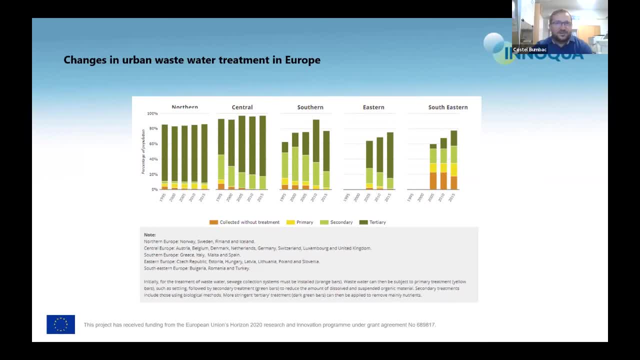 of the population connected and the level of treatment provided becoming higher. At the same time, the decline in collection without treatment or primary treatment has replaced by light and dark green bars signifying the secondary and tertiary treatment. The adoption of the Urban Wastewater Treatment Directive in 1991 promoted the improvement. 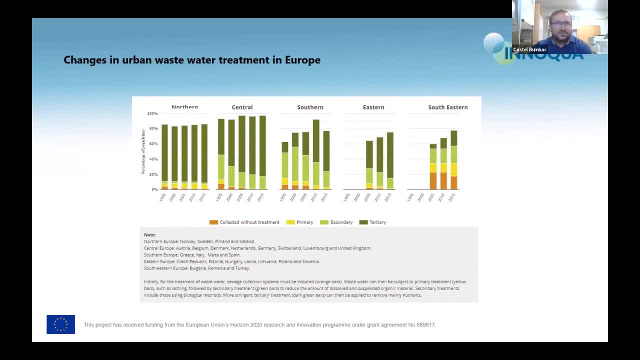 of urban wastewater treatment in the older European member states. As new member states joined, they improved collection and treatment, often rather rapidly, for example, Bulgaria, Croatia, Hungary or Poland. There was an increase in the number of new members since古-500.. 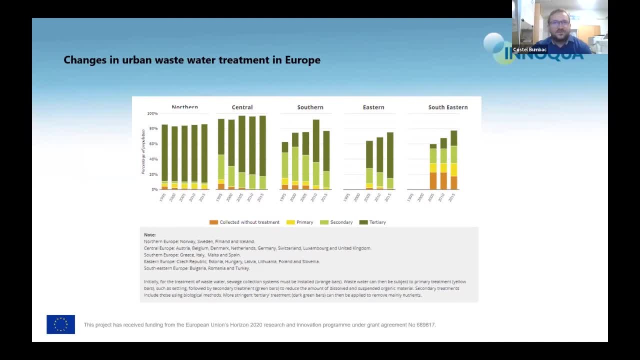 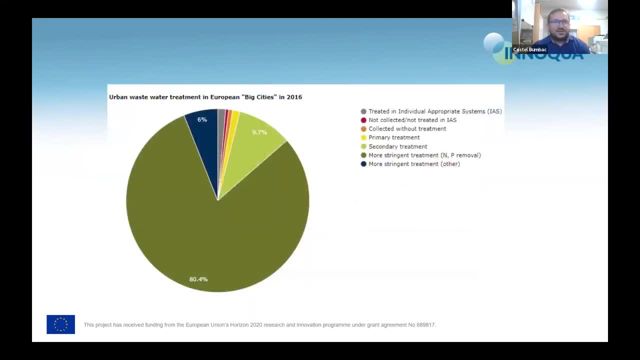 Implementation has been strongly supported by European Union cohesion policy, with impressive funds provided for the wastewater sector since 2000.. This chart summarizes the type of treatment applied in the urban wastewater treatment plants of big cities in 2016.. Where big cities mean urban settlements of over 100,000 people and urban water resources. of nawet 15,000 people, 50 000 people equipment. of the total load generated by larger cities, 86 percent receives more stringent treatment, typically to remove nitrogen and phosphorus, and may also include disinfection, while 10 percent of the total load receives only secondary treatment and one percent 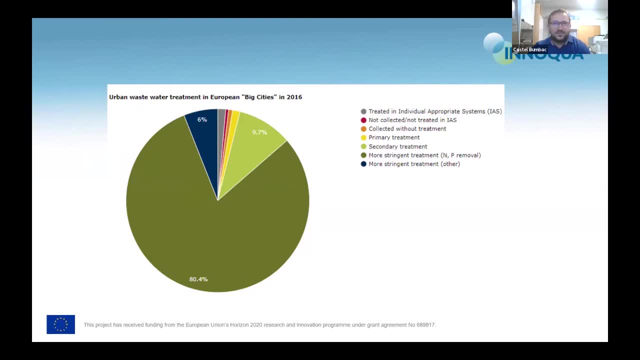 of the total load of all big cities receive only primary treatment, while less than half percent is neither collected nor treated. the large and medium-sized population agglomerations were the first team being provided by treatment infrastructures according to the directive schedule. meanwhile, the smaller population agglomerations with less than 2 000 population 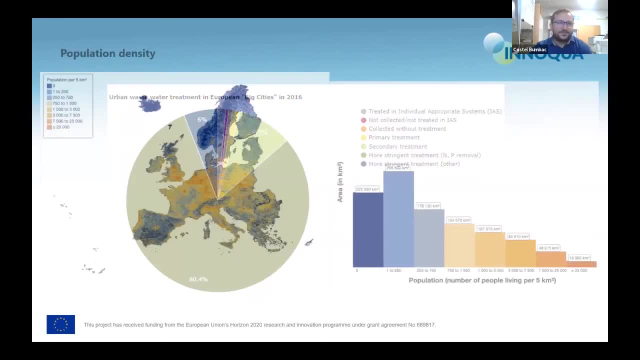 have been pushed into the background. the european 27 was 109 inhabitants per square kilometers in 2018. almost two-thirds of it's a very sparsely populated characterized by a population density less than one-third of the european average, which is marked in blue. 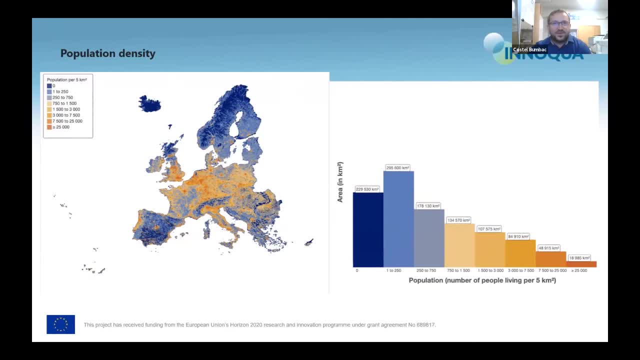 on the other hand, less than 10 percent, as shown by the two darkest shades of orange, were home to more than two-thirds of the european population, their average population density being over 1000 inhabitants per square kilometers, or nine times nine times higher than european average. when there is a low proportion of 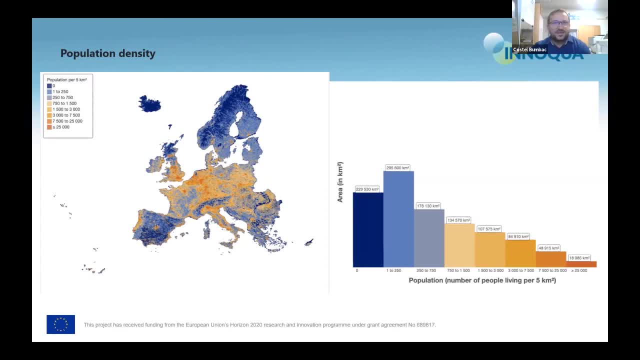 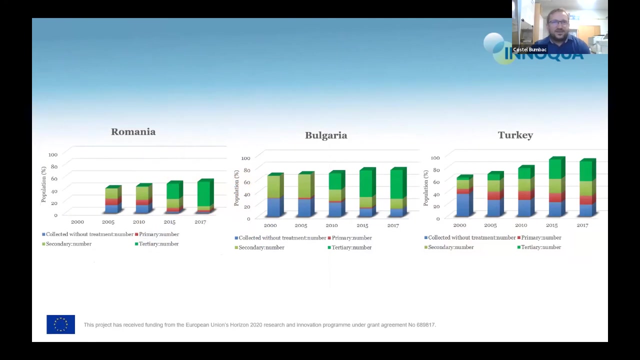 population connection connected to wastewater treatment facilities. it may be because of lack of financial resources or priority for providing sanitation services, low population density or too high a proportion of the population living outside agglomerations. this low level of connection to wastewater treatment system is caused by a combination. 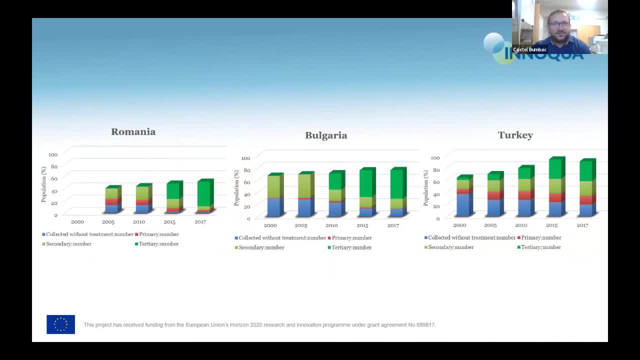 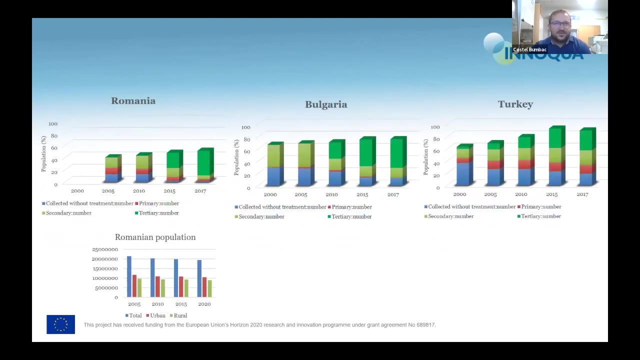 of the three factors mentioned earlier, especially the low population density and high proportion of the population density of the population living outside agglomerations. for the case of romania, approximately half of the population lives in a rural environment and only 10 percent of them are connected to central wastewater treatment systems. 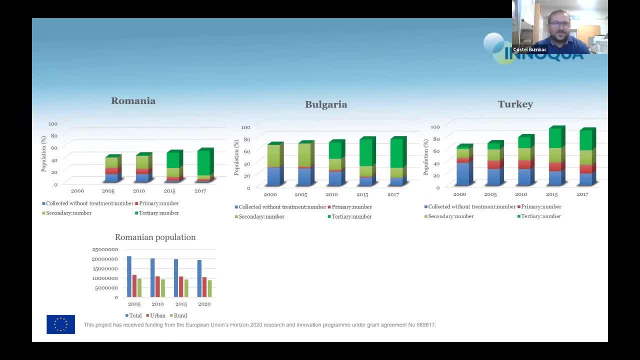 in dispersed communities, wastewater collection infrastructure may prove prohibitive in terms of cost, and the cheaper alternative would be the installation of several individual or group or group of wastewater treatment facilities in the region of the european region that are so close to the urban areas. so the goal for the district is to 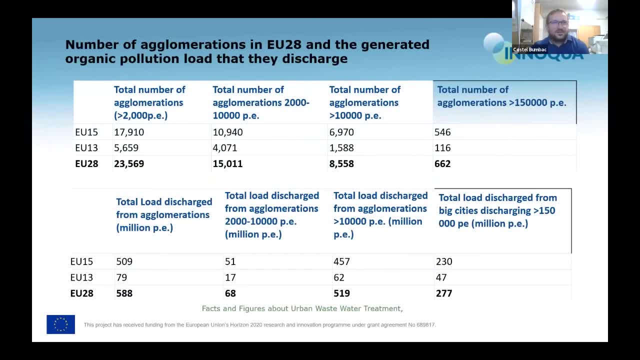 provide access to this to low number of water and to low level of environmental quality, but also at an even greater level, to ensure that the local Islands cannot be affected by the large amount of pollution as the city of arduous industrialization and ornamental pollution, and also facilitate the system adaptation of the local water and 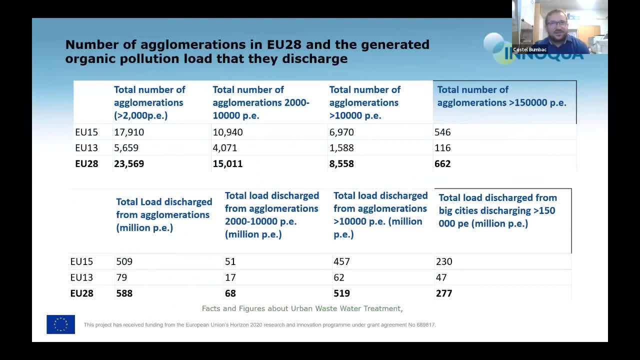 and the removal of the already dragging and not only the local pollution system, but also the local objectives and- why not? the United Nations Sustainable Development Goal 6, sanitation for all. A combination of drivers, including the utility market, restructuring water and wastewater directives and improved efficiency. have 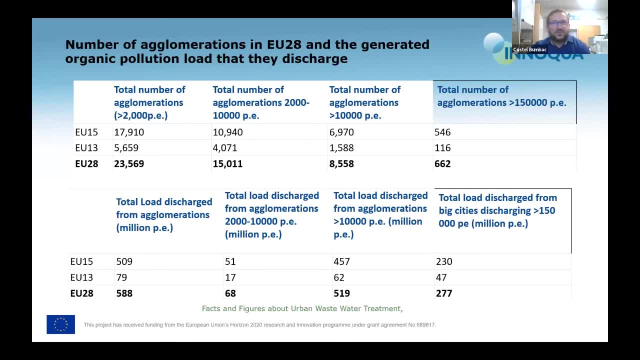 encouraged cities and public water utilities to resume the most aggressive investment programs Europe has seen since 2007.. Bluefield research anticipates annual water infrastructure investment to increase by 23%, from 46 billion in 2015 to 57 billion euros in 2025.. In many countries, small communities are. 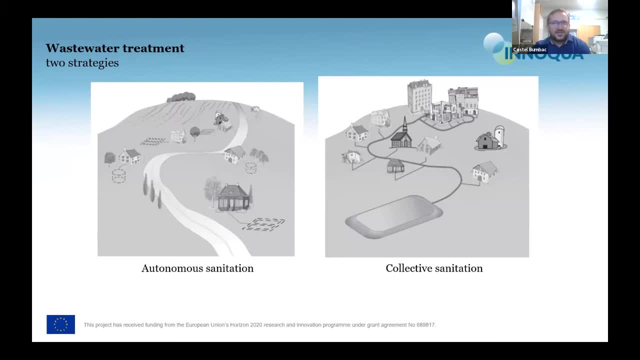 required to treat wastewater discharges to increasing standards of lesser environmental impact, but must achieve the goal that locally sustainable costs, While biological treatment, activated sludge or membrane bioreactors are quickly becoming the industry standard for centralized wastewater treatment plants and would also be ideally suited also for small plants. its investments 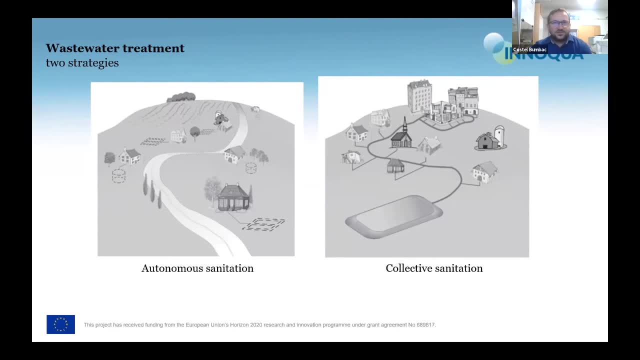 and operation costs are usually too high for that class of application. It is not always appropriate to connect to the public wastewater treatment system, for instance in remote areas or skydiving, for example with low population density. suitable alternatives to connection to the public. 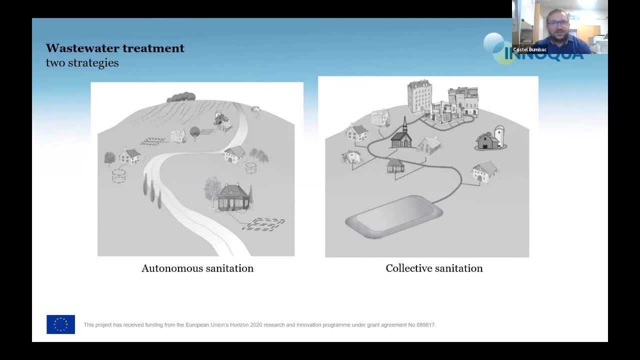 sewage system may include individual sanitation systems, package wastewater treatment plants or natural based solutions such as vermi filters, drain fields and even septic tanks, with the regular removal of solid waste waste would be better than nothing. Consequently, small treatment plants are better than nothing. Consequently, small treatment plants are better than nothing. Consequently, small treatment plants are. 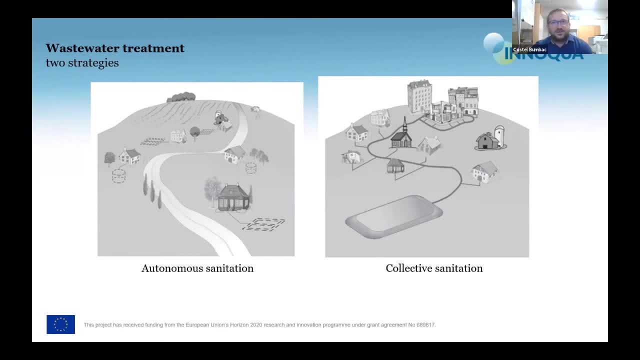 generally configured as anoxic or aerated biological tanks with little sedimentation, making them quite susceptible to hydraulic load changes, sludge quality changes and, consequently, performance loss. As ecological, on-site, low-cost and sustainable alternatives, natural based sanitation solutions may be used as being more reliable on longer term, such as vermi filters, drain fields, etc. 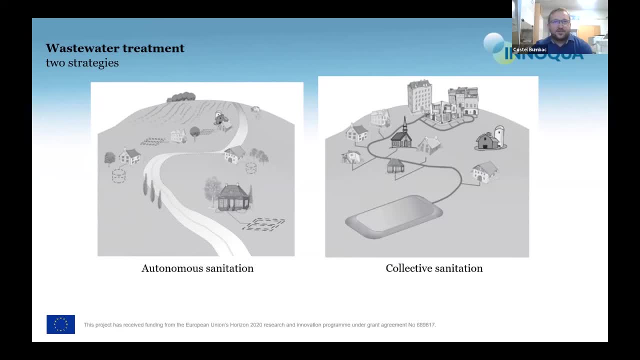 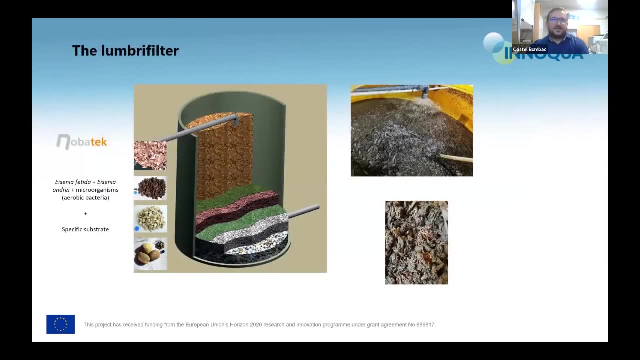 As ecological, on-site, low-cost and sustainable alternatives. natural based sanitation solutions may be used as being more reliable on longer term, such as vermi filters or constructed whelowing systems, which are gradually and successfully being introduced in some countries: The lumbree filter, as developed within 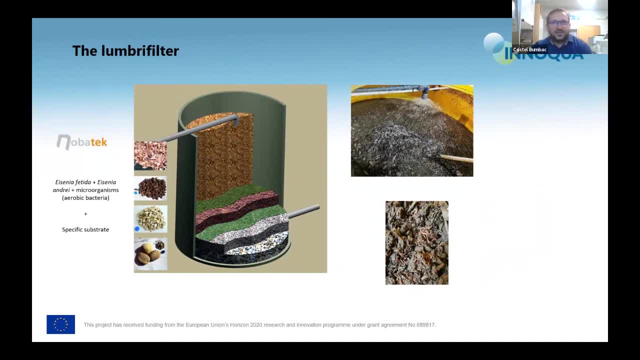 the inocua project is a reactor based technology operated as a treatment filter. The reactor is filled with successive layers of materials with different functions, from button to top. rib of gravels in 2 size ranges. as they feed from behind, different goes. 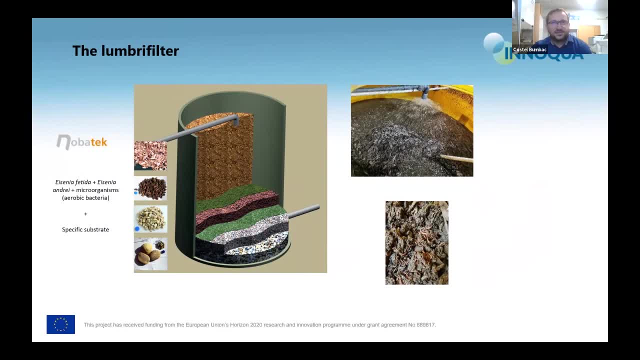 ьяйзros and streams can also所以 support wood chips or coconut husk chips or even wood shavings as active layer for microbial biofilm and home for the earthworm population. The earthworms we used were indigenous species. Mostly used have been Icenia, fetida and 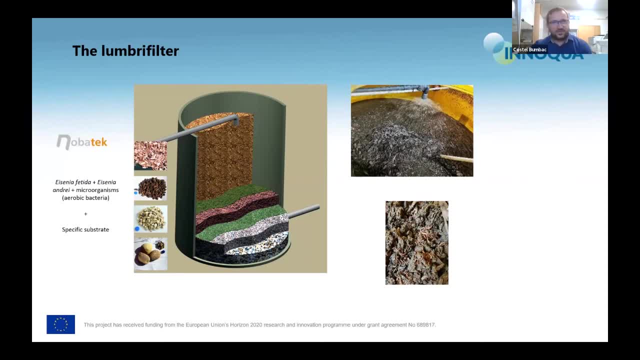 Icenia angrae. The influent is being sprayed on top of the active layer and passes through the active layer where bacteria removes dissolved nutrients, while earthworms provide the service of consuming the TSS and regulate the microbial biomass so that clogging of the system is avoided. There are many. 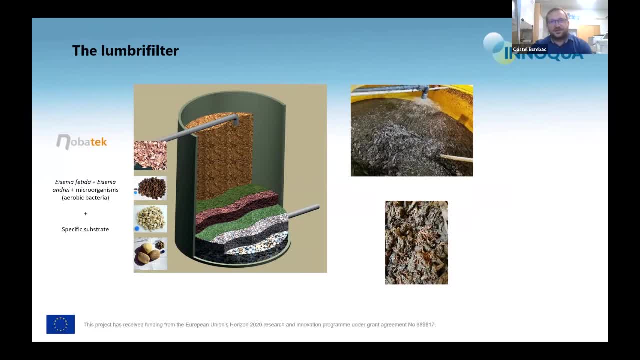 commercially available alternatives of the vermifiltration technology, including the Enoqualum Refinter, each with its specific advantages and disadvantages, and adapted to different wastewater quality contexts, able to meet various discharge standards. Constructed wetlands are designed to use the natural 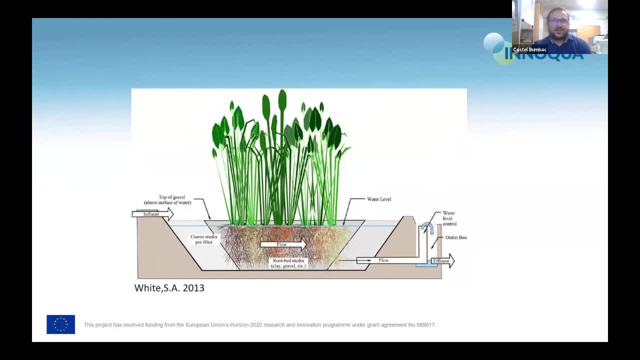 functions of wetland vegetations, soil and their microbial population to treat wastewater. Even though sometimes natural based solutions represent the more expensive approach for wastewater treatment, analyzing the merits and throwbacks of the various NBS in view of their sustainability potential might lead. 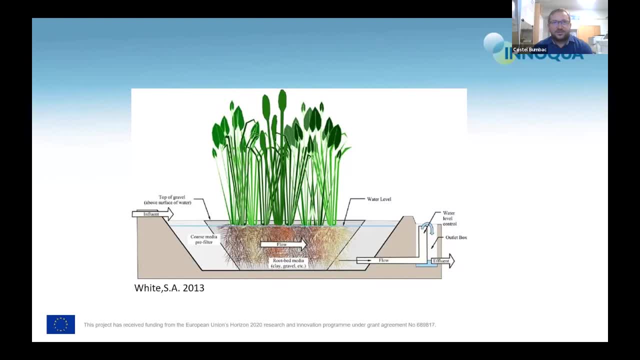 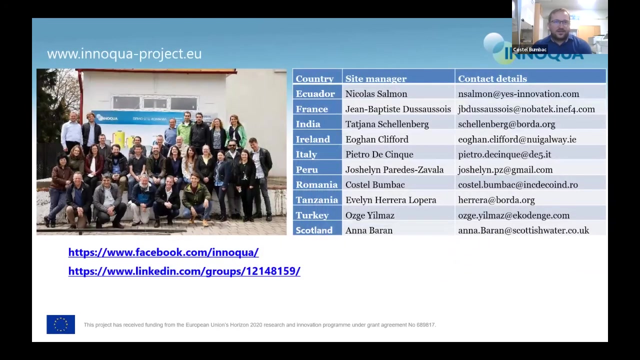 to the conclusion of a natural based solution could be the way forward towards the goal of sanitation for all, Encouraging the development of local water cycle clusters with local reuse and recycle of the resources and possibly local recovery of energy and or materials. This is the details. These are the details of the Enoqua project. 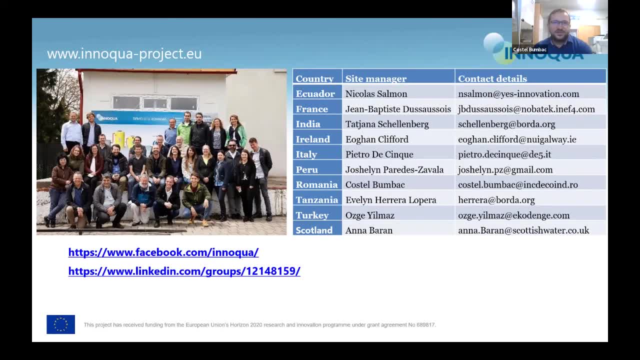 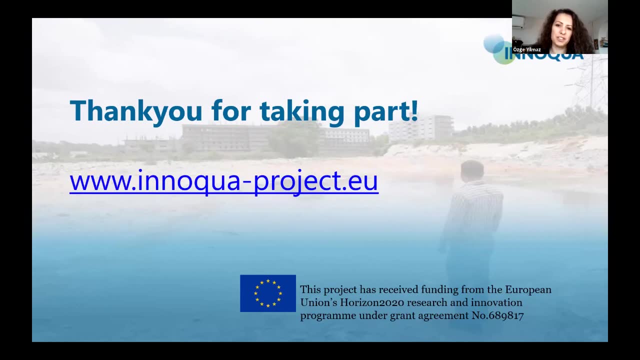 and I would like to thank the project managers and the project website and social media links. I would be happy to answer any questions if you have. We will also have some more chances for us to ask some questions to Costel. I don't know if there was anybody who would like to address. 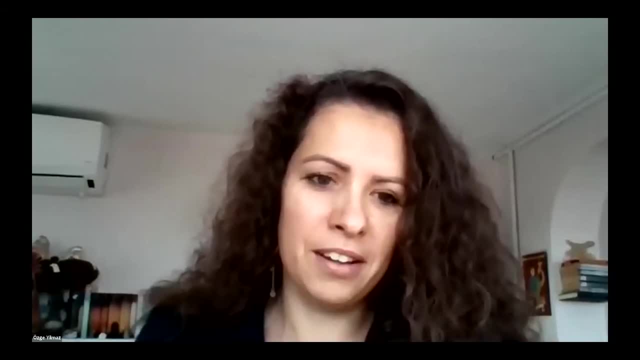 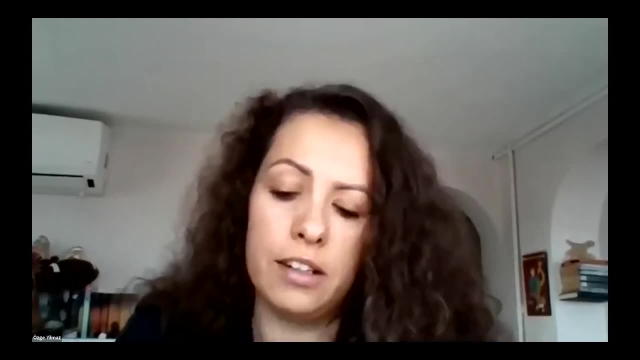 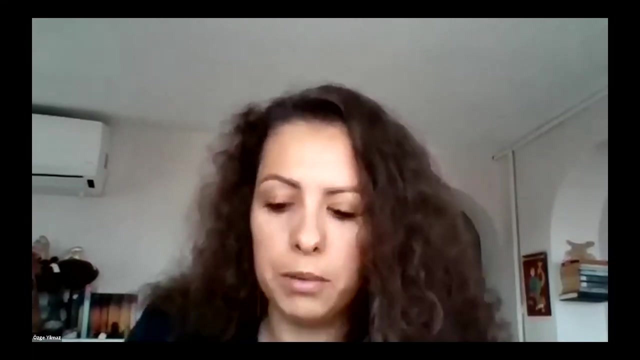 some questions at this point, If not Costel, thank you. I think this presentation clearly shows the ground. She raise a great effort to work on sustainable and affordable solutions, especially for dispersed communities. So, in an attempt to tackle this problem in a project, investigates applicability and 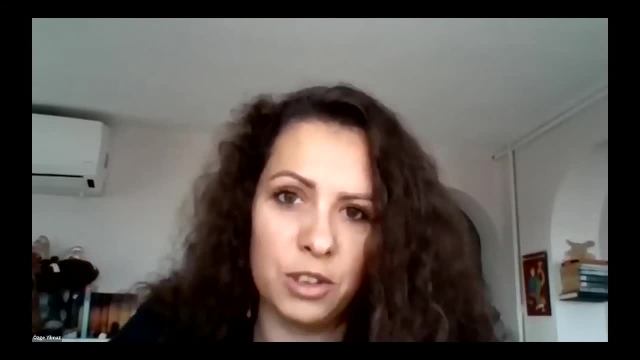 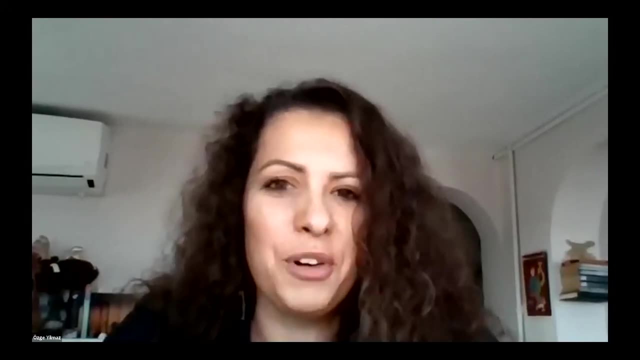 potential for nature based decentralized solutions. So I would like to welcomeanti Jim and Adele, who is not only the project coordinator of Enoqua project, but also the deputy general manager for international strategy and business development at NOBATEC, in miles of F4.. to welcome Mr German Adele, Who is not only the project coordinator of in a car project, but also the deputy general manager for international strategy and business development at NOBATEC in F4.. It's a project your talking about in happen 403 for zg inlogo. working with them. 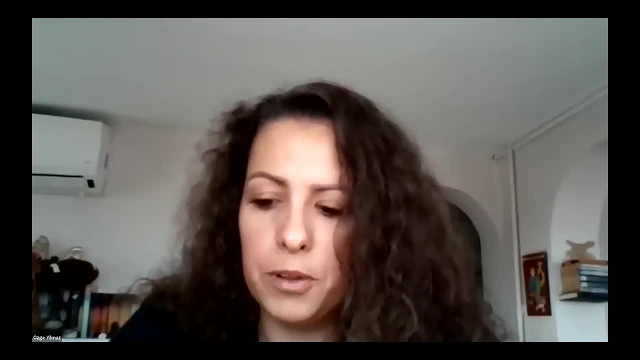 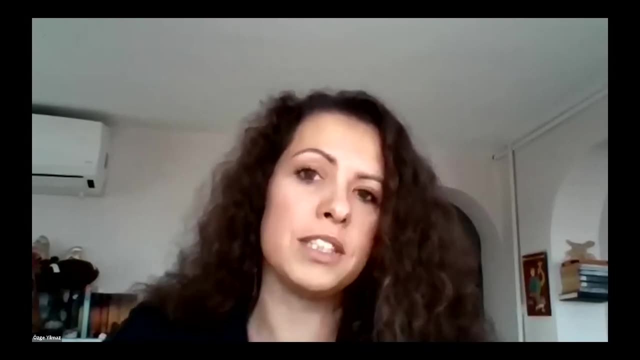 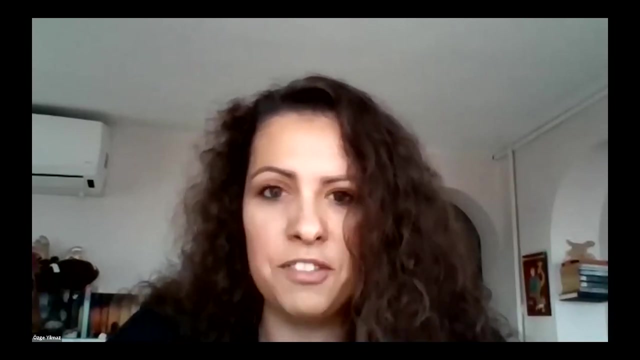 It's a private RTO that aims to co-develop innovative solutions to assist construction sector for greater energy efficiency and sustainable design, And he will be introducing in a core project and its demonstration strategy that we applied throughout the project itself. So, Germain, the floor is yours, Thank you. Thank you very much, Özge. 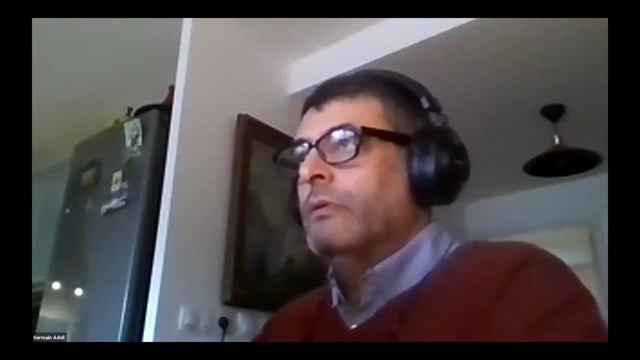 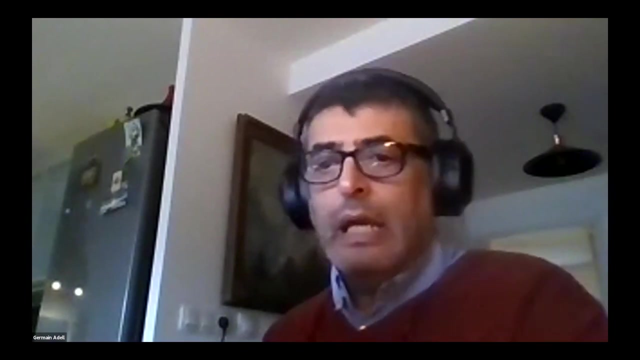 Good morning to everyone. So well, as Özge has said, the intent here is to explain a little bit our approach, Let's say I would say, our innovation approach to this project, So how this project came to reality and what was the, what was the general intent and the general strategy of? 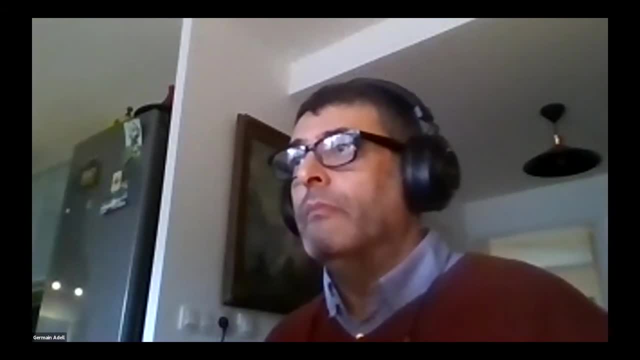 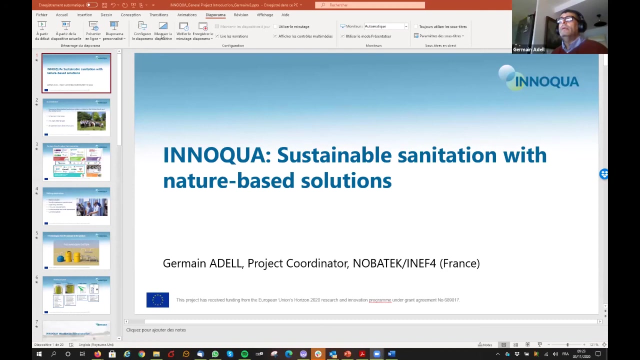 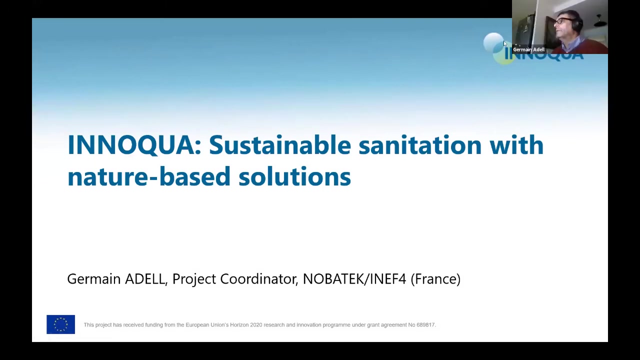 of developing a modular biobased sanitation system. I will share my screen. I hope it works. Is that OK? Yes, it is OK. Here we are. I don't know if it's the right thing to do. That's it. 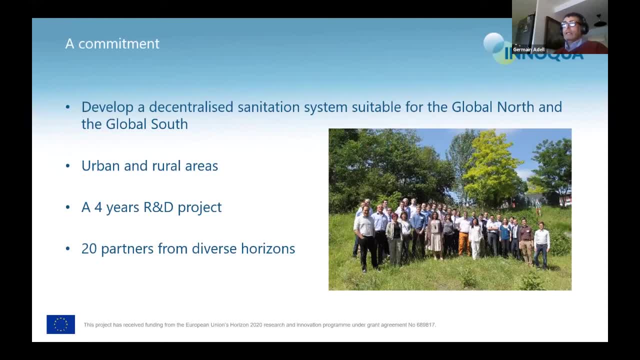 So so our commitment from the start, it was as we said before, and it's it's nice to have to have had a costal presentation before, because I think he has clearly demonstrated the interest and the need for such such decentralized sanitation system. 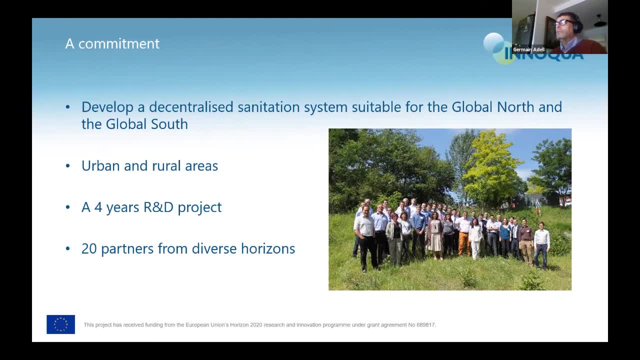 Not only in European context, but also, and perhaps moreover, for the global south. So we all know that the sanitation problems in, in, in, in big, in big parts of of the developed development countries. So we thought from the very start that this was really the thing to the thing to do. 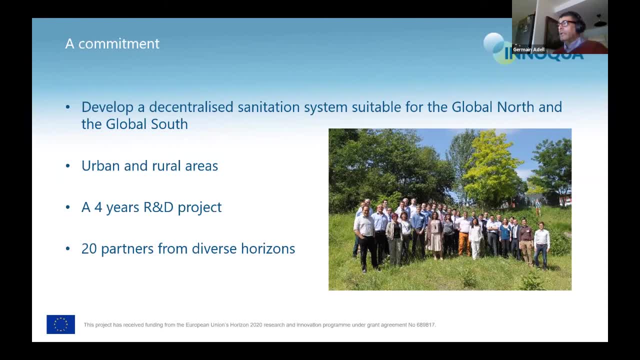 So, with the motto sanitation for all, of course, we were committed to to create a project that could deliver a very robust solution to that, But let's say that the the the history of the project is that well, of course, this is an horizon 2020 project, as you see in the bottom of the slide. 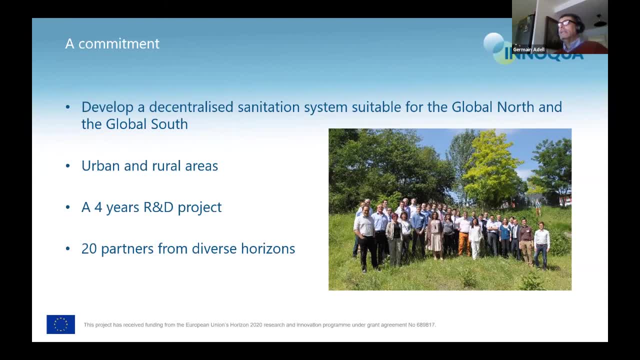 The first, the first, I think it's important to know, I think it's important to know the internal history of it. So the first, the first attempt to to to do this project was in 2012.. So we, almost with the, the same partners, we, we end up doing the project. 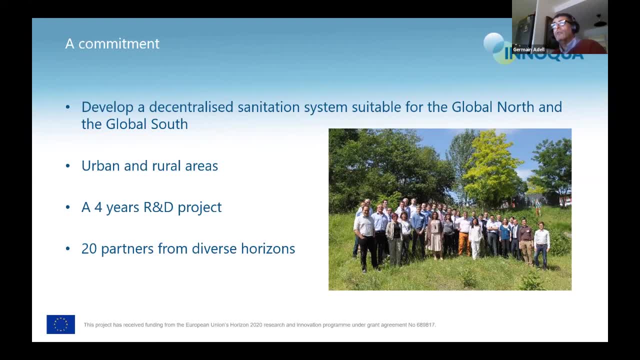 We, we tried once and so the first you know proposal and we were well ranked but finally didn't get funded at the time, And so we insisted in in 2016 and and at that time we, we, we finally got funded, and with a very little changes to both to the project and to the consortium. 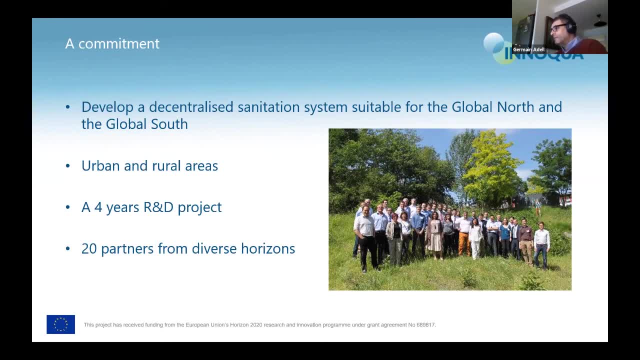 So so this, this, this, prove that if you, if you, you have something in mind and you know it's, it's true, it's, it's, it's worthwhile to, to, to try sometimes a second or third chance. Yeah, Because it can work. So this was. this is a four years research and development project. 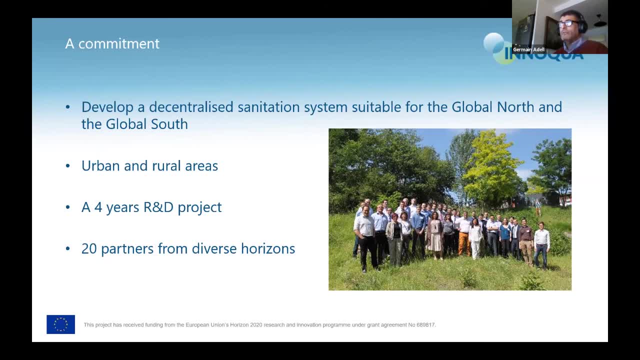 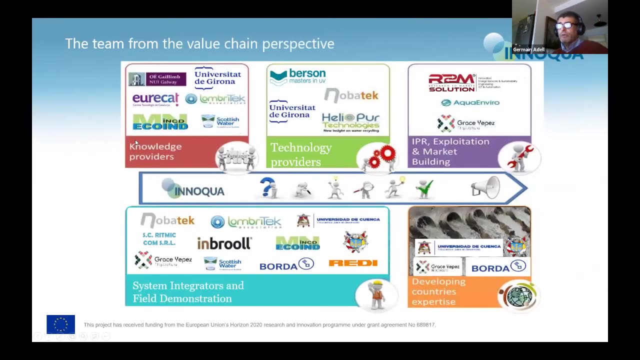 So an innovation action for for horizon 2020 jargon, And so this, this: in this picture you see we. we are 20 partners from quite different horizons And you can see in in all our projects we try to really develop the value chain perspective. 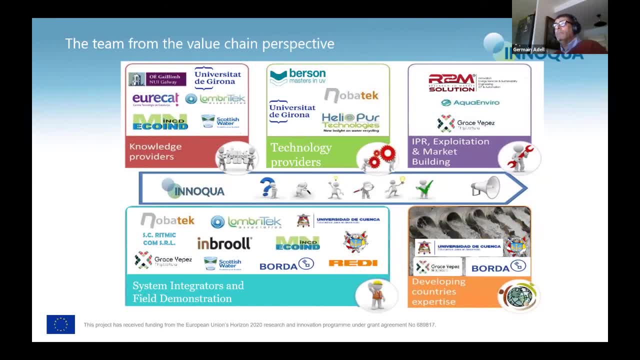 We we like sometimes we end up having very big consortia, But we we really believe that in in order to develop an innovation, you need really to have represented in the consortium all the value chain, because each actor from different sections of the value chains will will bring knowledge, needs, requirements to the to the project. 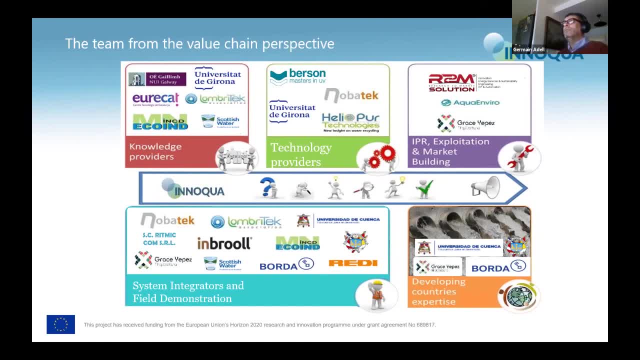 So you don't take for granted anything, Because you have the specific representative in the consortium that that bring the specific needs. So we have. we have some RTOS as as as so as Novotek. We are an FTO devoted mainly to the construction sector, to to architecture, sustainable architecture, urban planning, energy efficiency, nature based solutions. 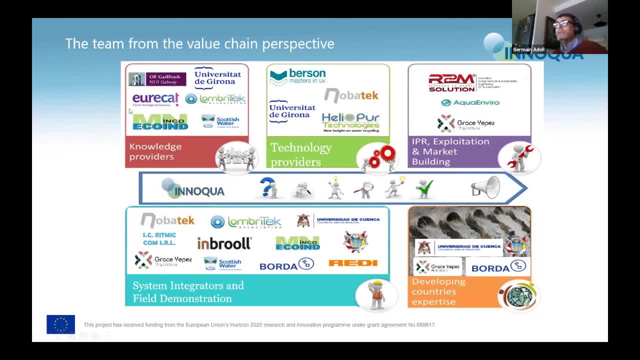 And also we have another RTO, which is, which is Eureka From, from Catalonia. We have some some knowledge provider And the other knowledge providers are also you. So we have a new IG University, got a new IG Galway University and Girona University. 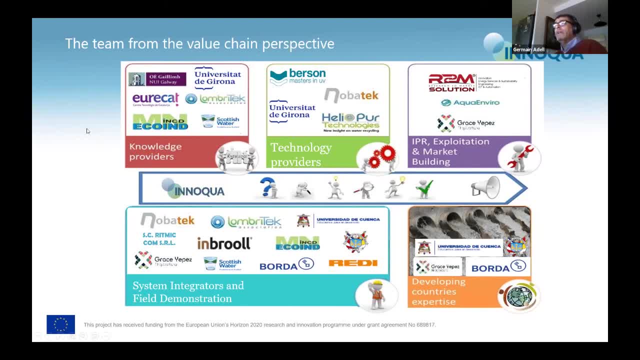 So some knowledge providers don't be taken, which had developed the lumbar infiltration knowledge during the years, And they coined also another LTO from Romania, From which coastal is Is the representative. Then we had technology providers. So, because this is a modular system, 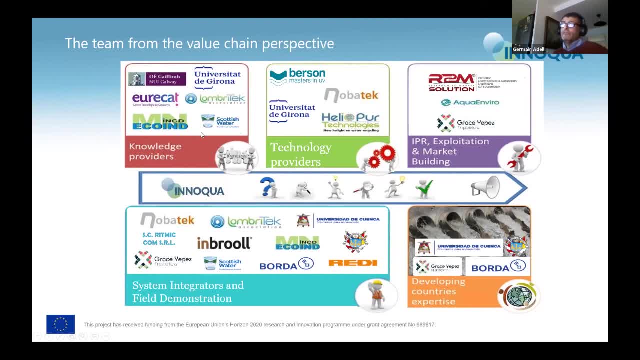 So we join effort at the, at the, at the moment of of creating the, the layout for the project. We, we, we found out that we have, we, we were some technology providers trying to push our systems And we, we end up thinking and creating a project where, in a modular way, 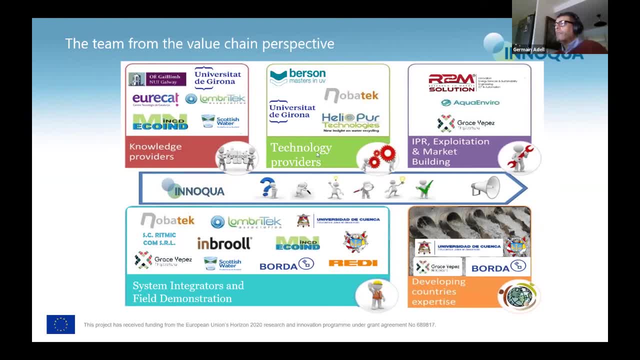 We could really put all of them together. So so basically no, no. but tech with a number of filtration, University of Girona, with with the Daphne filter, Helio pure technologies, with with the bio solar purification and Berson UV, with with already in the market. 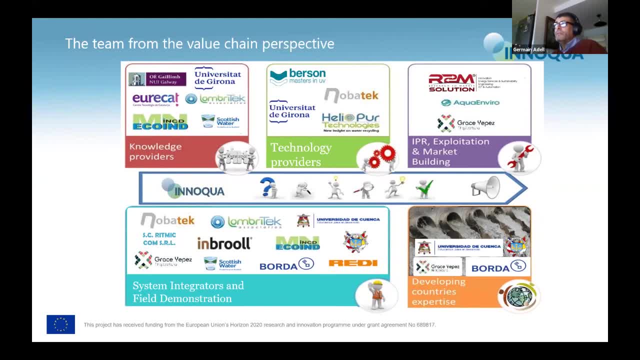 Ultraviolet technology to end up the purification process. So also we had specific, specific partners bringing exploitation and market knowledge. I circled solution at one video and and yes, innovation We see up is from Ecuador. Then we had a lot of integrator, integrator. 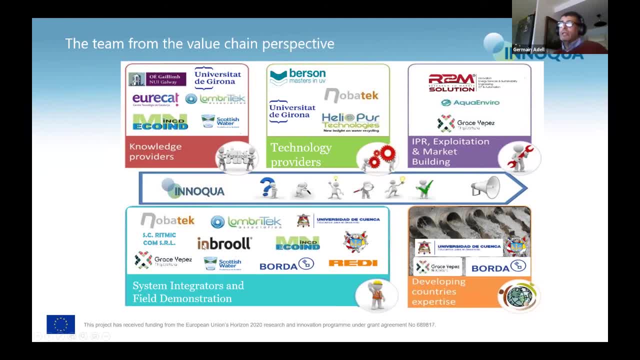 So we, we have integrated each, each, each, each module in in a full Almost, I would say, industrialized system. We are not at the end of the project, We are not fully fully scale up System, But I I mean we cannot just right now go to the market. 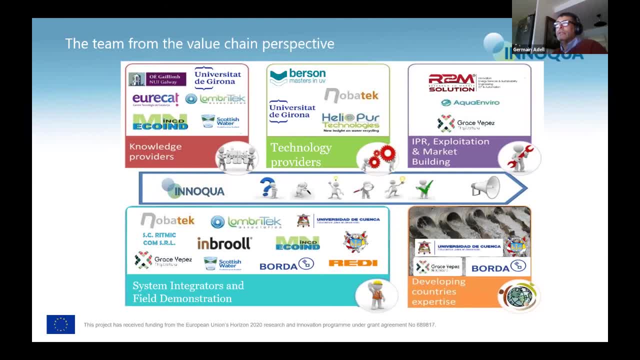 But but we we end up the project very close with some of the technologies, very, very close to the market, And this is also thanks to ready So which is an industrial, an Italian industrial For for from the sector Of of sanitation. So if they are a pure player in in in sanitation system, 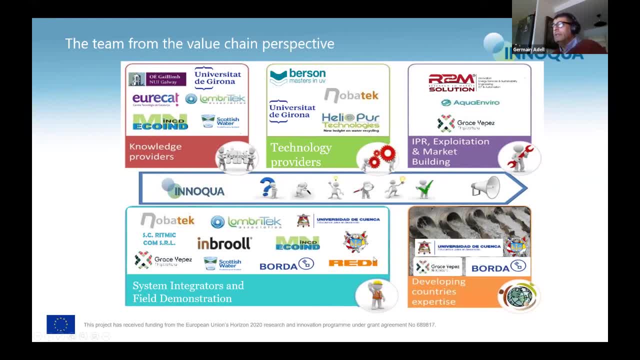 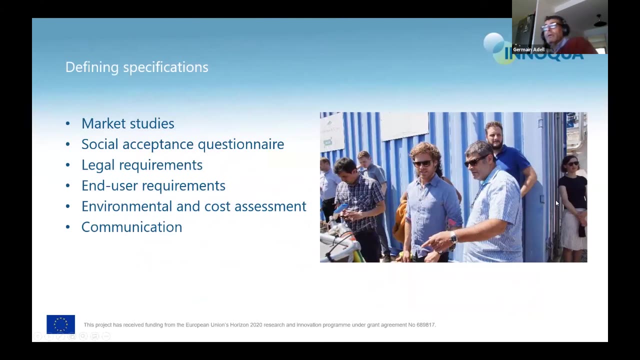 Also, we had some partners bringing developing countries expertise, as you say here. But at the end of the day, you see, the, the, the consortium is quite balanced with different kind of expertise and knowledge. So to the to, to, to develop the, The system. Of course we need not only 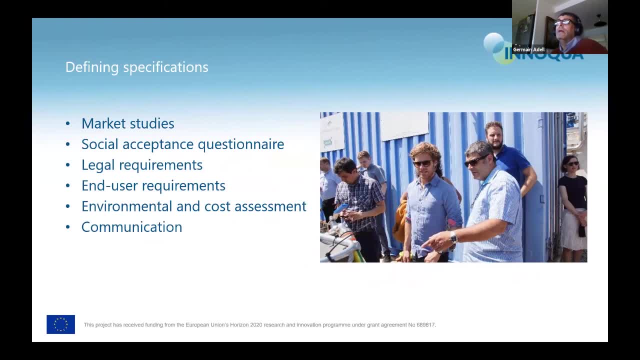 The technologies, we are bringing in the technical aspect. But of course we have to, We have had to to devote some time and effort To define the, the, the specific, the adapt specification, Not only for the general system but also taking into account the context and the market context. 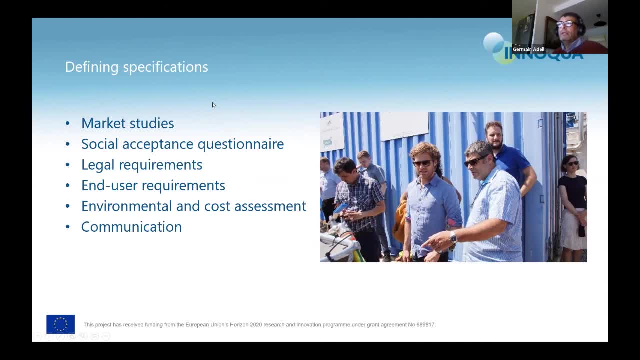 Of of of Our possible System for for each of those contexts of these include market studies, social acceptance, Legal requirement and user And elicitation of requirements, even even participation of of of of the local population and taking into account their needs And, of course, the environmental and cost assessment. 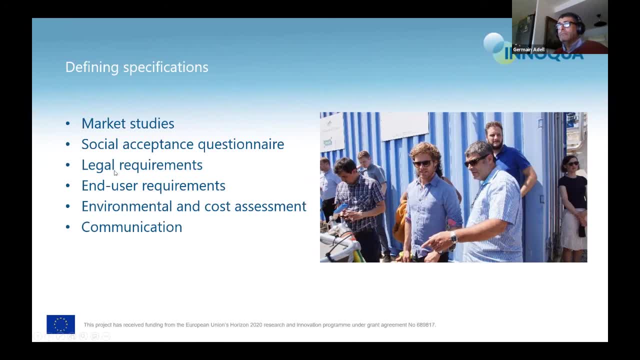 I have to say that this, this, this system. One of the main Features is that that is, the- the environmental impact is is really is really low, Because mainly the we- we produce a very, very slow amount of sludge And and, and also they are natural processes, as this one was one of our main features and we have been able to confirm. 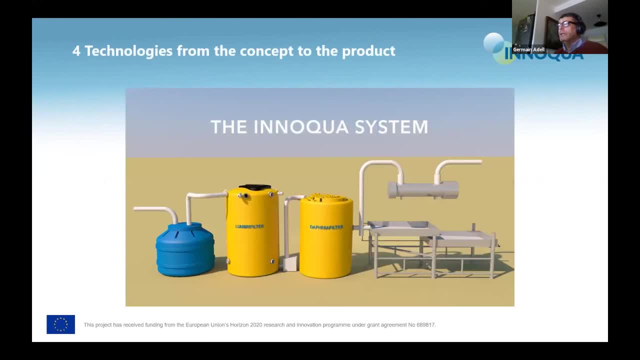 That this system works well in in that sense. So we have four technologies And and from that we brought from the concept to a, To an industrialized product. So you see here The number filter that I'm, the filters, The biosolar purification and the last stage with the UV, the UV filter. 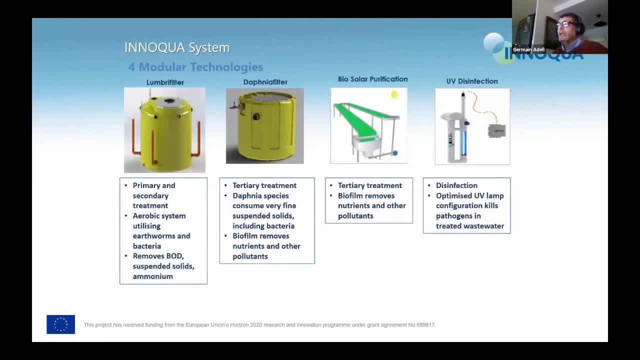 So here are the, here are the technologies. So I want I won't comment A lot on them, But while the number filter has been Presented by by coastal, But it's a primary and secondary treatment based on, based on The, the, the, the activity. 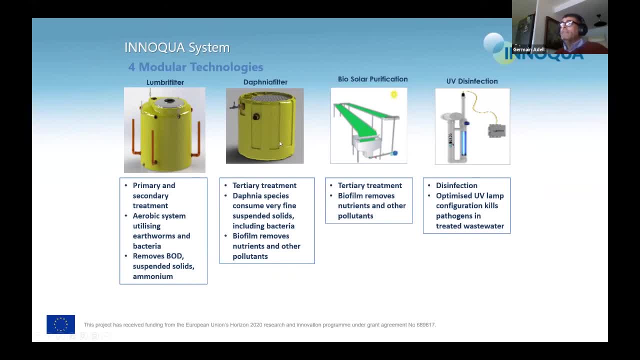 Of earthworms and bacteria, The Daphne filter. So it's, it's, it's a tertiary treatment. So for us, We had the modular technologies, where we have always had the lumbar filter as a first stage. Then we have Daphne filter, with Daphne. 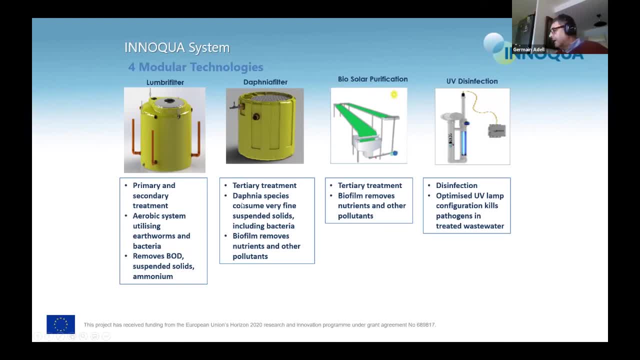 Daphne is a little, Are a little crustaceous, That that That can consume. So they they feed, they, they feed themselves with a very fine suspended solid And And then. so we have the alternative of use Daphne filter of or biosolar purification. 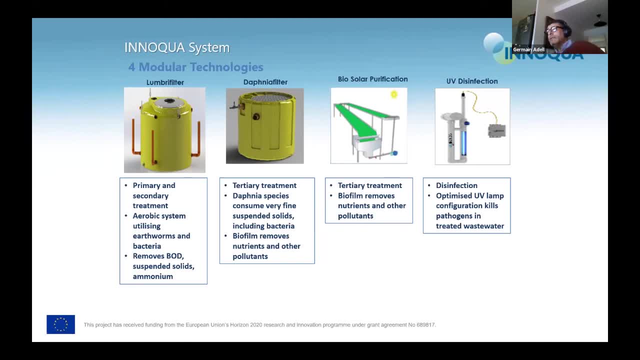 Which, which was a is, is an innovative, innovative treatment, You see, using the, the, the, the solar activity and biofilm, Of course. biofilm, micro algae, That that removed some, Some nutrients and pollutants And then, when needed We can, we can have at the last stage, 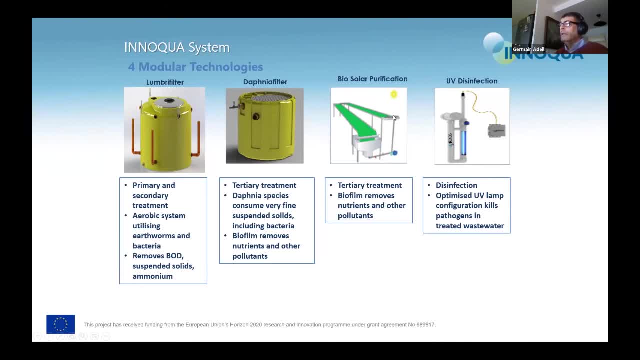 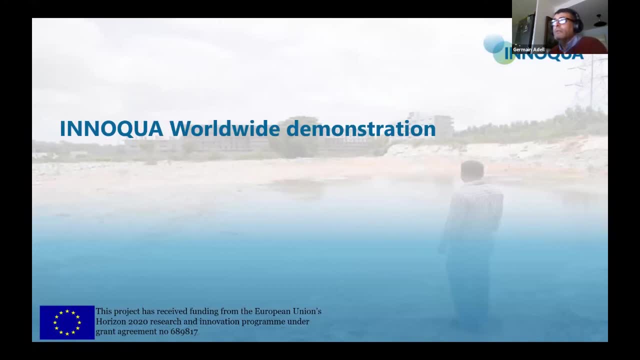 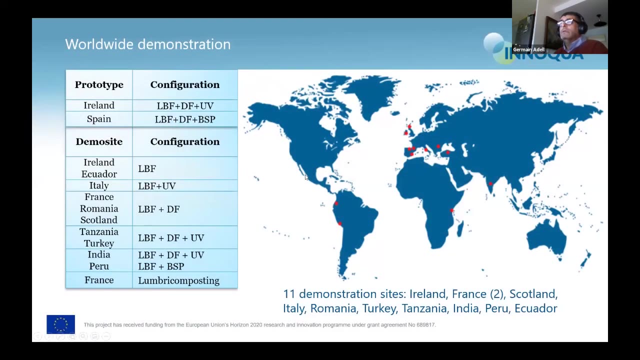 The UV disinfection. So all this makes a modular system That of course, at a certain moment we have. we have had to plan how we demonstrate it. So here you see, This was already demanded or suggested by the topic. at the time, The topic suggested that we could use invite extra European partners. 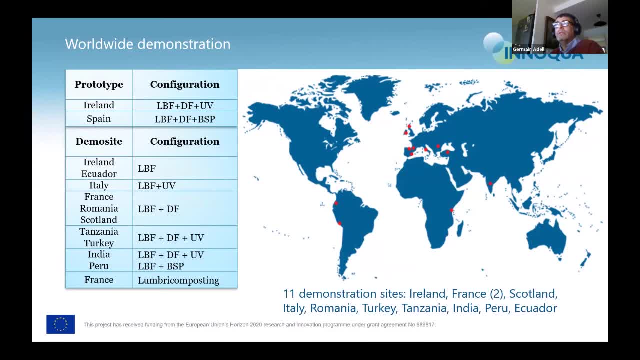 And so we, we really did that. We we went for that because we consider that the sanitation is a global problem. So, at the end of the day, we ended up with a strategy With, with which was twofold. First of all, we started. 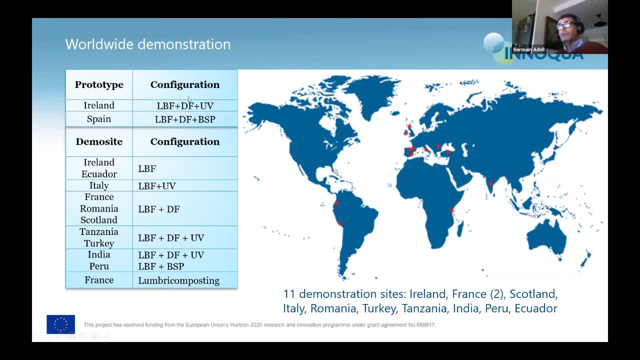 With a non control, A control- Sorry, I control the environment- Testing and development phase That was performed both in Ireland and Spain. In Ireland but in UI Galway, So National University Ireland, Galway, And in Spain by University of Girona. 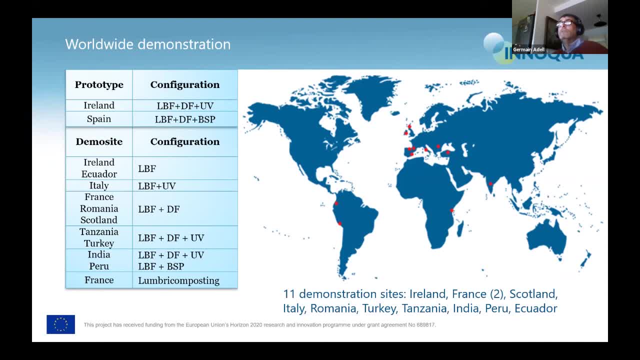 So there we installed The first prototypes of the system, The first the full modular system. We're installed there In a control environment. That means that we could really control the quality of of the water And and we had a full source of local wastewater sewage system. 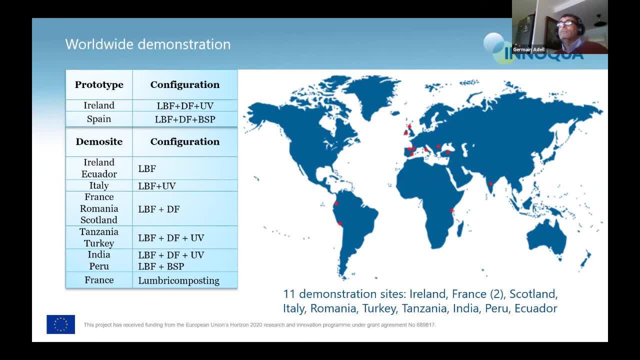 Bringing the water to, to our system So we could control the, the, the input And and also, of course, controlling the output very closely, Making necessary changes to the system Before. So this, this started before The, the, the demonstration phase, Which, which is you, you can see here: 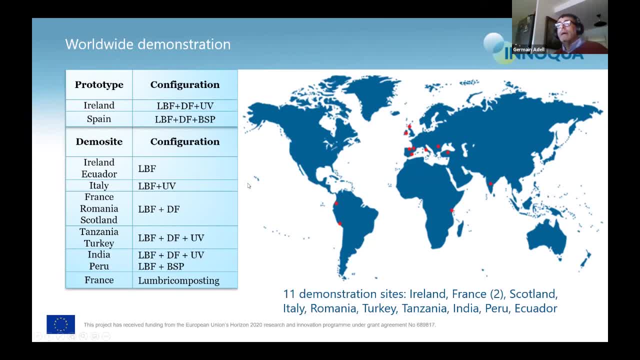 So we had. We have pilots In Ireland itself, In Ecuador, So this is lumbar filter And I'm in Ecuador, In Italy, lumbar filter Plus UV rays. In France, Romania, Scotland, We have lumbar filtering. 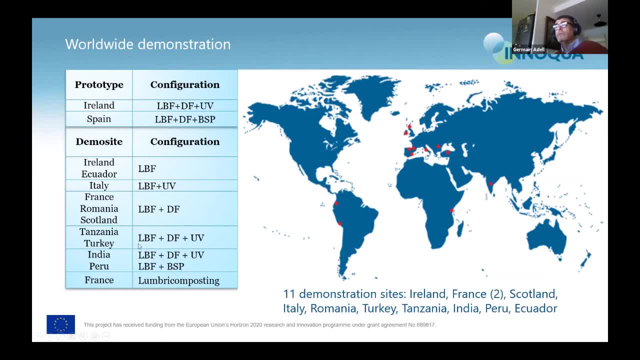 But plus Daphne filter In Tanzania and Turkey We have lumbar filter, Daphne filter and UV And what so and so forth. So these are our 11 demonstration sites And, as you see, Also it was important to. 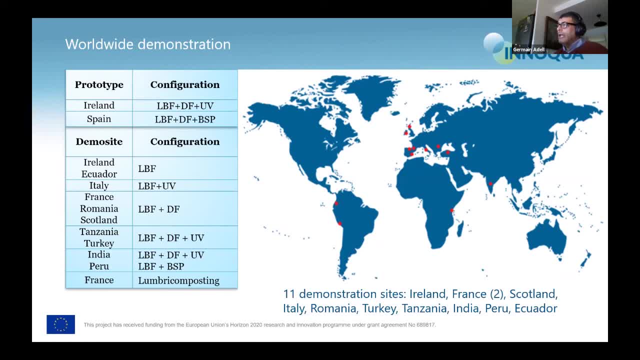 To check if our system was Able to penetrate, So to bring something interesting to different global markets. So you know, of course, Sanitation programs in India, Which which are really very acute, And also So we we had Thanks to border. 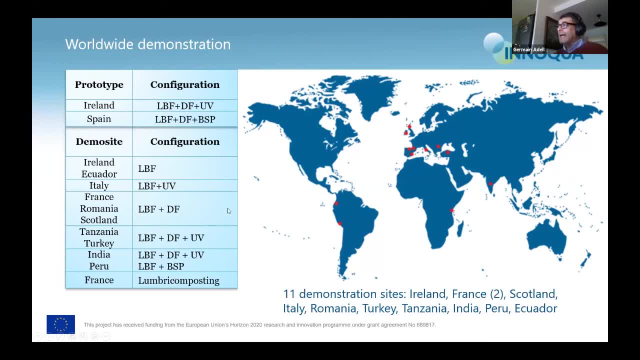 Which is a German ONG Active in developing countries. We have had The possibility to So to have demo cases In in India and Tanzania, And then also in Latin America and Ecuador and Peru. We We also have this. So this beside, 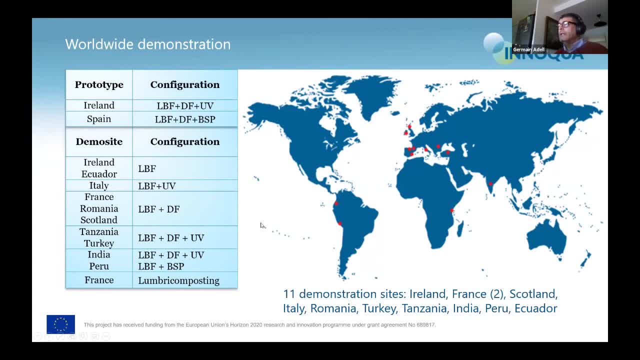 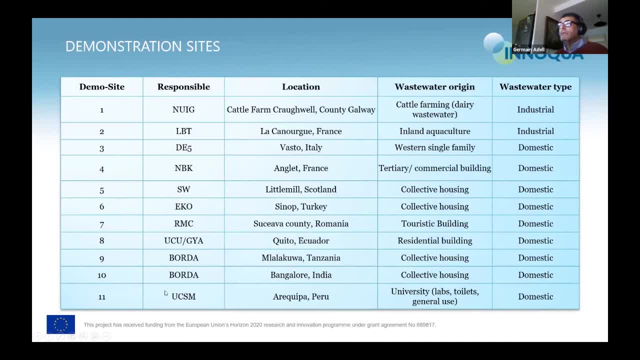 There are. There are. These are The site, What they have recorded for the shipping To be onBS. There is The partner responsible for them, Ple, Their location. There is what Their origin Under wastewater type Here. 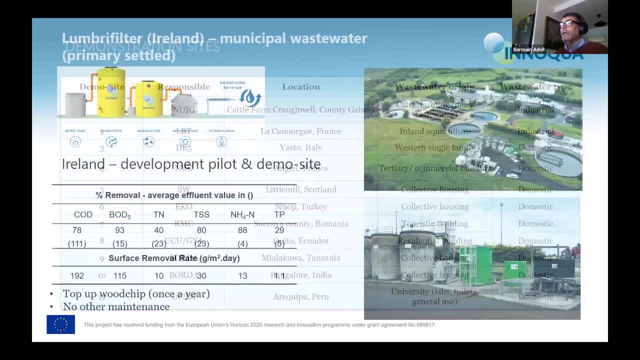 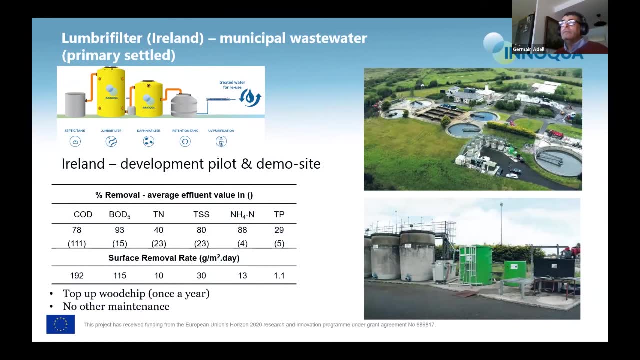 I want, I want A set More on this And so, as an example, I would just show some Some of the and the The demonstration and development cases. So this, This one Was internal At this, No IG premises. 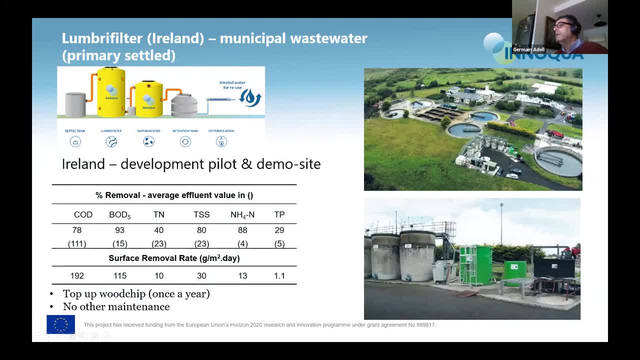 So here you, Ge, Даже, you have. you have it really close to a local sanitation. so urban scale sanitation system. so our lumber filtration you see there in in green. so of course we had all the wastewater we had, we we needed, and, and so the nuig worked in with the full system and worked, testing it. 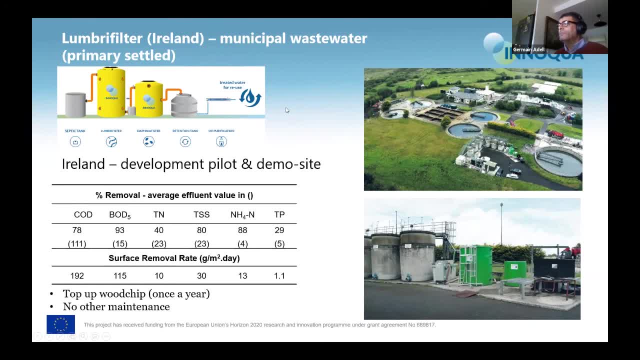 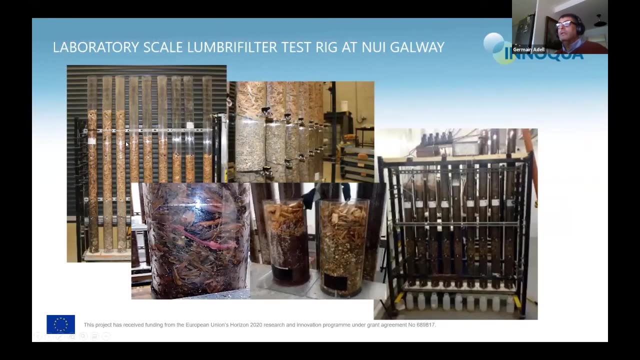 develop, developing the substrate and and let's say, gathering, gathering scientific information on on the system and testing different solutions. so here you can see what they worked. this, this was their testing of different layers of wood chips or or substrate. so it was really very, very thoroughly analyzed and developed by nuig. so we we ended up improving the first idea we had. 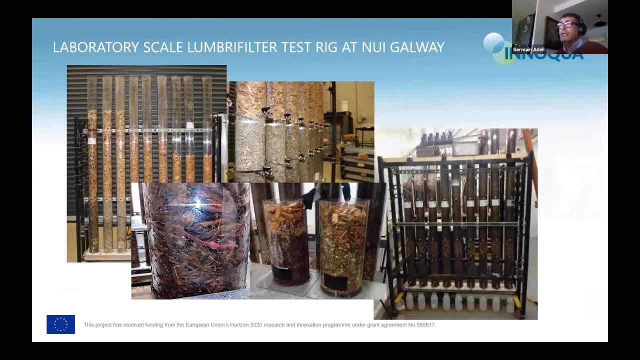 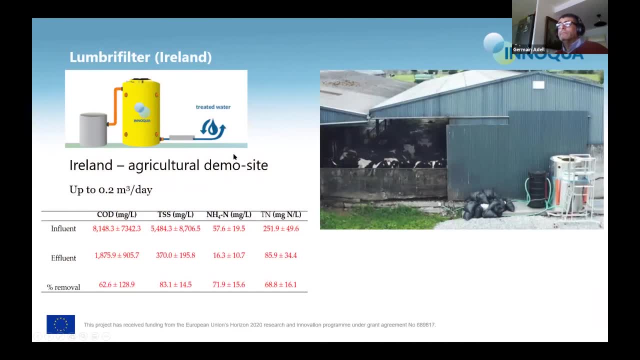 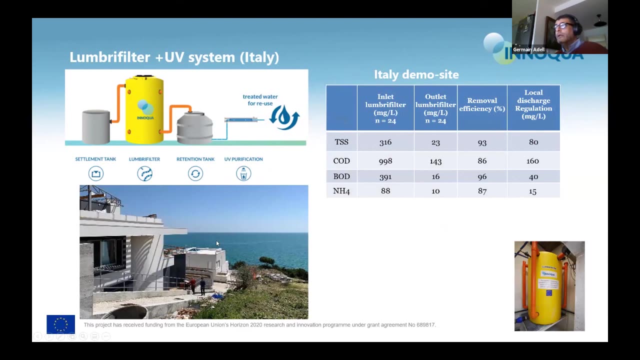 as technology provider, thanks to the help of nuig and other partners. they had also an agricultural demo sites, so cattle farming. this is one of the examples of domestic wastewater. so this is a villa in the seaside in in italy. so we have this configuration here. this is novatec. so you see our, our main building, our headquarters in in the south of 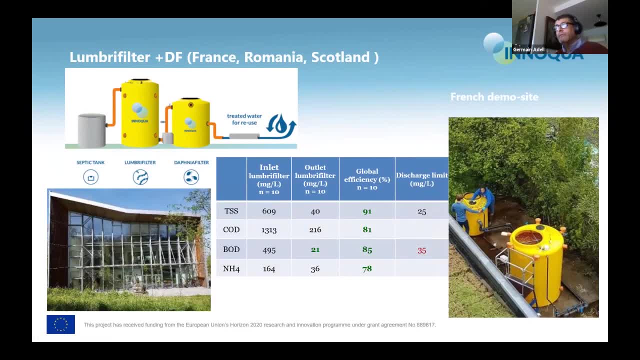 france. so we had we, we had this: the, the system installed, installed in our premises, so attached to a tertiary building, and here in the in the picture you see i am the project coordination, but i i have had these two projects in the past and i have been working on this project for a long time. 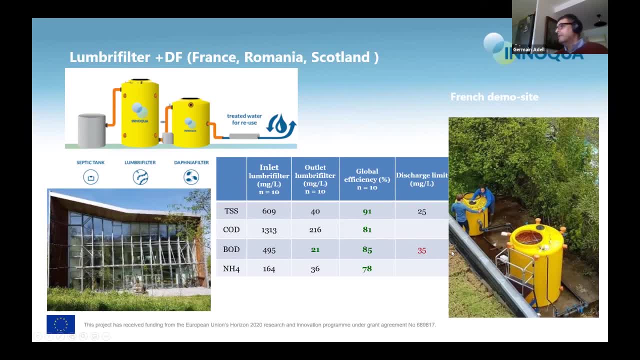 with two guys helping me: john batista, who which which has really be the project manager of of of inokua and and has taken the the most of of the project on on his shoulder, and and alex, also his who, who is another engineer working with him. so they couldn't attend today, but 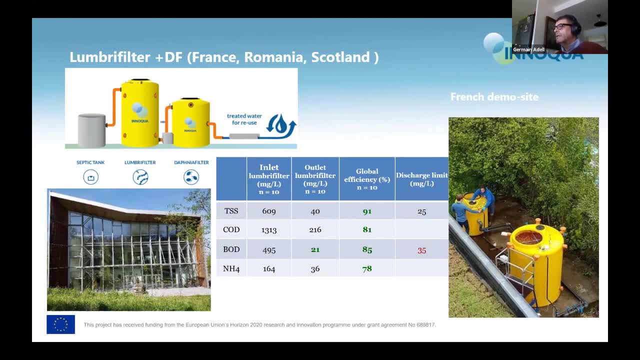 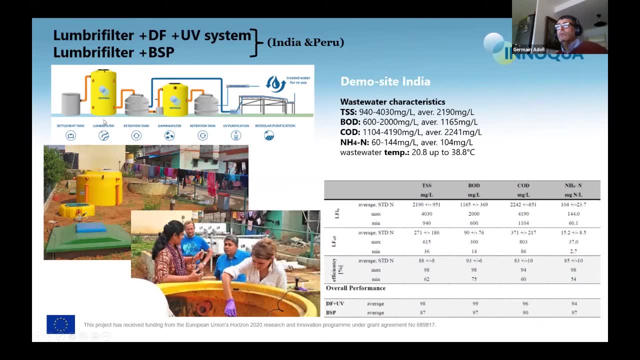 they were very, very, very good at at managing the project. here is the case of india, so in bangalore. so here you. you see it's, it's a, it's a complex solution where we had the lumber filtration, the daphne filter and also uv, uv purification and bio solar purification and and uv, so we have the full. 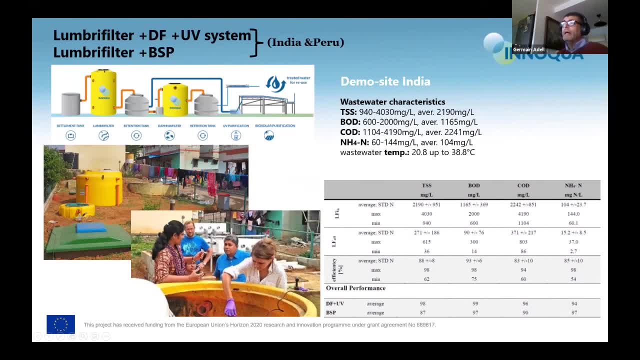 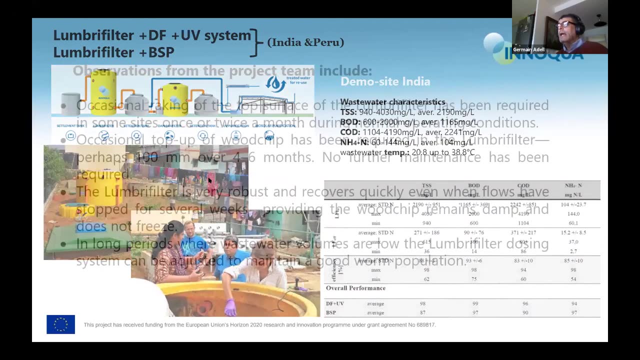 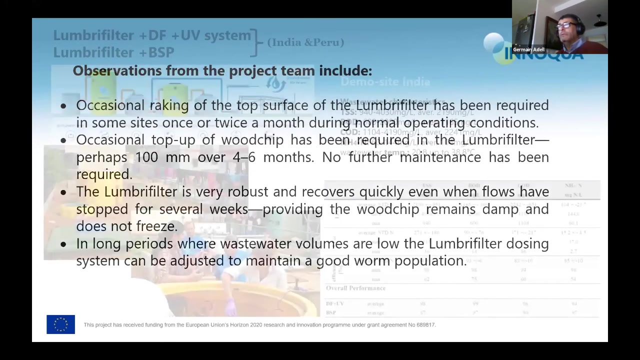 the full system working here, really nearby a local small domestic neighborhood. so this, this was a very, very nice uh pilot site. i i'm not commenting on the results. if you have any question, i cost will be more than able to comment and perhaps coastal you i would like you to comment. 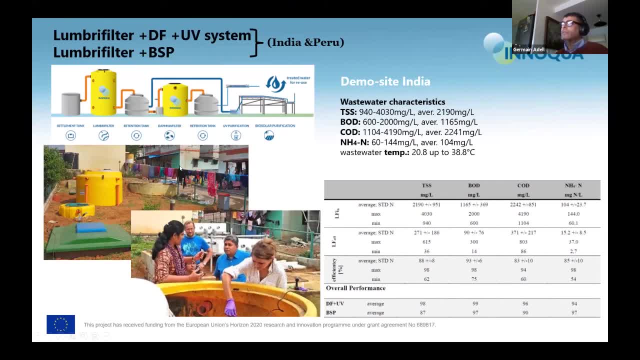 the. the last two slides are more the results of the of the pilot sites. if you don't mind, i i because you have been, because it has been the pilot manager of of india, the full project, and i think he's more qualified than myself to comment on the last two slides. 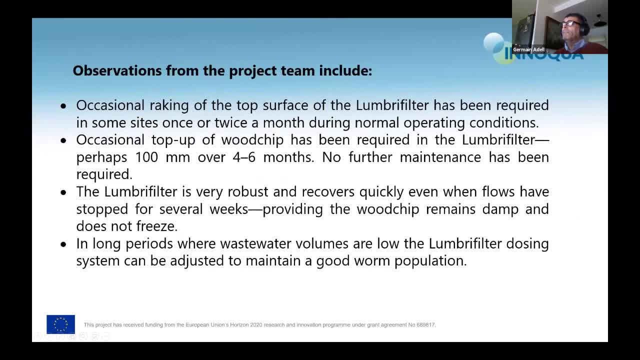 which, which are the summary of what the project team um found out after the the the demonstration phase, because, are you okay with that? would you like to comment on this? yes, of course, thank you very much, so i i leave you on the floor to these two last slides. okay, thank you very much. 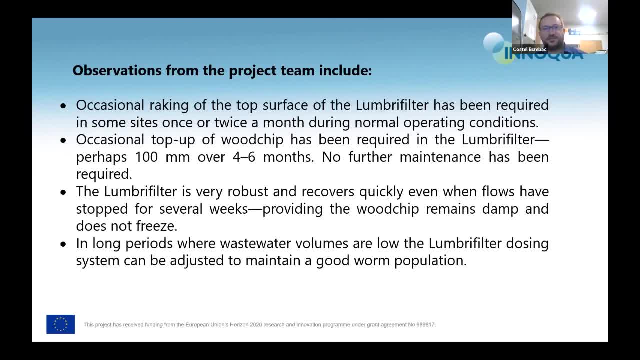 so the lessons learned from all the 11 demonstration sites were that, for the lumber kilter itself, which is the core technology of the project of the inocua system, the modular natural based solution we offer is that the lumber kilter is a very low maintenance system, meaning that within more than one year of operation, 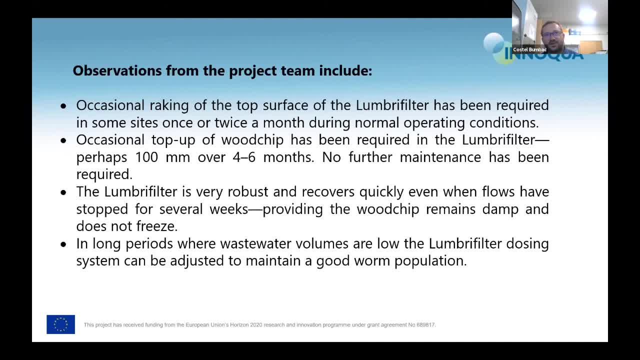 of the demo sites. in normal operation conditions the systems need only to be occasionally top up with the wood chips to keep the height of the active layer to at least one meter height, and also the lumber filter proved very robust in terms of hydraulic loads fluctuation large. 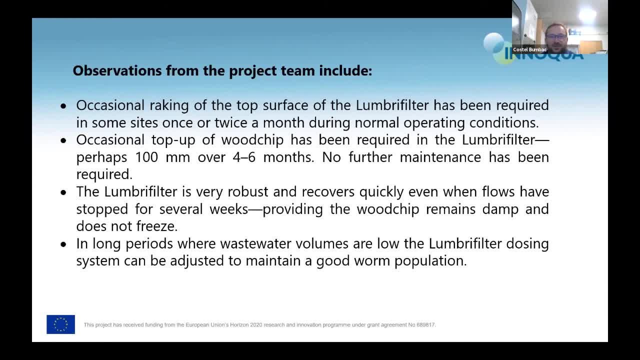 operation, meaning that it was able to cope even with the higher hydraulic loads than design- up to double the design parameters in terms of hydraulic load and also was the very robust in terms of no flow for long periods of time, as we had the opportunity to experience due to covered. 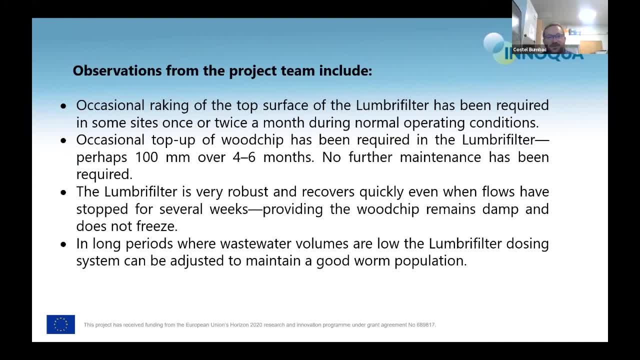 crisis. there were some demo sites where demo sites where, for example, in Novatec, the COVID crisis forced the workers to work from home, thus leaving the laundry filter at the Novatec offices without any wastewater for more than two months, and once the system was restarted and fed again, the performances. 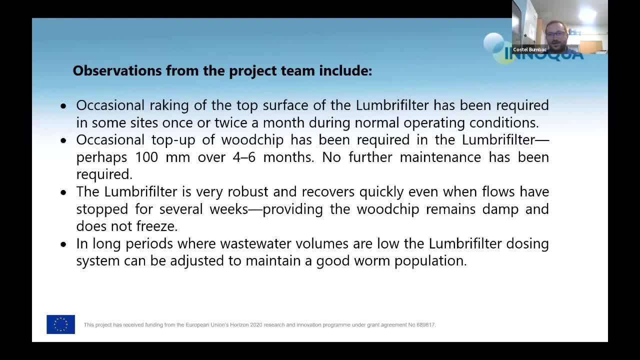 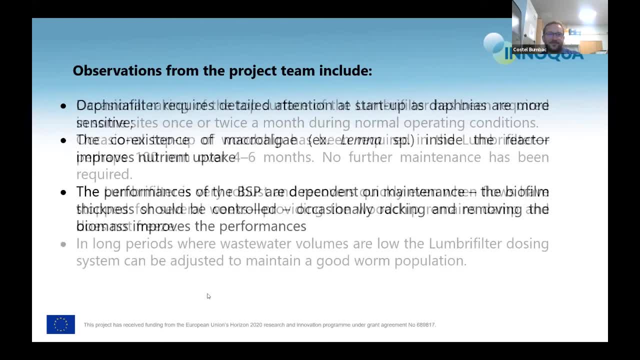 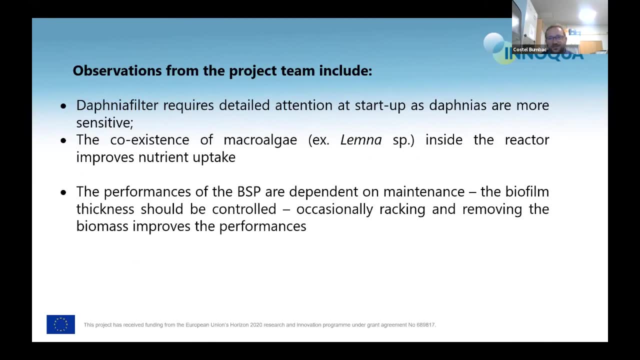 were recovered really, really fast. On the other hand, can you pass the next slide, Germán? On the other hand, the daphnia filter requires a little detail attention at startup. as daphnias are known to be sensitive species, they are usually used in ecotoxicity studies and at 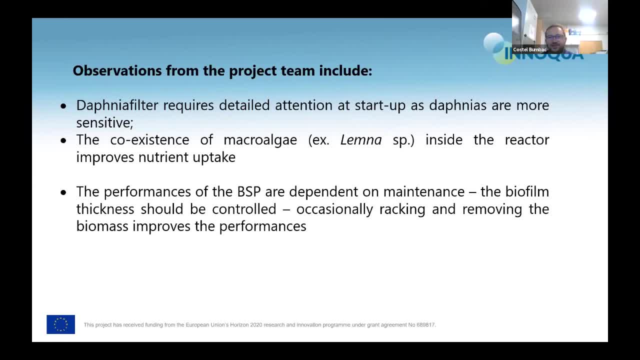 the same time, the coexistence of macroalgae or even water plants in the daphnia filter improves the reactor nutrient uptake rates. On the other hand, the performances of the biosolid purification which is the microalgae-based wastewater polishing step as module in the INOQUA system. the performances of the BSPE. 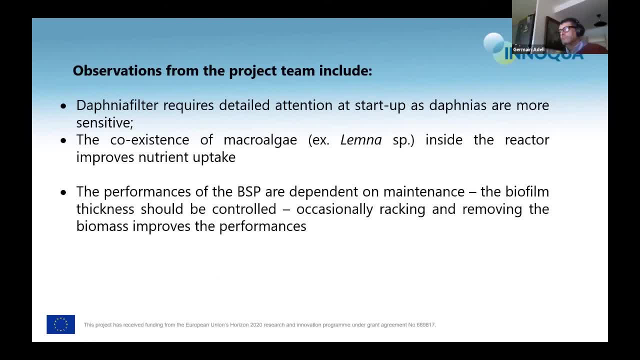 are dependent on maintenance, meaning that the biofilm of the microalgae biofilm should be occasionally racked and removed in order to keep the nutrient uptake rates, as the main mechanism of nutrient uptake in the microalgae-based wastewater treatment system is by biomass uptake. 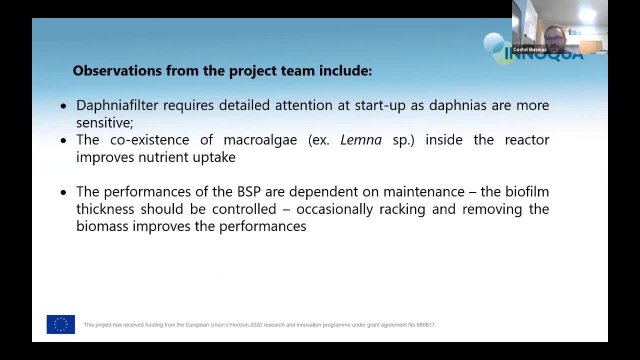 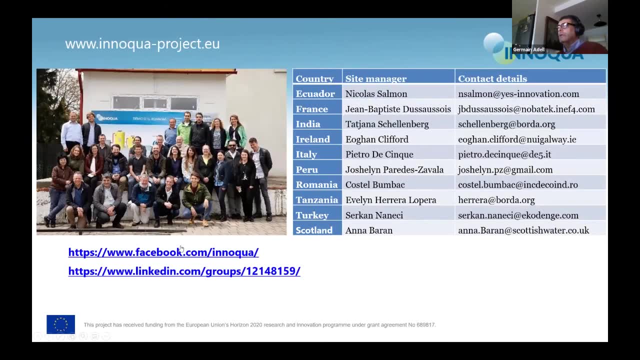 This is pretty much all. Thank you very much, Kostan. Thank you very much. Thank you. So this is it. So, here you have a picture of the full team in Romania, Our site managers for all the demo sites, and the final word is, first of all, as coordinator. 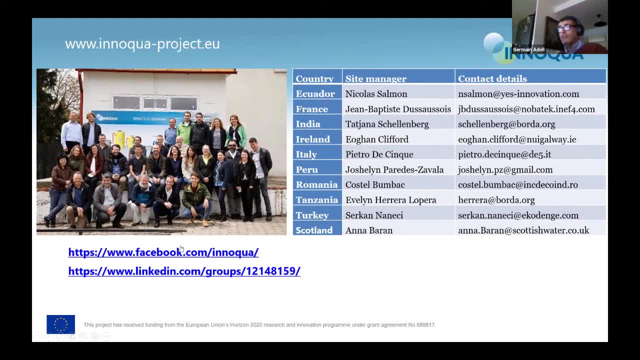 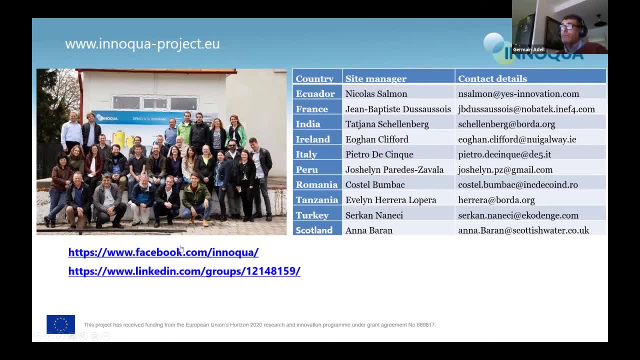 At the end of the day, we end up the project with while all the systems have been tested we had, so the history is long. but for instance, with biosolar purification, we started with a system, then one of the partners crashed and so we had to keep on developing Novotek. 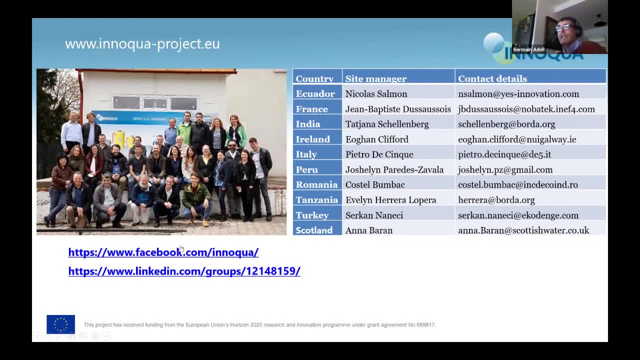 Ecoin developed another version of the biosolar purification system. so at the end of the day, as scott has said, the daphnia filter is is more sensitive, so it's still. so we what i what i mean is that we end up the project with different. the different modules have different, let's say, virtues and problems. 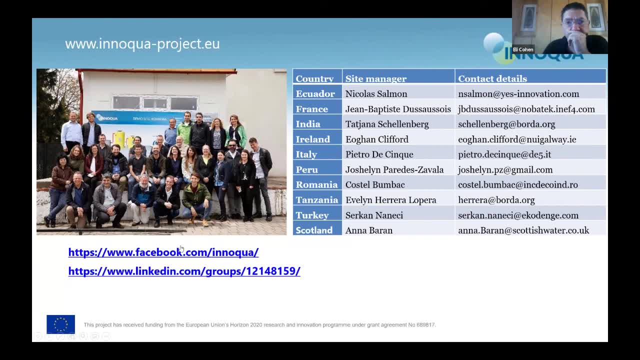 of by themselves. also, they are at different, perhaps distance from the final market, but the interesting thing is that all the partners are committed to keep on working on on the system. so we have decided to to create what we call the inoco alliance, which is, you know, as you know, the project. 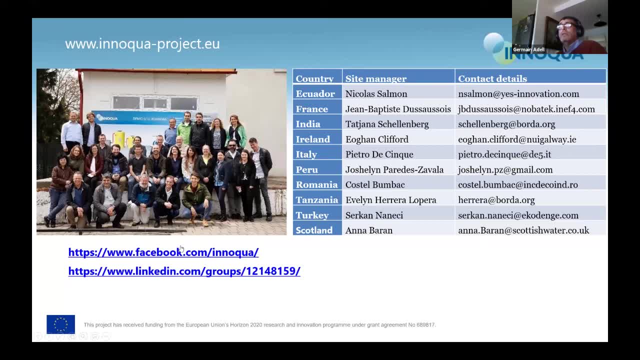 is finishing now, and so we are committed to keep on working with us to help each other in order to push forward the national project, and we are committed to keep on working with us to help each other in order to push the system to the- when needed, the last stage of development. 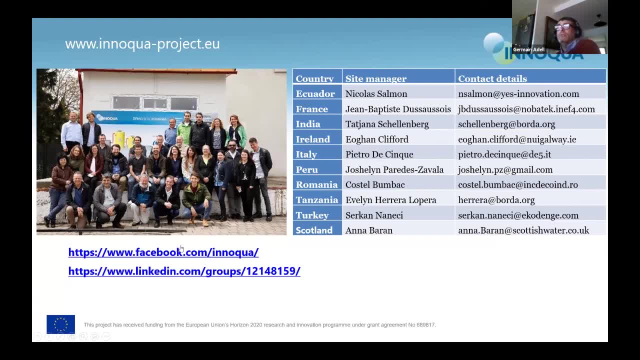 before reaching the market and, of course, pushing the system to the margin. we strongly believe that what we do has sense if we bring a final product to the market to the market or the markets, let's say, in different countries. so this is for me, this is a proof that 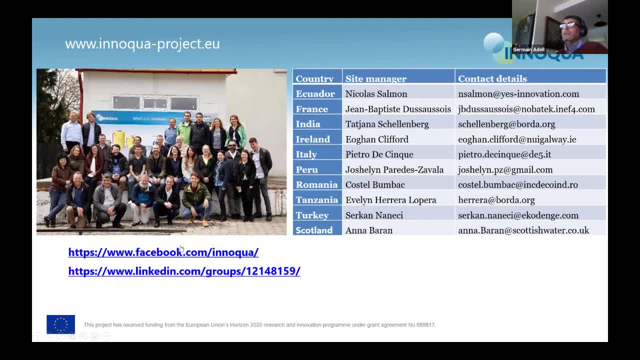 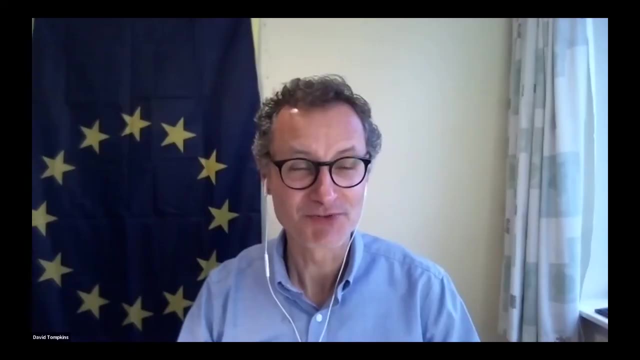 the European Commission. funding research and development can bring something very concrete and real in order to respond to the needs of the people, not only in Europe but worldwide. so thank you very much and if you have any question, we will be happy to answer. moving on to another excellent presentation, 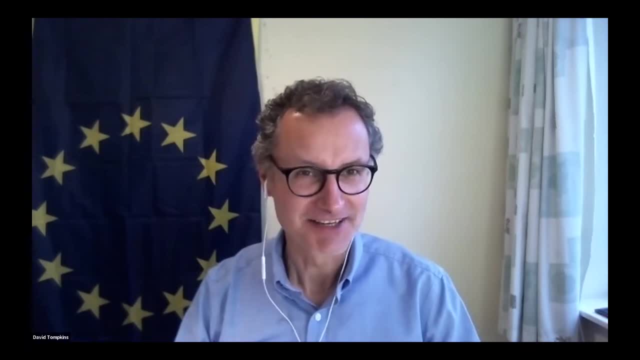 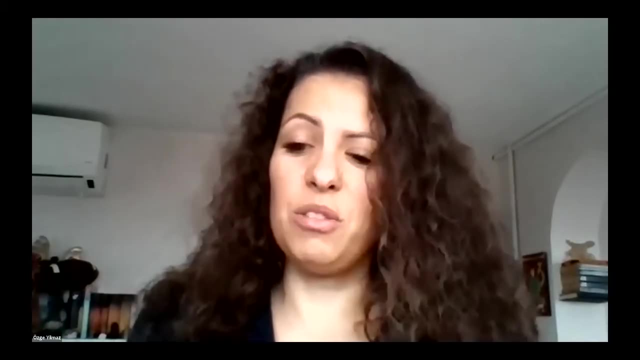 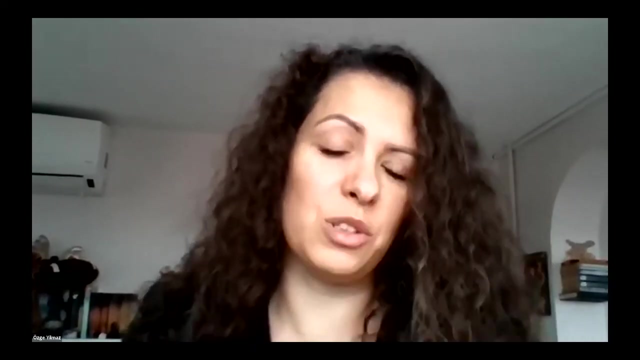 as I hand over to our host today, Erskine. so if you'd like to introduce yourself, and please, the floor is now yours. thank you. yeah, thank you, David. thank you. so one quick announcement from my side. so this is kind of Murphy's law. I lost the power at my house right now. 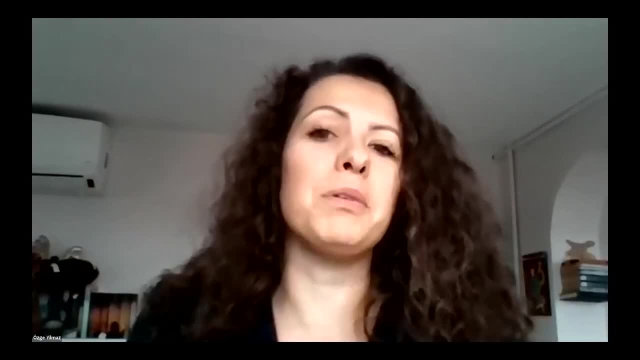 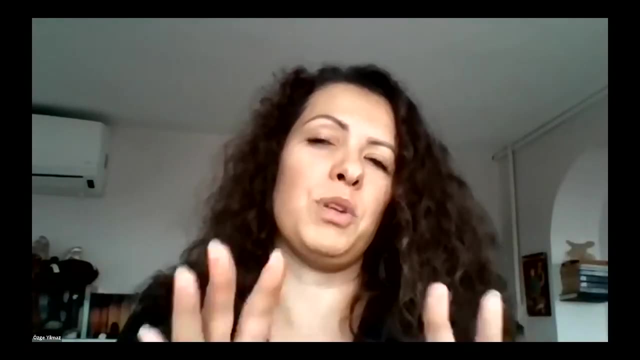 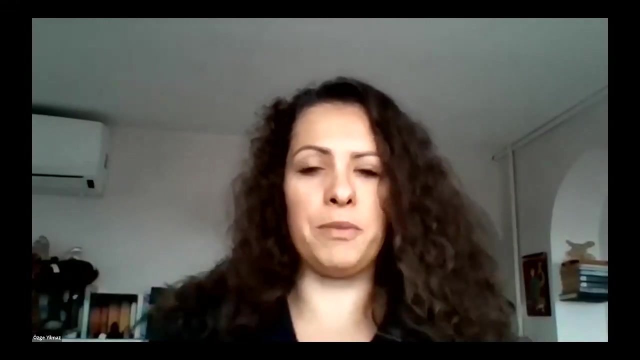 so I'm connected through my phone. so if there are any problems with the presentation, with my voice or the video that I'm about to show, please let me know. we can. we can stop and just try another time, but hopefully everything will work. so, as I very briefly introduced myself, 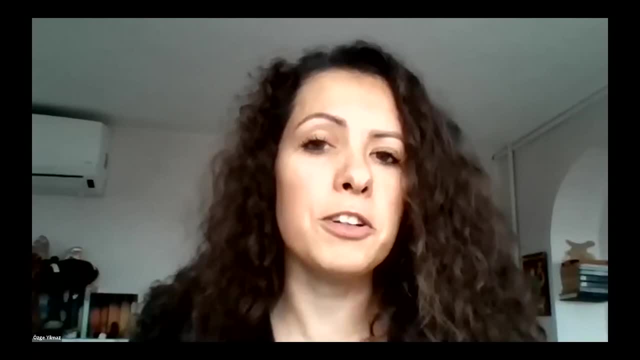 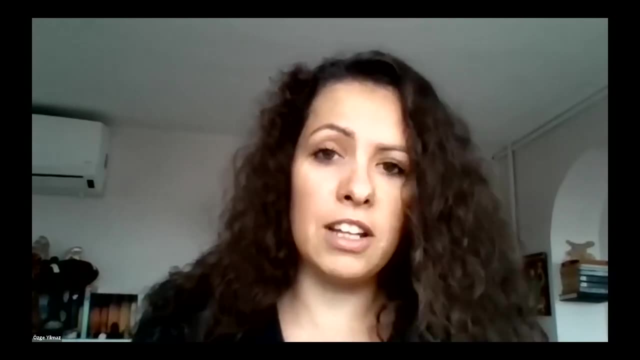 my name is Özge Yılmaz, so I'm from. I'm working with Ecodenge. we are an SME in Turkey. we are coordinating the Turkish demo site in Sinop. what we have done during the project. we were supposed to have some open days. 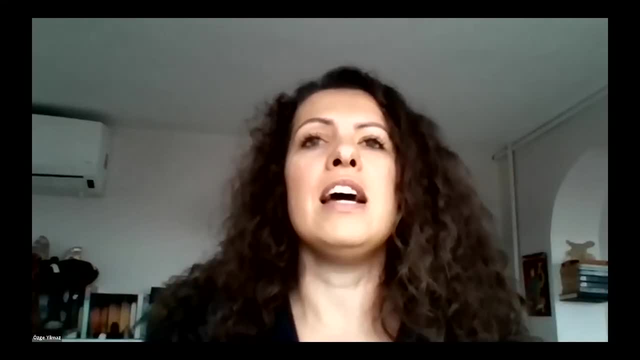 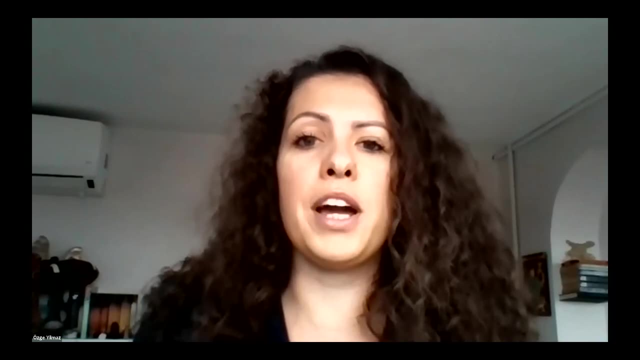 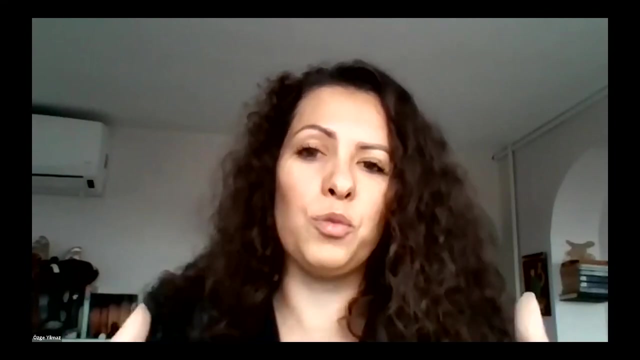 so invite local stakeholders that might be interested in, you know, replication of the system where we have implemented already and in fact try to get some attention from other stakeholders that we can, you know, convince them to try in a co-op project. some other places, some other regions in Turkey. 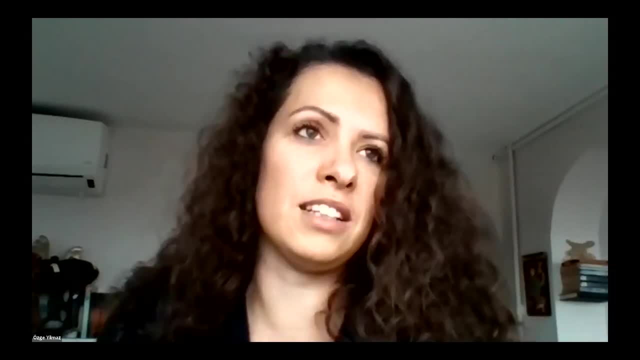 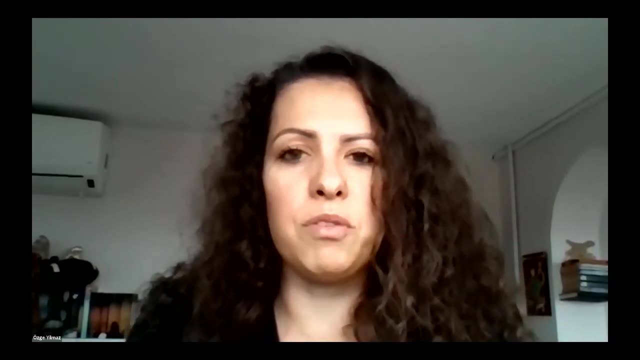 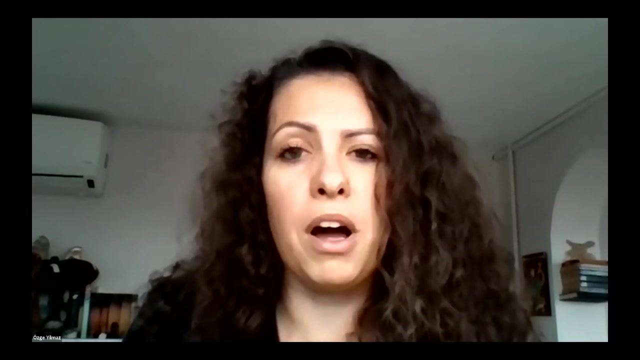 so Cermen is quite right about our commitment to the project. although we are at the end, we are very much committed to it and we would like to see in a co-op system to be implemented in other places, because we are very much also convinced about its applicability and affordability. 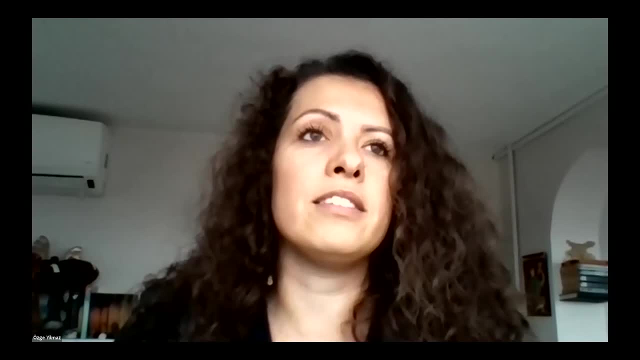 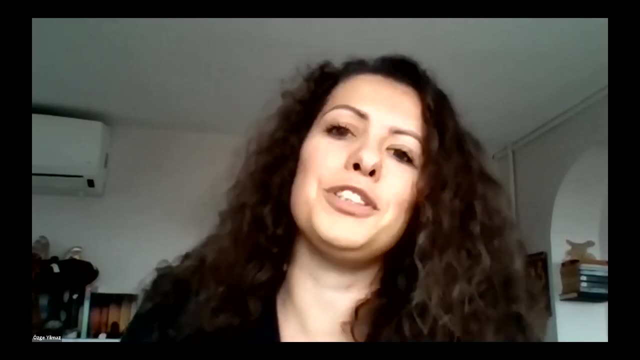 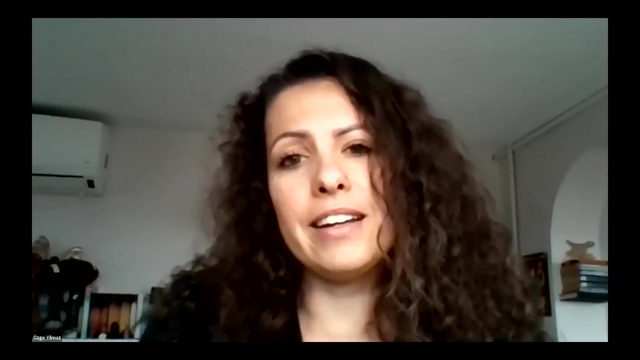 so thank you very much. thank you the low maintenance aspect of it. we have already seen it. So, because of the COVID situation, we were not able to set up open days, but what we have done was to shoot a small video, a virtual tour of our demo site. 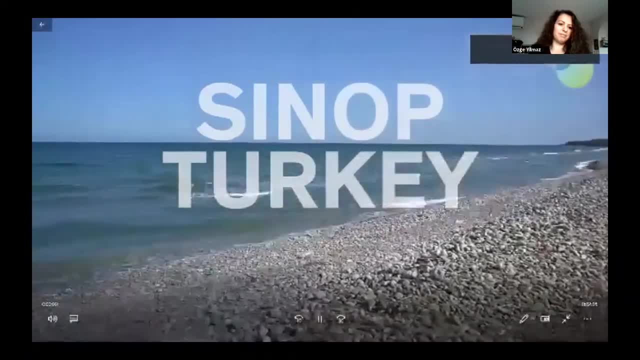 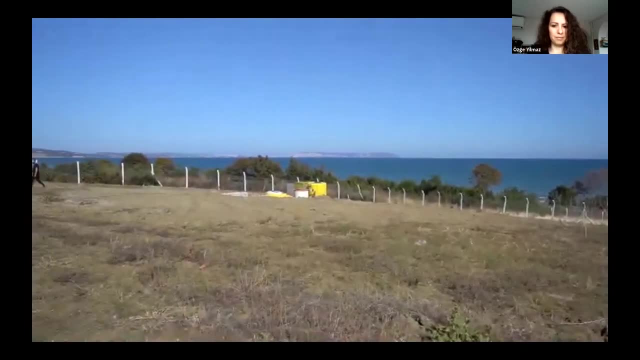 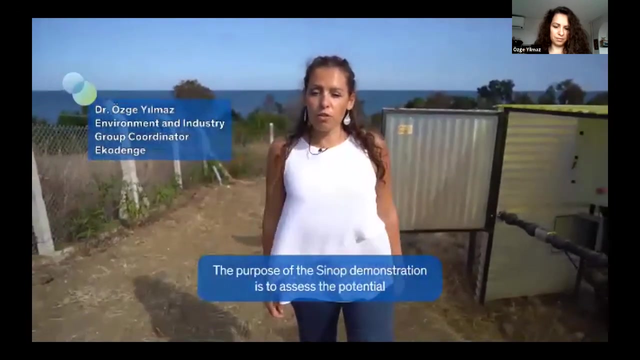 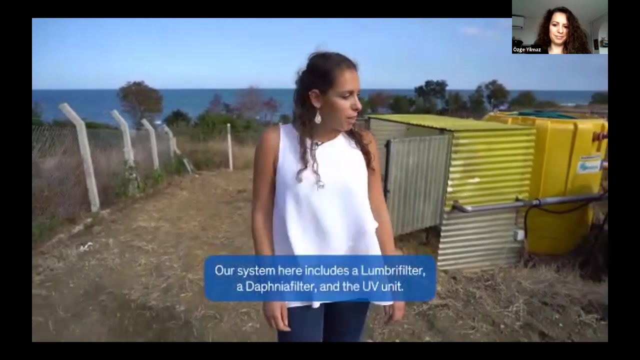 and I'm about to show it to you. The purpose of the SINOP demonstration is to assess the potential of Inukua technologies in residential housing, as well as potential for reuse in irrigation. Our system here includes a lumber filter, a daphnia filter and a UV unit. 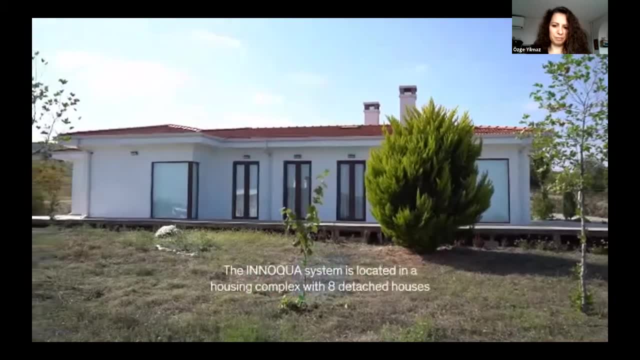 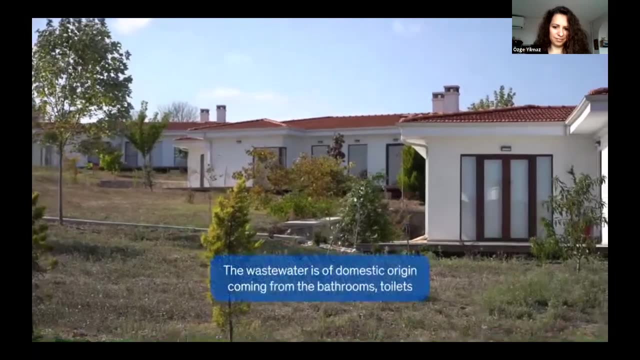 The Inukua system is located in a housing complex with eight detached houses and hosts up to 55 people. The wastewater is of domestic origin, coming from the bathrooms, toilets and kitchens. Inukua is the largest water supply system in Turkey. 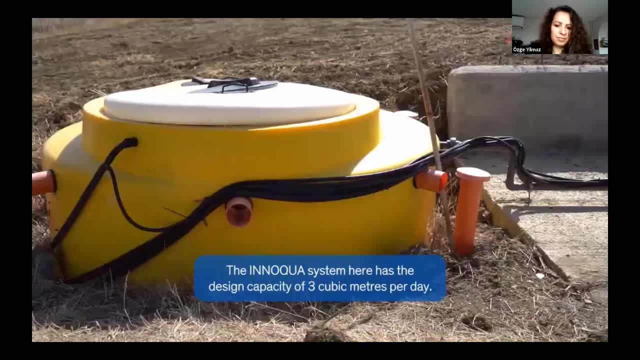 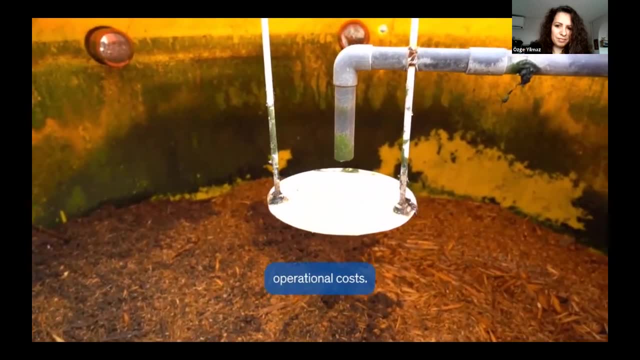 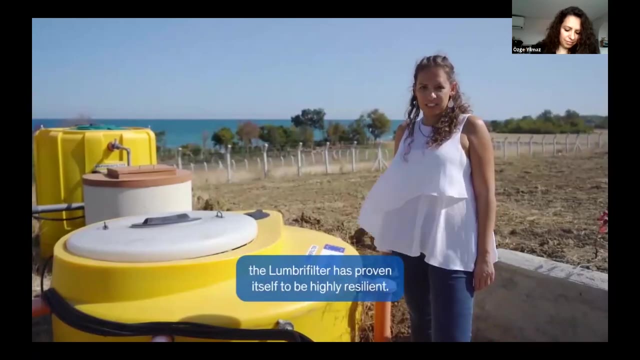 And the Inukua system here has a design capacity of three meter cubes per day, And the lumber filter presented the benefit of reduced maintenance and operational costs Throughout the operation. even with varying quantities of wastewater, the lumber filter has proven itself to be highly resilient. 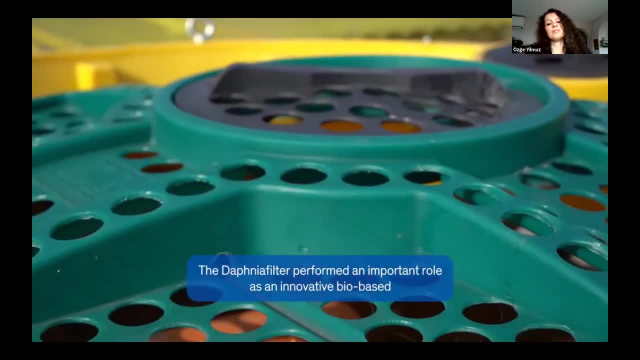 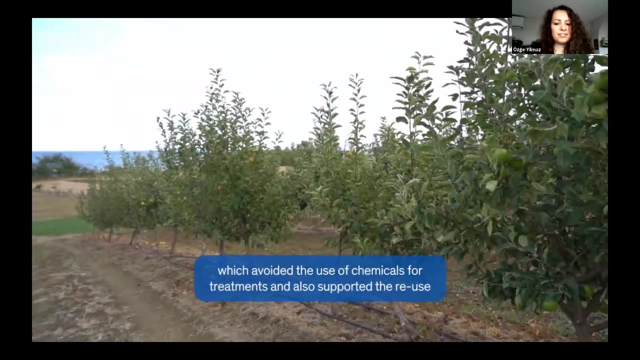 Daphnia filter performed an important role as an innovative bio-based tertiary treatment which avoided the use of chemicals for treatment and also supported the reuse of treatments. In addition, the Inukua system was able to reduce the use of chemicals for treatment and also to reduce the use of chemicals for treatment. 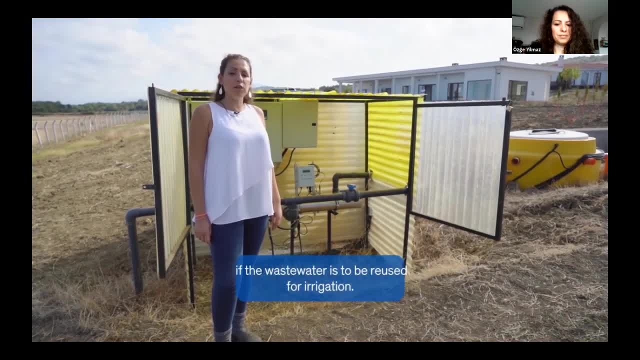 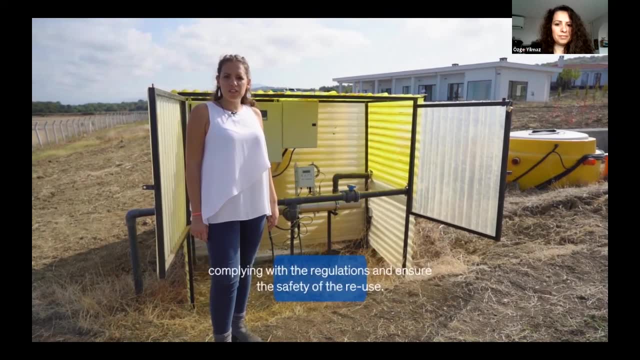 Turkish regulations on water and wastewater are especially strict in terms of the presence of pathogens if the wastewater is to be reused for irrigation. With this UV unit, we were able to disinfect the treated wastewater, comply with the regulations and ensure safety of the reuse. 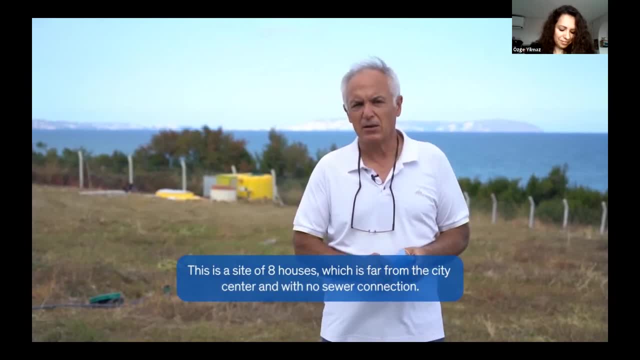 This is an eight-house site. We are far from the city. We don't have a sewer system. We are very close to the sea. We were trying to manage it with a POSEPTICS. well, As you can see, we have a beautiful fruit garden on one side. 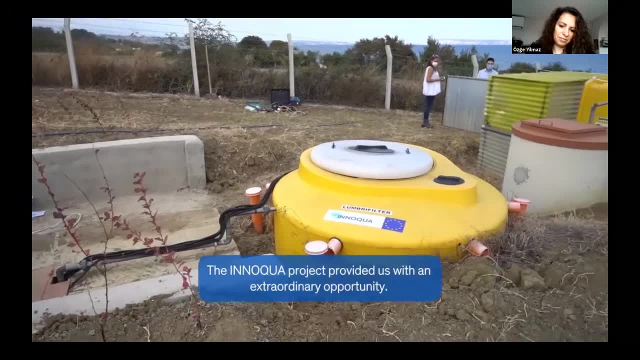 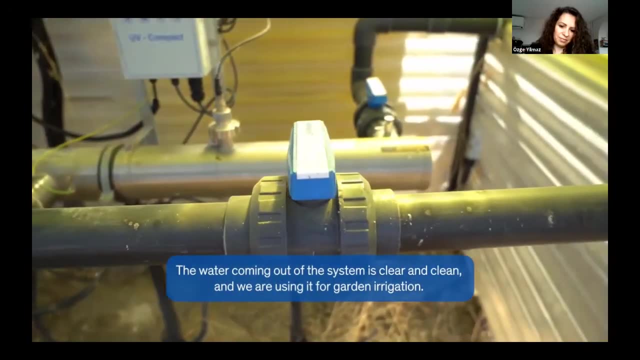 We don't want to pollute the environment. With the Inukua project, this provided us with an extraordinary opportunity. The water that comes out is clean and we use it for watering the garden. We don't pollute the sea. we don't pollute the environment. 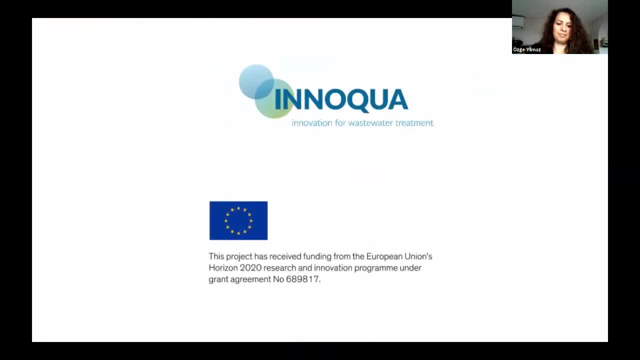 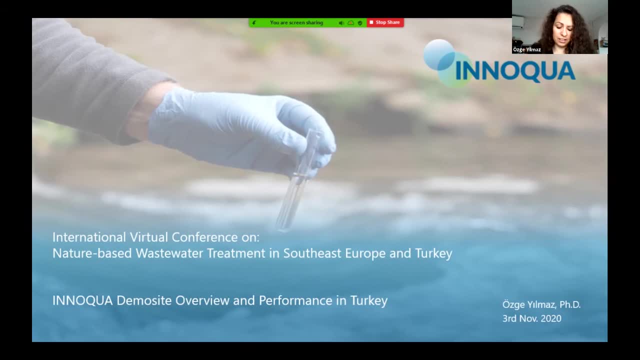 We are very happy in this respect. So this portion after the conference it's dedicated to us, Kostel and me, trying to give you some information about our respective demo sites. So I will start with Turkey and Kostel will go on with the Romanian demo site. 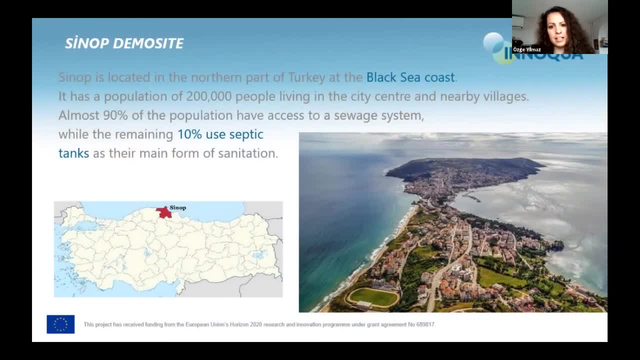 So Sinop is located on the northern tip of Turkey. It's on the Black Sea coast. It has a population of about 200,000 people living in the city center and nearby villages. Almost 90% of the population have access to the sewage system. 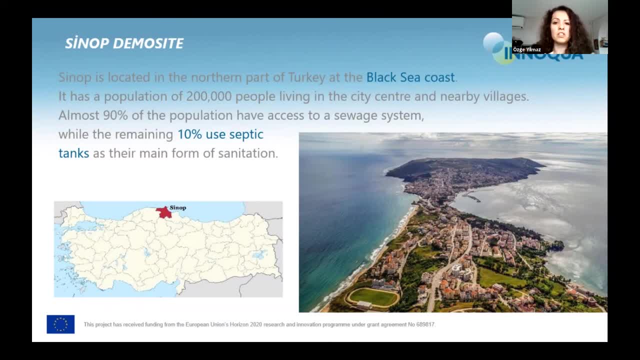 but 10% of the population use septic tanks as their main form of sanitation. The septic tanks: usually they infiltrate into the water, So we can easily say that the water is infiltrating into the groundwater without any treatment. So instead of the wastewater and the septic tanks being collected, 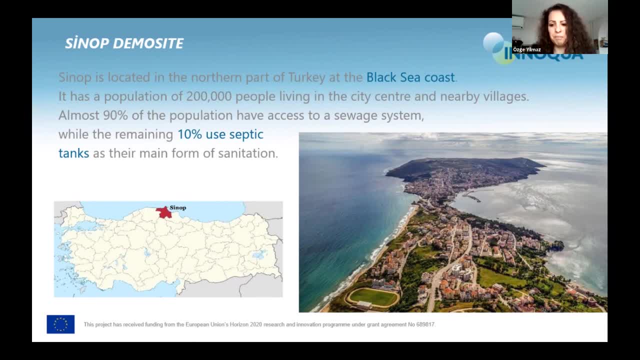 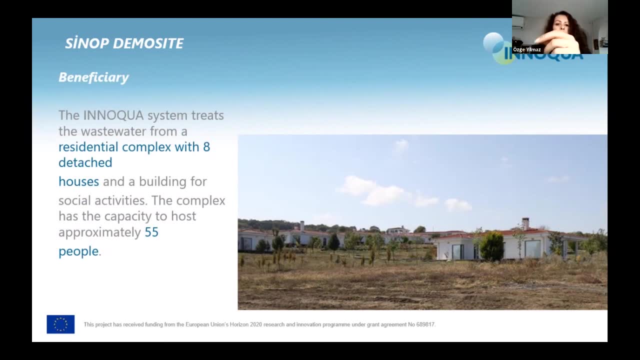 it goes into the ground infiltrated. So our beneficiary was this site which hosts up to 55 people. It's a residential complex with eight detached houses, The site owners. they are very aware of the possible environmental pollution they might be creating. 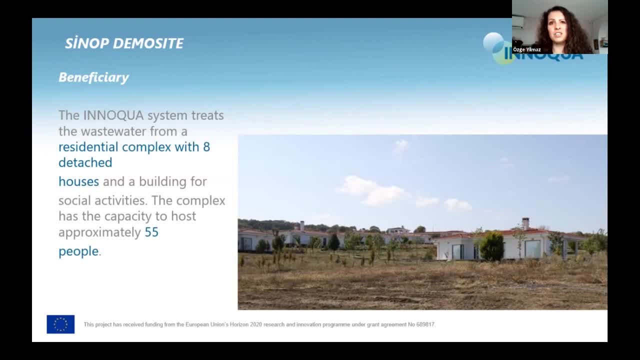 while living in this housing complex. It's actually a new complex being established, so there was some settlement started at the beginning of the project, but we did not reach full settlement, So not all the houses were occupied until the end of the project. 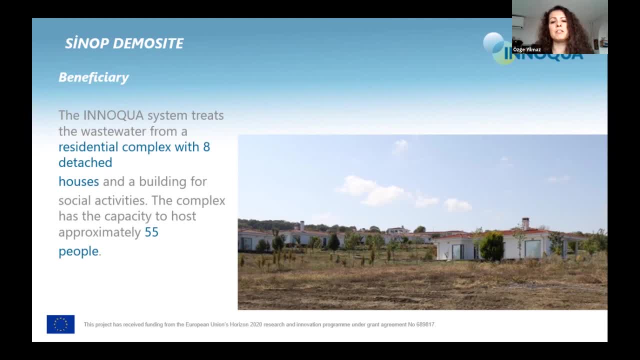 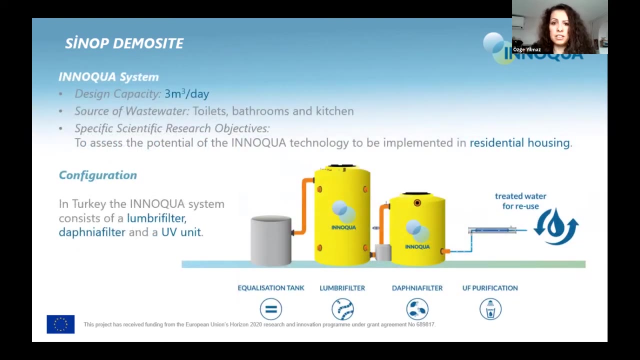 So this site is still under development, but they wanted to make sure that a treatment, an affordable treatment system, was ready on site for them to be using The system that we implemented on site. as you have seen on the video, it has a capacity of three meter cube per day. 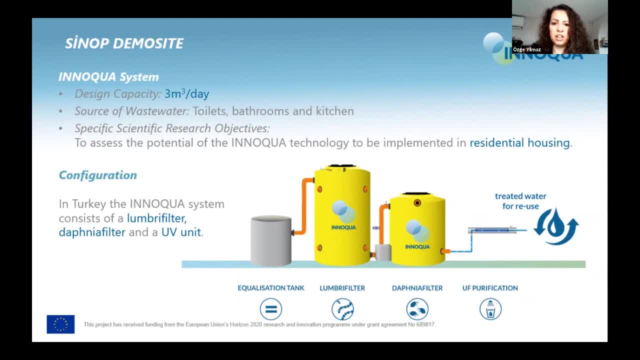 So the source of the wastewater is very domestic. What we wanted to do to assess the potential of the Inukua technology to be implemented in residential housing. Of course, one interesting point for this demo site was the site owners really wanted to use the wastewater after treatment. 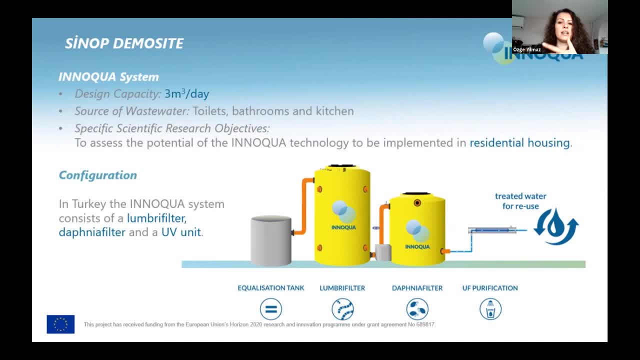 for irrigation purposes. They had some orchards and they have some greenhouses. They had some green areas that they wanted to use the wastewater for irrigation. For this purpose, it was found out that the best configuration was to use the Lambren filter. 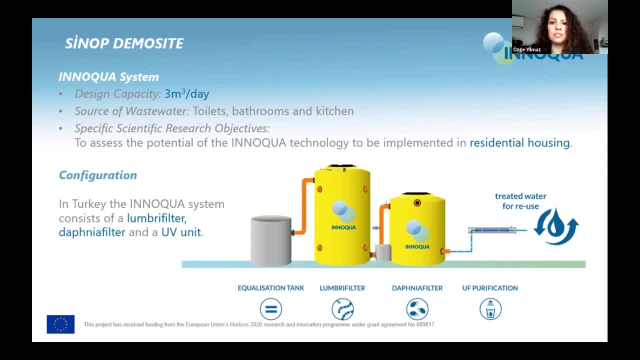 the Daphnia filter and the UV purification. So disinfection was especially necessary for the reasons because the Turkish legal limits for reuse of wastewater is rather strict, So we needed some sort of disinfection at the end of the treatment, As I said. unfortunately, 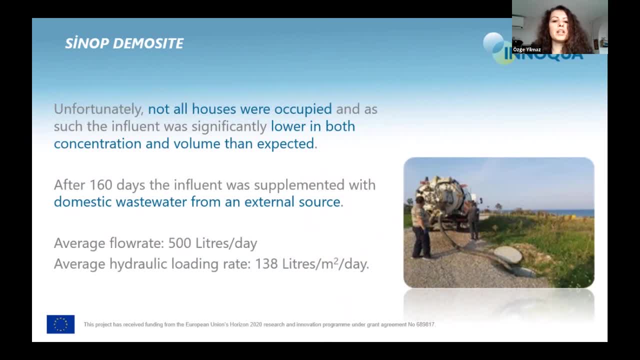 not all the houses were occupied throughout our demonstration, So the influence was significantly lower in terms of both concentration and volume expected. And also one side information, Sinop, the Black Sea region in Turkey. it receives a lot of rain throughout the year. 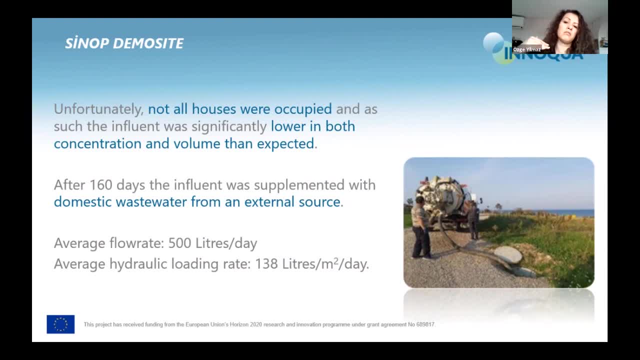 especially in autumn and winter it receives a lot of rain, So we also have a lot of stormwater rainwater infiltrating into the sewage. that also caused the concentration to go even lower After the first 160 days. we needed to find a solution. 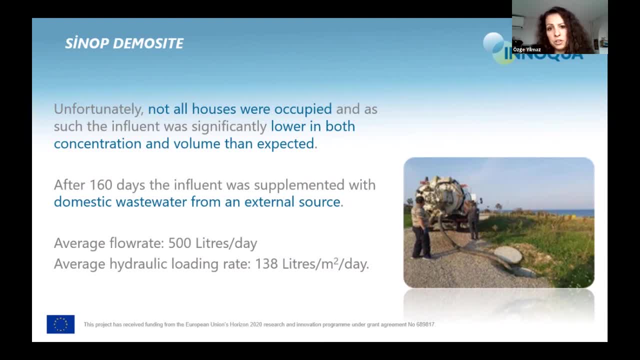 So the influence was supplemented with domestic wastewater from external source, meaning that we needed to carry some raw domestic wastewater from other sources to the site for system to be operational. But instead of reaching up to three meter cube per days, our average flow rate was around 500 liters per day. 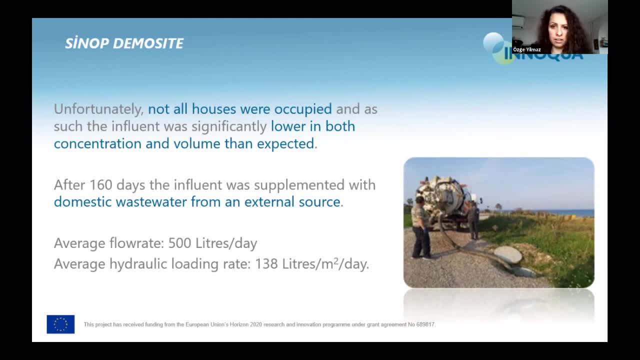 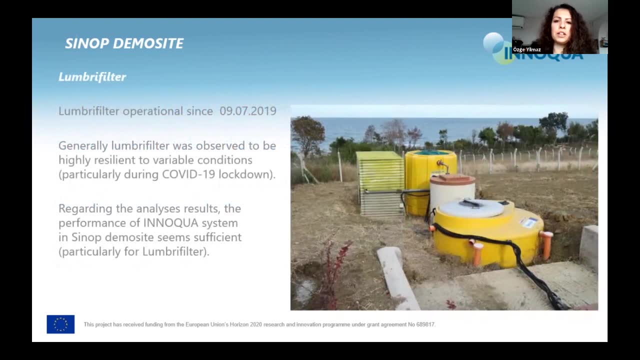 And the average hydraulic loading rates were also a little bit lower than what we were expecting. The lumber filter: we put it into operation in July 2019.. In general, the lumber filter was observed to be highly resilient to variable conditions And, on top of the lack of wastewater, 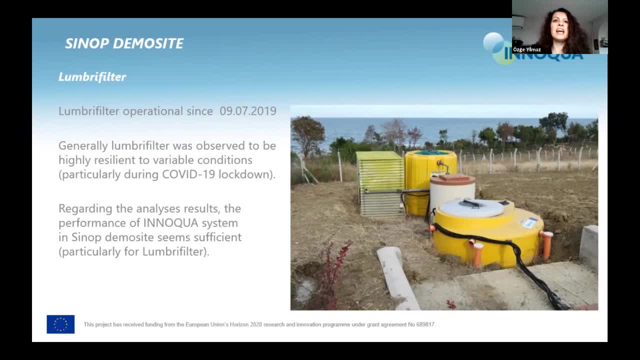 we also had to go through the COVID situation, the lockdowns and everything. So the site was almost empty because the residents weren't able to travel to their. this is kind of like a summer house for them, So they were not able to travel at all. 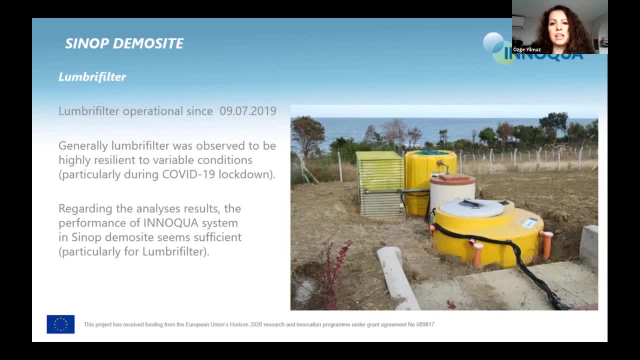 But particularly during the COVID-19 lockdown, we have seen that the lumber filter is very resilient and very, very robust. Regarding the analysis results, the performance in the demo site seems sufficient, especially for lumber filter, to provide the primary and secondary treatment that it needed to provide. 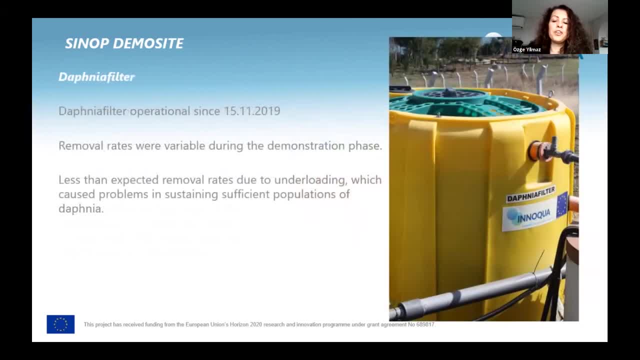 And our second system, the Daphnia filter. it was put into operation a little bit later, in November 2019.. The removal rates were variable during the demonstration phase because the consistency of the wastewater and the COVID it actually impacted Daphnia filter. 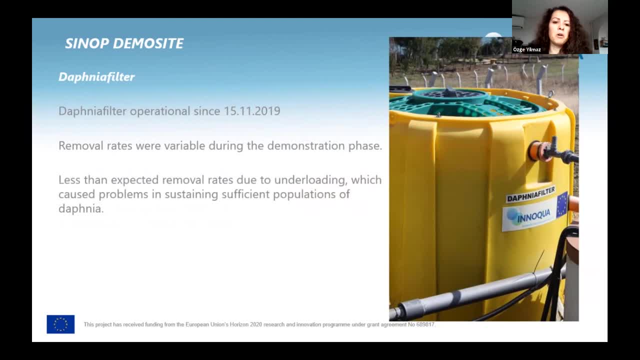 a little bit worse than the lumber filter. So we have received less than expected removal rates due to underloading, which caused problems in sustaining sufficient populations of Daphnia. So this Daphnia being a little bit vulnerable, more vulnerable than lumber filter. 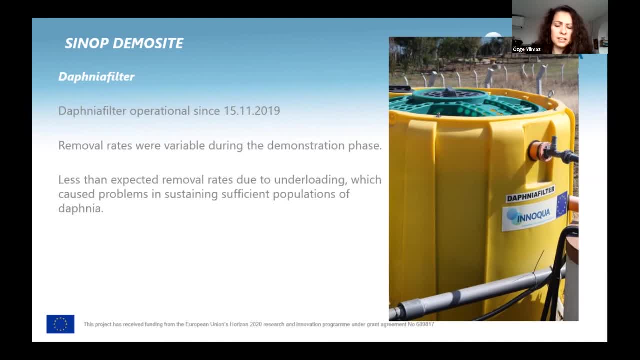 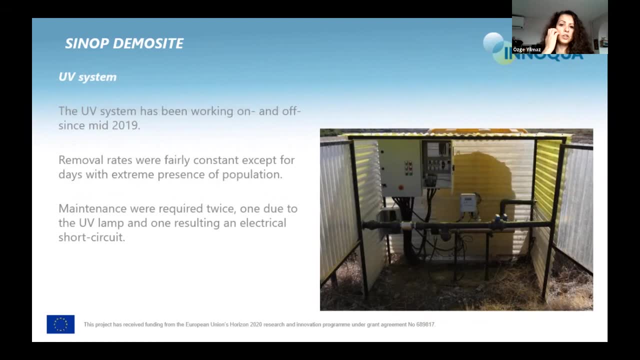 we have experienced it. So it was a little bit hard for us in our case to sustain the sufficient populations. The UV system has been working on and off, because this was kind of a learning experience for us: the UV system When it's working. 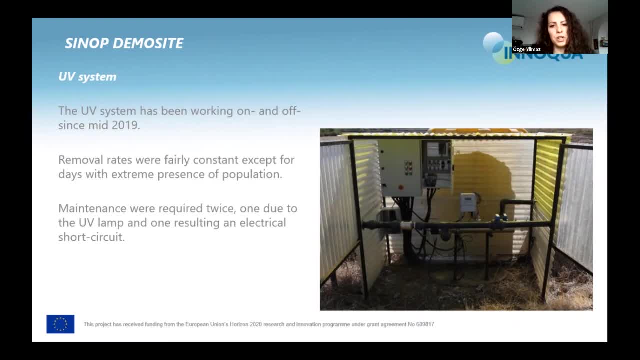 we had double of glitches throughout our demonstration phase, which needed replacement of the UV lamp once And right now we are dealing with sort of an electrical issue in the UV system. But when it is working it's very easy to operate, no need for any experience. 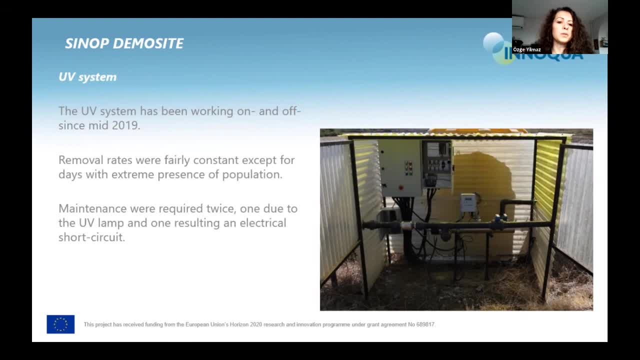 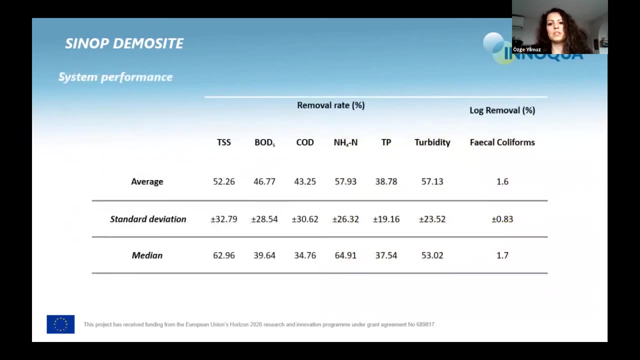 in operating the UV system itself. So the removal rates were fairly constant, except for the days with extreme presence of population. Sometimes that happened. The maintenance were required, as I said twice. So when we look at the system performance overall, 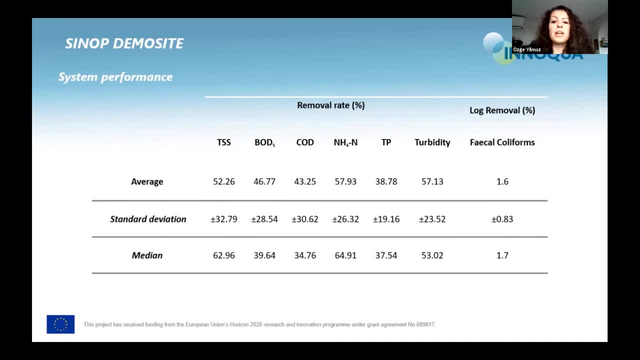 the average performance. so we have seen removal of total suspended solids, VOD5, CO2, COD, ammonia and total phosphorus. Also, turbidity was reduced because of the treatment in the system And we, of course, seen removal of faecal coliforms. 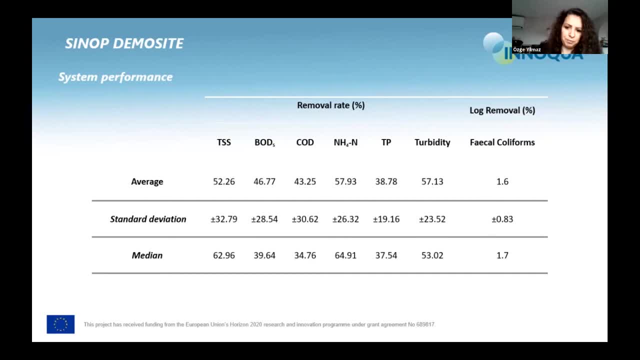 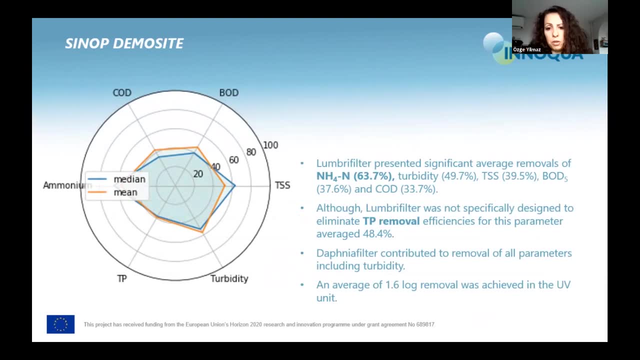 because of the disinfection. So I will just give you a brief summary of the removal performance. let's say, The Lumery filter presented significant average removals for ammonia, ammonia and turbidity, and also TSS, BOD5 and COD were removed, Although LAMBRE filter 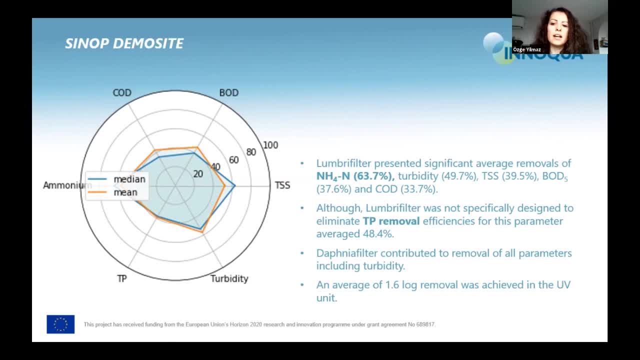 was not specifically designed to eliminate phosphorus. the efficiencies for this parameter averaged around 48%, which was very good news because if the LAMBRE filter is without to be used with another tertiary treatment option, it can still remove some nutrients. Daphnia. 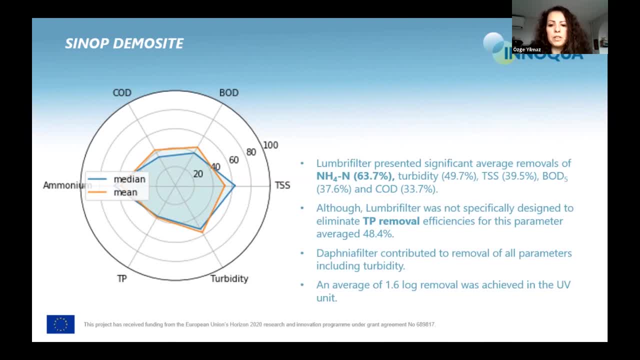 filter contributed the removal of all parameters, including turbidity. So we have seen that the combination of LAMBRE filter and Daphnia filter was effective in terms of removing the key parameters that are desired to be reduced according to our legislation. An average: 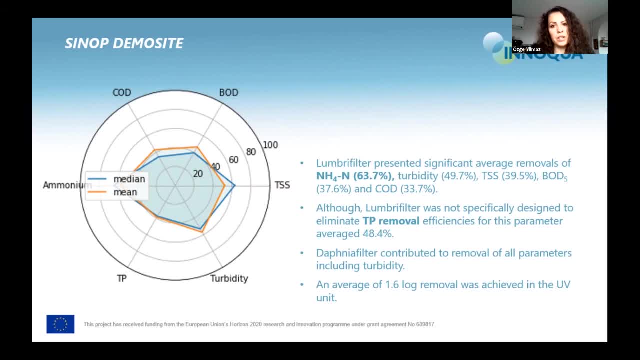 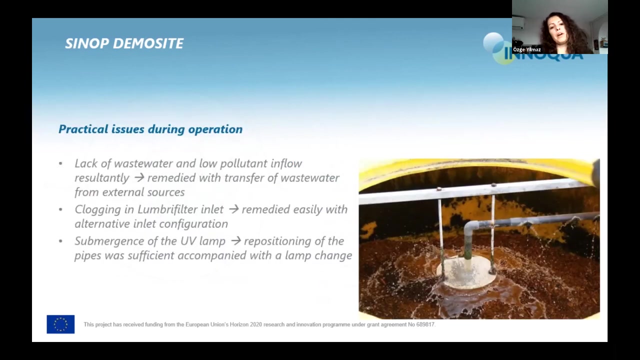 of 1.6 log removal was achieved in the UV unit. So in the end we are sure that with more constant waste water removal the LAMBRE filter was effective. So we have seen significant removal despite our conditions. So what were the practical? 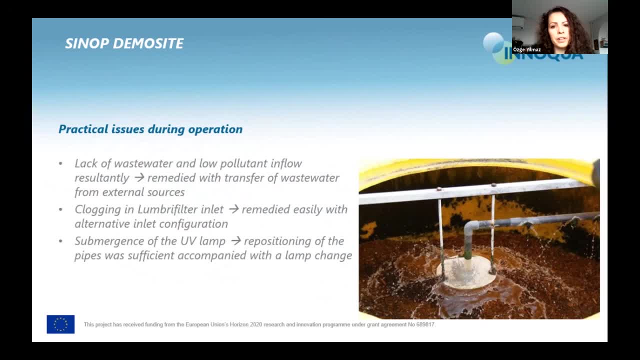 issues that we encountered during the operation. Lack of wastewater and inflow was a problem. We remitted LAMBRE filter and Daphnia filter. We have seen significant removal, despite our conditions. So what were the practical issues that we encountered during operation? Lack of wastewater and inflow was a problem, We remitted LAMBRE filter and Daphnia filter. We have seen significant removal, despite our conditions. So what were the practical issues that we encountered during the operation? Lack of wastewater and inflow was a problem. We remitted LAMBRE filter. We 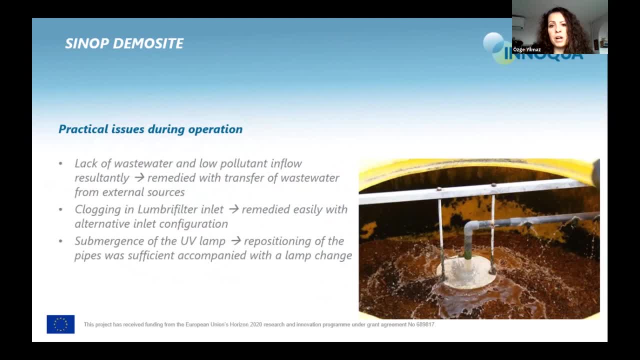 did it with the transfer of wastewater from external sources, But of course, there might be other, maybe solutions, because we were discussing maybe, since these are earthworms- they are, to be honest, they are magnificent in terms of consuming almost everything, So there might. 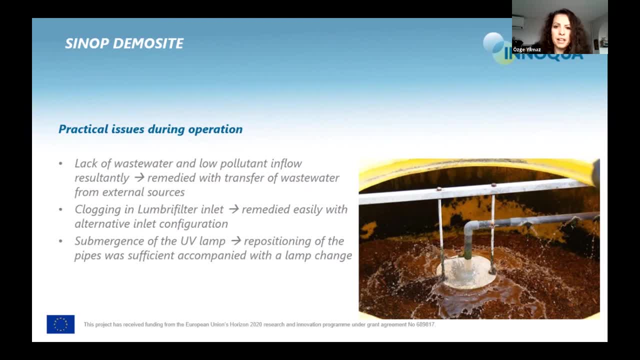 be other solutions to keep them alive, even if in future years on site there might be some lack of wastewater. It's a very big issue. We had some clogging in the LAMBRE filter inlet, but that was remedied very easily with. 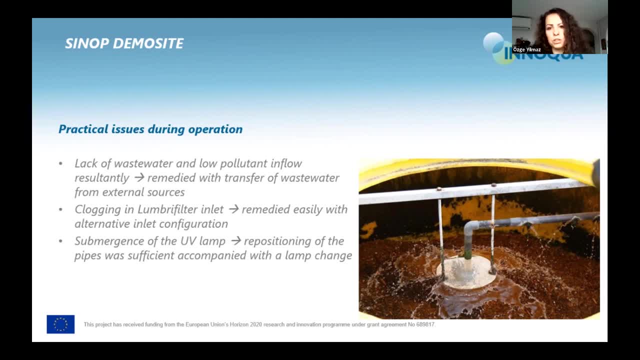 alternative inlet configuration. That was one day's work for us, So it was very easy to handle these type of situations. with the LAMBRE filter, We had a little problem with the submergence of the UV lamp. It's always need to be submerged in water, So we just 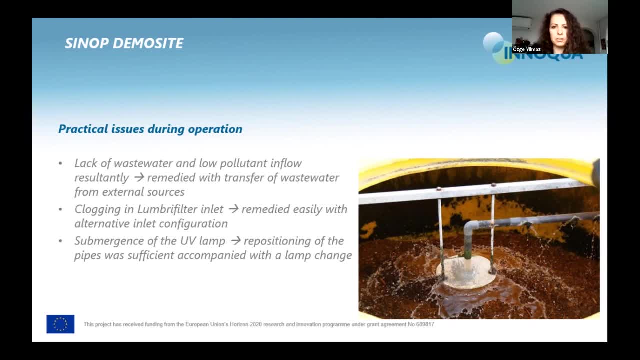 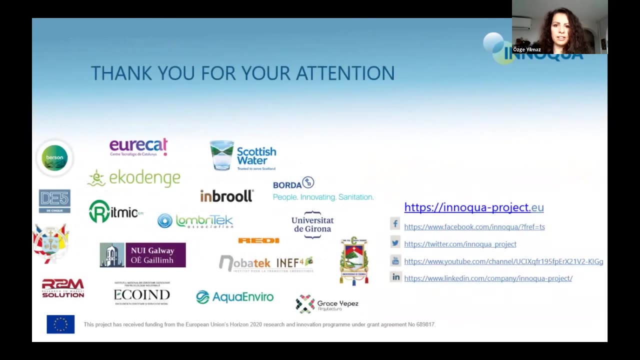 needed to reposition the pipes. That was very sufficient to solve the problem. So the thing is, except for the wastewater situation, whichever operational problems we had, it was easily remedied. Thank you for your attention. I hope the quality of the video and my sound and the presentation. 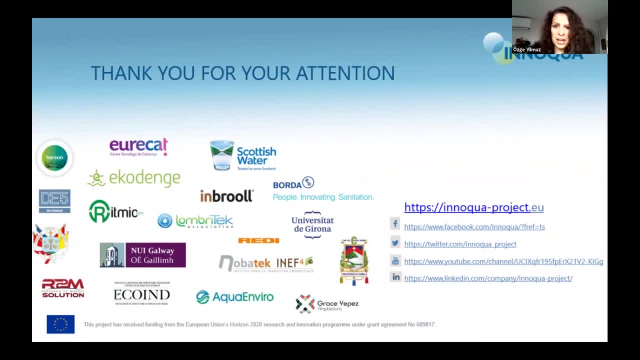 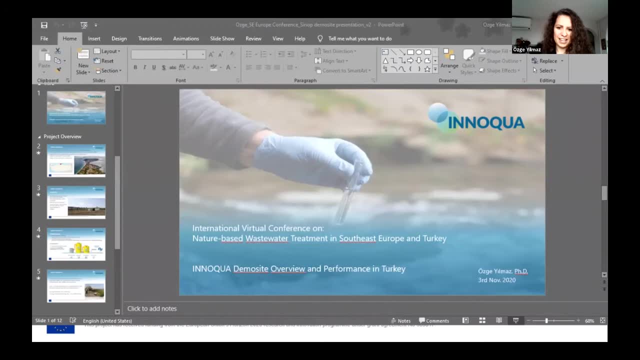 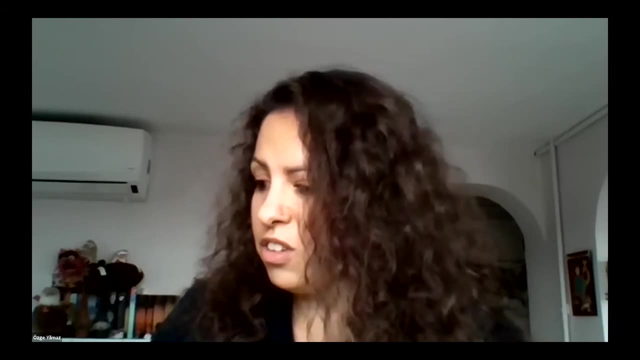 was good enough for you. If you have any questions, I would be happy to answer. If not, you can always ask questions in our panel and a question and answer session. Thank you very much. So I will just stop sharing And then I will move on to introducing. Yes, David hi. 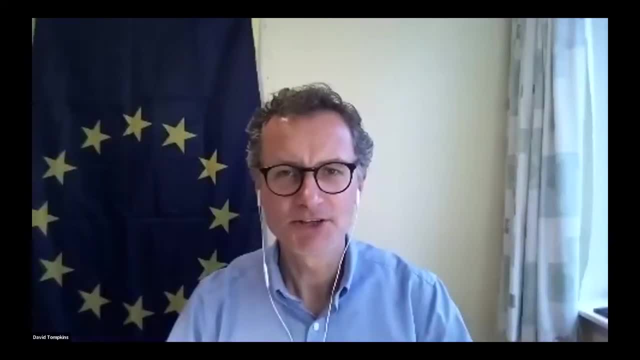 Just a quick question, Özge, if I might, Just on turbidity. So do your regulations have turbidity limits for any discharge from centralised and decentralised systems? It doesn't matter, It's the set that there's a limit on turbidity. Is that correct? 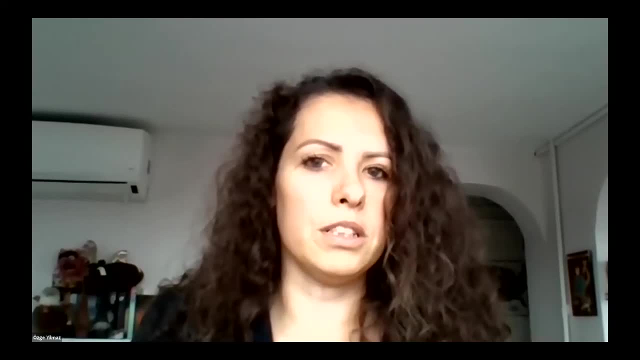 No, it's usually more related to the receiving environment. For example, if you are doing some still, for example, deep discharging, it's usually more related to the receiving environment, For example, if you are doing some still, for example, deep discharging. 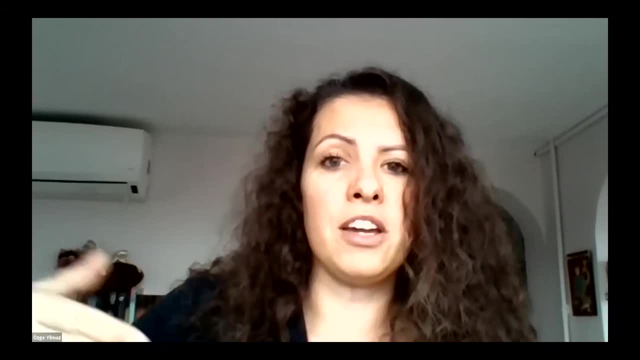 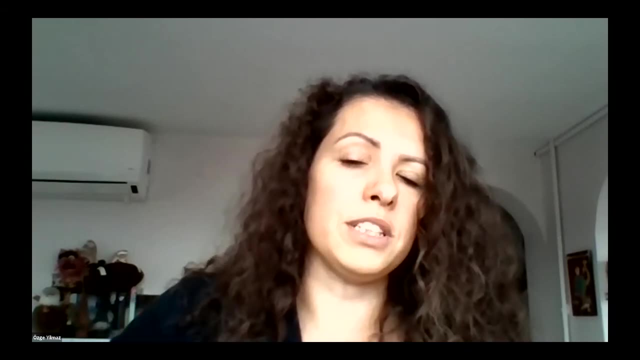 it's usually more related to the receiving environment. For example, if you are doing searched and see, this charge is allowed in Turkey. That's why many of the coastal towns in Turkey they are discharging to see. So if you're discharging into a surface oats. 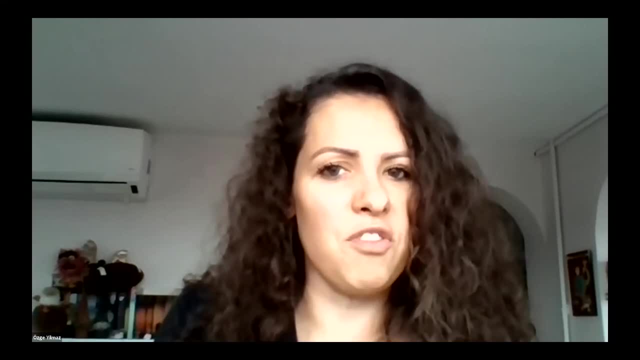 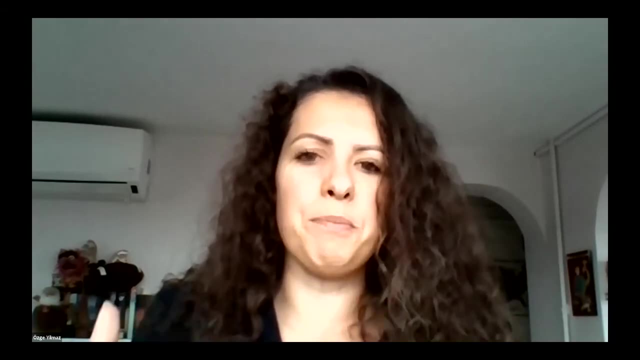 then the quality should be different, So it depends on the receiving environment, rather than being centralised or decentralised, And also they are trying to implement sort of this: you know, the limits based on the vulnerabilities of the receiving environment, as well as the possibilities of the receiving environment as well as desses, And is there further feedback required from those or processes? No thanks, Yeah, thank you. So simply, the enterprise could use this, put this position. I would want to place your question to protect me or some of the others we are involved in Isis. 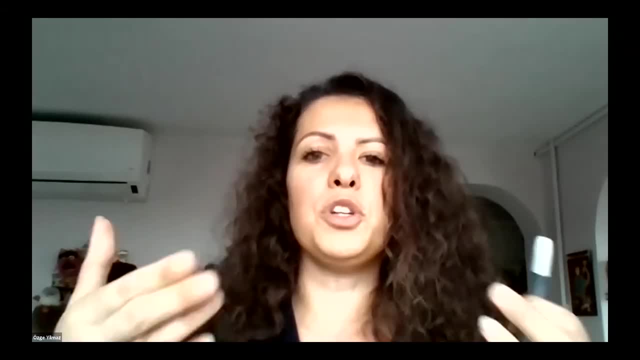 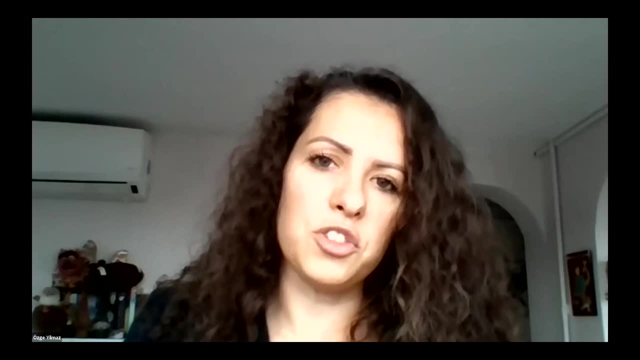 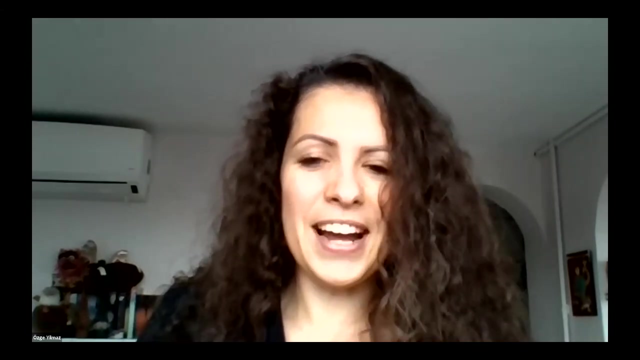 Especially if, for example, there are too much already nutrients in the receiving body- water body- then the limits should be even lower. So this type of changes happens, but not because of the capacity or it's being central or decentralized. All right, So we move on to I believe it's Kostel's turn again. 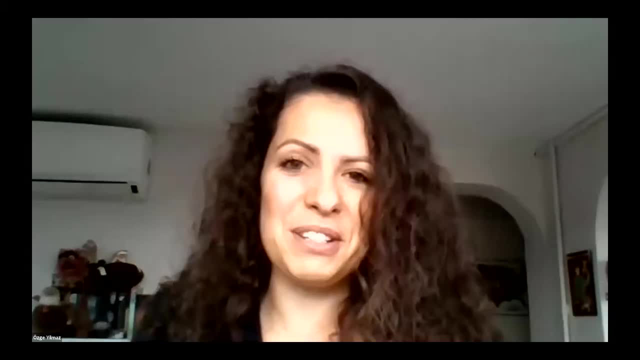 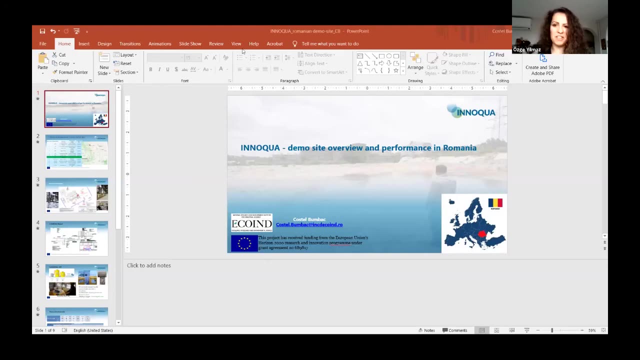 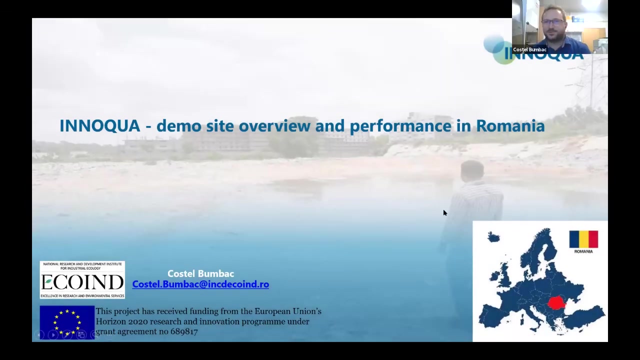 Kostel. now for the last presentation before our break. he will deliver his presentation on the Romanian demo site, the overview and performance. Kostel, the floor is yours. Thank you very much, Özge. I will try to be short and give a brief presentation of the demo site in Romania. 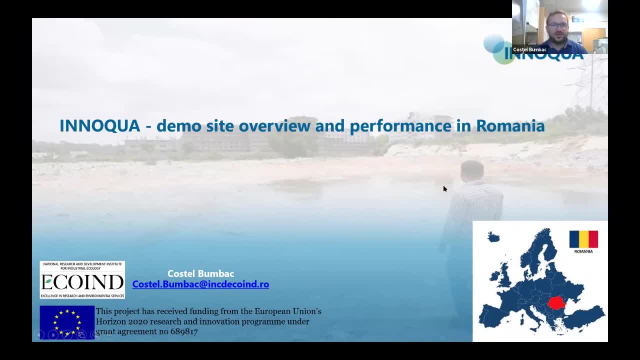 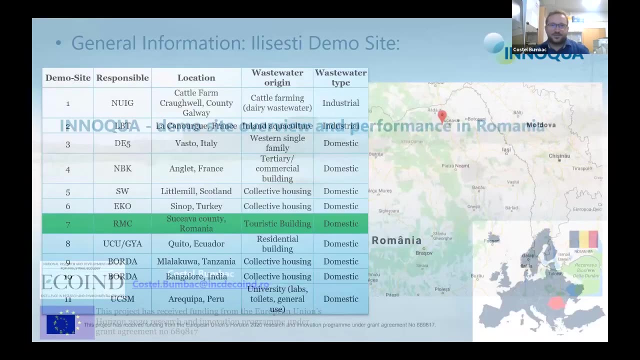 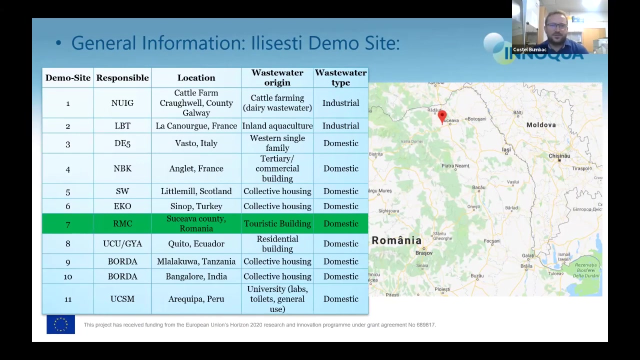 As I said earlier this morning- almost out The presentation. The Romanian population lives in rural areas and only 10% of this population is connected to centralized wastewater collection and treatment systems. The system, the demo site in Romania, is located in Ilișești, which is a small village of 2,400 inhabitants in the region of Bukovina, located on the northern slopes of the central eastern. 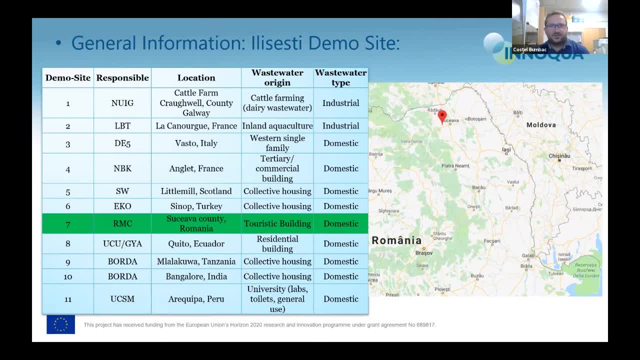 bay of the Carpathians. It's a very touristic area. Rural tourism has blossomed in this region during recent years, creating a potential niche market for decentralized wastewater treatment solutions. The UNOPA system initially treated the wastewater from a holistic building. 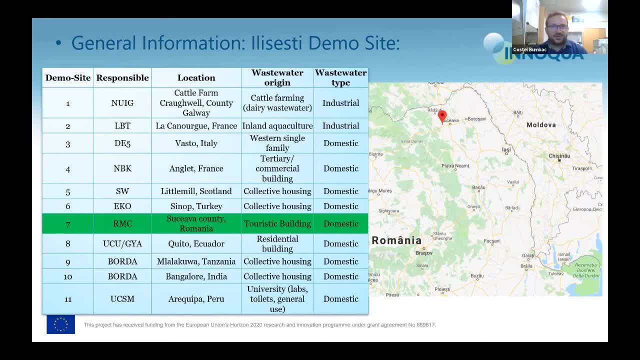 Gathering the wastewater from 10 guest rooms, a restaurant of a large guest house- maximum 100 seats- and a conference hall of about 40 places and some small offices- administrative offices. After four months of operation, our local project partner needed more office space. 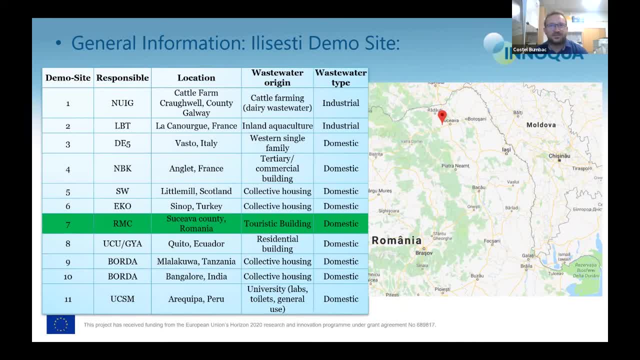 for the administrative staff of their growing waste management and recycling business. Thus, the touristic building has been converted to an office building accommodating 30 staff. The treated wastewater is being discharged into the nearby river. The source of wastewater originally was toilets, showers, grey water from the restaurant and kitchen And after 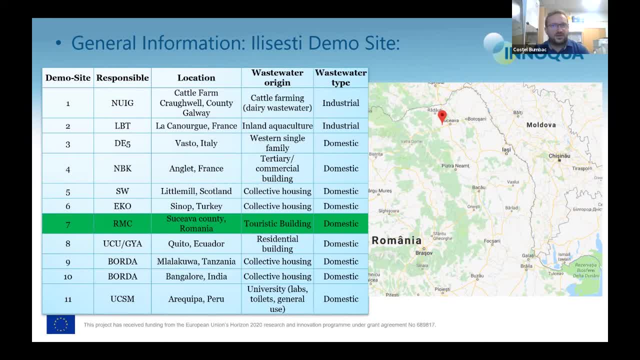 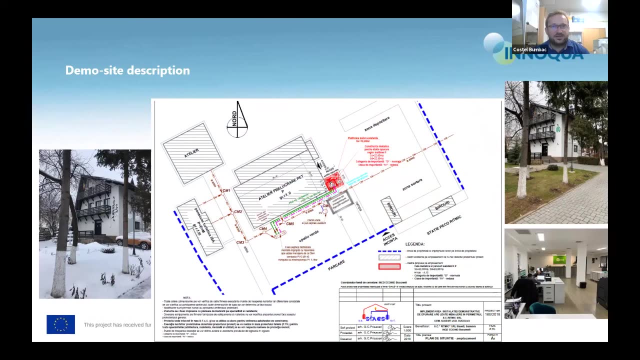 the conversion, the office building. the sources were mainly toilets, garbage and grey water from the restaurant's kitchen. The Romanian demo site aims to demonstrate the long-term performance and suitability of the centralised wastewater treatment in real operational conditions, with the extremes of temperature from minus 25 during wintertime. 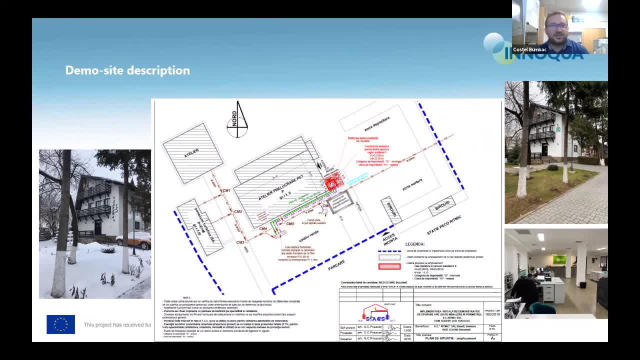 to plus 25 during summertime, with an annual average of only 7.9 degrees. In such conditions, wastewater treatment should be considered to be a core element in the management of waste management. This way, we can guide the ultimately producing of waste management. 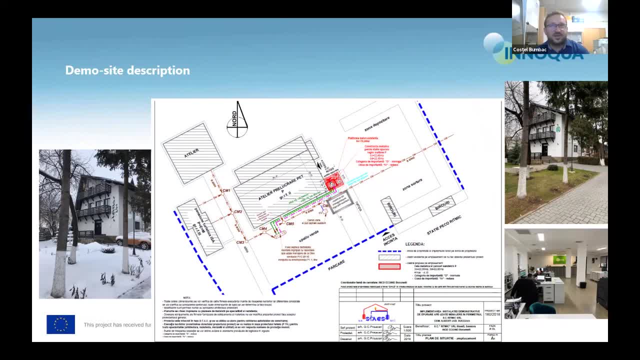 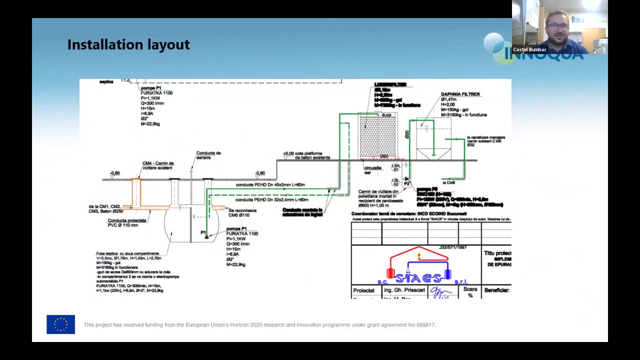 should would typically be installed underground. however, to give the possibilities of technical adjustments and dissemination to larger audience and showcasing, the inocua system has been installed in an above ground insulated by a filtered room located next to an industrial building. the inocua system installed in romania consists of a pre-settler. 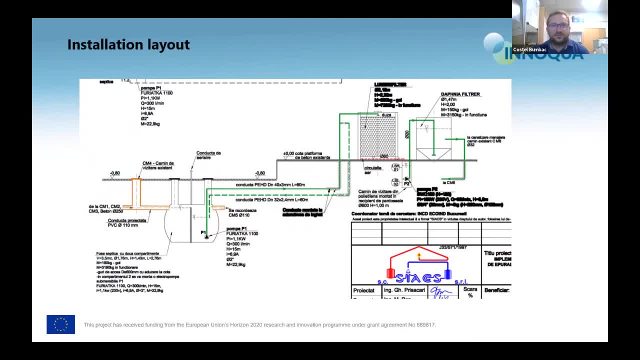 a lambda filter and the daphne filter, all monitored by a monitoring and control unit. before inocua, the wastewater on the premises was collected and discharged after a septic tank with within the nearby river uh. we installed the system next to the existing sewer line serving the premises, diverting the flow towards the inocua. 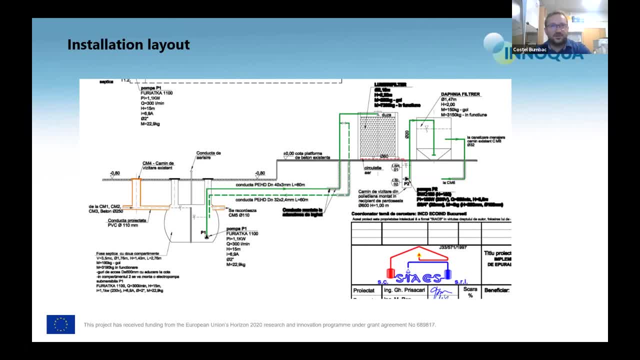 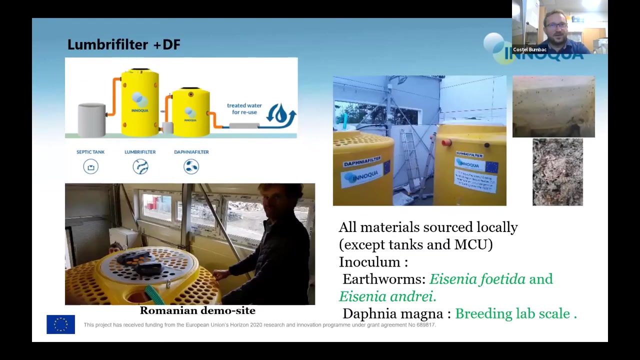 system. the water is being pumped on top of the lambda filter, which is the core technology of the inopa system, and afterwards the water is being re-pumped to the daphne filter. so the influence is being sprayed on top of the active layer of the lambda filter and passed through. 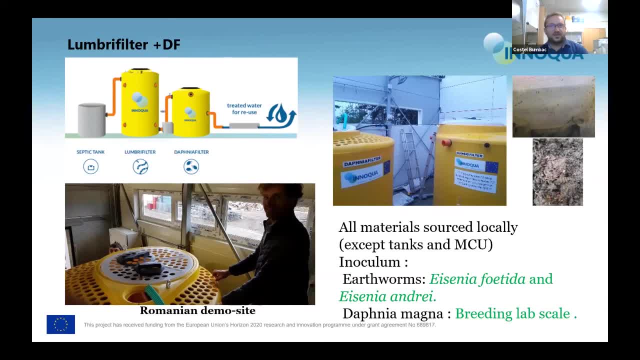 the act and passes through the active layer, where bacteria removes the dissolved nutrients, while earthworms provide the service of consuming the tss and regulate the microbial biomass so that clogging of the system is being avoided. then the effluent of the lambda filter is then 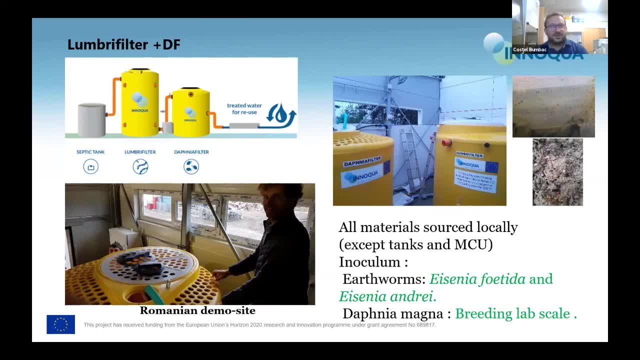 passed through the daphne filter and the inocua system is being re-pumped to the daphne filter, which is configured as a tank inoculated with local species of cladocera daphnia magna, which are free to move up and down the water column in the daphnia filter. there are some. 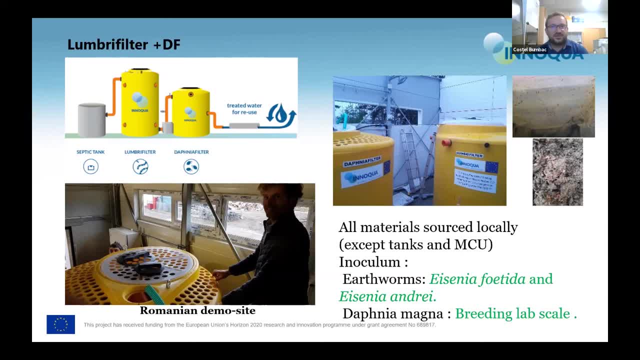 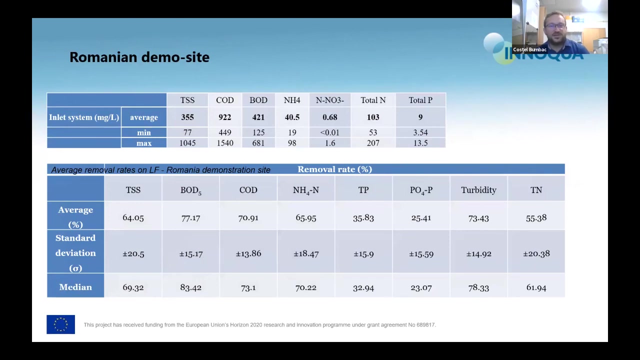 internal beer and baffle mechanisms which ensure that the daphnids remain within the reactor, while additional surface area is being provided for the establishment of microalgal or bacterial biofilm which help in the nutrient removal process, being operated in real environmental conditions. the influent wastewater quality varied widely, with concentration of cod ranging from 400 from. 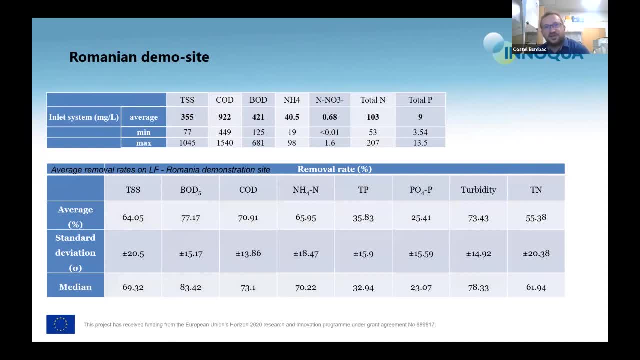 450 to 1500 milligrams per liter, bod from 125 to 681 milligrams per liter by lautron, london, Sharon. what does the yield- a reduced Parcello- tell? more information about the use in the tube for the inocua system between bluetooth and web4 couldn't show what theweedAY snapped. it was like to the inoc Council. the Delta system range from 0.3 cubic meter per meter per day to 0.8 cubic meter per meter per day and for 10 000 light meters per day. was it job? including the water is the level of which, not the lobby design brickette? 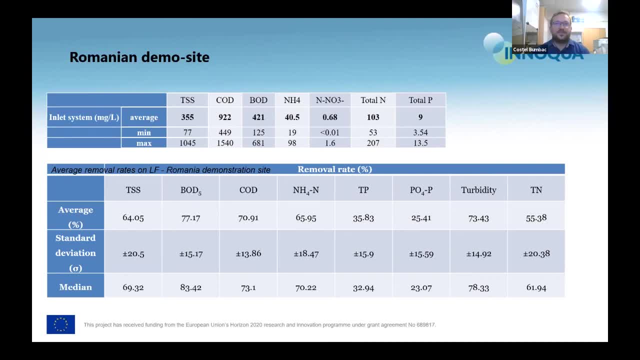 cubic meter per square meter per day. moreover, during the conversion of the building from touristic residence to office building, large amounts of unauthorized discharges of wall paint residue and other construction specific chemicals were discharged into the system, and these discharges affected the treatment performances of the lambre filter to a certain extent. while for daphne- for daphnia- population. 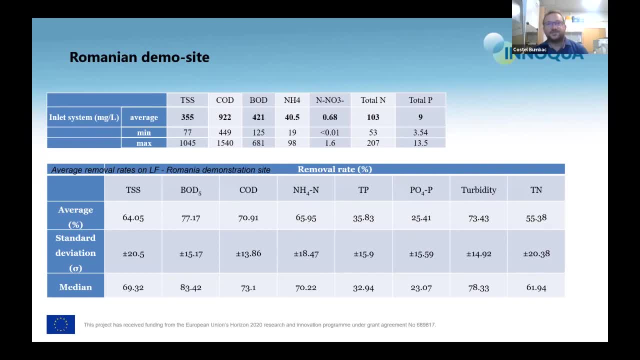 in the daphnia filter was quite fatal at some point. the global efficiency of romanian demonstration described here are taking into account only the lamp infiltration technology. therefore the global efficiency on romania demonstration site presented average removal rates of uh: 64 percent. for pss removal 77 percent. the dod removal 79, 70 percent for cod removal. 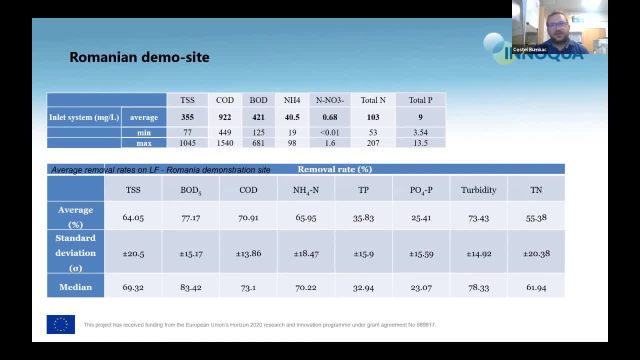 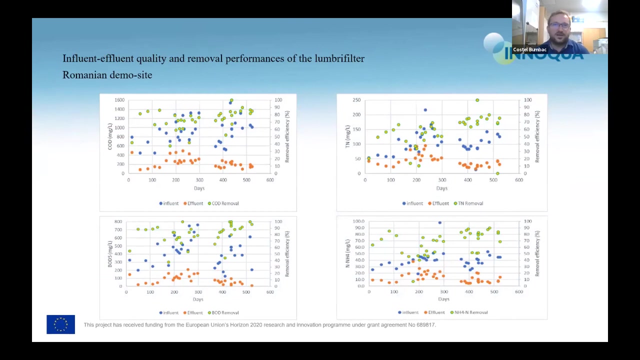 and less significant removal rates were observed for nitrogen ammonium: 66 percent removal rate, 35 percent removal rate for total phosphorus and 55 percent for total nitrogen. however, uh you can see here that after approximately one year of operation, uh once with the decrease of hydraulic loading rates from 0.7 to 0.3 cubic meter per square meter. 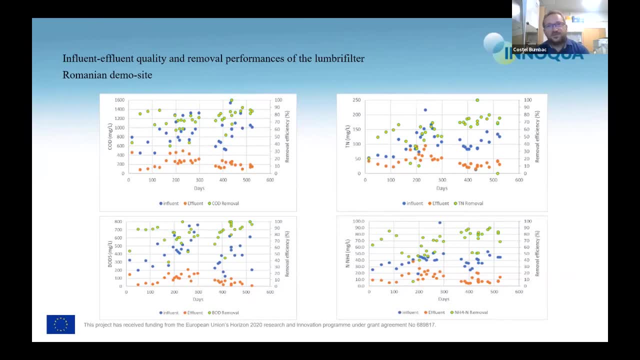 per day on the system. the treatment performance is improved considerably, uh making at most time the discharge limits. the lambre filter proved reliable as a solution for this system and is now in the use of the daphnia filter as a solution for the daphnia filter treatment. 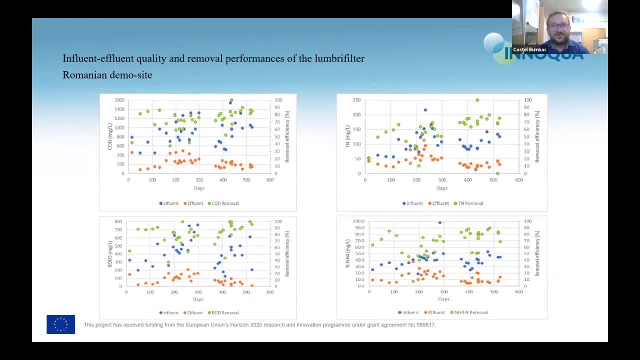 as a solution for the daphnia filter treatment. however, due to some issues with the daphnia's adaptation, as we have used the laboratory-treated daphnia species usually used for ecosystem studies, so your culture of daphnia's- we couldn't assess properly the feasibility of using daphnia filtration. 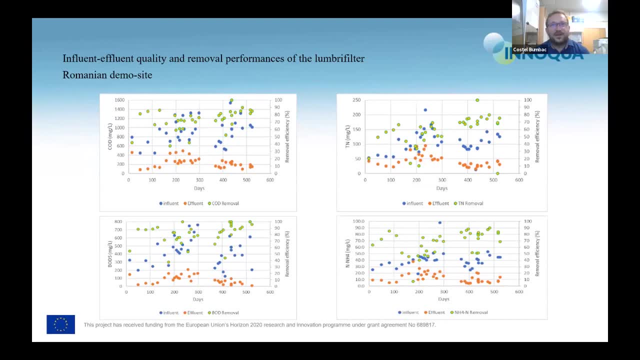 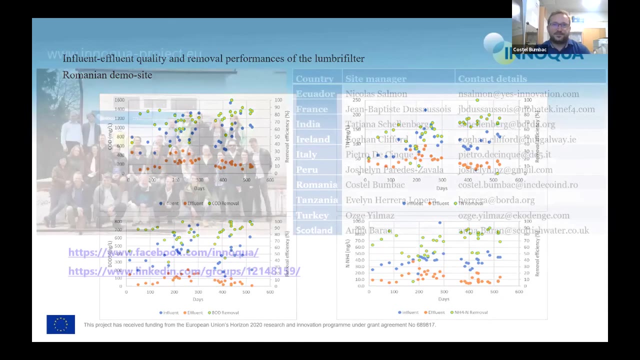 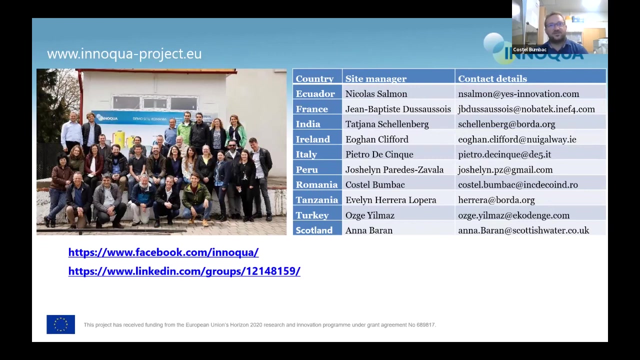 as a polishing step for the specific climate of romania. however, in other demonstration sites, for example in spain, india and peru, daphnia filtration has worked consistently and proved usable. thank you for your attention. you may find here, as i said, contact details of all demo site managers. 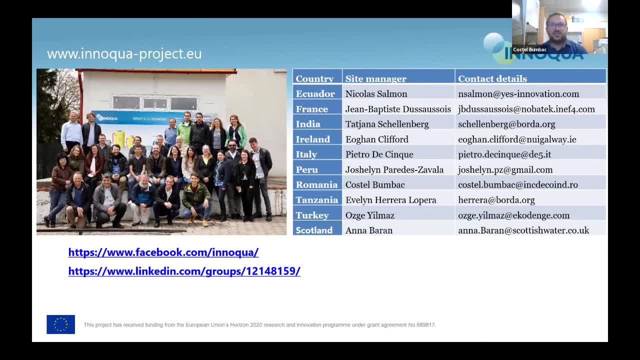 the project website, where you may find additional detailed information on each specific technology or demo site, and the the things for our social media, where you will find project updates and networking opportunities. i would be more than happy to answer any questions. costa, maybe one question from my side. sorry, david, would you like to go first? 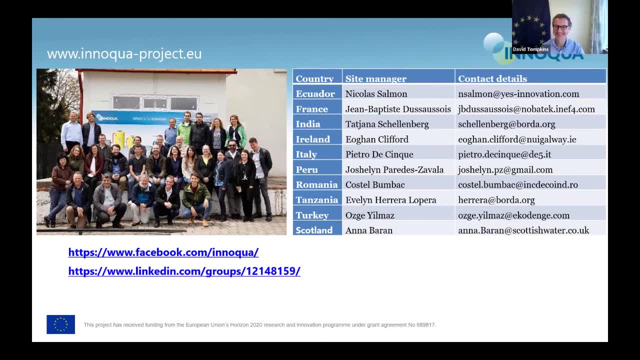 yeah, you go ahead, eska, you okay, thank you. so i was. i was wondering about the legal limits and and and. uh, how, how the, the site, performed in terms of obeying the, the legal limits, what type of parameters you need to look at and what type of discharge conditions that you needed to meet. so, once we adapted the 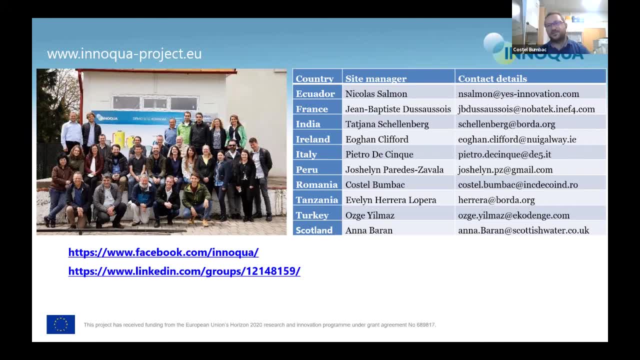 infrared characteristics and the hydraulic load of the system, the system requirements, the systems, the system itself. the lambda performed well and achieved the discharge limits in terms of minimum percentage of nutrients removal in terms of tss, cod and nitrogen. however, it's not really well defined in romania. what are the limits for? 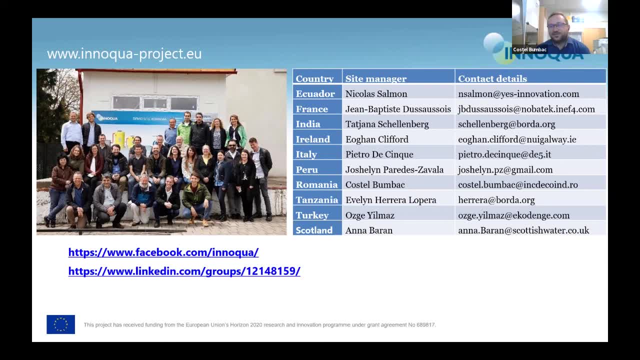 this central, small-scale wastewater treatment systems serving, for example, a flow of equivalent for 10 people. equivalent because the legislation in romania transposes the urban wastewater treatment directive, meaning that addresses the population agglomerations above 2 000 people. equivalent. i see, i see, but, but there's still. there's this: 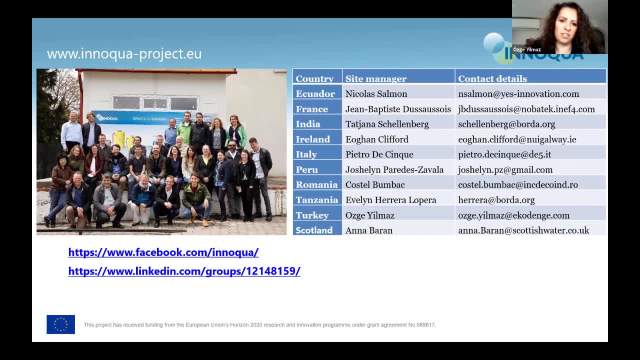 potential to to meet the, the, the, even though if it's not agglomerated, there's still the potential to meet the standards. i can see it met's the standard regulated for a small wastewater treatment plant, meaning 2000 to 10,000 people equivalent. okay, okay, that's good news. 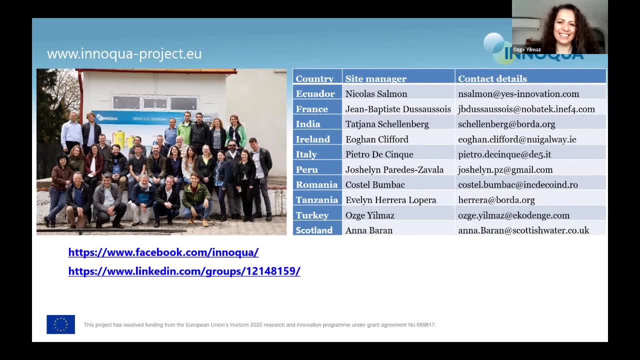 david, please you can ask your question. thank you, it's actually related to that and it's it's two. The first one is the regulations for discharge from septic tanks into water bodies, So I'm assuming that the base case is absolutely compliant with the regulation. And if that is the case, then what is the additional cost of something like the Enoqua solution compared with a simple septic tank and discharged water? So for the first question, I'm not aware of any discharge limits for septic tanks. 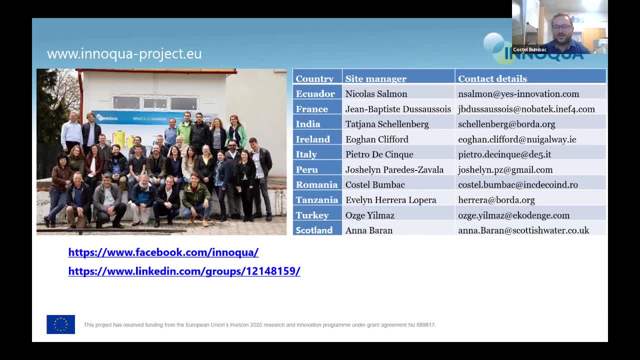 Usually there is the obligation of installing any treatment system which has a technical agreement, So it meets a certain standard, But there is no certain discharge limit for the effluent of that treatment unit. And the second question: It's around cost. So the context is if you simply need to install a septic tank and can discharge to water, 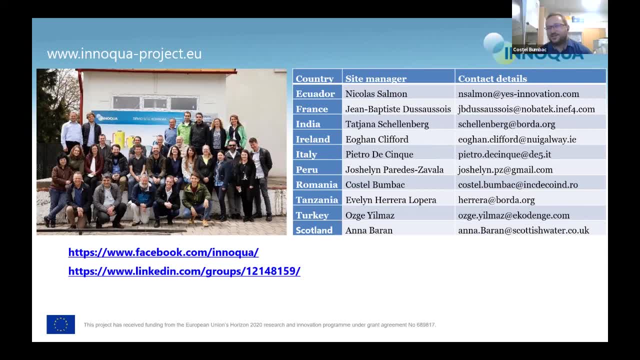 that to me seems a very low cost solution, whereas if you go to Enoqua- Sorry, this is a little tricky question- Meaning that, for example, a lambda filter for 10 people equivalent treating 1.5 cubic meters per day. would cost something like 600 euro, based on European manufacturing. However, this is the cost If you have a pre-settler, meaning that if you reduce the TSS load previously, you may use a smaller footprint lambda filter. However, if you want to go with low wastewater and give the full stream and test the full capacity of the lambda filter, to treat the low wastewater, TSS included. you will need a larger footprint for the lambda filter itself, But even so the cost would be competitive for the septic tank. That's reassuring. So you get better treatment than the septic tank at equivalent cost broadly. 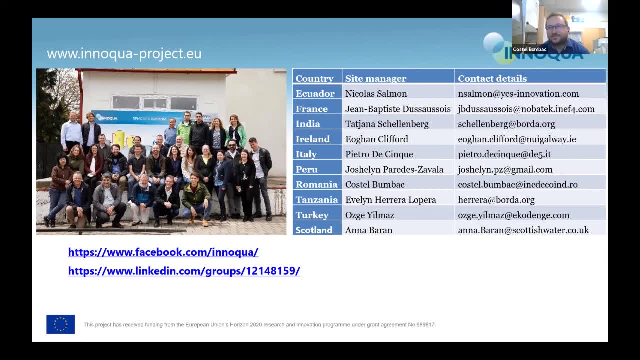 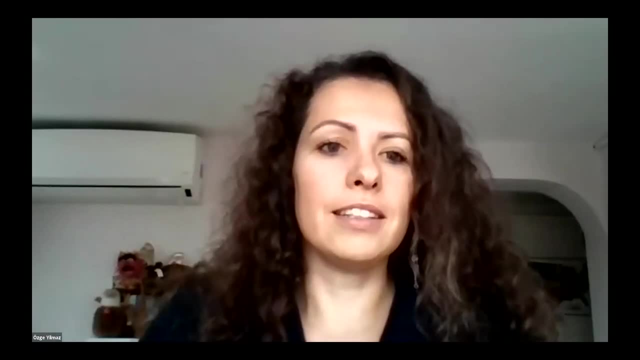 Yes, more or less equivalent. OK, thank you, I'm just checking the audience if there are any other hands that I can see for questions. I guess at this point not, So let us. Yes, please, Volkan Can. 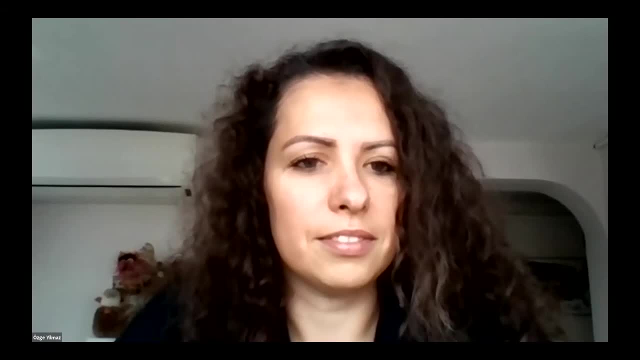 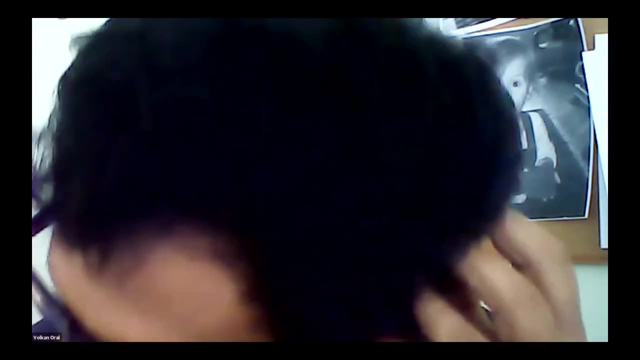 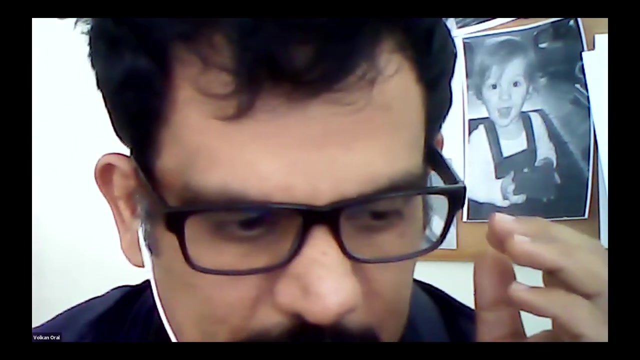 Please Did I mute myself, OK, so can you hear me? Yes, Thank you. Thank you for the wonderful presentations I have heard right now. Thank you, Kostum. Actually, I would like to keep this question for the panel session, but I think it will be asked right at the moment. 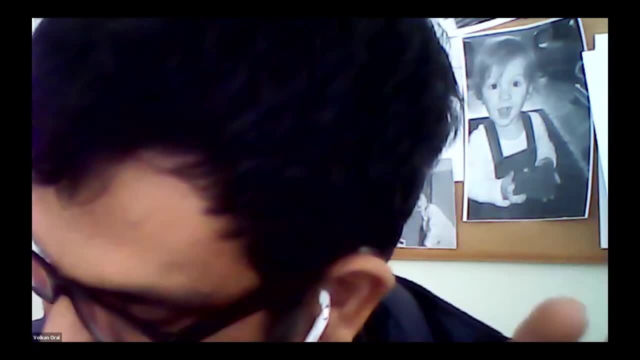 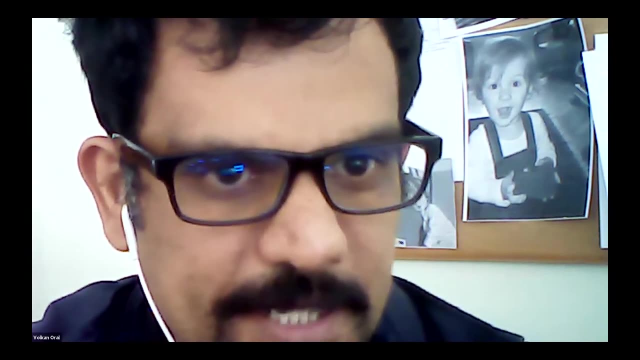 Have you, Have you, you know, compared your results about the discharge conditions, your results with the Turkey, the one, the results you obtained from Turkey? I mean, could you make a comparison with them, Because the geological barriers or the 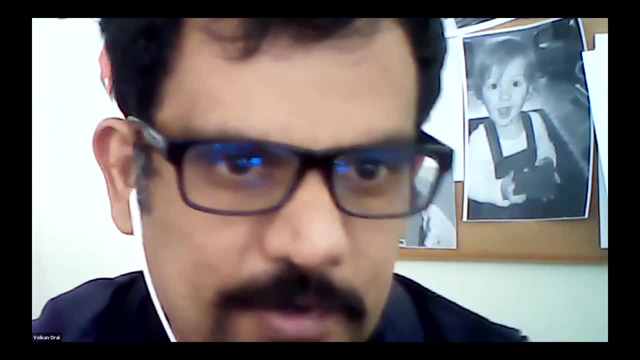 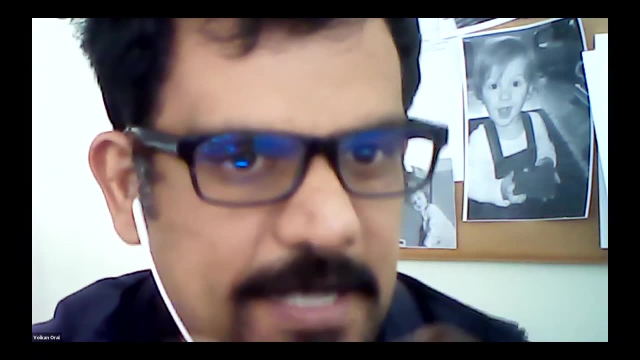 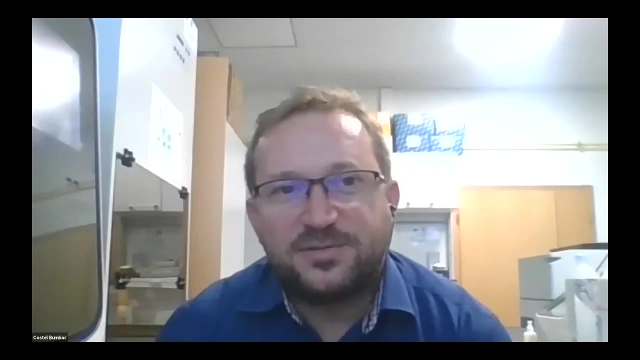 I mean, the locations are also important and climate factor is important, So could you make a comparison with them or could you reach any kind of suggestion? Depends on the corporation. OK, Any comparison between the Romanian and the Turkish performances of the UNOQA system will be forced as each of the demonstration sites have different loading rates in terms of hydraulic and pollutants load. 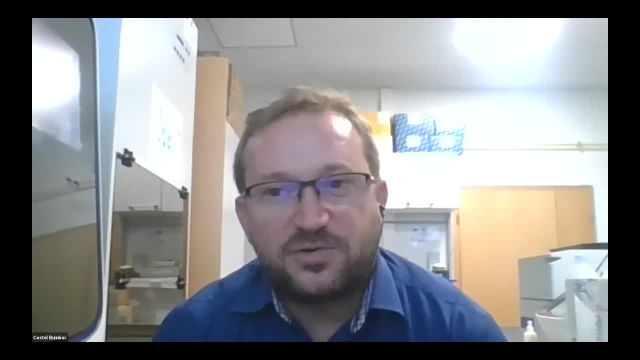 Meaning if the Romanian demonstration site acted with good performance is that If the Romanian demonstration site acted with good performance, is that hydraulic loads of 0.3 cubic meters per square meter per day, given the loads which are indicated, which were, let's say, typical for a high-strength wastewater with concentration of COD above 1,000 milligrams per liter COD. 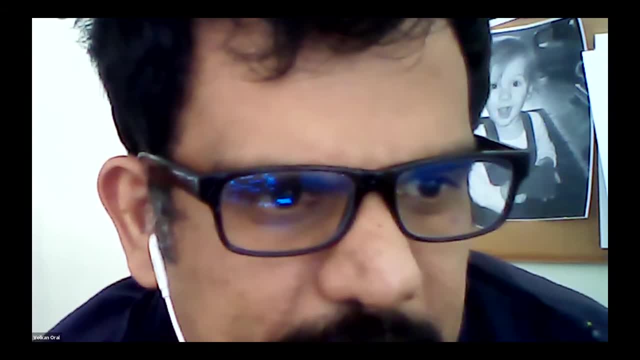 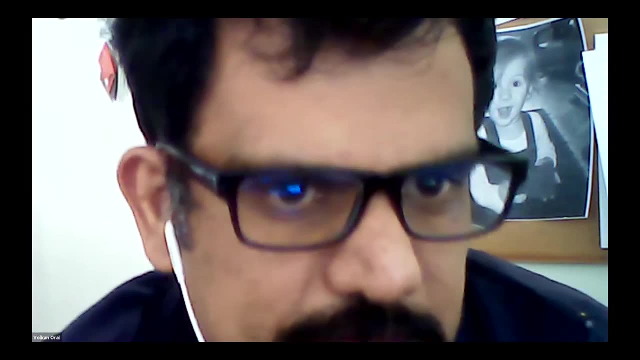 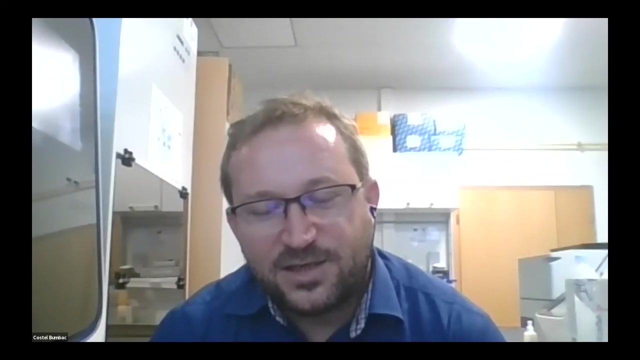 Hydro grades are different, So maybe comparing with them should be taken, or should have taken for other parameters, Not for them. Yes, Even though the hydraulic load and pollutants load were pretty much different. totally opposite, The specific removal rates in terms of grams of COD or grams of PSS per square meter per year. 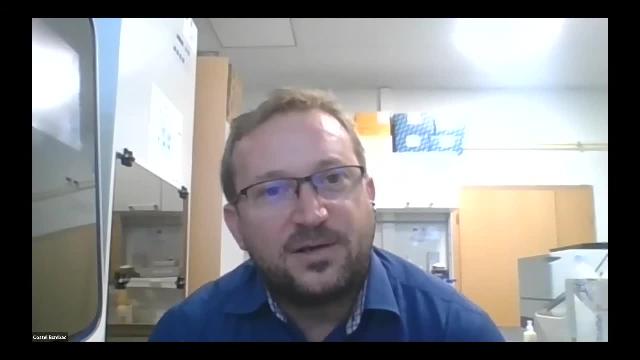 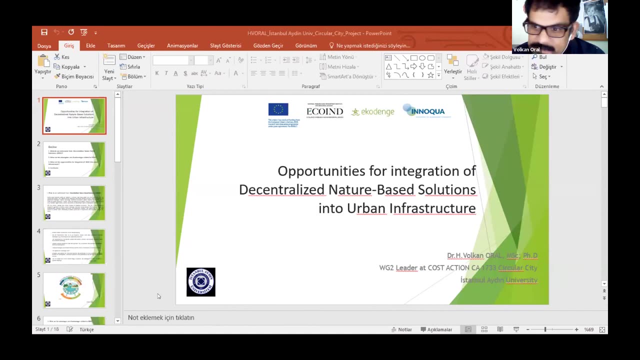 Yes, OK, So the total load of COD per day of reactor were pretty much the same. First of all, thank you so much for presenting and organizing tonight's organization. Actually, I feel myself as a kind of a privileged person to make a presentation here. 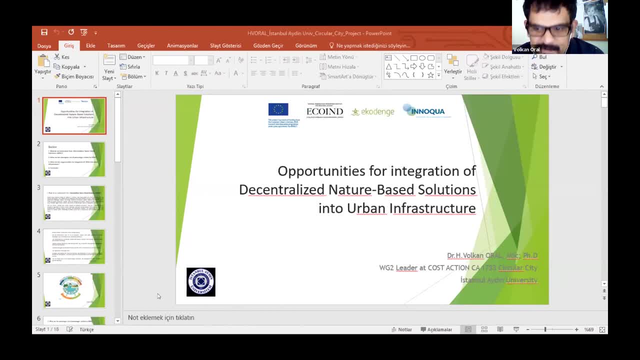 I like the music, by the way. Thank you, Christoph, And thank you, David, And OK, So if you allow me to talk, I would like to say something about opportunities for integration of the UNOQA system. Yes For integration of these samples by nature-based solution. 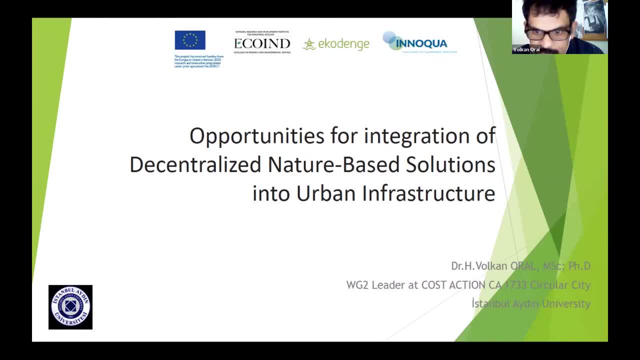 How can we integrate into urban infrastructure? Before starting my presentation, actually, I would like to say also that I'm the member of one of the cross-section which is dealing with nature-based solutions And here in this conference, I will see I'm seeing some of my colleagues. 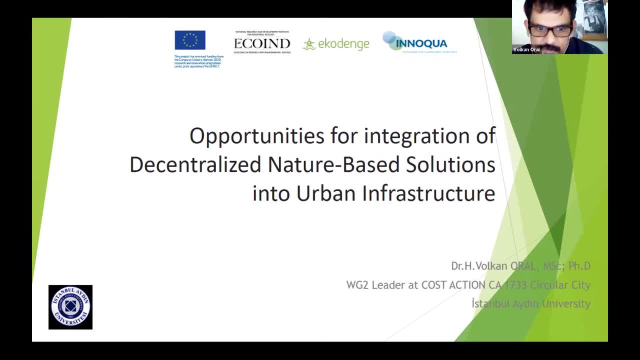 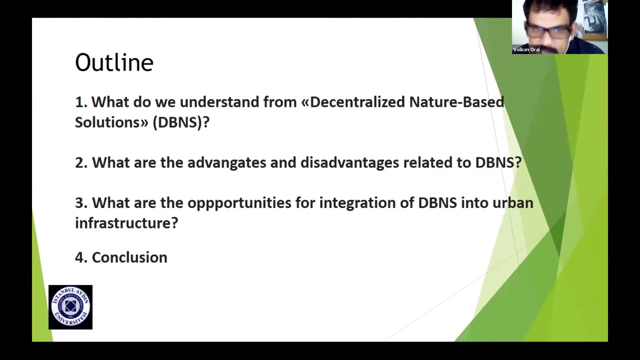 Asman and Sabina. We both, you know, took place and participate the conference we had previously on March in Istanbul. OK, So what is the outline? There are three important topics I would like to share with you know under the outline. 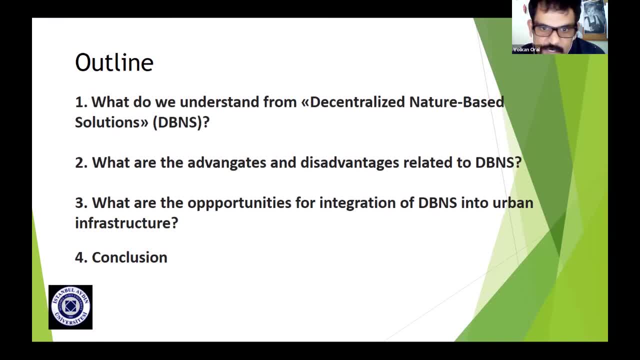 What do we understand from this terminology, What are the advantages and disadvantages And what are the opportunities? And, at last, finally, the conclusion. I will do my best to fit at 15 minutes, as previously informed me. Number one is, I think, the most important thing that we need to define, because here in the cross-section we're still working on to define out the meaning of MDS. 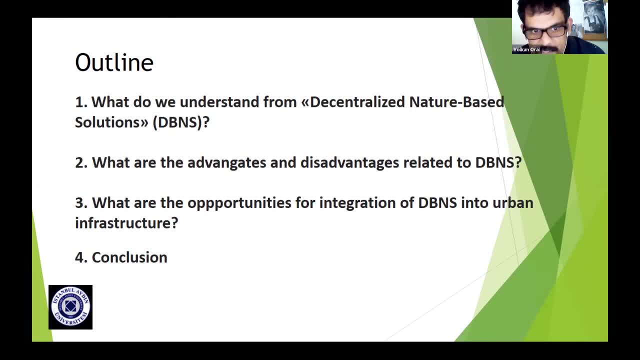 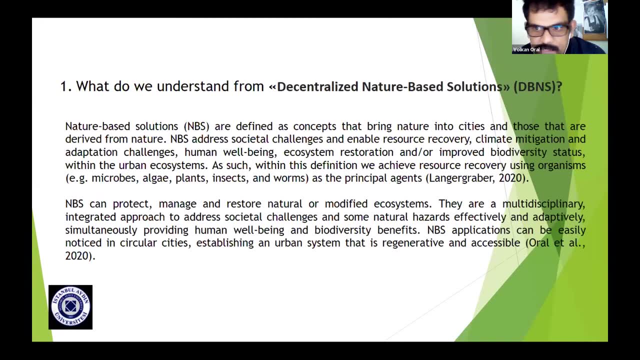 So this is why, you know, I left a special part for this topic. OK, You could see two definitions. One is already made by, you know are also the cross-section chair, Gunter Langedaber, And also I made a citation of my article, which is also published on the cross-section. 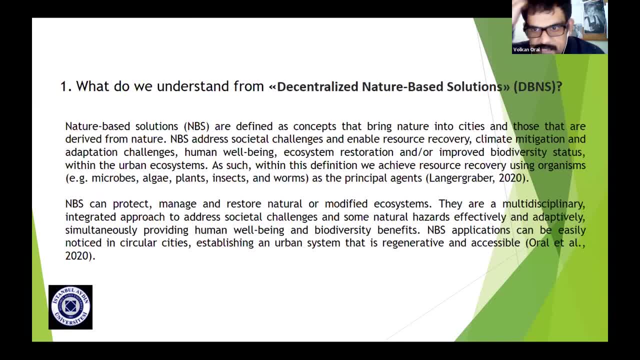 But briefly, MDS are defined as concepts that bring nature into distinct and understandable form, And MDS address social challenges and enable resource recovery and other environmental solutions to the problem. But still, let me now highlight: During the panel, I also would like to hear your comments. 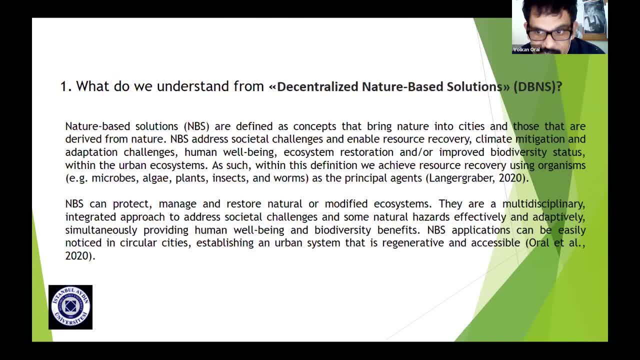 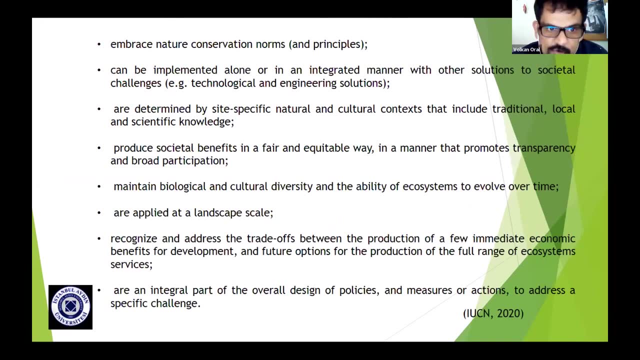 The exact definition of the MDS still cannot be done because there are so many aspects could be taken places or could be taken under these concepts. OK, So there are also some aspects related to the MDS. They embrace nature conservation norms. They produce social benefits in a fair and equitable way. 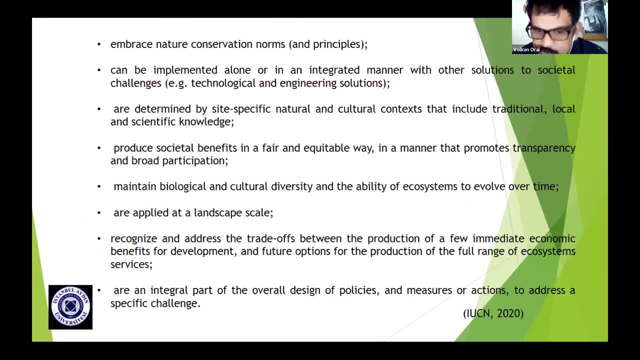 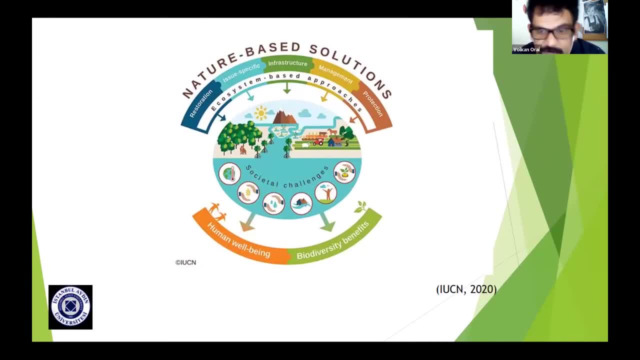 They are applied at the landscape scale And they are integral parts of the overall design of policies and measures or actions on a specific challenge. As you may already know, there is a most-term standard one-man figure that relates to MDS or nature-based solutions. 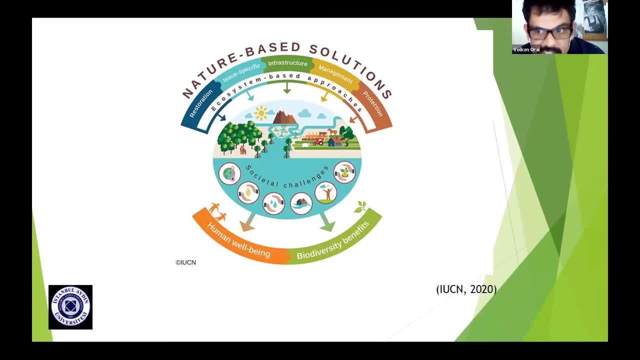 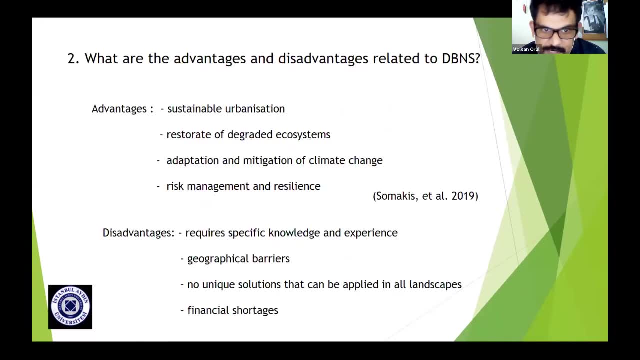 You can see the types and you can see the approach And, in the end, you can see the outcomes or the benefits. what shall we say? I mean the human well-being and biodiversity benefits. So what are the advantages and the disadvantages related to DD? 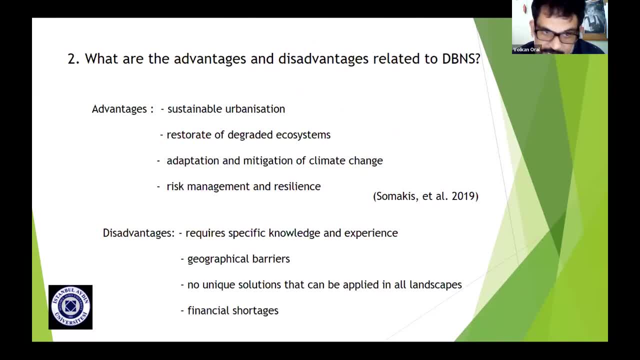 You know the advantage. we can see that and we can say also the sustainable urbanization, respite of the degraded ecosystems, adaptation and mitigation of climate change, risk management and resilience. Actually, according to me, the last two parts- I'm talking about the resilience and adaptation and mitigation of the climate change- are the utmost important things in here. 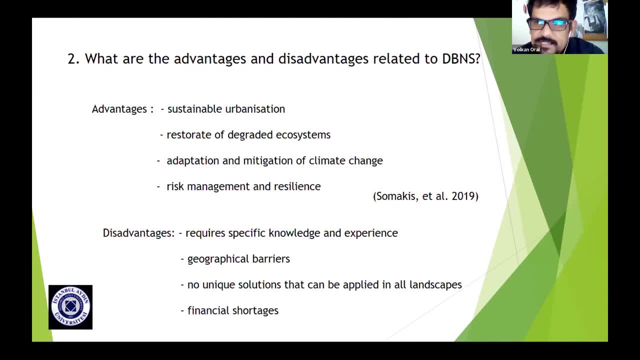 But also there are some disadvantages, because you know MDS are not the. you know the knee or the toe. You know they're not the toe, They're not the toe. They're not the knee or the toe, They're not the toe. 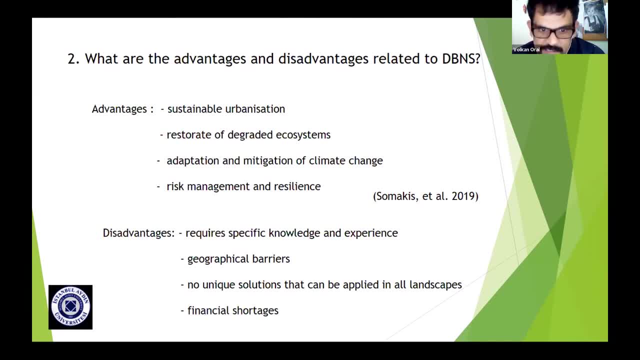 You know, and these are the advantages. you know the knee or emerge. you know terminology which has been discussed in the last 10 years And, of course, these are the you know. it requires past knowledge and experience. 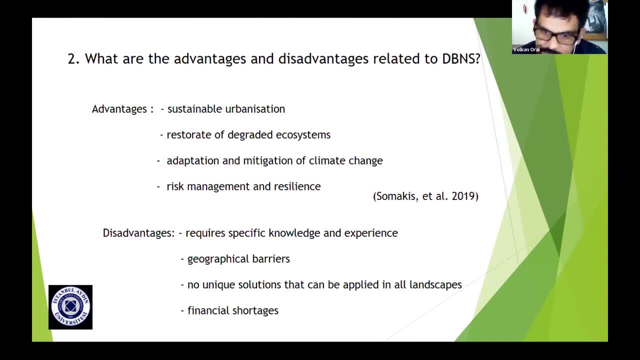 There are also some geographical barriers. There is no unique solution that can be applied in all landscapes and, of course, you know financial shortage, Or you can say: money, money, money is in the shortest form, Okay. So what are the opportunities for integration of DD and as into urban infrastructure as it does? 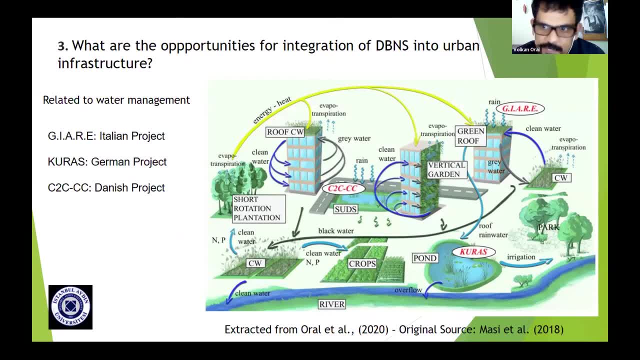 infrastructure. related to this concept, I would like to say something in, you know, under two groups. one is related to water management, and I can also give an example about some other projects which are currently being done, already finished horizon 2020 projects. okay, actually, I would like. 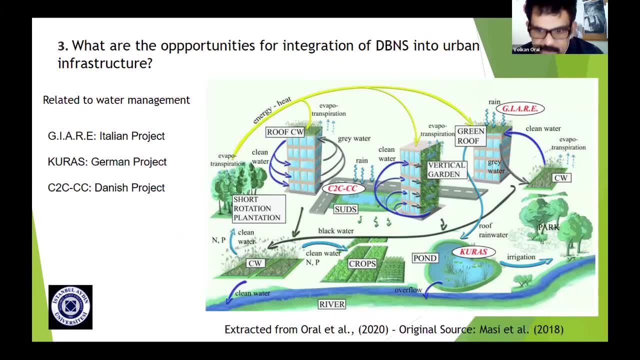 to share the figure which I also used. my paper and also the original source was made by one of our colleagues, Fabio Mazzi, from Italy. okay, if you pay attention on the figure, you could see that the opportunity for integration of CB&S into urban structures are dealing with. you know the. 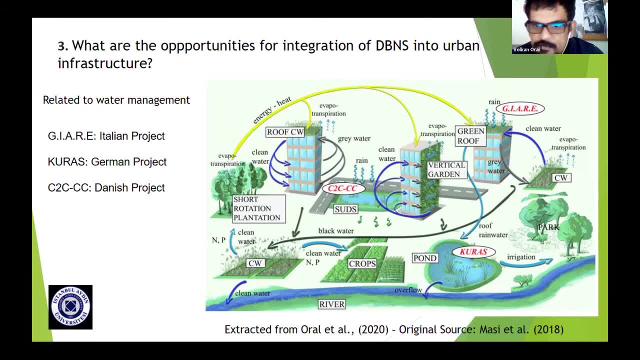 vertical gardens or reusing the waters again from the buildings directly to the agricultural field and used as an irrigation of water, and also the project you know the Italian, German and the Danish projects are currently using these. you know tools as a kind of a reach about the 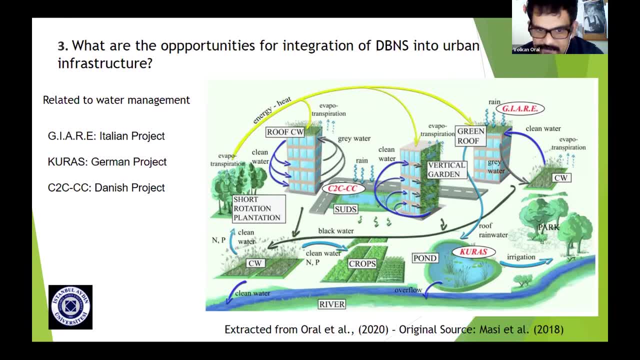 direct aims of the MBN. but what is important here? if you pay attention on the bottom of the figure, you could see a kind of an agricultural irrigation is also one of the important things that we can say. something related to water management and DB&S can contribute the urban landscape there. 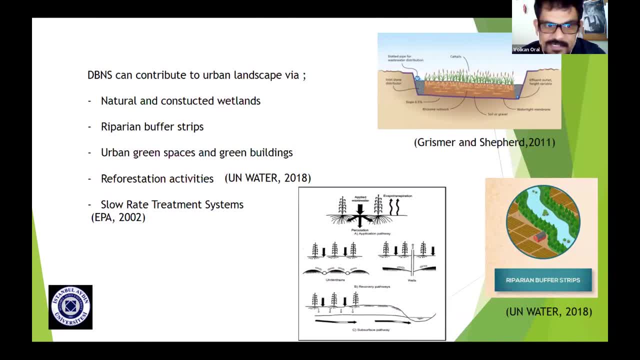 you know five important things. I would like to say that the nature and constructed flatlands, the perrine buffer streets, urban buildings and the green pine and the bird outflow on the control area and the green potted reduction on the landscape there are. you know, five important things. I would like to say that the nature and constructed flatlands, the perrine buffer streets, urban. 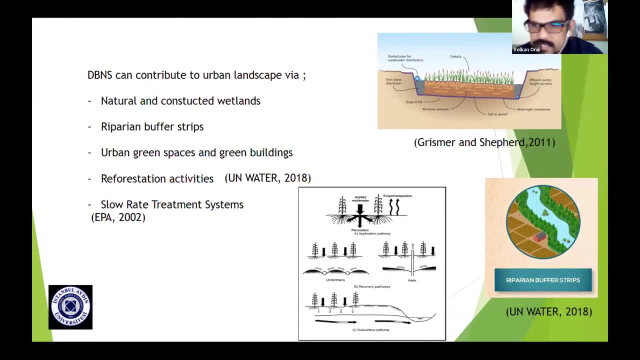 green spaces and green buildings and reforestation activities. but there is one more thing i would like to share. as you know previously, you know, uh, our colleagues mentioned about the two demonstrated sites, one in turkey and one in romania, actually under, basically, they're trying to relate it with 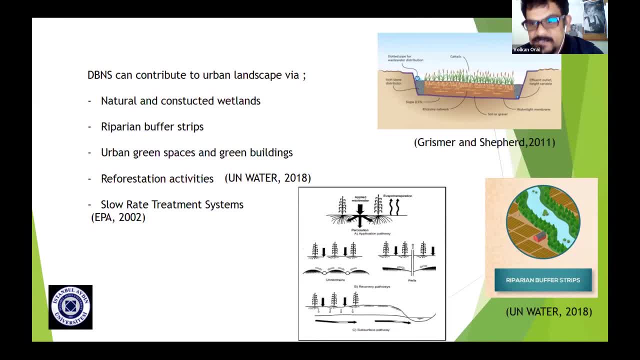 a kind of a slow trade, uh, that slow rate treatment system. so we can say that these types of envy is the kind of improvement methods or it's based on slow rate treatment. but of course there are some modifications and implications are going on, but basically we should say that, uh, it was the. 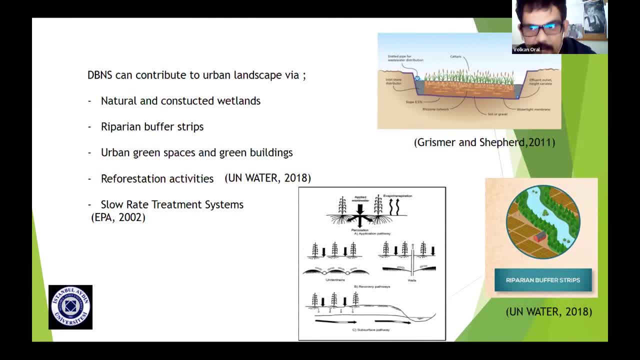 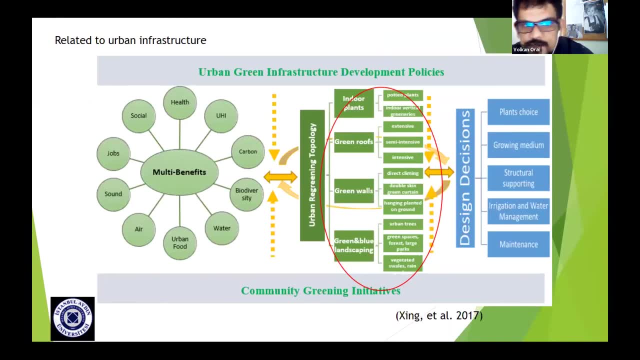 first we deal about the slow rate treatment systems. time by time it's developed, and now we're speaking something about the nature-based solution and related to the urban infrastructure. i would like to share a figure which is about a diet by a chinese researcher. actually, i made a circle with the red red phone and on the red phones you can see green rules and 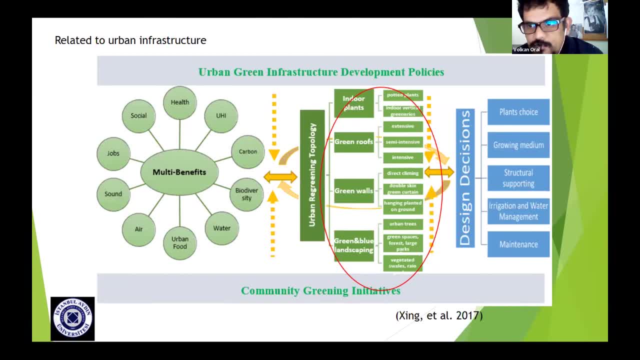 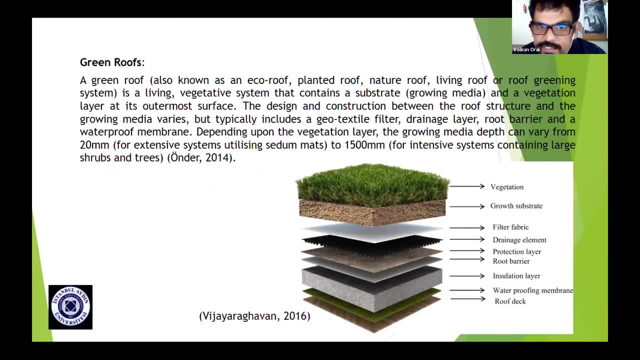 green walls they are in. according to me, they are the most important. you know the examples of related to urban infrastructure and green room, with the kind of, and also known as the eco roof or the planted foods, and you can see on the figure there are some layers. actually it's very convenient. 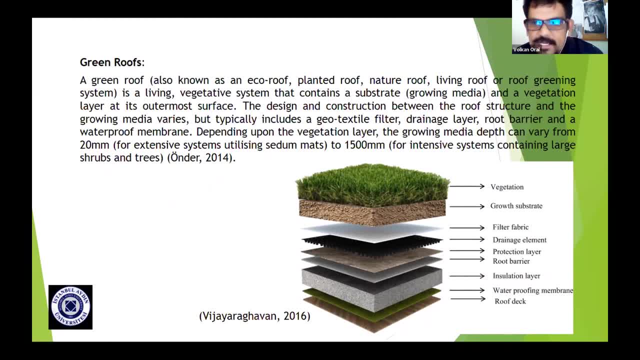 and feasible use and you can see and nowadays in many you know the locations and the locations in all over Europe. in some you know locations in the world. actually, the vegetation layer is so important because couple of months ago I read the news from China and they use the green roof. but the wrong types of the meditation. 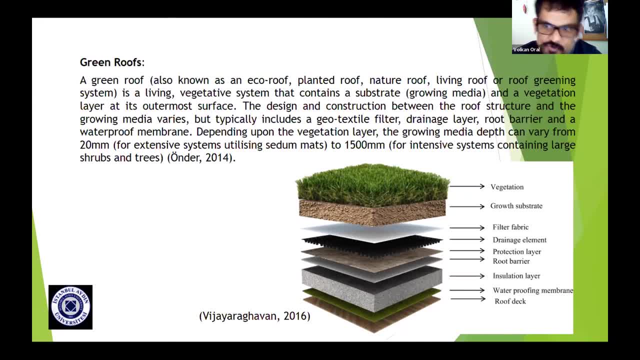 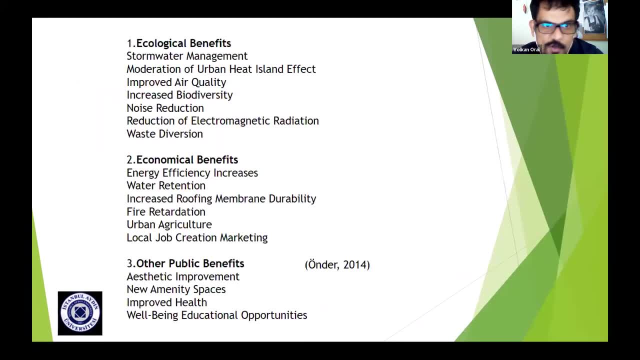 made some you know troubles about. you know the root- cohesion and root problems or some kind of dewatering problems in the building structure. and also the benefits. there are three types of benefits: ecological benefits, ecological benefits and other public benefits. and as for the ecological benefits, of course that relates to water management, storm water management, that 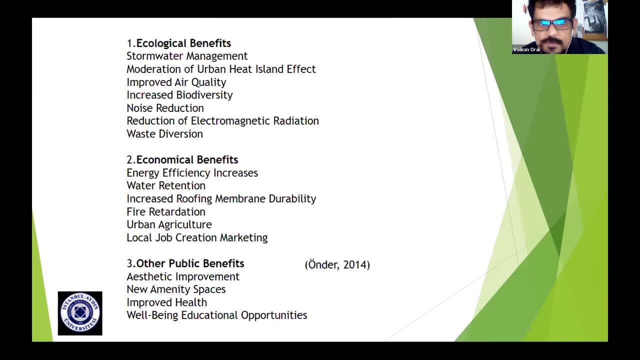 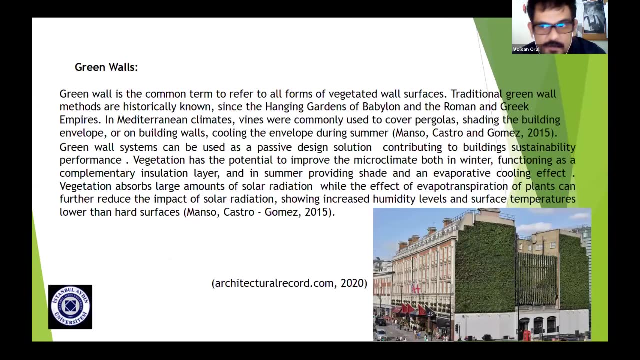 we can say: first, improve the air quality. and for the economical benefits- fire retardation, urban agriculture- which are so popular right now, today, then other public benefits. you know the static improvement, improved health, well-being, educational opportunities, green wall- it's coming from the, the history. I mean it's not a new thing, but you know using 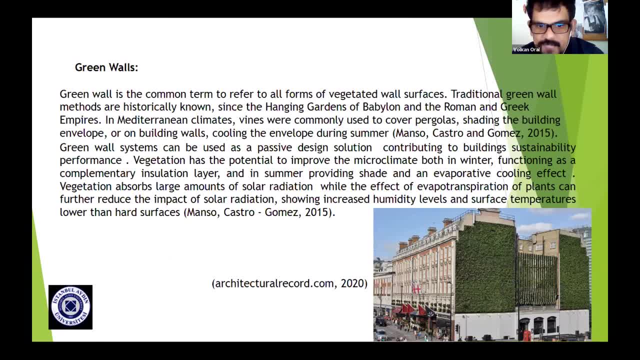 only a vegetative side, or the vegetation side and, according to you know, the architectural point of, also, the aesthetical values are so high. but also, during the hot summer, it provides us, you know, providing some kind of, you know, shade opportunity and because of the evaporation take place on the surfaces. 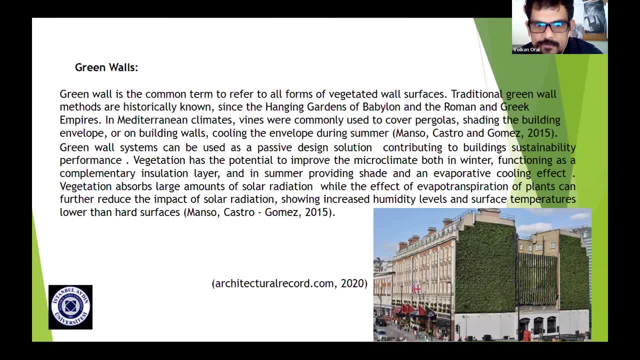 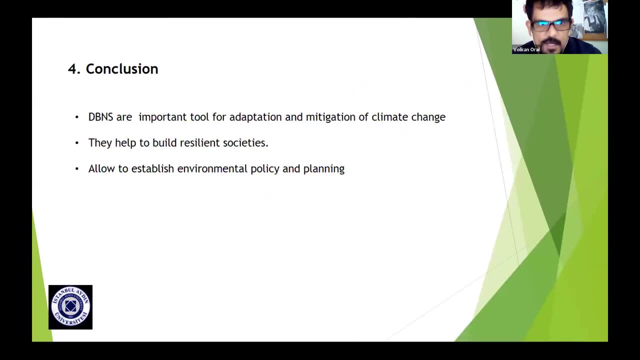 if you, it is a kind of the, you know the, some kind of to be used on the walls of some buildings, okay, and the main idea is vegetation absorbs large amounts of solar radiation and the wildly effect of aws transpiration, if you know this with you, okay. so in the conclusion, i should like to- i would like to be a kind of simple as i can. 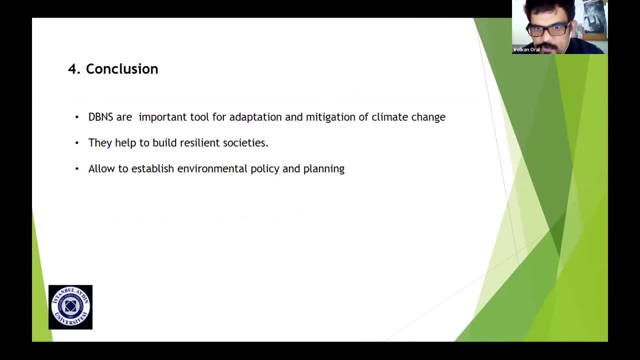 these are the important tools for adaptation and mitigation of the climate change. of course, you can insert something under this one and the most important for me. they help to build resilient societies and allow to establish environmental policy and climate. these are diverse. i would like to share it here with you, and this is the references and this is the internet. 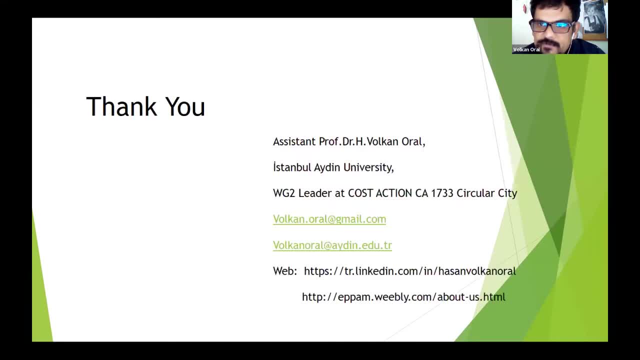 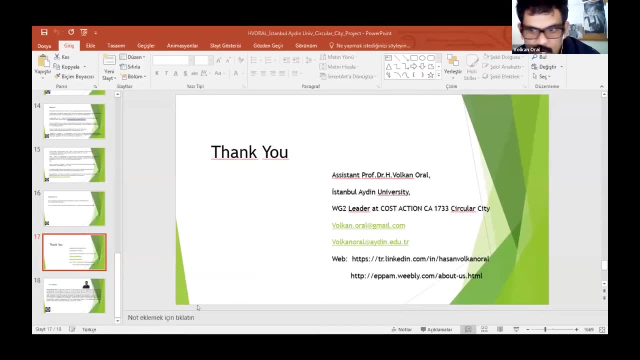 sources i use. if you want to address me any more questions, i'm here, thank you. thank you. first i would like to ask one question, maybe two, because this is. this is very interesting topic and, uh, you presented very well about especially the multiple benefits of mvs. 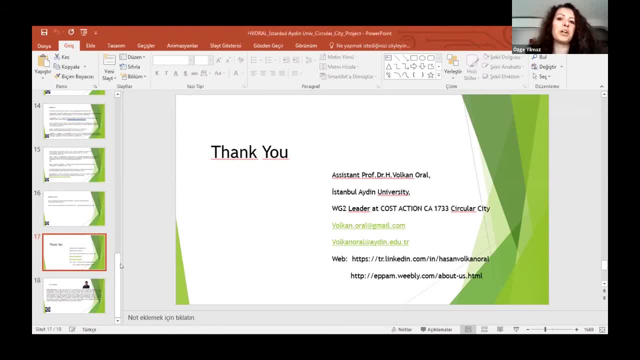 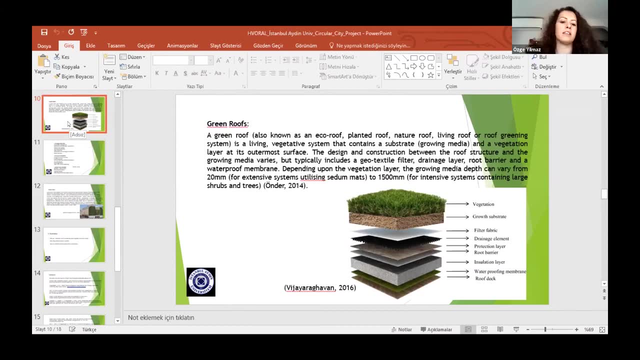 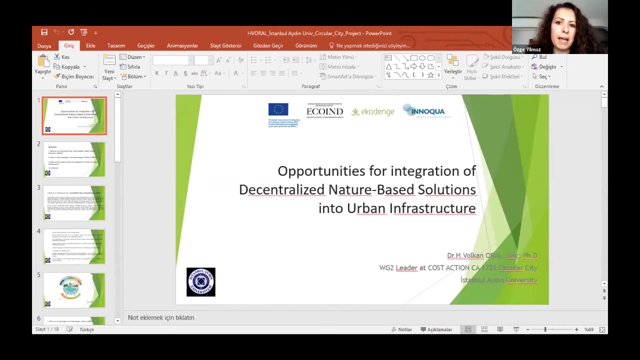 because this is something that we should also be aware of. not only we are gaining environmental benefits when we apply nature-based solutions, whether within the cities or in rural areas there, there are always multiple benefits: societal benefits and economic benefits as well. so you mentioned the importance of selecting the way. 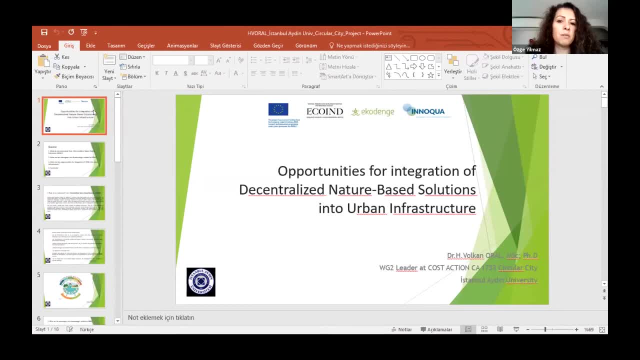 also, it can also cause some structural problems as well because, for example, in another horizon project, we are working on the cultural heritage and implementation of mbs to up to a certain extent. so it's important to choose what type of system we are implementing, whether if it's green roofs or green facade, based on some conditions, local conditions. i. 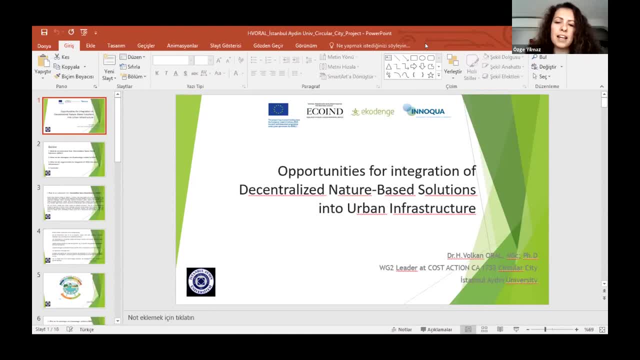 guess. can you give some examples how we can determine these type of conditions? thank you, okay. these types of conditions, as i told you before you know, depends on the geographical conditions. for instance, if you run a project in, in greece, for instance, i would like to give a project. 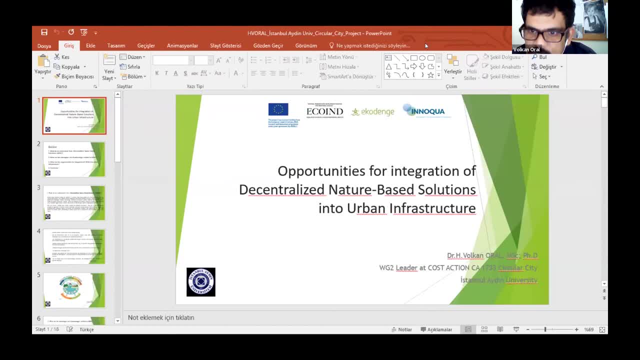 named hydro usa is going on in greece. you need to pay attention to local conditions, so the local conditions on the microclimatic effects, you need to pay attention, of course, that the one that you will pay attention on in denmark, on the northern, you know, the peninsula, or the northern area, or the 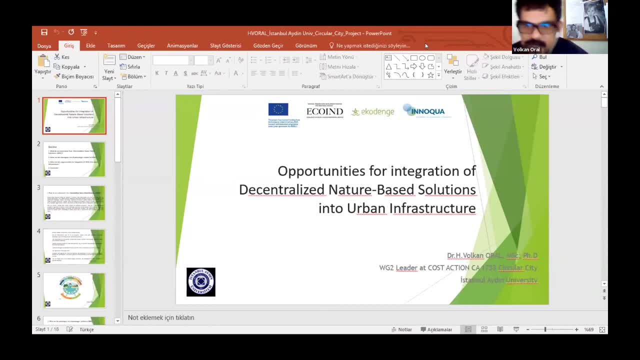 one that you will attention in greece or the mediterranean area are totally different. there is also one thing which i noticed during running other projects: the some kind of you know, the cultural experiences are important because you know people are used to do this is coming from. 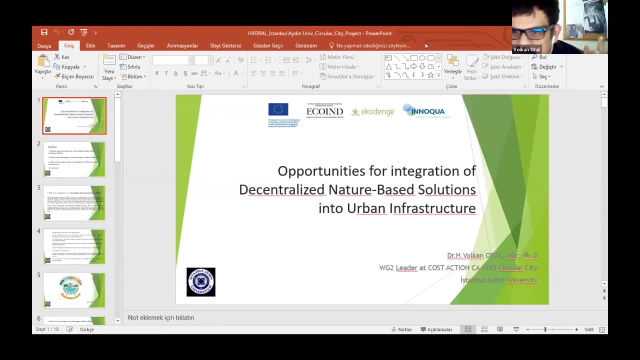 the story. they are nothing so new for them, as i told you before, what you do as a kind of a demonstration area, 20 years ago we already mentioned some kind of slow rate treatment system, the kind of an employment way. so cultural points and the cultural notifications are. 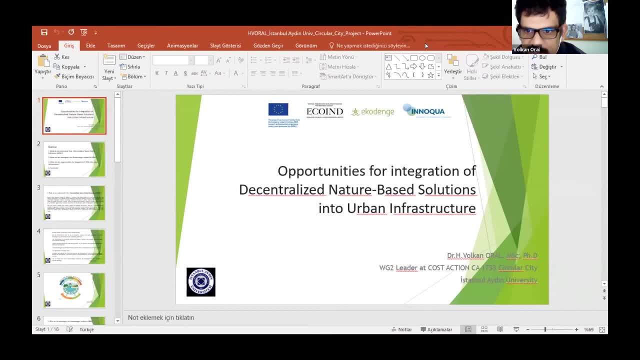 important. do you have any more questions? are you told that there are two more questions or one you already addressed? let me just give the floor to the participants. if any other questions we have, then if not, i will ask my second question. okay, thank you. thanks a lot, yep. 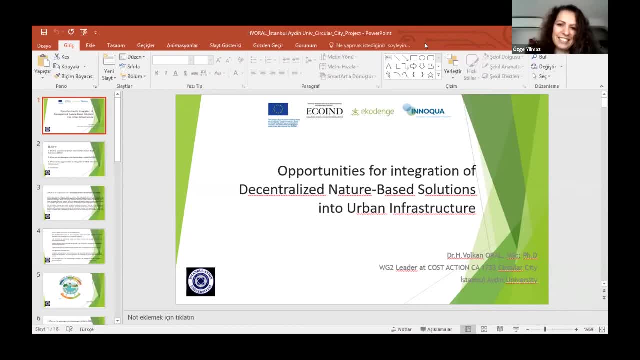 yes, please, david. uh, yeah, and it's a question on definitions. so, for example, would a septic tank be a nature-based solution, because you're relying, yes, on physical settlement, but also on biological activity in that system? well, well, okay, if you address about the definition related to septic tank. 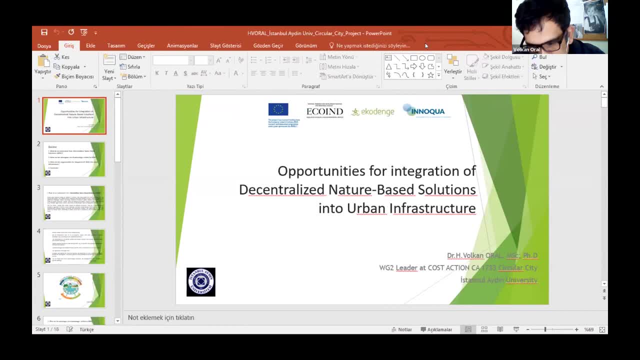 what shall we say about the nature-based solution? nature-based solutions, the kind of thing that i mean reducing the amounts of the pollution- maybe could be taking place, but this definition can be also only related to the environmental impact of septic tanks. so what i'm saying is that if you, if you. 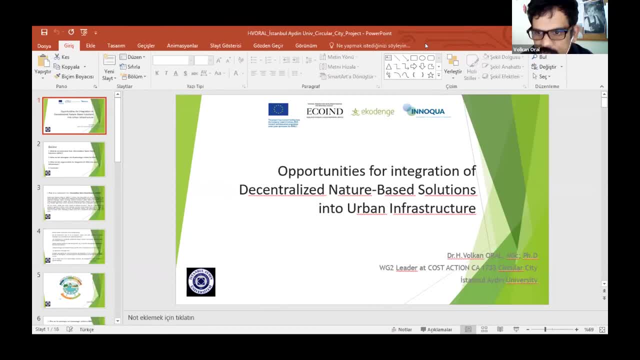 put on the septic tank as a focal focal point. but if you use any kind of other thing, that of course you need to change the mbs. you know the definitions of the mbs so it can be- you know- adaptable or it can be changeable. what i say to you depends on the point you address. this is what i think, but 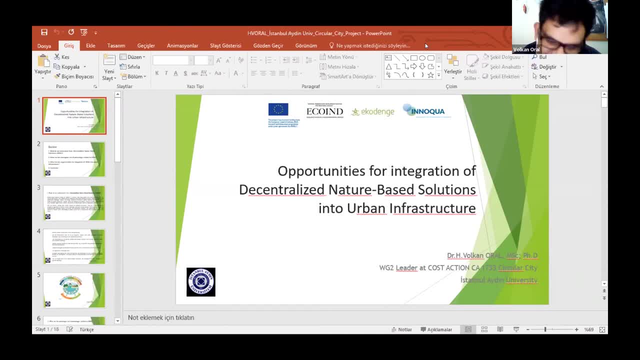 i mean, but i mean, believe me, that this is the most difficult thing, that we are dealing with our current questions right at the moment. we still couldn't find one unique or the one common. i mean, the definition is accepted by everyone, even for writing state of the art papers. 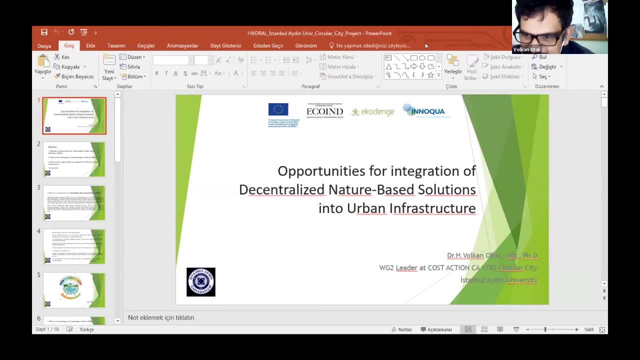 this is the problem we are currently having, sure, thank you, i apologize, it's a bit of a cheeky question we have. we have the same. we have the same issue with with definition of decentralized. i mean decentralized on-site non-sewered. what do we mean? what do we mean? and? 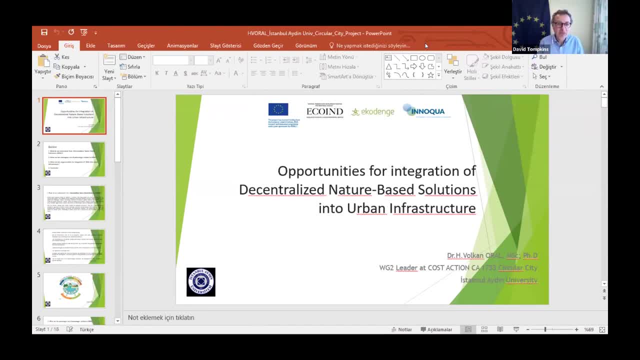 and really is it important at the end of the day? well, i mean, i mean, if you're looking at the literature survey, you could see that you can. you can categorize some papers on the decentralize, but some, some papers are not mentioning about this one. but if you look at the 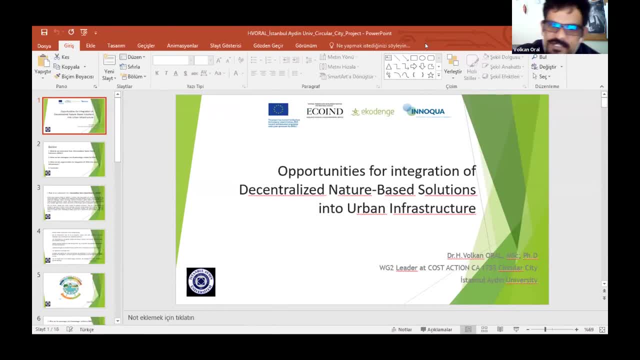 european union. you know the report and most reports. you could see the decentralization nature page, so maybe, maybe you could ask your question by yourself. okay, so in in what terminology should i deal with decentralize? or you know, because when you propose me to make a presentation, this one i 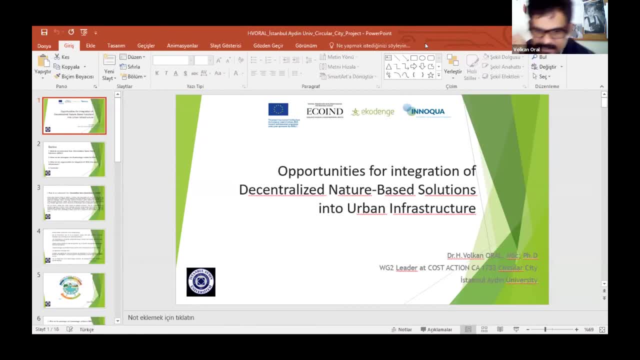 saw the. you know the title and i i asked myself the same question: which type of mbs should i focus on? which type of mbs should i, you know, put and try to be as simple as i can- to share the audio. okay, thank you, you're welcome. so, um, okay, you, you're supposed to have the another question. 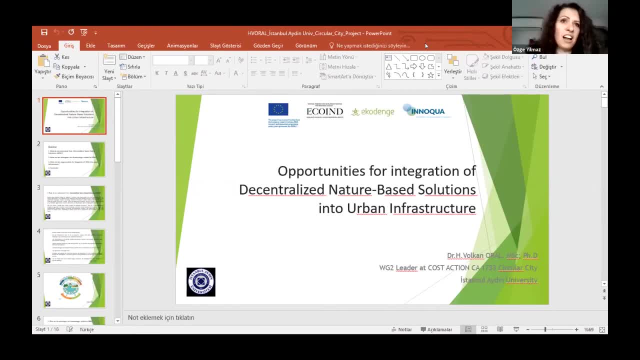 i think, yeah, it's, it's actually uh, i, i, i really was interested in the topic and the presentation itself, because, you know, we are talking about mbs and the water management uh, but of course, uh, whether it's rural setting or urban settings, uh, when we think about water management, mbs, 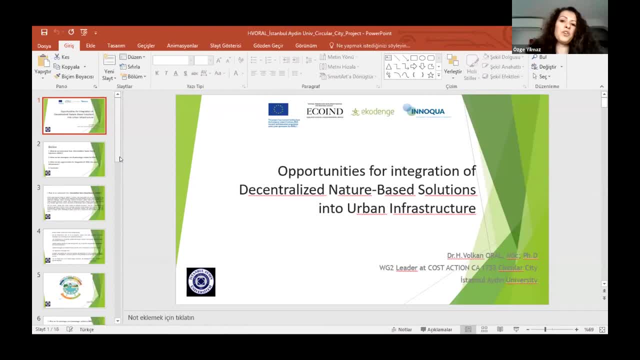 offers a lot of different opportunities. so you mentioned- uh, you, you selected very nicely the green roofs, green facade type of mbs which can be implemented in the cities. uh, maybe a little bit more easier than some other mbs, but of course there's this water management. 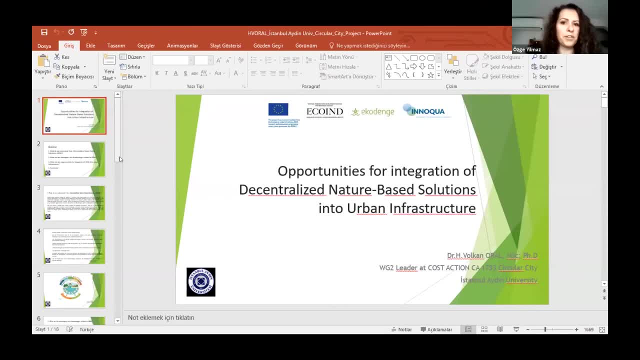 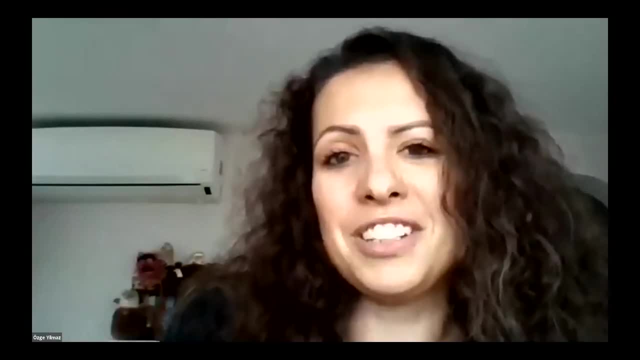 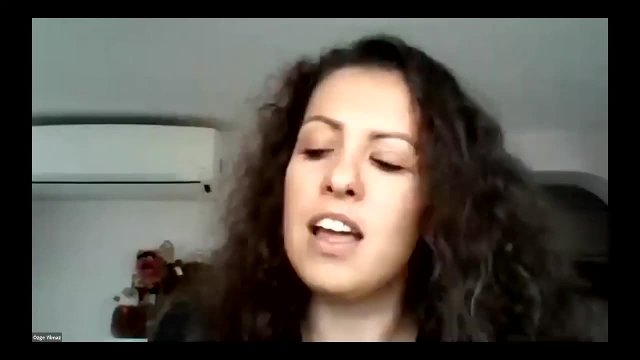 part of it because, when we look at it from a life cycle point of view, uh, when we implement a green facade or roof, there might be some, uh, irrigation requirements, so that means we are in, in fact, increasing the water consumption of, let's say, the, the building itself. uh what? my second question was: 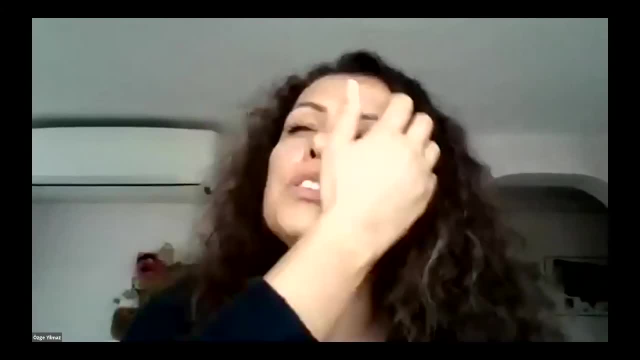 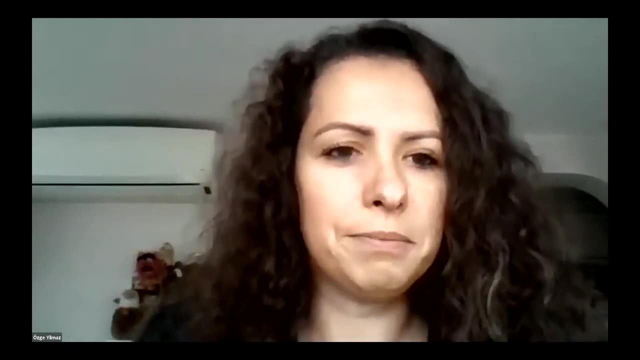 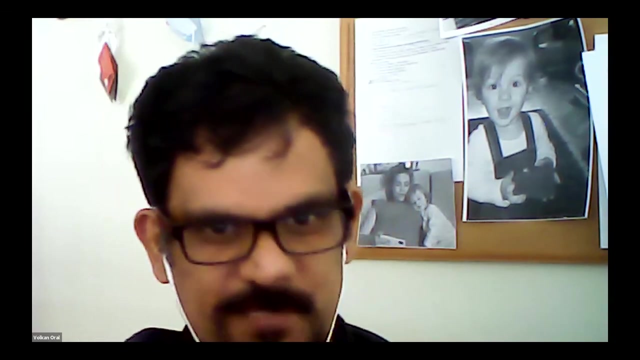 uh, how do you see the potential to to combine this type of mbs with some kind of rain harvesting? well, it could be possible. it could be possible, or what? what shall we say? that rain harvesting matters should be the right, the right term that you know? maybe you know it means the answer of 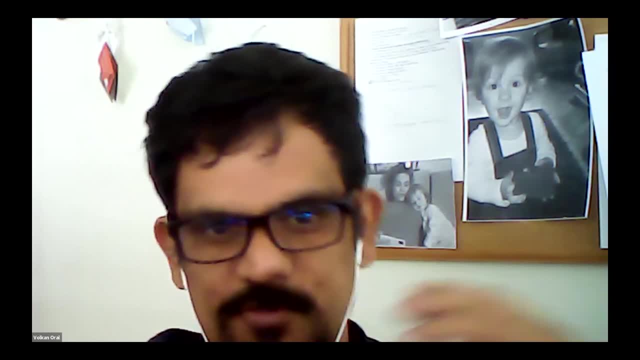 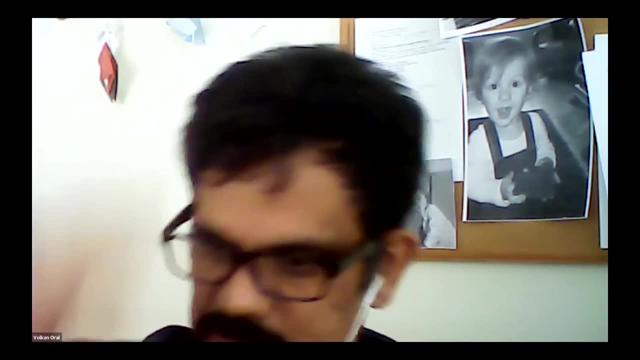 your question. i see the high potential. i see the high potential but on the other hand, maybe I mean it would, if you want to, you know, adapt it on a kind of a top of the, you know, the building. I think there are some also other properties below the the uh construction or the building very. 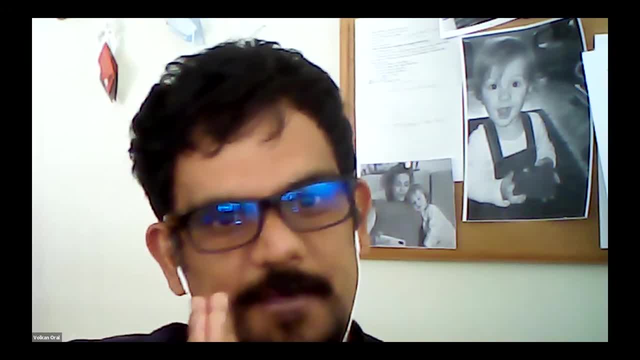 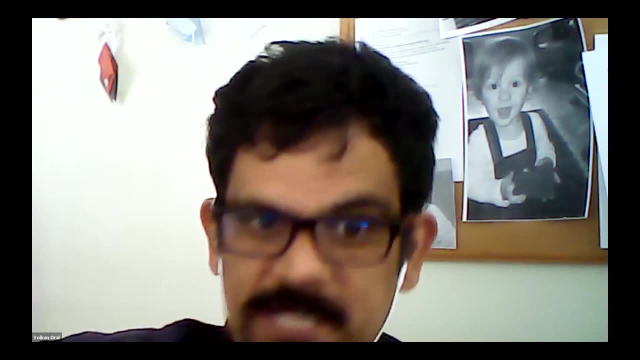 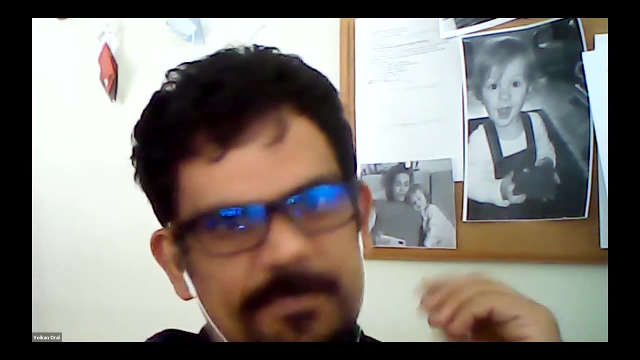 in theory yet, and in the theoretical aspects, yeah, I mean, I see a huge potential to be implemented, uh, in cities, for instance. if I'm not mistaken, I live in Istanbul. actually, in in some some part of the you know, the European, European side, some companies you know started to do as a kind of thing. 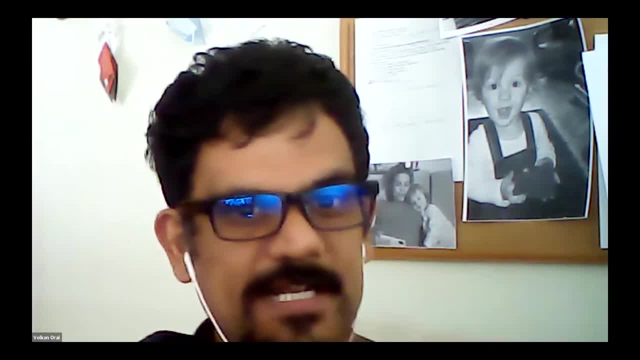 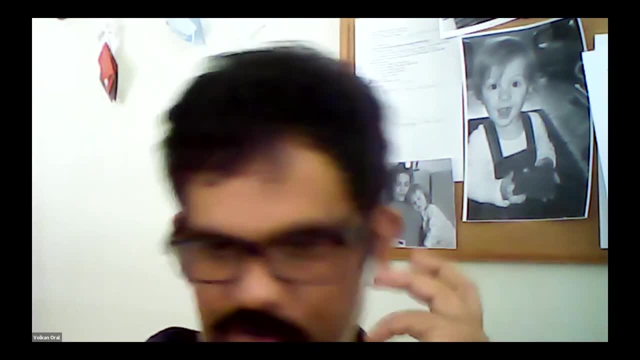 you know the implementation, things related with the harvesting grain and use the kind of mbs purposes. but uh, if you ask about the about or for Turkey, it's a very you know um the novel approach. but in theory, yes, there's a you know high potential to. 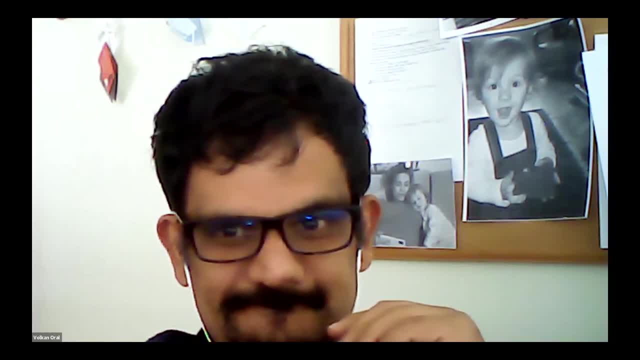 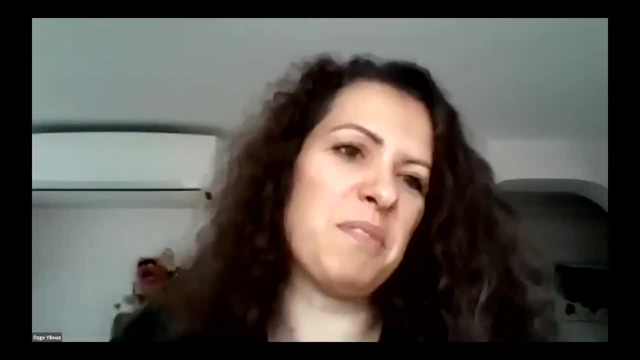 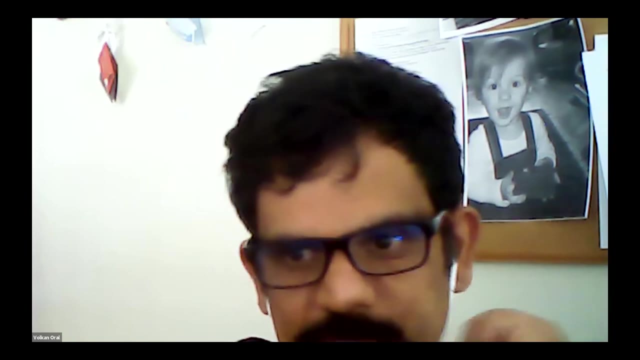 implement this? yeah, I guess it still depends on the local conditions, right? maybe the selection of the vegetation, maybe you're not implementing grass or something that may need a lot of water, maybe I mean selecting the vegetation, if you, if you say about the selecting the vegetation, the 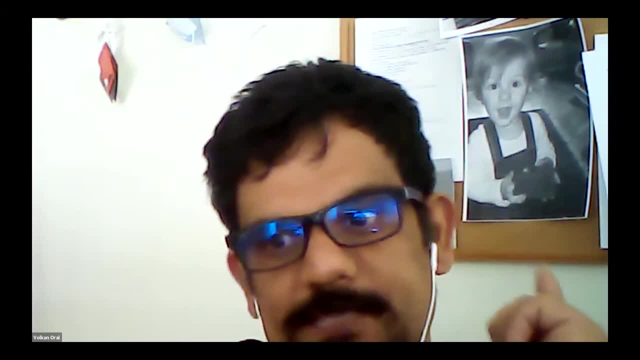 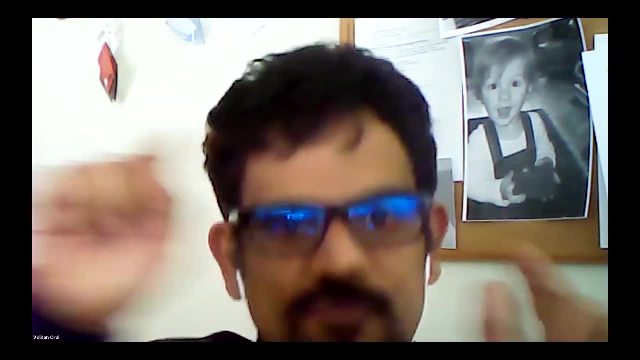 root component is important because, as you know, I'm in the. in some kind of the plants which we plant with annually, or the weed or kind of the, you know the vegetation, their root systems comes in a conical shape. so the root system is important and on the 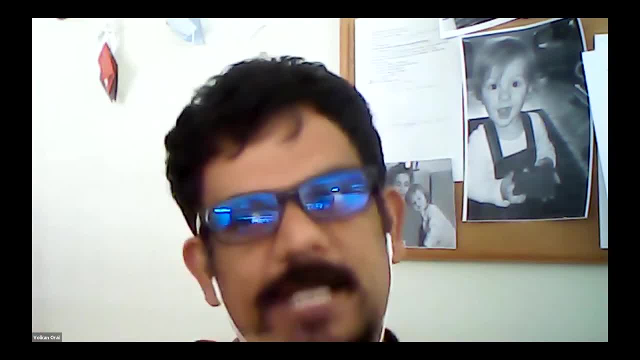 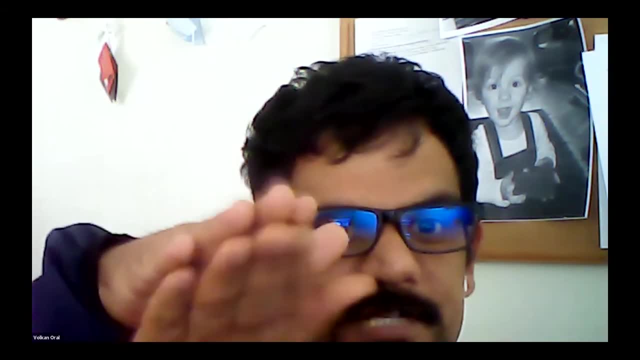 other hand- maybe it's a kind of a technical approach, but I can say this, depending on my agricultural engineering background- the stomatal capacities which are, you know, taking places under the leave, they're also important. so about transpiration, the root, you know the performance, all the stomatal activities. 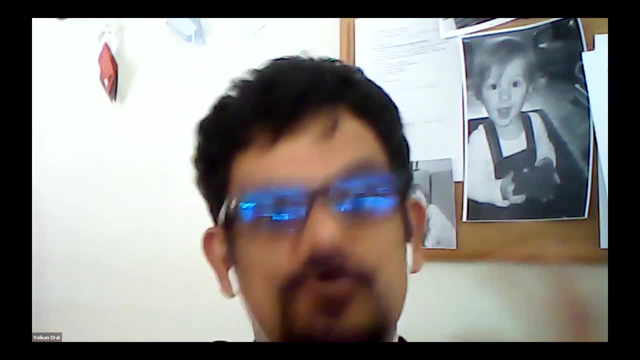 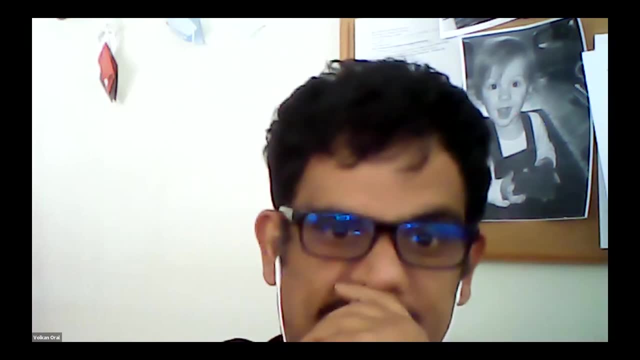 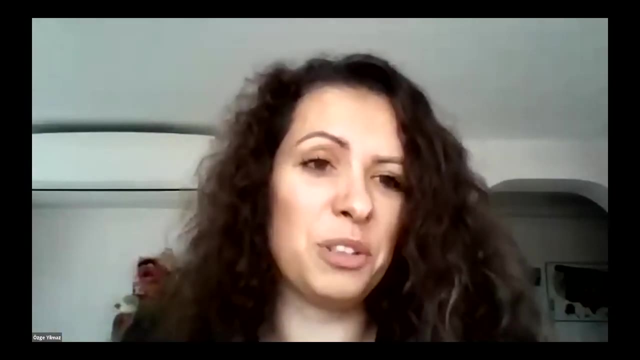 everything can be, you know, taking place as a combined study. so yes, in theory you can apply this, but you know, the plant structure and the root structure is also mainly the vegetation structure is important. so obviously there are many parameters. so this is. this is, uh, coming into a very interesting 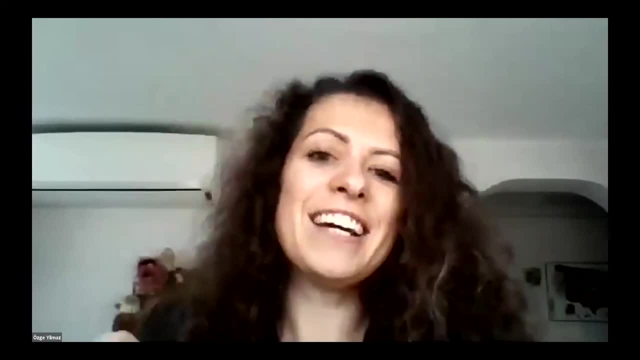 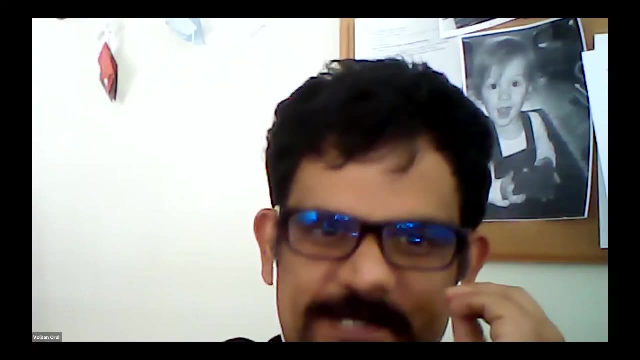 discussion. maybe we can continue this in the panel session. uh, I don't want to make Dario wait uh much longer, but thank you for your, for your presentation and, if my pleasure, if I, if I took so long time of the audience. I'm so sorry for this, but you know I have enjoyed to be no, not 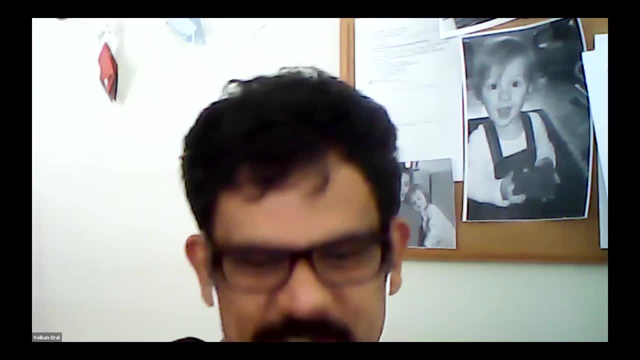 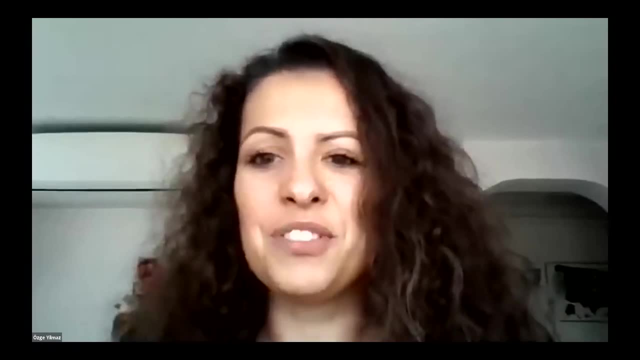 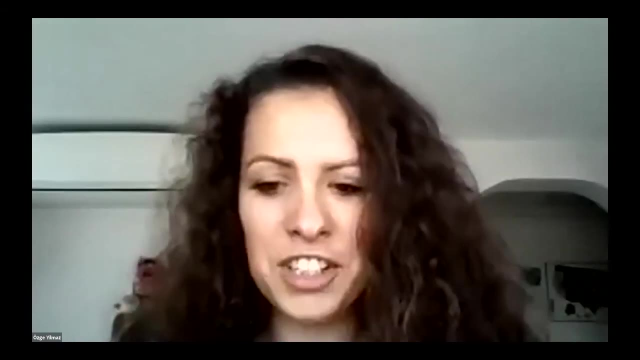 at all. it was. it was very interesting. thank you so much. thank you so much. so next we will have a joint presentation, uh with Daria Stanich and Savina Bokal, which will be delivered by Daria. Daria. she holds a bachelor of science degree in biology and a PhD in environmental protection. 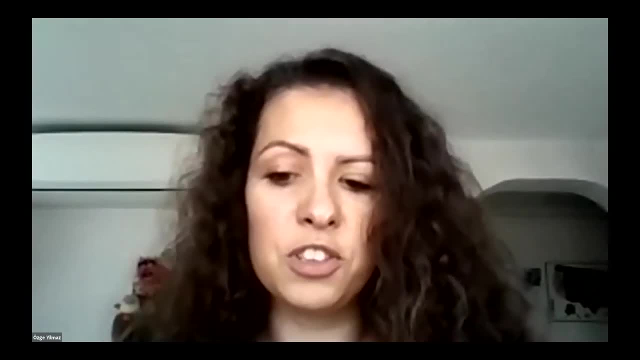 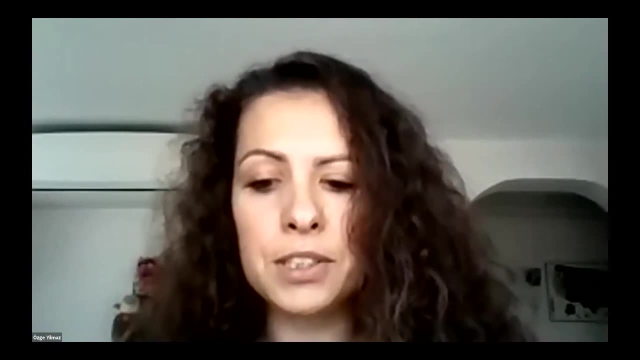 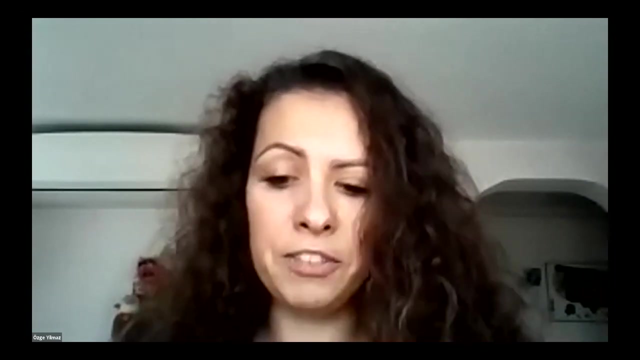 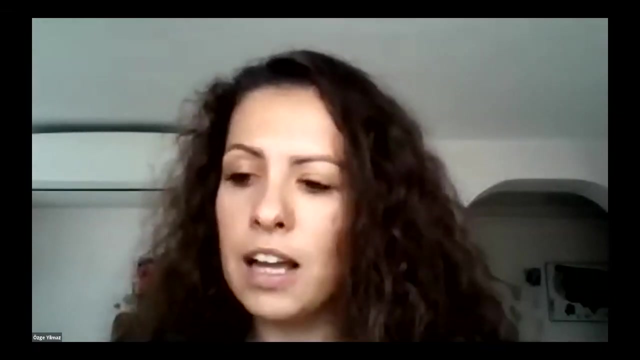 she has a wide experience in development and implementation of constructed wetlands and other MBS. currently, she is employed at University of Ljubljana, where her main research fields are nature-based solutions for wastewater treatment and reuse of treated water in agriculture. especially lately, her research includes wastewater treatment in high-rate algae ponds and MBS for food production. 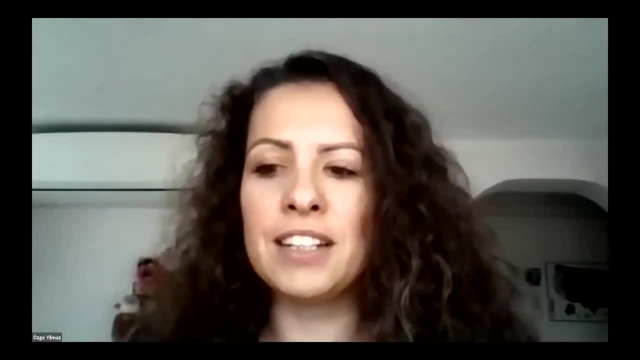 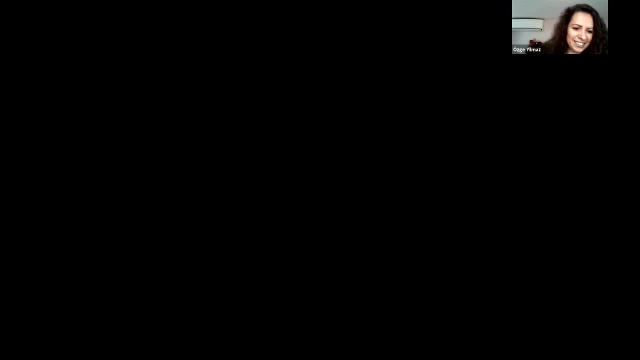 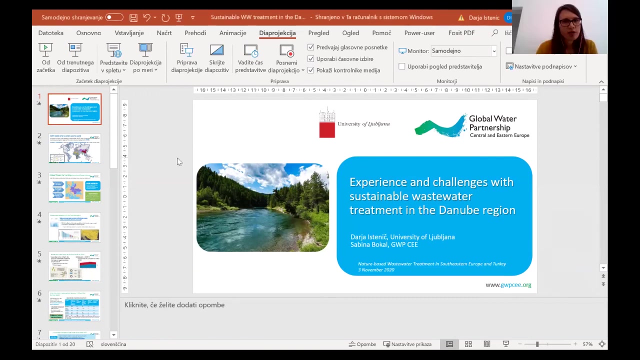 in cities. today, she will talk about experience and challenges with sustainable wastewater treatment in the new Bay region. please, the floor is yours, thank you. thank you very much for a nice introduction, um. so, as already mentioned, um, the presentation was prepared together with my colleague, Sabina Bokal. Sabina is from Global Water Partnership in Central and Eastern Europe and she's already also 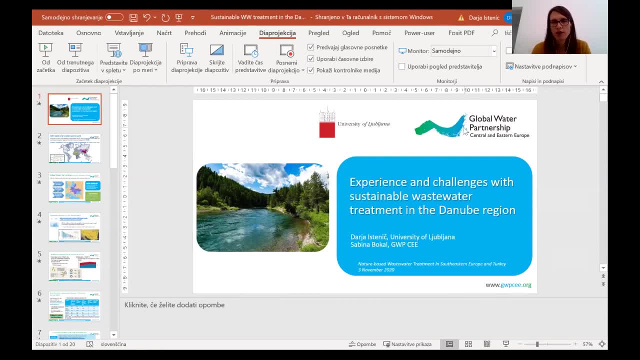 here present at this meeting, so if you will have any questions about the GWP Network, you can also refer to her. Bokal Sabina is won the title of graduate student under double montreifting record holder. so, um, do you see my screen? we can, yeah, okay, what about now? it's in presentation mode, but it's on another screen. 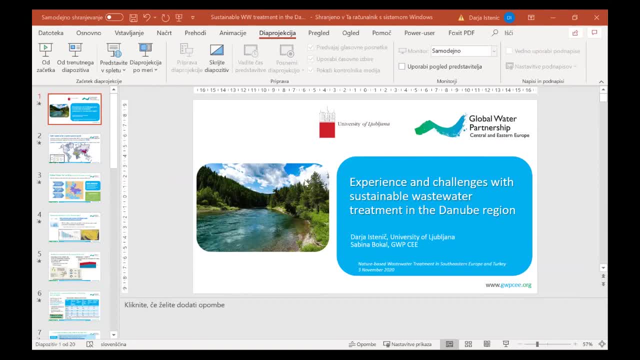 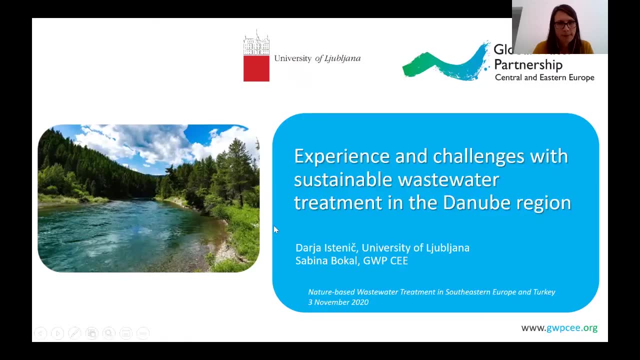 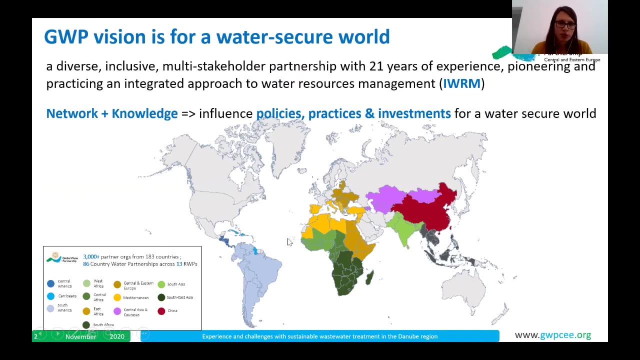 yeah, yeah, yeah, because i have two monitors, but now you should see it. yes, we can. yes, and i have another question. let me show you my screen. First, I would like to say a few words about the Global Water Partnership Network. It's a global network with a vision for a water-secure world. 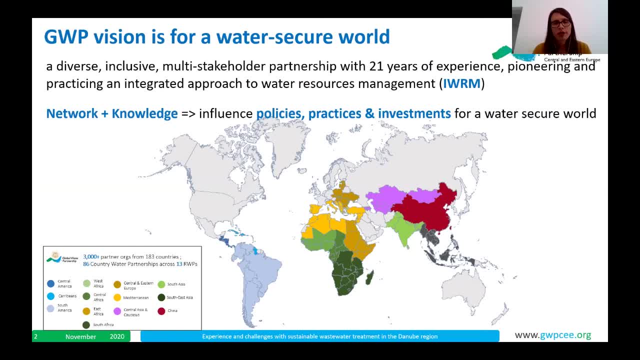 It's an inclusive multi-stakeholder partnership that exists for more than 20 years and has the goal of pioneering and practicing integrated approach to water resource management. So it joins the partners from different regions and their knowledge in order to influence policies, practices and investments for a water-secure world. 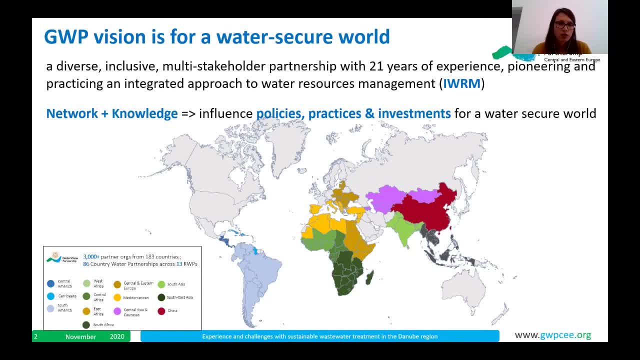 The network is organized into regional networks, as you can see in this map. So the regional networks are mainly private. They are present in developing countries. In South and Central America we have three regional networks. In Africa we have four. European countries actually belong to two networks. 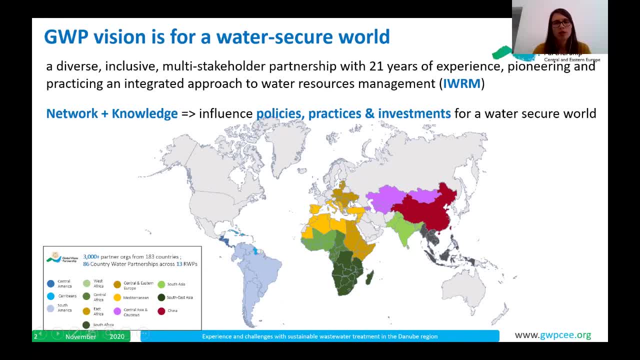 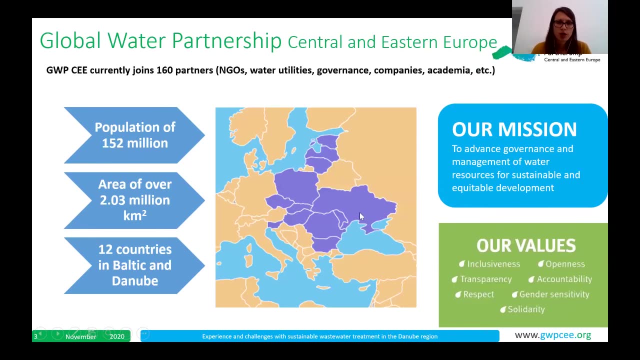 One is around the Mediterranean Sea And the second one is Central and Eastern European network, And then in Asia. there are four additional networks there. So in Central and Eastern Europe the regional network of GWP joins 12 countries from Baltic region and from the Danube region. 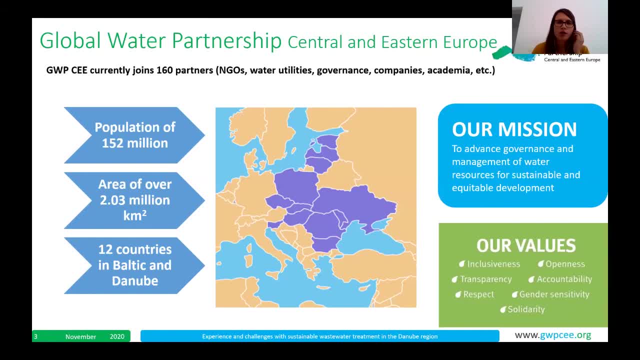 It currently has 160 partners. They come from their NGOs, water utilities, governance bodies, companies, academia and similar, And they have the common mission This is to advance governance and management of water resources for sustainable and equitable development. So some countries of the Central and Eastern Europe also belong to the Danube region. 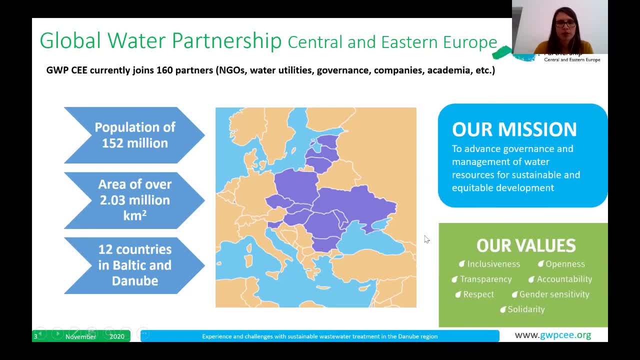 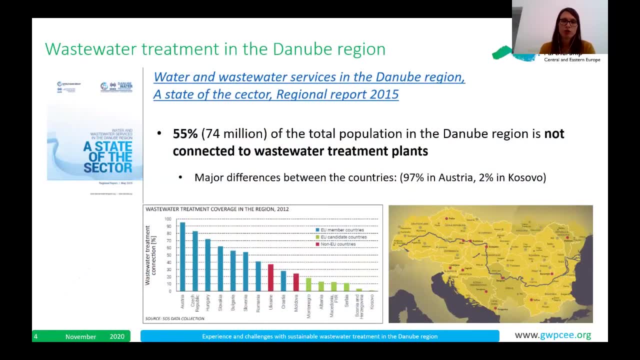 And I will focus more on these countries today. So if we want to see the situation of wastewater treatment in the Danube region, it is best to refer to the State of the Sector report. It's available online on the Danubis website. 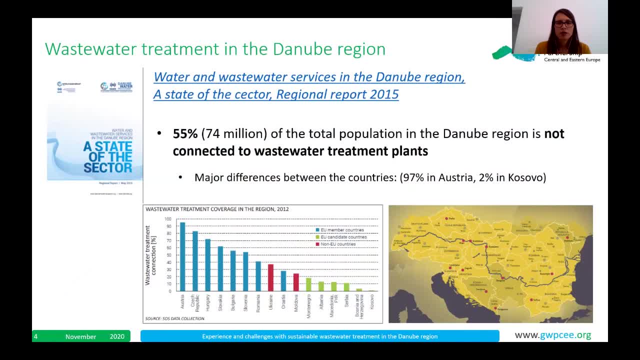 It's from 2015.. And it represents really nicely the situation of wastewater treatment in the region. Some of these data are actually quite similar, like it was presented by Kostel in the morning, But here actually the focus is on the Danube countries. 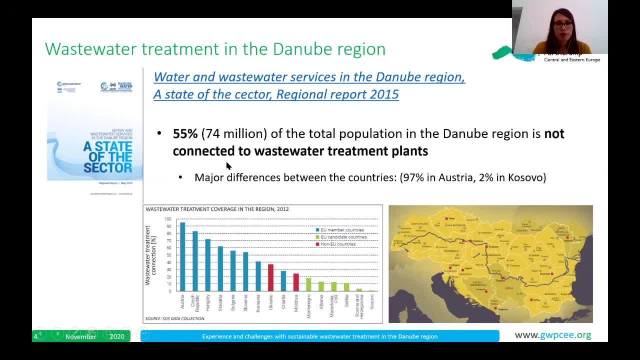 So from the report it can be seen that 55% of the total population in the Danube region is not connected to wastewater treatment plants. Of course there are major differences between the countries: 97% of connected population in Austria And on the other hand, 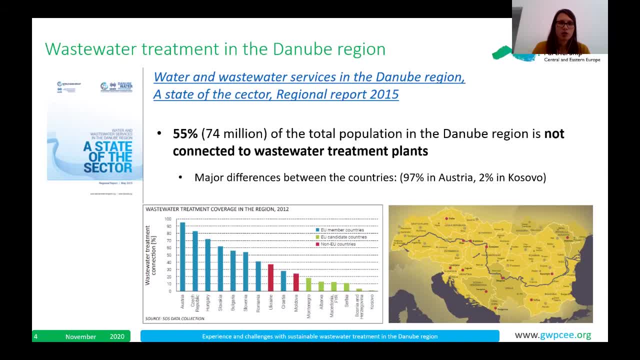 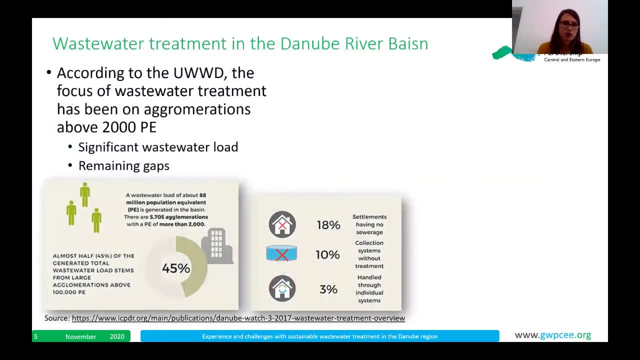 we have Kosovo, with only 2% of population that is connected to wastewater treatment plants. Of course, the report that I just mentioned and the data. they refer to the agglomerations that have more than 2000 inhabitants, because this is what 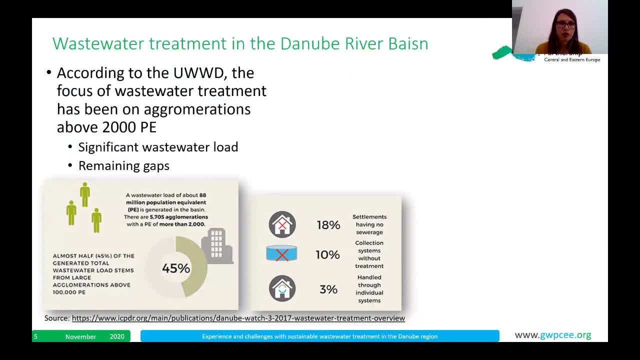 the Urban Wastewater Directive from European Union demands from the countries, Of course. these agglomerations have significant water load to the environment, And specifically the agglomerations that have more than 100,000 inhabitants. they actually present 45% of total wastewater load in the Danube region. 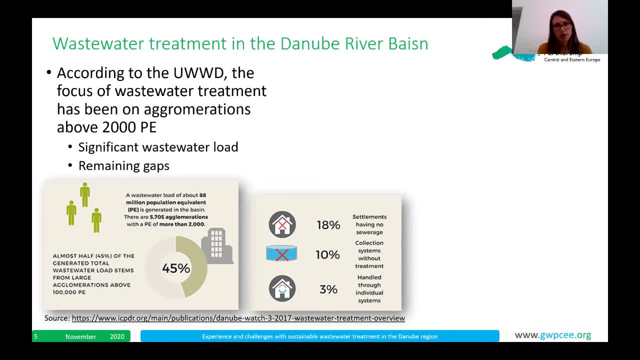 And still in this area. so with the settlements with more than 2000 inhabitants, there is a lot of work to be done, because 18% of these settlements still has no collection of wastewater And additional 10% has wastewater collection. 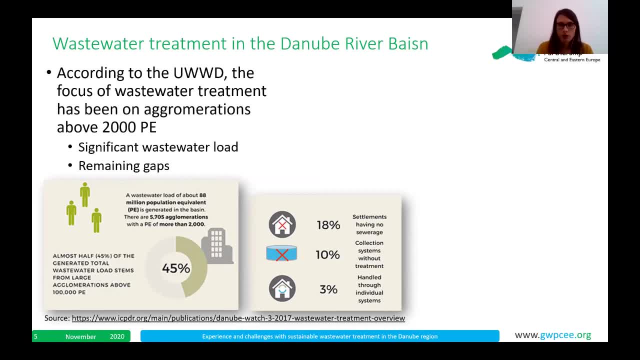 but no treatment. And then if we look into the settlements that have less than 2000 population equivalents, the situation is even worse. So these settlements actually present 45% of total wastewater. Settlements actually present 40% of the population in the Danube River basin. 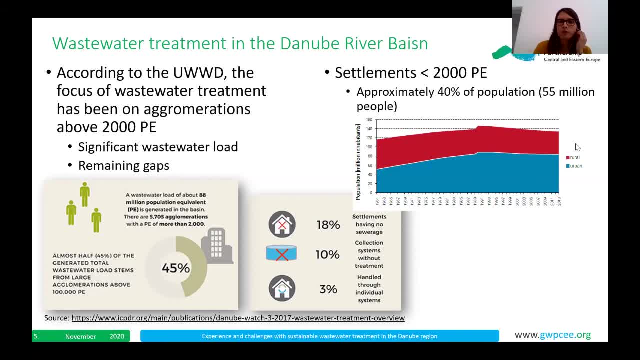 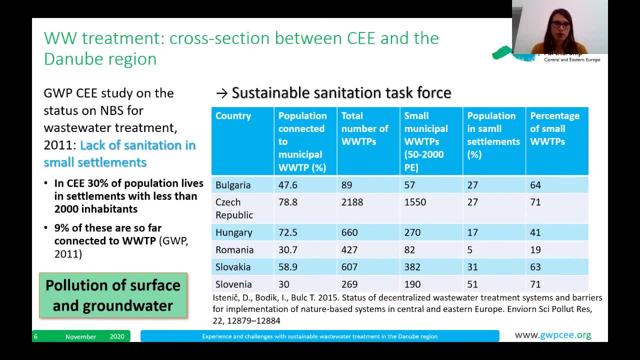 which is actually a lot, And in Global Water Partnership in Central and Eastern Europe. we actually found similar data for the Central Eastern European region In 2011,. we did a small study that actually was focused on nature-based solutions for wastewater treatment in these small settlements. 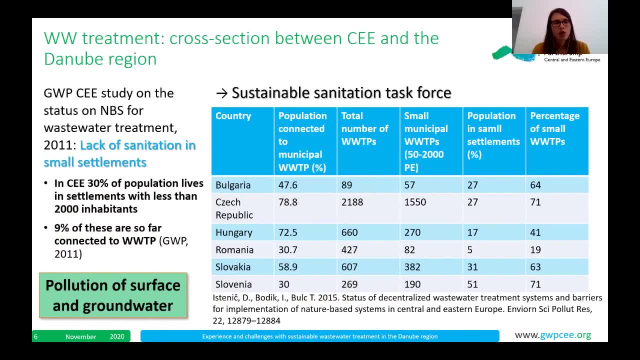 But what we found out with the study was that, of course, a lot of population lives in these small settlements. For CEE this is 30%, so a bit lower than for the Danube region, And what we found out was that only 9% of the population. 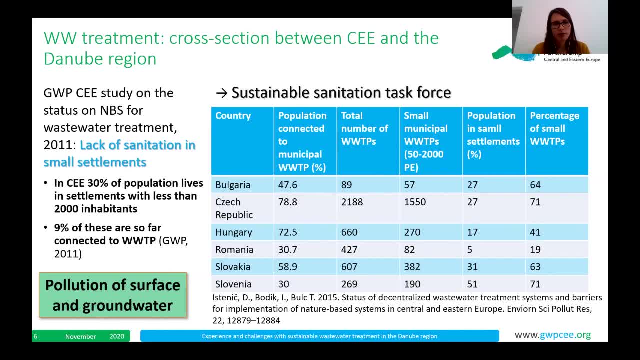 at that time was connected to wastewater treatment plants. In this table you can see a cross-section of the countries that belong both to Central and Eastern European region and to the Danube region, the number of treatment plants and the number of small treatment plants. 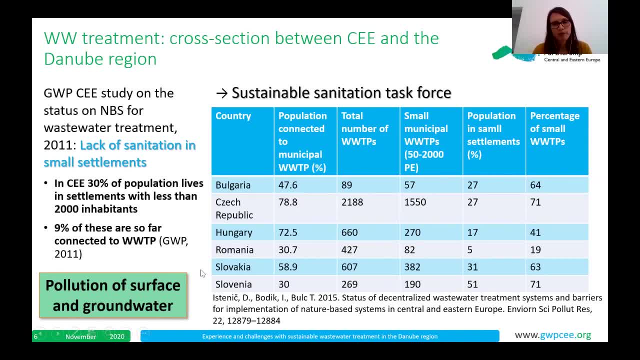 So, because the situation is actually quite bad, the GWP in the region decided to establish a Sustainable Sanitation Task Force. This is a special network inside the GWP network that joins the experts working with sustainable sanitation, And the group was quite active since 2007,. 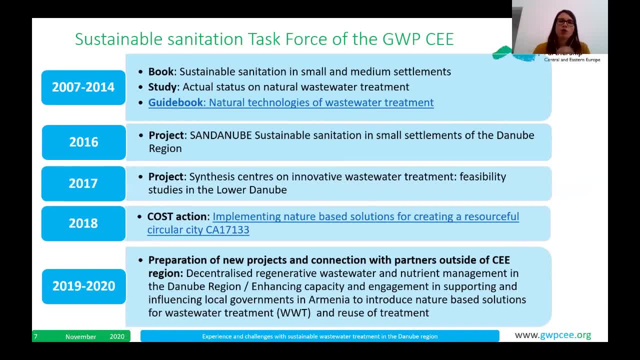 actually, And since that time, we have published a few books and literature that were mainly focused on nature-based solutions in rural areas. Among them was also a guidebook on NBS for wastewater treatment that is available online and is also used as a textbook at technical studies in the region in some countries. 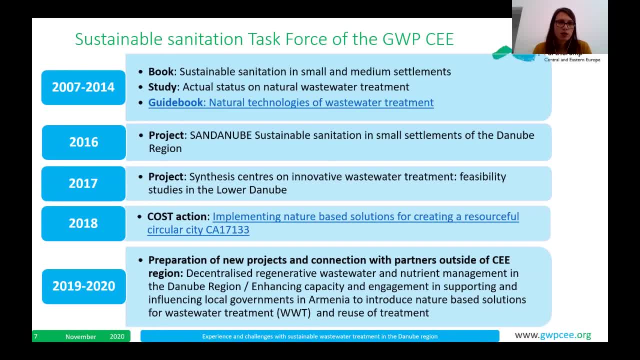 Then later on in 2016,, we were involved in a San Danube project. This was a smaller project that was focused more to the Danube region, And here the GWP CEE got a chance to also increase the network and to get more stakeholders also from the Danube region. 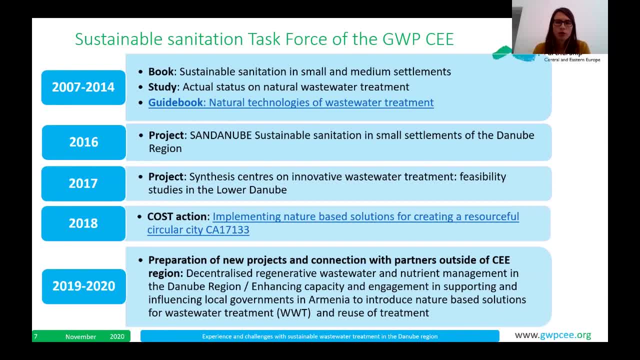 In 2017, we were involved in elaboration of a physics project And in the collaboration of a feasibility study for innovative wastewater treatment in the Danube region. this project gave some interesting results and I will present them later on. Since 2018,: 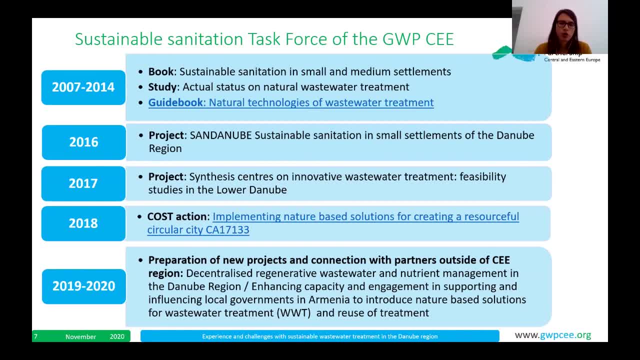 we are also involved in the cost action which was also mentioned by Volkan's presentation just now, And in the last two years our main work was actually applying different international cross-border horizon projects where we could apply these sustainable sanitation topics. 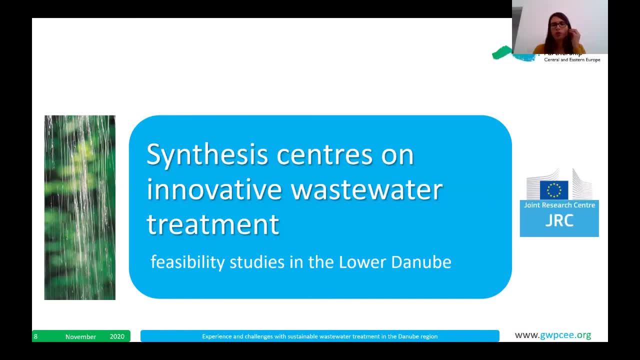 So I mentioned that GWP, as well as the University of Ljubljana or our members, were involved in the performance of feasibility study on innovative wastewater treatment system in the Danube region. The project was financed by GRC, Joint Research Center of the European Union. 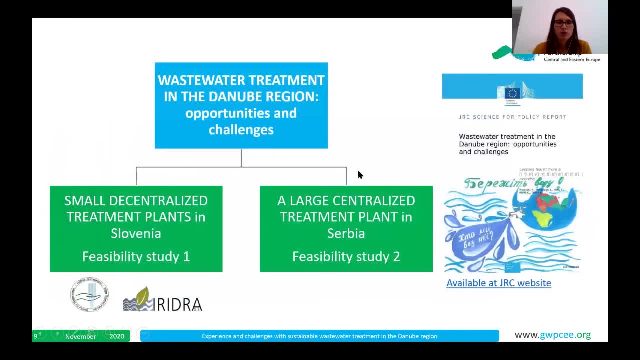 And was actually divided into two lots. The first one was focused on decentralized treatment plants and the feasibility study was done on a case study in Slovenia, And the second lot was focused on a centralized treatment plant in Serbia with resource recovery options. Both feasibility studies are presented in a common final report of the project. 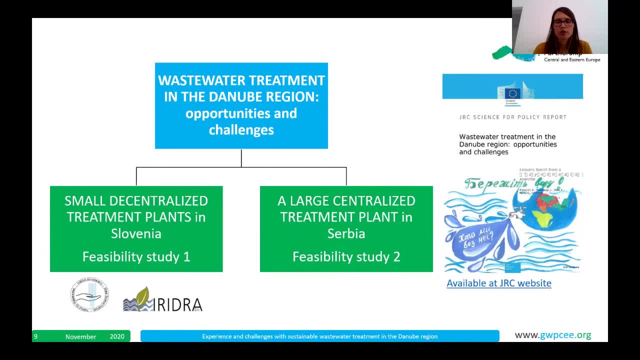 that you can find online at the GRC website. So GWP was a partner in feasibility study, one which was done together with Water Science Institute, a small SME from Slovenia that is dealing with environmental modeling and databases, And Iridra, an Italian company specialized in design and implementation of nature-based solutions. 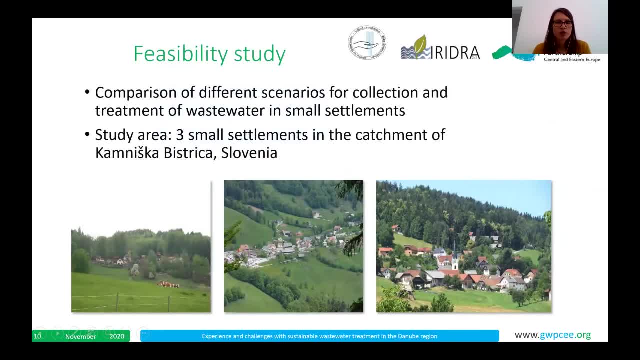 So in the feasibility study we compared different scenarios for collection and treatment of wastewater in small settlements. We selected three representative settlements in Slovenia which would be somehow representative for the whole Danube region. You can see them in these pictures and you probably see not much difference. 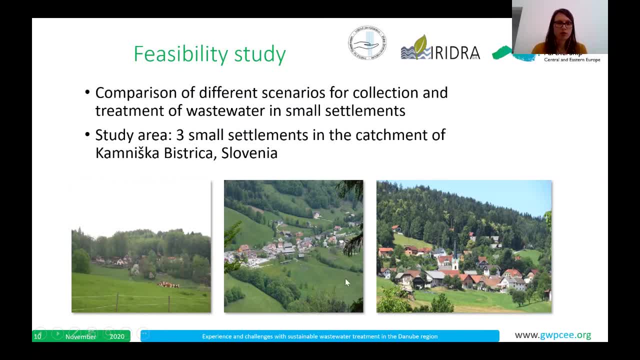 So they look very similar but in practice they are quite different. For example, this settlement in the middle is positioned in steep slopes. The soil here is clayish. There are potentials for landslides. You cannot infiltrate the treated water. 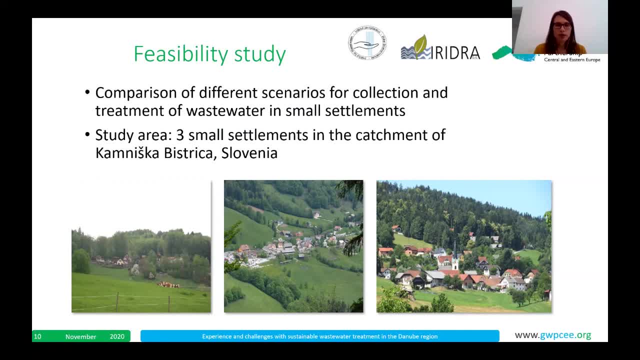 Additionally, the settlement gravitates to different sites so you cannot collect all the wastewater to one point only by gravity. You need pumping, And the village also has some tourist activities. They have a hotel and a big restaurant. So the hydraulic and pollutant fluctuations are very high. 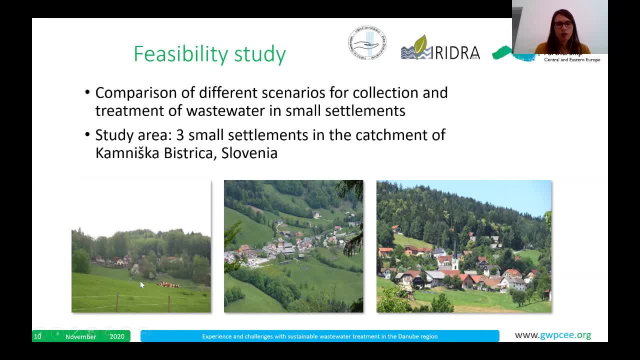 Then the second village was in Karstik area. There's limestone in the ground with lots of sinkholes, And additionally it lies in the water protection zone. The settlement is very scattered, So the houses rarely stick together, but they're very spread all over the area. 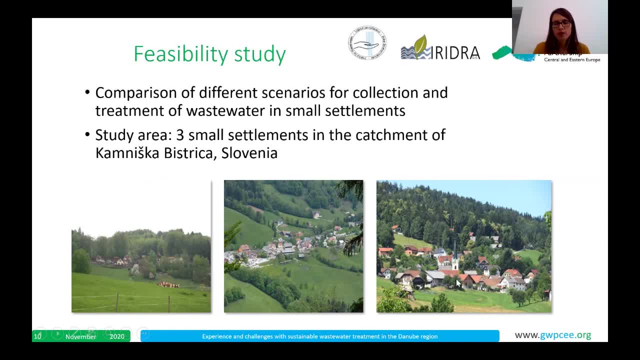 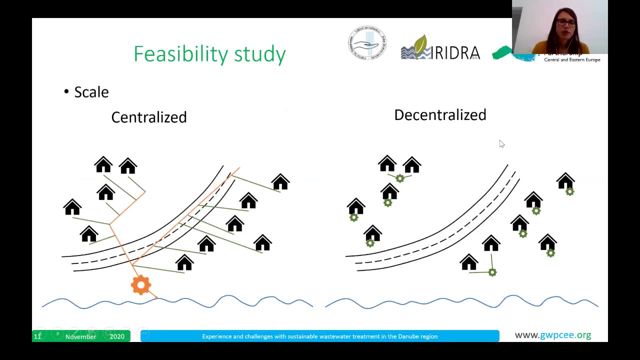 And the third example was a more dense village which actually consists of more small agglomerations, which can be then treated all together at one point or separately. So in the feasibility study we evaluated both scales that were already mentioned today, So centralized option and decentralized option. 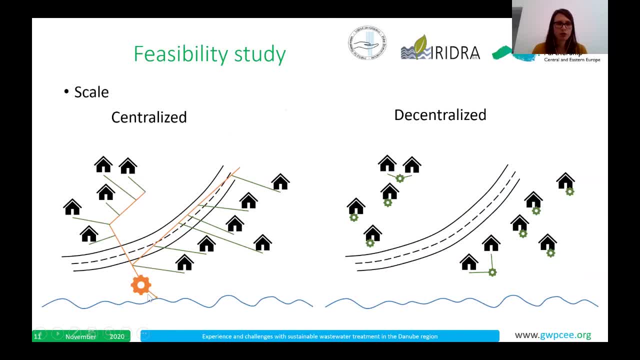 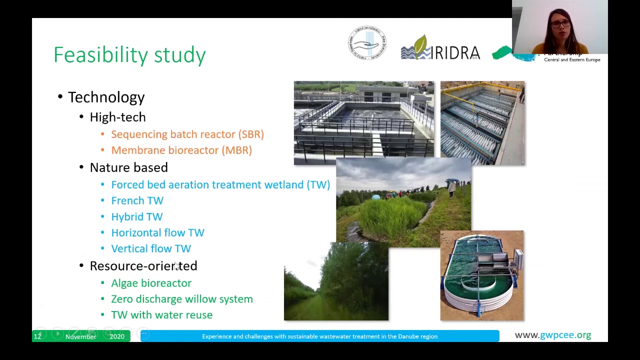 In the centralized you can have a treatment of wastewater from the whole settlement at one treatment plant, And in decentralized options you can have treatment of wastewater at individual houses or in few houses together. So the technologies that were included in feasibility study can be grouped into three major groups. 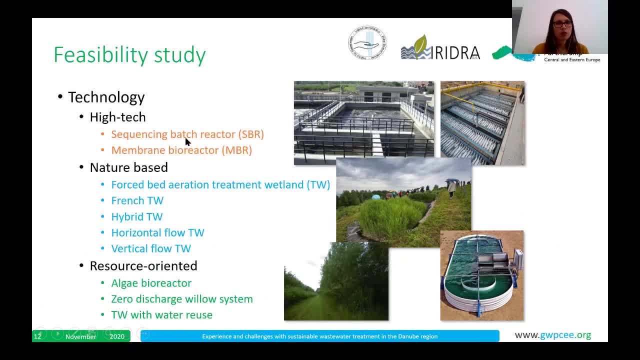 The high tech group included sequencing batch reactor and membrane bioreactor. These are actually two technologies that are quite commonly implemented in this region. In the nature-based solutions we had different options of treatment wetlands from more sophisticated forced bed aeration wetlands. 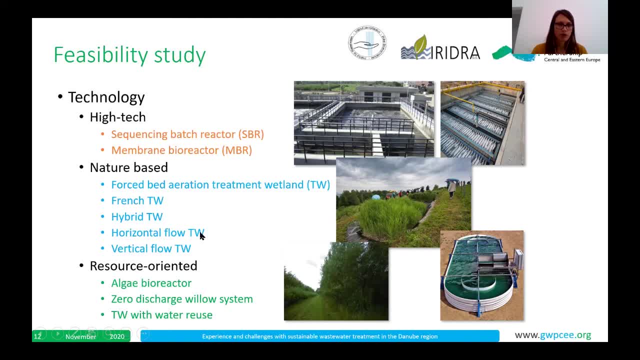 and to more classical or robust ones like horizontal flow treatment wetland. In resource-oriented group we included in the study the algae bioreactor, with which one can produce algae biomass that can be used as a fertilizer in agriculture, Then a zero discharge willow system to produce willow wood chip as an energy source for household heating. 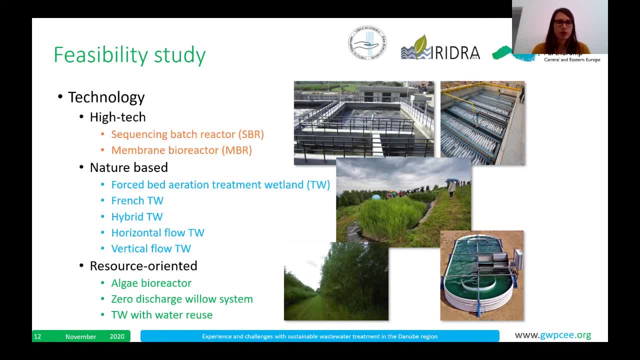 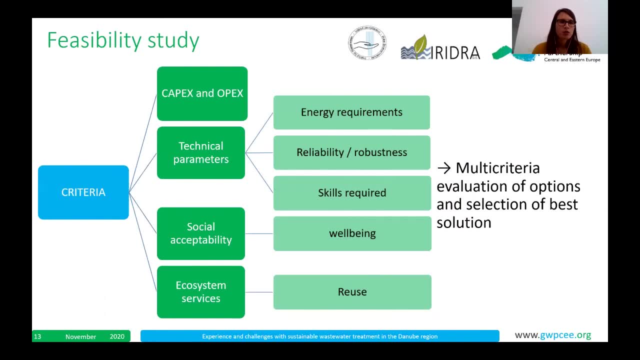 And we also included treatment wetlands with water reuse as resource recovery. So we set a plan. We set a bunch of criteria in the feasibility study. The criteria included capital and operation costs, expenditure. Then technical parameters. that included energy requirements, the reliability of the technology. 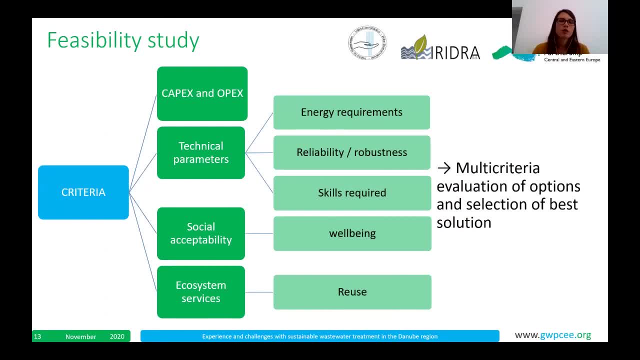 its robustness and also the skills that are required from the maintenance staff. The social acceptability included well-being, which is actually from providing jobs to the satisfaction of the local community with the system, And the criteria were also different. ecosystem services, including waste water reuse. 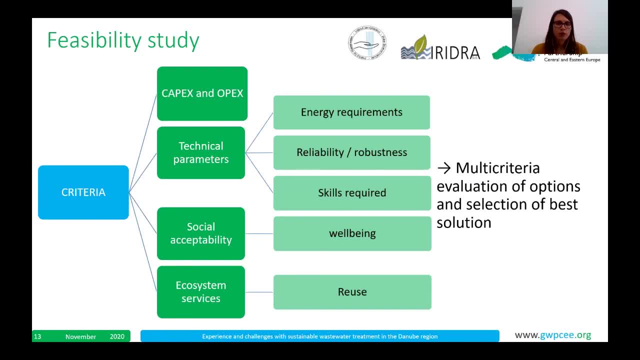 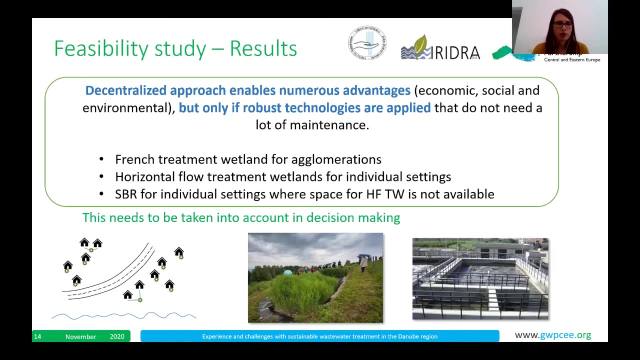 So, after setting all these criteria, a multi-criteria evaluation of different options was carried out, And then we selected the best solution. I wouldn't go into the process of this selection, but I would like to point out the result. So the results showed that decentralized approach can enable numerous advantages. 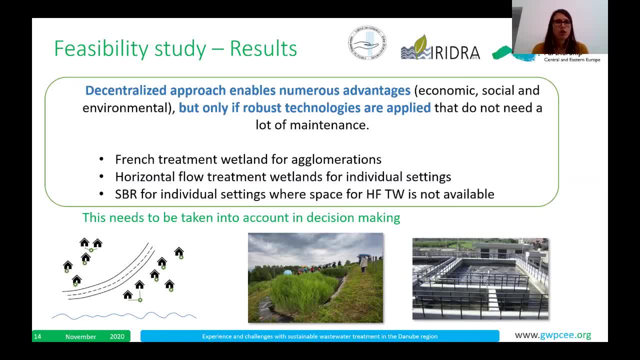 economic, social, environmental, but only if robust technologies are applied, So technologies that are reliable, that can withstand hydraulic and pollutant load and that do not demand a lot of maintenance. So in this case, this would mean that we would suggest French treatment wetland. 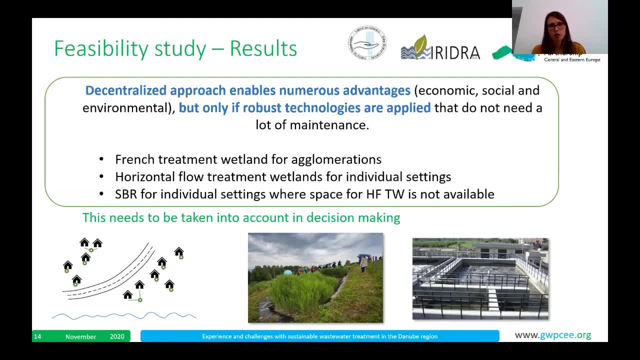 in case of treating wastewater from the whole agglomeration- because with French treatment wetlands, as you may know, you can treat raw wastewater and you don't need pretreatment- Then for individual houses a horizontal flow treatment wetland would be most visible option. 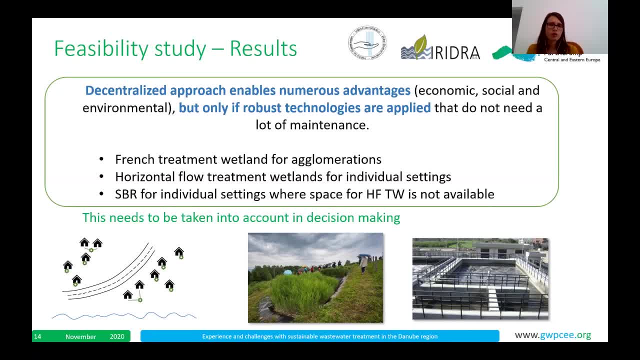 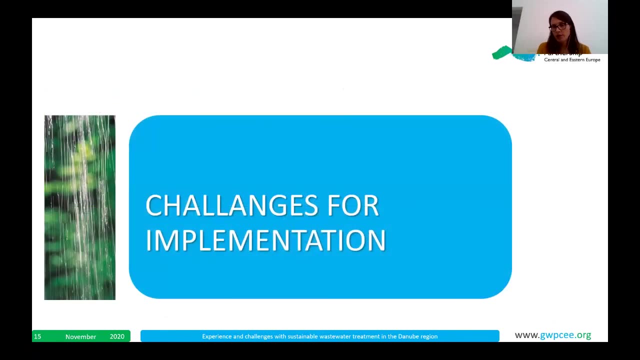 And in cases where there is not enough space available, then SBR would be most visible. So we know which approach to take and we know which technologies to promote, And now the next are the challenges that we face for further implementation of these solutions. 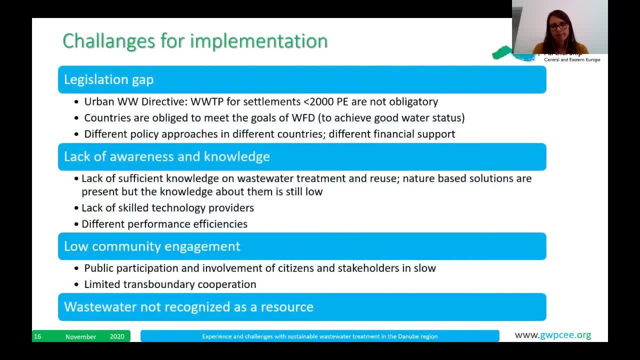 I would list just some most important challenges, or the ones that we recognize as the most abundant, as the most present. So one is of course the legislation gap. As was already mentioned today, the Urban Wastewater Directive does not refer to the settlements below 2000 PE. 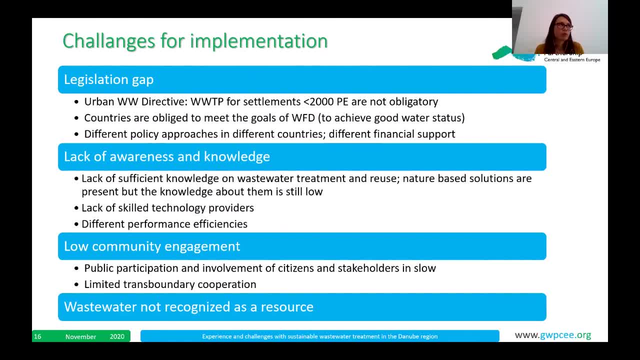 And the countries are then have to solve the problem by themselves. But on the other hand, luckily there is the Water Framework Directive and they have to meet a good water status of their surface and groundwater. So this is somehow an indirect obligation to also treat the waste waters. 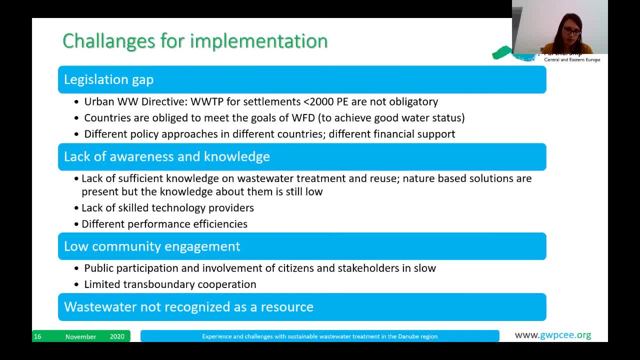 One thing that GWP finds as a challenge and is very important is still lack of awareness and knowledge. It's hard to admit that this is still a challenge in 2020.. But there is actually really lack of skilled technology providers. There is slow transition of knowledge or transfer of knowledge from academia to practitioners. 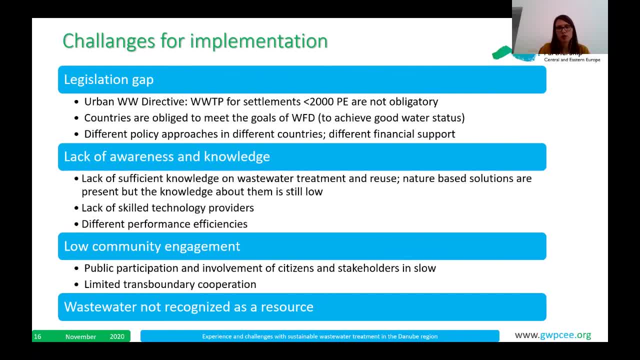 Luckily, in the last years, nature based solutions gained some importance and are more known, But it's still. there are many difficulties with their application And, on top of this, there are some solutions that were implemented, maybe with some lack of knowledge, and they are not functioning properly. 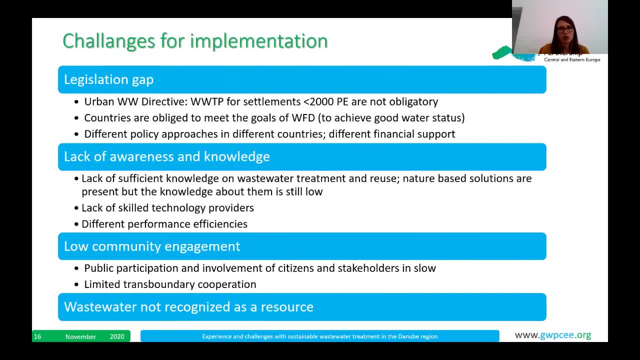 And this gives a bad light on the whole set of solutions. The community engagement is low. Actually, it's much bigger than in case of centralized approach, But still it should be much more emphasized. Different types of stakeholders should be involved in the decision making processes. 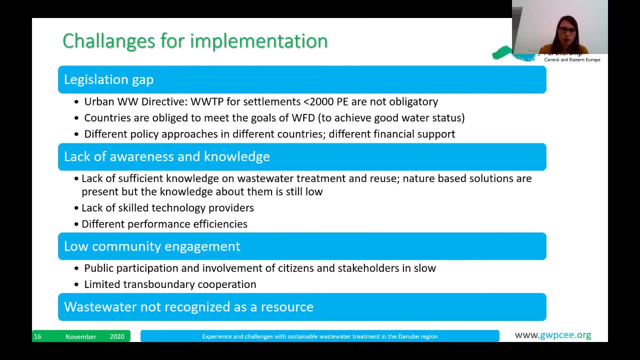 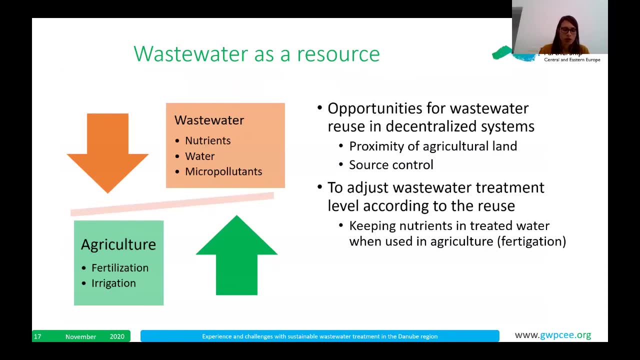 And this is also one of the goals of GWP network. And last but not least, one of the challenges is also that wastewater is not recognized as a resource, But in our opinion it should be especially in decentralized settings, because the opportunities for wastewater reuse in decentralized systems are actually big. 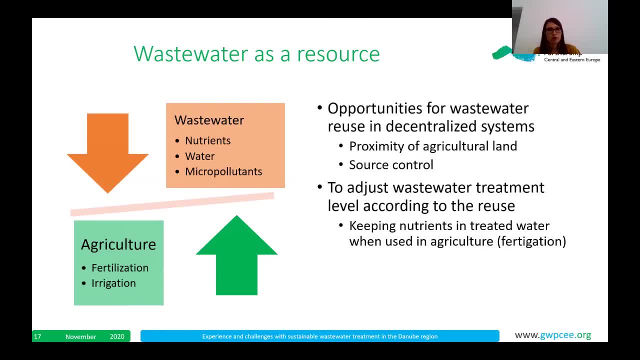 These small villages, small settlements. they are in proximity of agricultural land, So the reuse of water for irrigation can be easily implemented And if you have decentralized systems, you also have a better source control and less micropollutants in the wastewater. 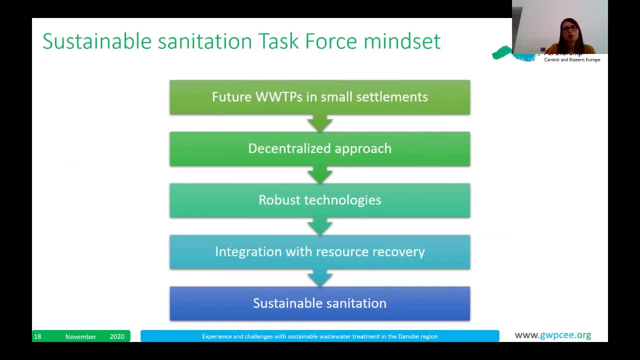 So the Sustainable Sanitation Task Force of Global Water Partnership Network has somehow defined mindset. We know that in the future we will need a lot of small treatment plants to treat wastewater from small settlements. It will be needed in the central and eastern Europe, as well as in the new region and elsewhere in the world. 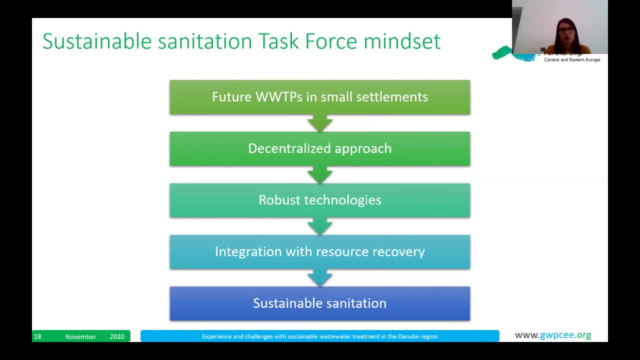 We know that decentralized approach is the one that can bring more benefits and that robust technologies have to be applied. We also know that these technologies have to be integrated with resources. So I would like to address the question: what are the best and most critical elements to? 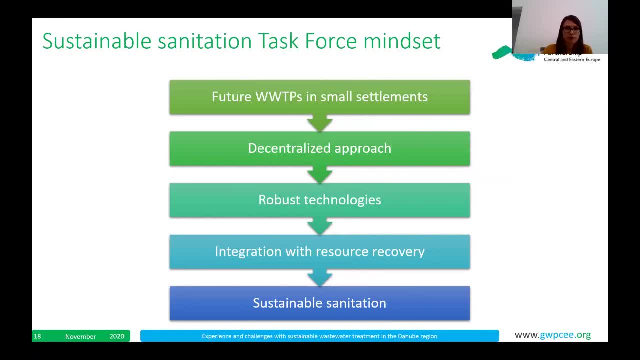 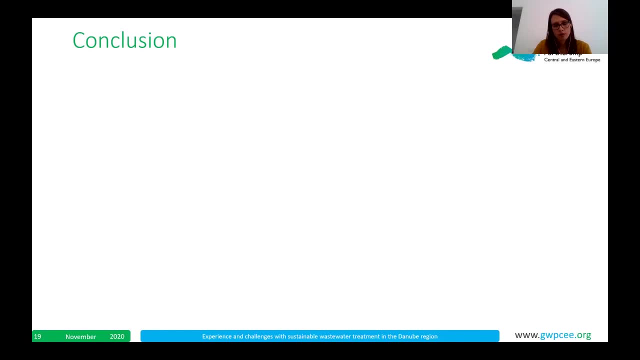 the city's recovery, because this is actually the only way how to reach sustainable sanitation. So for the end, I would somehow point out the basic findings and our way to go. So Global Water Partnership in central and eastern Europe wants to promote nature based solutions as robust technologies that can offer integrated water management. 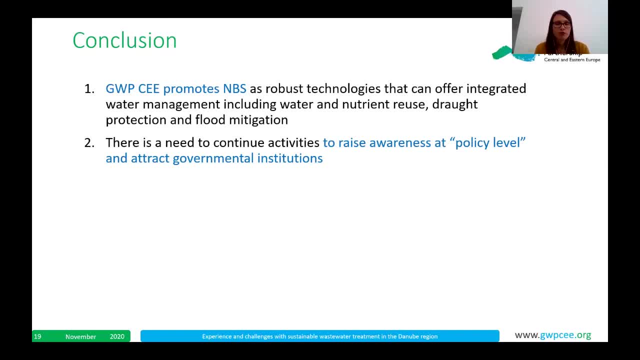 And there is still a need to rise awareness with different stakeholders, also at policy level, and to attract governmental institutions in such projects. So from our work it's actually we can say that it's difficult to attract governmental institutions into projects because they somehow don't see so big interest in this sustainable sanitation in rural areas. And, as I already mentioned before, there is a need to bridge the gap between 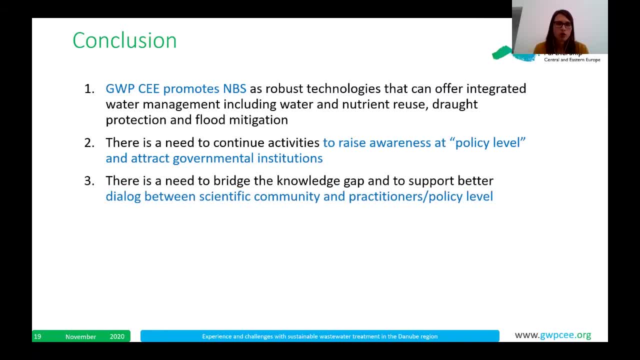 the scientific community and practitioners, because a lot of knowledge already exists, which, but we can also see from today's presentations that the knowledge is there. we just need to transfer it faster and better to the practitioners and to the policy level. Additionally, there are many good practices also in the Danube region and CEE and they offer a very good opportunity to do this. so to transfer the knowledge and to disseminate the ideas. 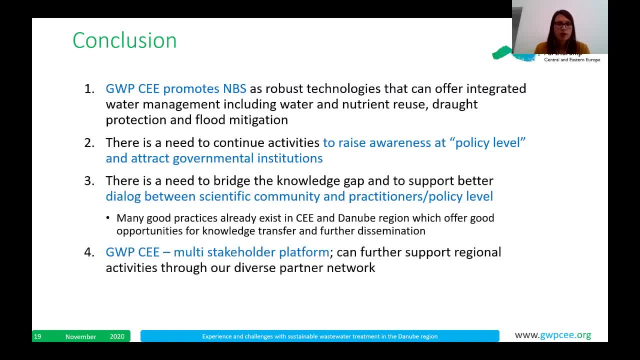 And last but not least, GWPC is a multi-stakeholder platform and has actually all the capacities to further spread the information and to join the partners in common goals. So if anyone is interested, you are also very welcome to join freely to the network of GWP. 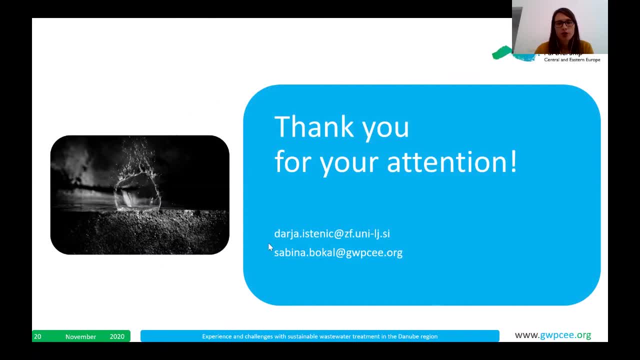 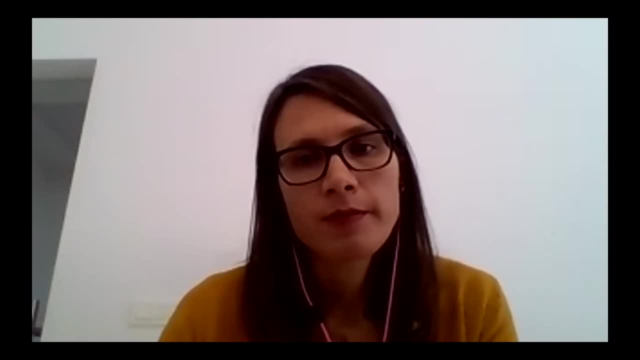 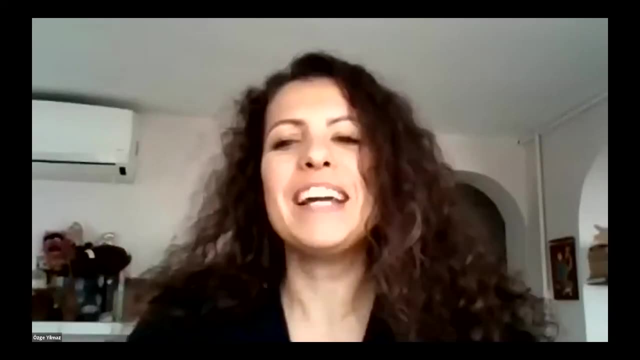 Thank you very much for your attention. If any questions, welcome. Thank you, Daria. Let's start with David. We should also thank Sabina, Sabina hello, So you both prepared the presentation, So you're all also here. Thank you so much. 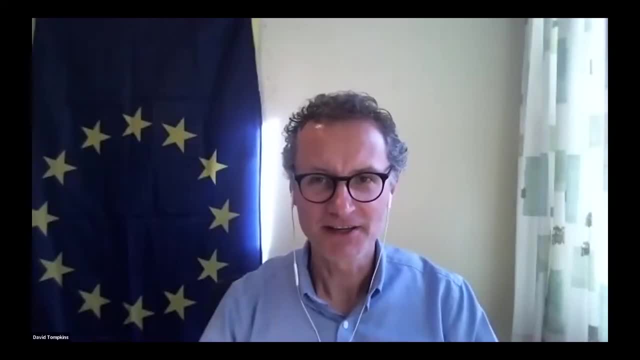 Thank you. Great presentation, Thank you, And just a question on standards and developments with the Water Framework Directive in Europe. I'm not so familiar with the ongoing work on it, but is any of you familiar with the project, familiar with the ongoing developments, but do you think there's any prospect of universal 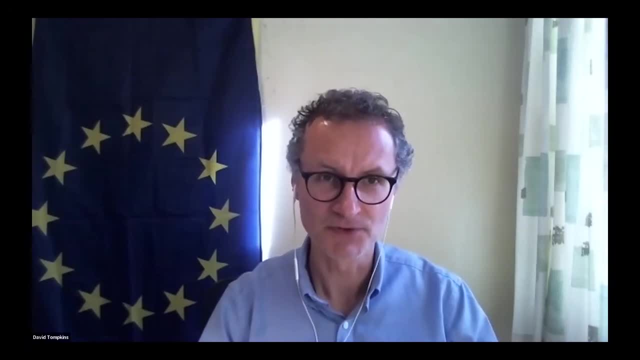 treatment standards for small works or for individual discharges in the future, because from from your presentation, one message i'm getting is that a huge variety of approaches to implementing treatment at the small scale. so i wonder, if you have you, you could kind of perhaps provide your, your thoughts on whether we might see some, some guidance from europe, or whether 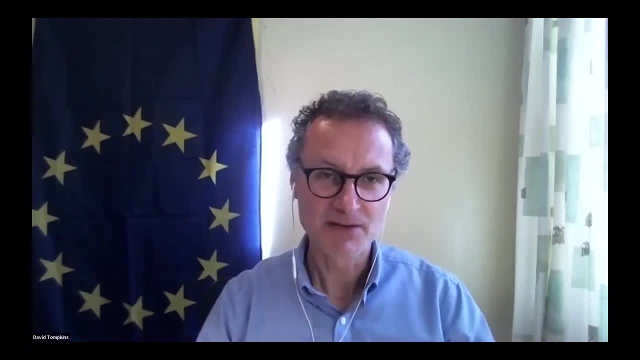 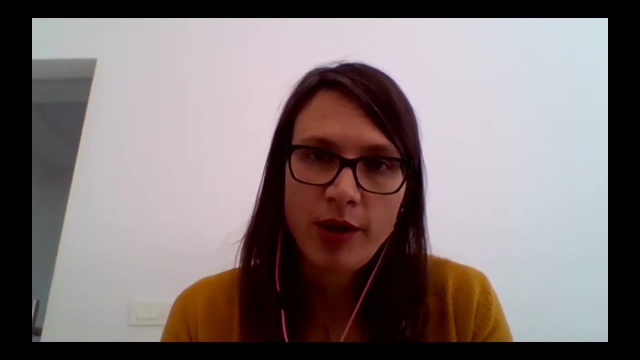 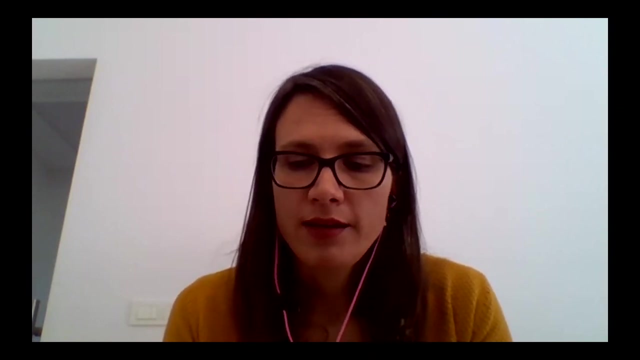 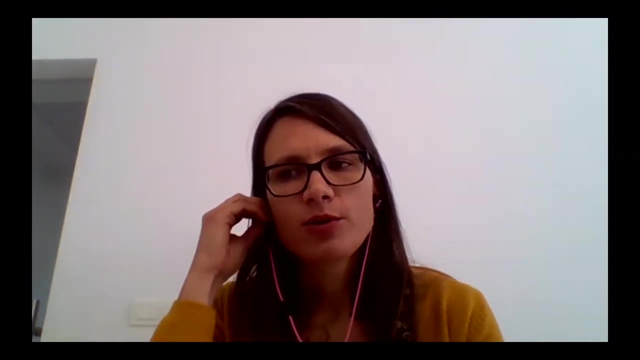 there are other initiatives that can implement similar treatment standards across the countries. yeah, thank you. actually there was a lot of discussion about this in different networks, so how to set common guidelines for these small settlements, and actually no real conclusions because the situation is so diverse. so also nowadays the countries have very different. 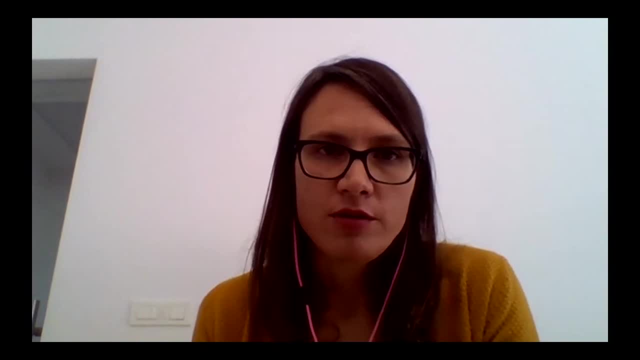 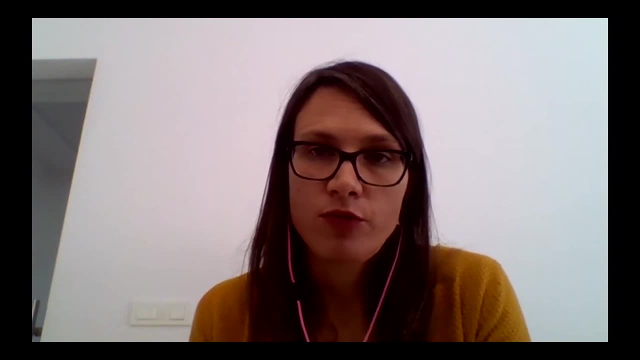 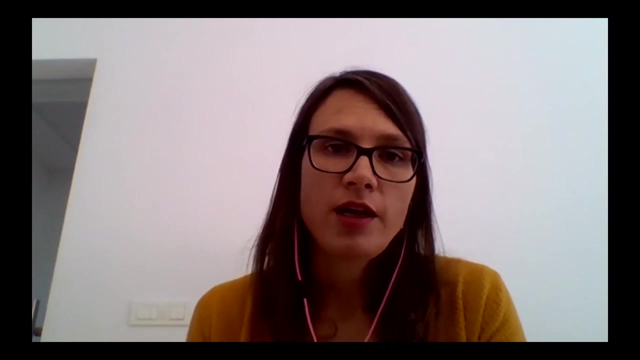 approaches to these small settlements. some countries, for example the balkan countries, have very strict demands for wastewater discharge, also for single households, i mean the. the standards can be almost like drinking water, because they are actually copying the same treatment levels as are needed for big systems. so this is one extreme, while the other extreme is having no. 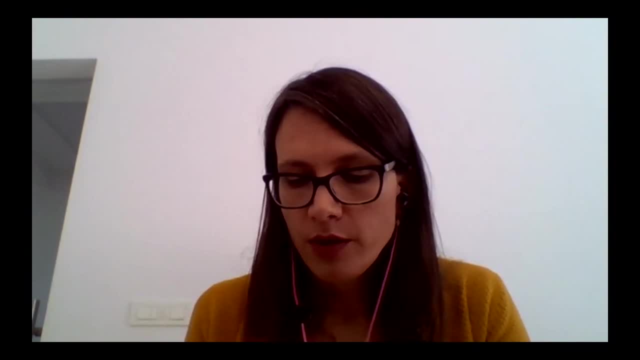 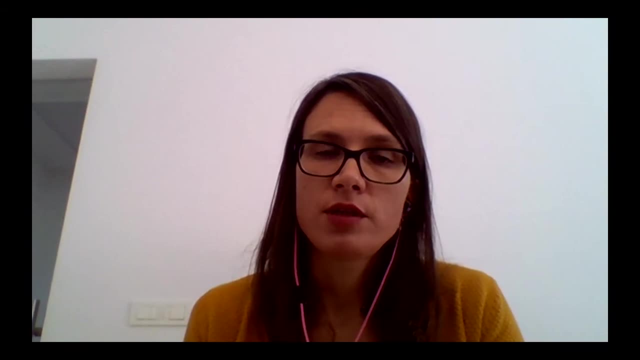 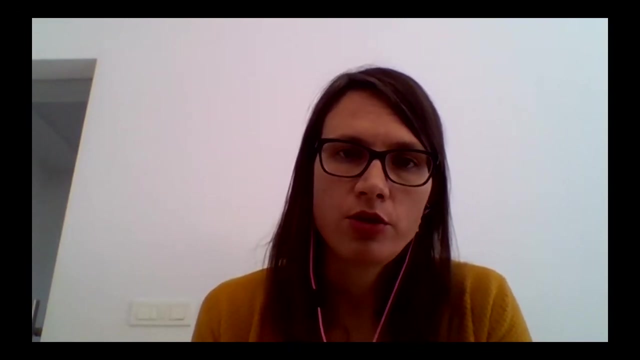 regulation at all, but in my opinion, this has to be adjusted to every country or region, because there are also different sensitivities of the environment. for example, in countries where natural water courses have high self-purification capacity, you don't need to remove so much pollutants as in the countries 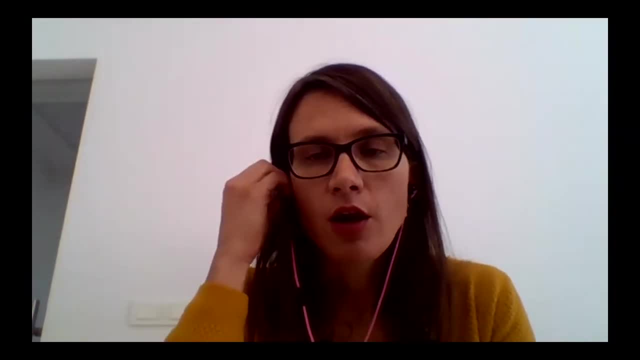 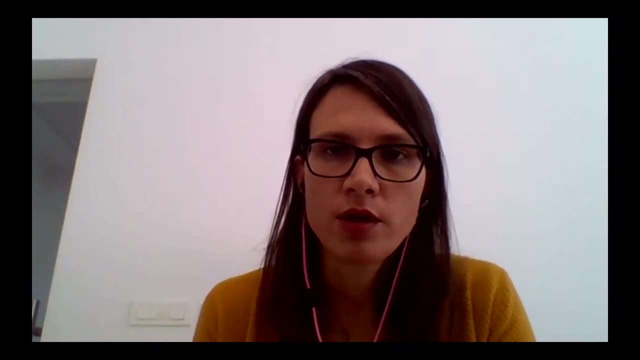 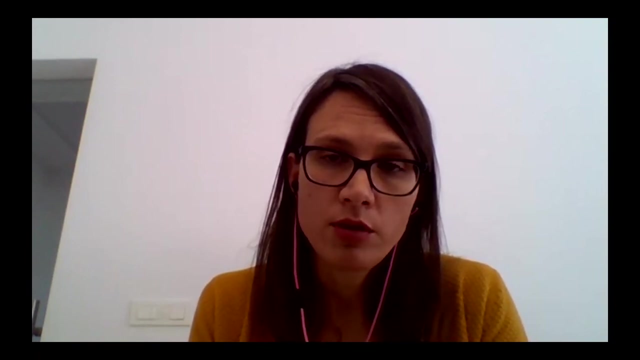 where they have more sensitive areas and like lowlands and more sensitive water courses, and it's important to remove, for example, all the nutrients and, on the other hand, the treatment performance should also be linked to the wastewater reuse. so if we are going to reuse the wastewater in 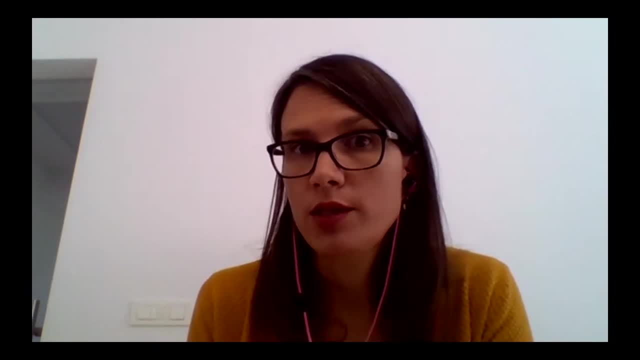 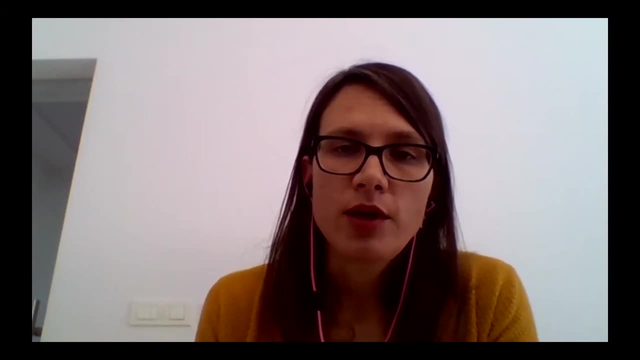 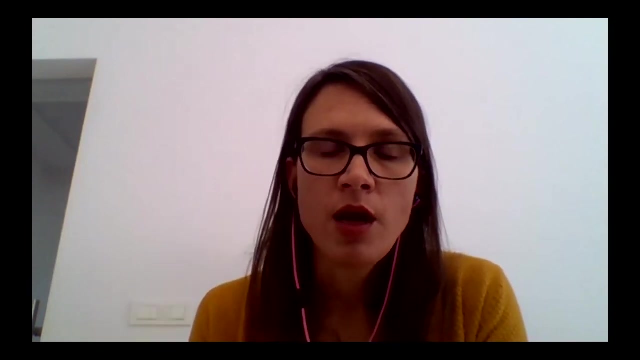 agriculture, then we don't need to remove the nutrients during summer, but during winter it's of course the plants do not need the nutrients and you have to do something with them. so i can see the solution in somehow flexible technologies that can adjust also their treatment performance during the year and to really reuse the 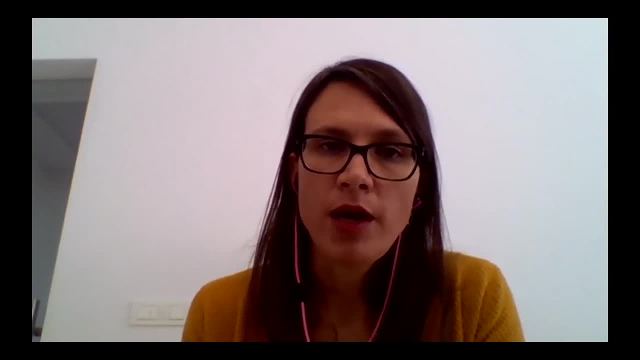 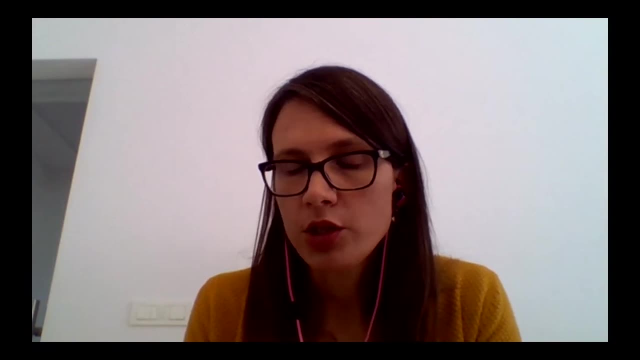 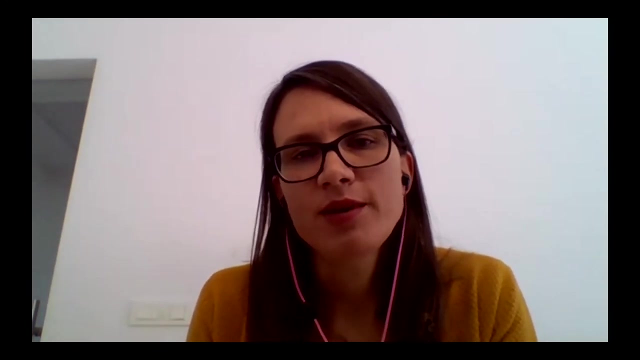 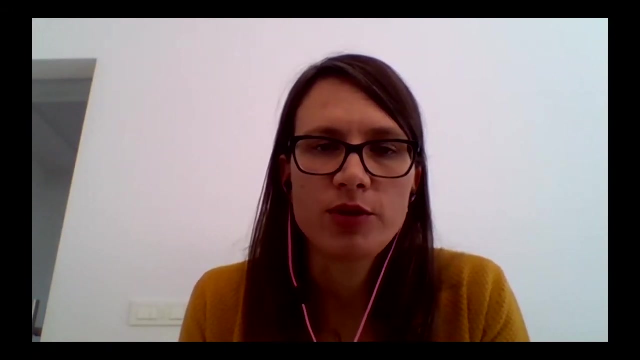 water wherever possible for agriculture or for other purposes, but to find like to set some common legislation limits for the whole europe. maybe it's not really the best solution, maybe some raw guidelines, but to set some specific numbers. it's not necessary that we will solve the problem with this. okay, thank you. thank you. 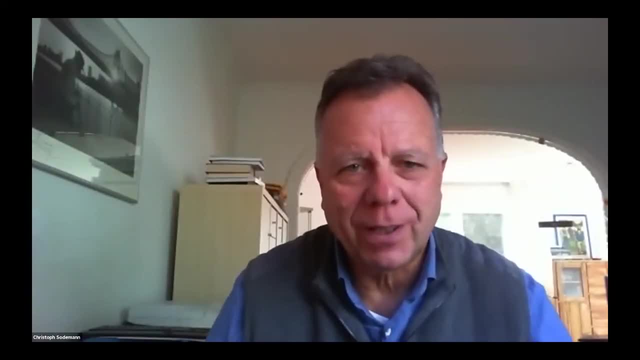 crystal, please? yeah, thanks for this really interesting presentation. i have one question, which you, let's say, partly mentioned already this topic. when you are dealing with the municipalities or the local authorities, what is your experience do they? are they open for decentralized solutions or are there rather having reservations? i think the situation is getting better because, um, also now with our 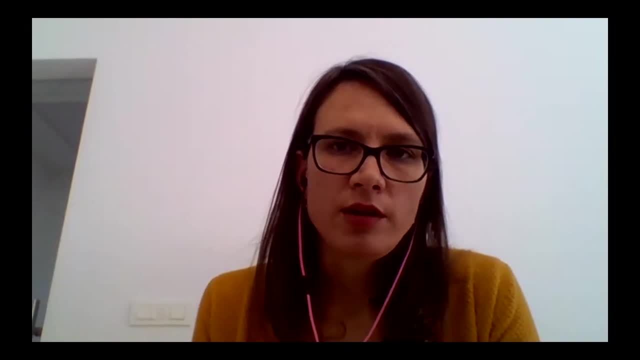 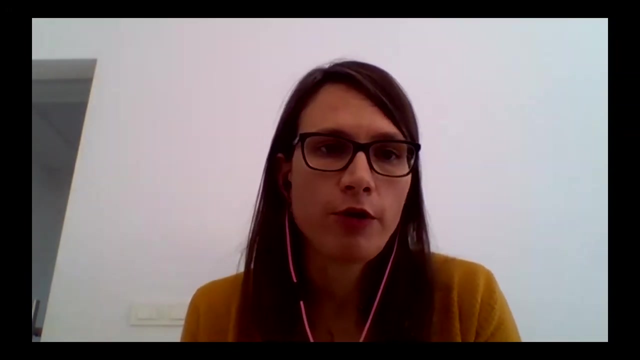 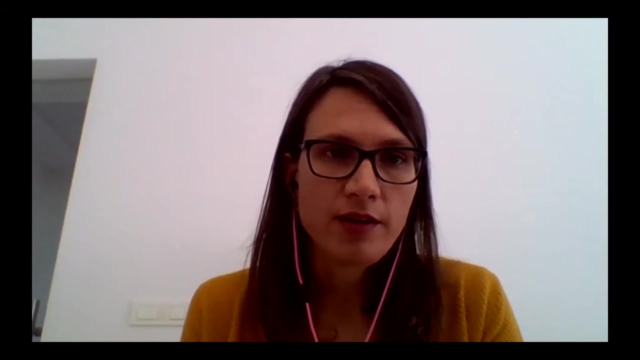 projects and networking, we can somehow attract the governmental bodies and municipalities to participate in the events. also, when we were doing this feasibility study we invited municipalities, ministry for environment and other governmental institutions. so with more effort to inviting them we can really get them on board. but it's not so easy with 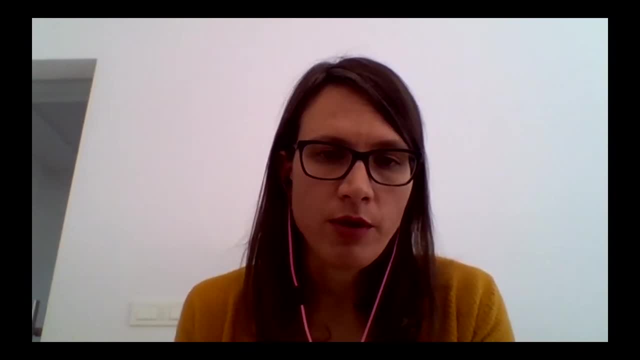 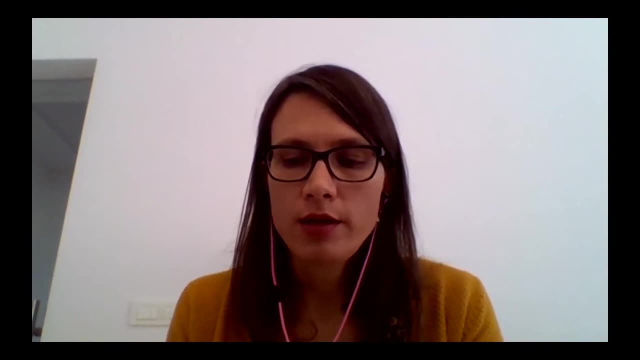 like with some other partners that are really more cooperative. so this is getting better and they are also more keen to decentralized systems as, for example, 10 or 20 years ago, because now there are more examples of good solutions existing and they like to go there and 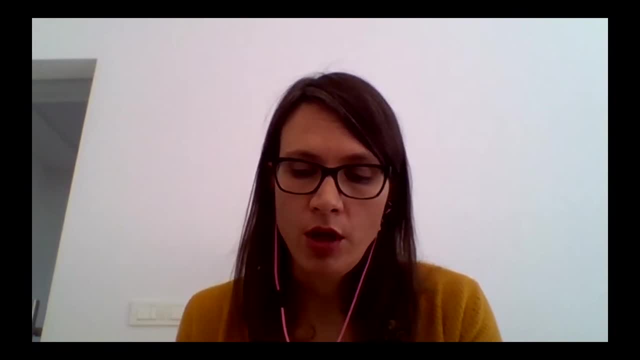 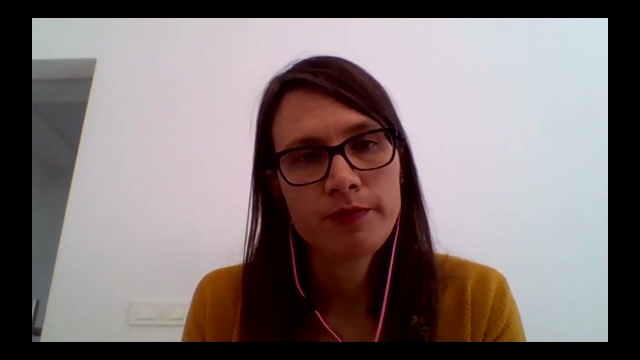 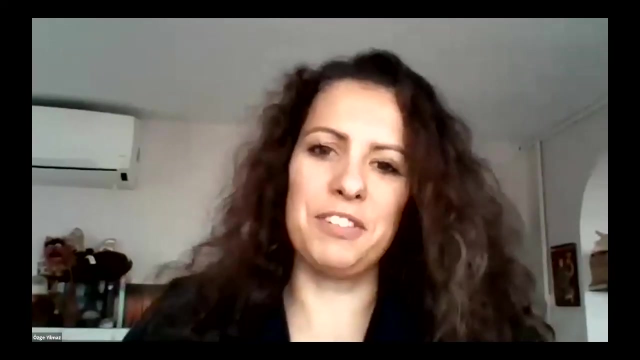 see the real example working in function. so somehow this type of awareness rising and knowledge spreading is, i think, quite important. so to show the the examples of best practice. uh daria sabina, thank you very much for your presentation. so i think i also have some questions. 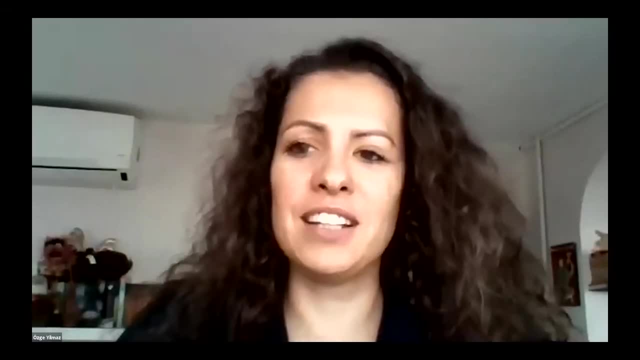 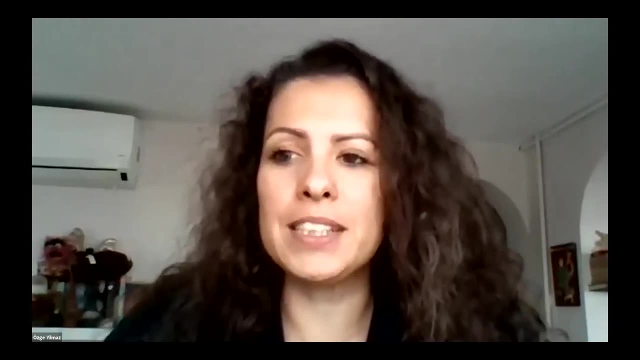 but we can leave it to the panelists, if it's all right, so that we can move on with our program. uh, so it's time to move on to the presentation from olga tyron, who is another researcher from echo in romania, one of our 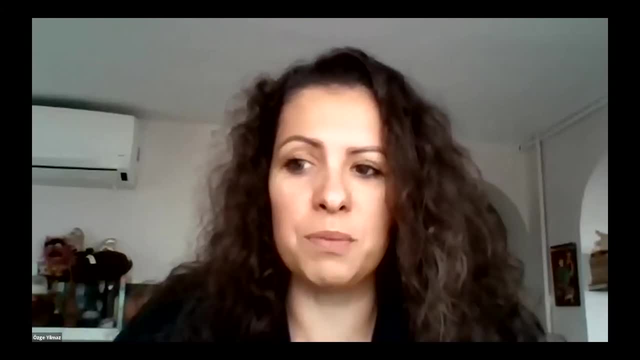 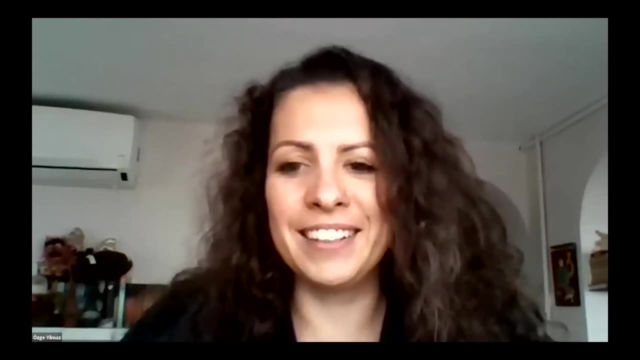 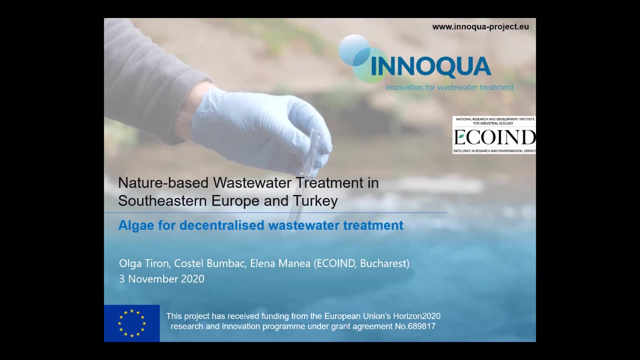 research. research topic is the wastewater treatment with microalgae systems. today, she will share her expertise on algae for decentralized wastewater treatment. uh, olga, the floor is yours. thank you, uh, good afternoon. uh, thank you for an introduction. uh, i am olga tyron. yes, from echo in the institute, working with um costello in the department of 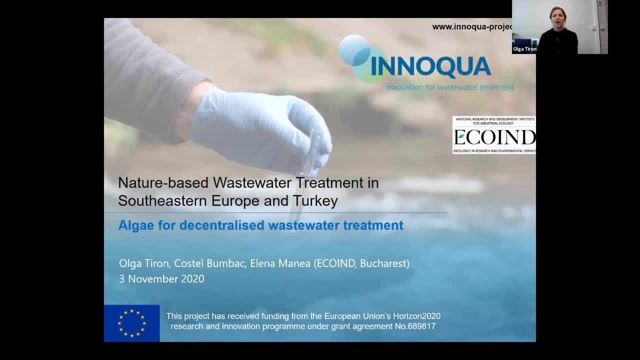 environmental technologies and technological transfer. the next presentation emphasizes the impact of the microalgae integration in wastewater treatment technology, represented as an alternative solution for sanitation, rising problems and overall for a wastewater treatment sector. topics covered will be why microalgae population uh technology principle achieved performance and recognized constraints identified during. 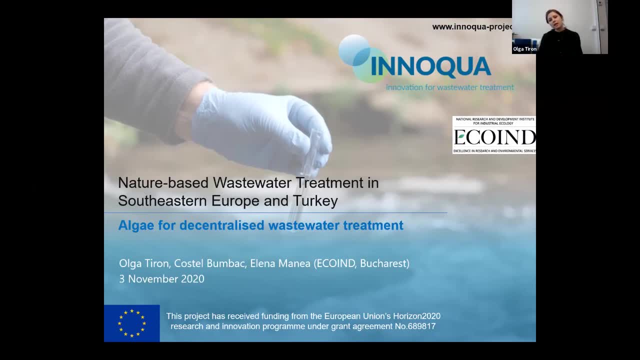 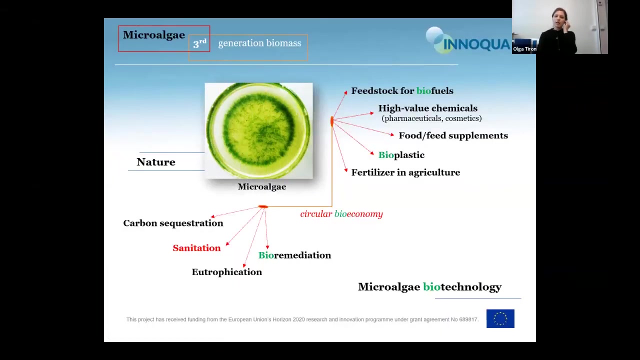 biotechnology testing, covering both reported results and the experience gaining from several demonstration sites tested, the within the inocua project. i'm not. micrology represents one of the primary producers of the aquatic ecosystems, which means that nature provides us with the specific microorganism. uh full cellular composition and metabolism led to. 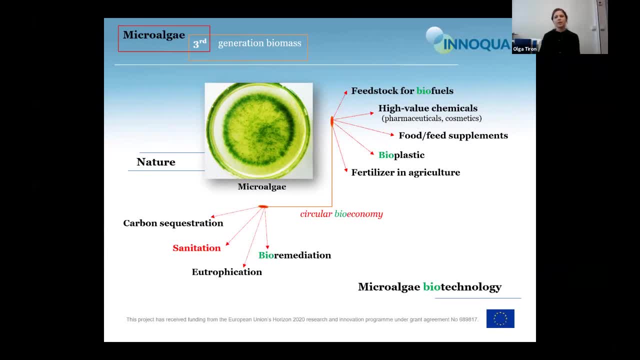 the development of a worldwide multiple branching industry. referring to microalgae biotechnology being applied in socioeconomic sectors such as biopulse production or pharmaceutical industries, and addressing as a solution to cool environmental issues, as for example greenhouse gases, emissions by carbon sequestrations, ecosystems, pollutions via bioremediation potential, or even to sanitation uh issues, all these features. 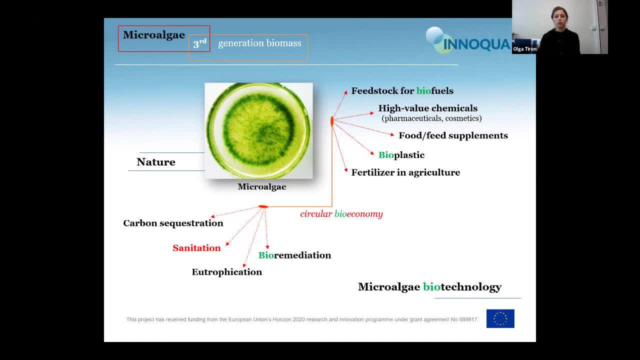 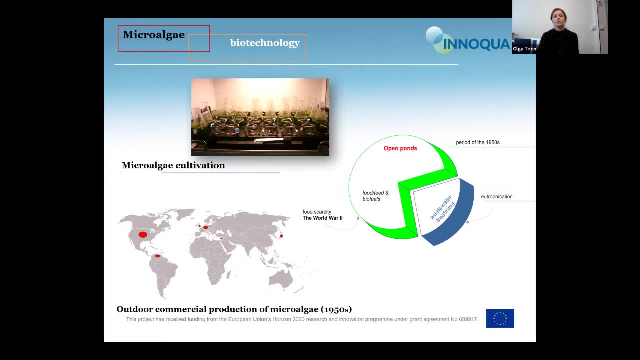 made microalgae as one of the targets of the circular bioeconomy. the beginning of a microalgae biotechnology path was represented by biomass cultivation direction, initiated mainly as a result of the food resources that were used to produce microalgae as a source of food resources, 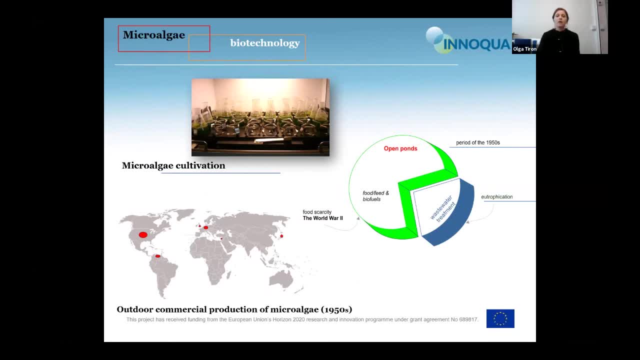 depilation caused by world war ii period. once agriculture recorded an upward trend after world war, the interest for microbiology cultivation from protein production decreased. however, the interest switched to use microbiology for domestic wastewater reflux, polishing the idea being to harness uh microalgae metabolic features to avoid the ultrafaction phenomena. 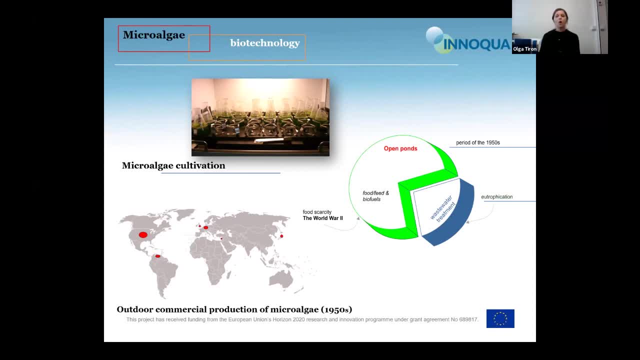 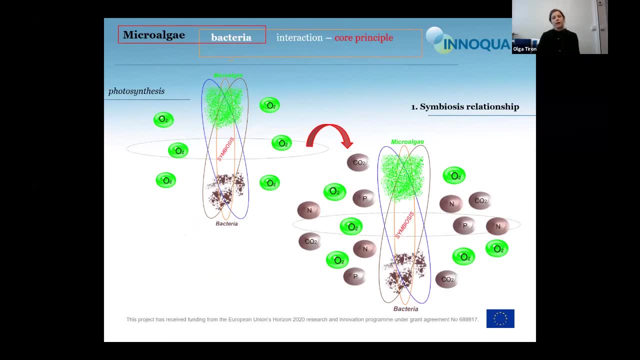 caused by the discharge of the nutrient-rich effluents overloaded with uh- nitrogen-rich. There are two main criteria that sustains this idea. First of all, we are speaking about the symbiosis relationship occurring in natural ecosystems between microalgae and bacteria, The core principle of the symbiotic relation harnessed into the wastewater treatment process. 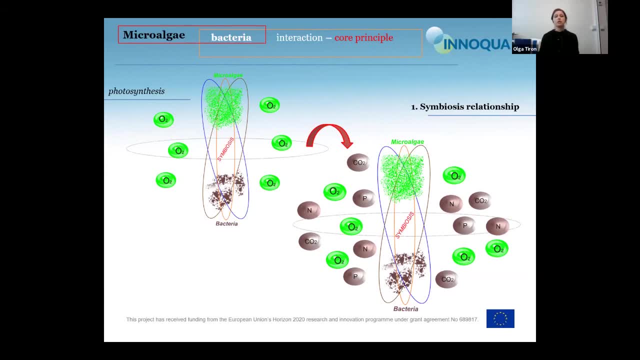 is represented by a nutrient support exchange established between microalgae and bacteria Multi-population. provide oxygen supply by photosynthesis, which is consumed by aerobic bacteria for organic matter degradation and nitrification processes as well. Release macronutrients after degradation, mainly nitrogen, phosphorus and inorganic carbon, being captured by microalgae. 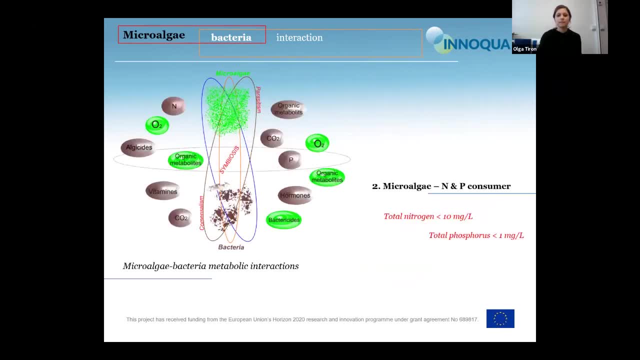 point cell group implicitly for photosynthesis. Besides the core principle of the macronutrients exchange, the interaction between microalgae and bacteria population is very important. they tend to be apart from each other because macronutrient interaction is more complex. 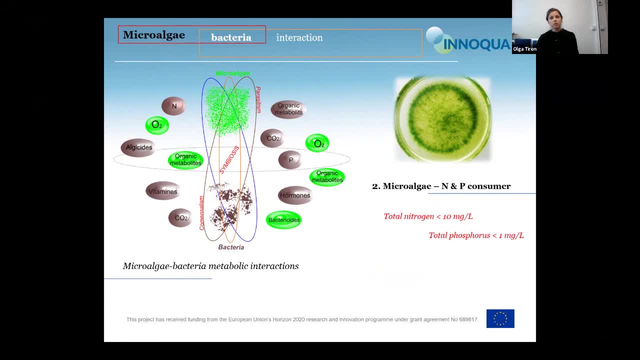 and could comprise unidirectional relationship or parasitism relationship, as well as also toxic interactions. could be interspecies, intraspecies, cross-kingdom or inter-kingdom. Besides macronutrients, growth stimulatory compounds could also be represented by other 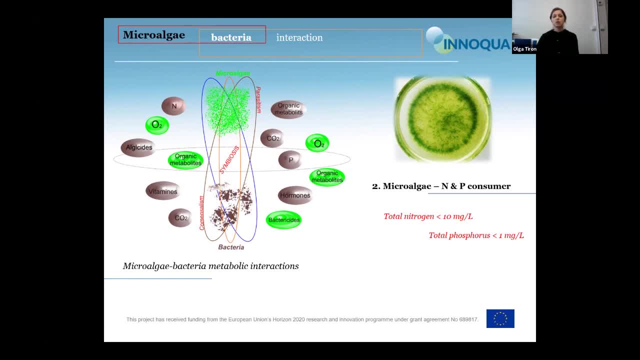 metabolites, bacteria species being providers of essential for microalgae cell group compounds such as vitamins and hormones. the criteria that sustains the use of a microalgae bacteria biomass for effluent polishing is represented by the microalgae cell ability to consume nitrogen and phosphorus at even very low. 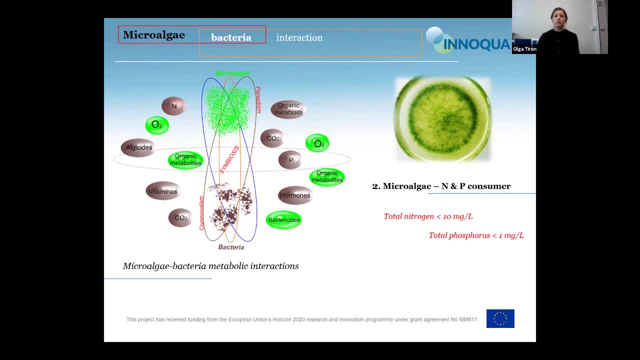 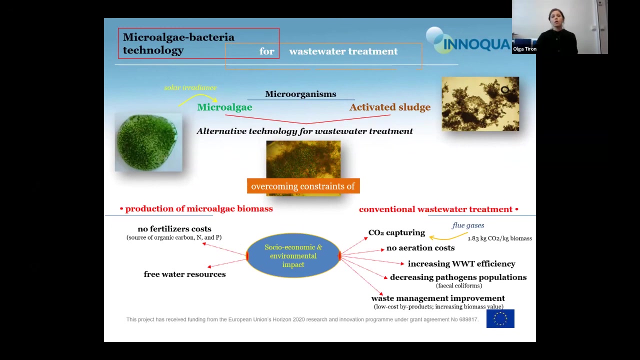 loadings when our applied technologies are proven to be inefficient. Moreover, as in the case of accumulating, bacteria used in an enhanced biological phosphorus removal step, while microalgae are able to accumulate higher phosphorus content than that required for cell development. But now let's take a closer look on what impact could have occurring microalgae-bacterial 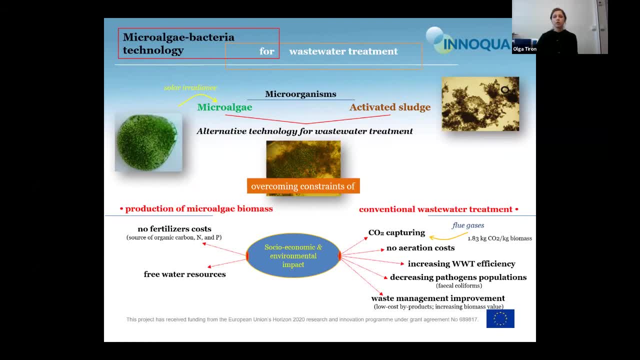 interactions on both wastewater treatment operation and microalgae cultivation systems. First of all, microalgae can be used not only in tertiary treatment steps, but as also for secondary treatment, resulting in an integrated technological flow for increasing the socio-economic and environmental impact. as the microalgae cultivation and the wastewater 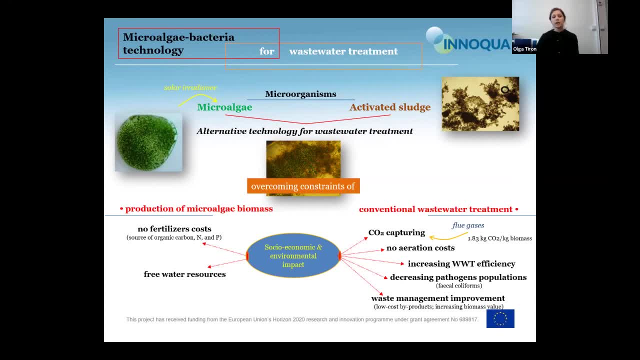 treatment technology based on activated sludge, facing various constraints and the drawbacks Regarding production of a microalgae biomass. wastewater provides for microalgae-bacterial interactions and microalgae-bacterial interactions. The microalgae population necessary nutrients and the water resources only require inorganic. 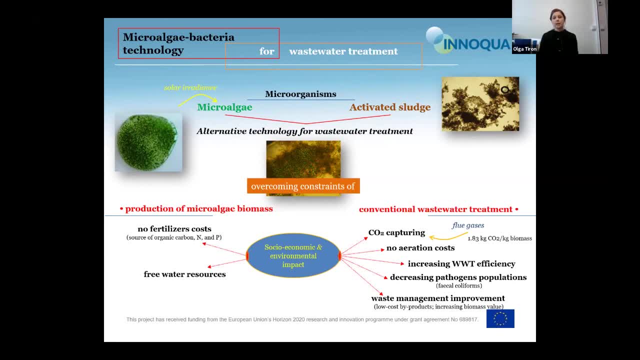 carbon supply, representing up to 27% of the total cultivation costs. Moreover, phosphorus represents a limited resource with a high deflation risk in the next decades, and the nitrogen is considered an important limiting factor in assessment of the microalgae biorefiners' sustainability and potential scaling. Regarding the advantages that could be achieved, 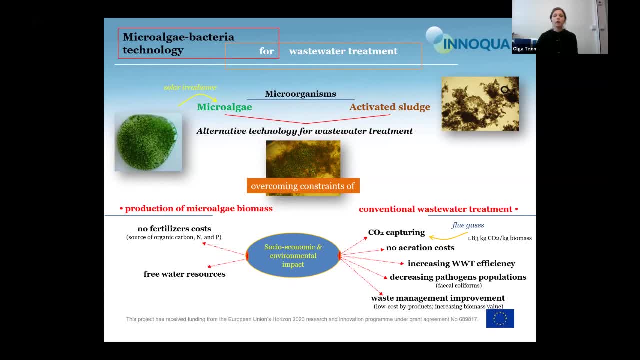 by using microalgae-bacterial biomass for wastewater treatment, could be pointed the following: Decreasing the elimination of the CO2 gas emissions, which is the main contributor to the greenhouse gases emissions. Moreover, conventional wastewater treatment technologies represent the top. conventional wastewater treatment technologies represented the top. 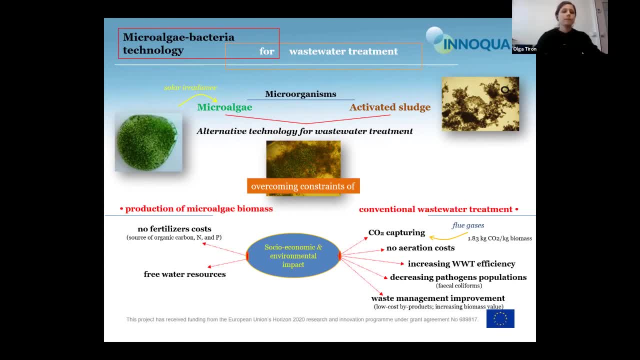 contributors of the greenhouse gases emissions and the water industry and one of the three top contributors of the greenhouse gases emissions worldwide. CO2 could also be used from flue gases such as was resulted from natural gas power plants. Microalgae provides also free oxygen supply. Mass aeration is the most energy-intensive process during wastewater treatment. 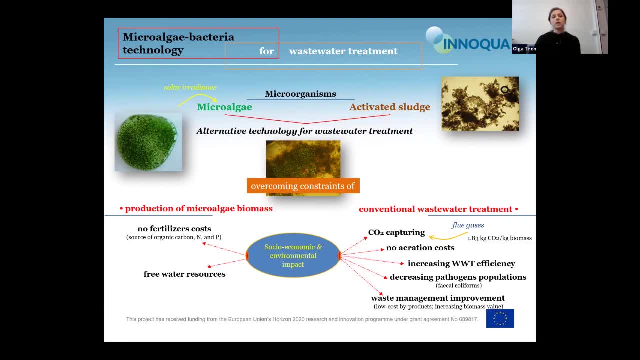 Accounting for about 40-60% of overall operation costs. Experimental results obtained by Quinn's team in ongoing microalgae related projects showed that microalgae biomass could not only sustain the necessary oxygen level required by aerobic bacteria for both organic matter degradation and amplification, but as also could frequently. 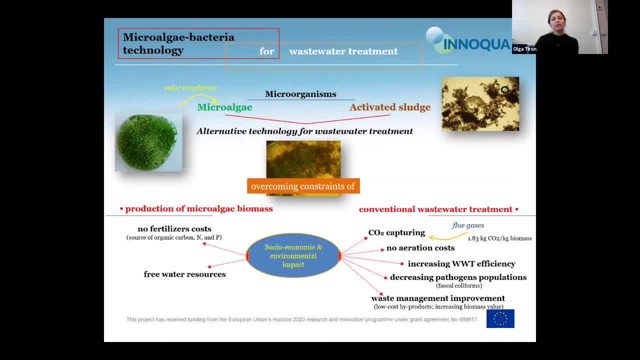 exceed 100% of oxygen saturation during the light phase, being maintained only with a small amount of water. In general, the amount of sodium in the microalgae, which is used as a free source to generate oxygen, is more than 30-50% during the night. 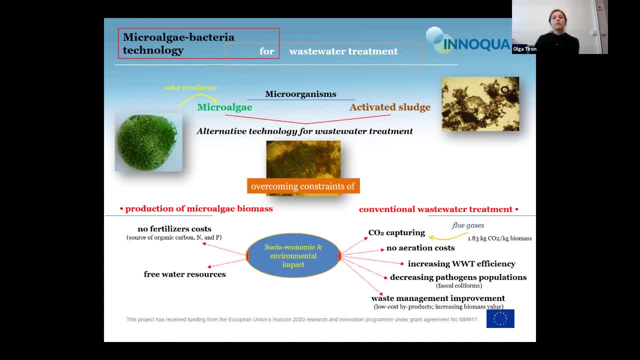 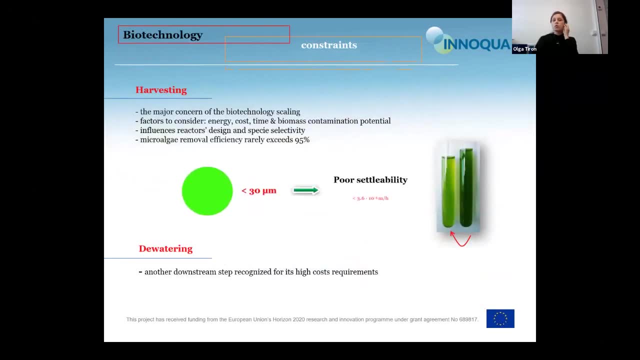 period, depending on operation treatment sizes. Moreover, replacement of a mechanical aeration with a biological-based oxygen-generated process decreases the risk of pollutants volatilization. However, besides several social and economic impediments, data from the microalgae biotechnology region. 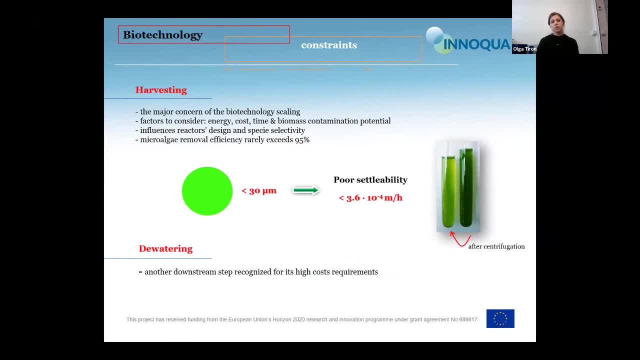 which influence outdoor scaling of some biotechnology branches, One of them being applications for wastewater treatment. Which are the biotechnology limits? First of all, harvesting Cost and energy input linked to microalgae harvesting remained a significant issue even from the first years of experimental investigations. 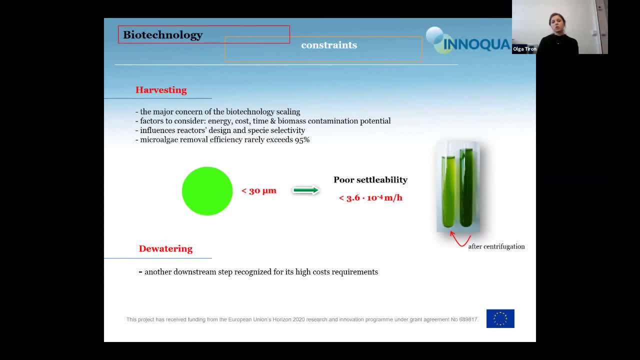 of the microalgae biotechnology and represents the measured concern of the biotechnology scaling. More than 50% of the research papers addressed the algae-based wastewater treatment technology, or microalgae cultivation, bringing into question the harvesting step. A lot of efforts were and are made in this direction. 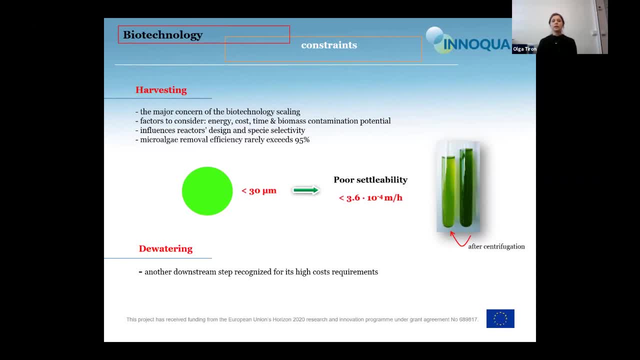 to overcome harvesting-related problems, such as those linked to energy cost, time and biomass contamination. Moreover, reactors design and microalgae species selectivity are highly important. However, there are many problems to be easily influenced by harvesting efficiency. The harvesting problems come from microalgae cell particularities. 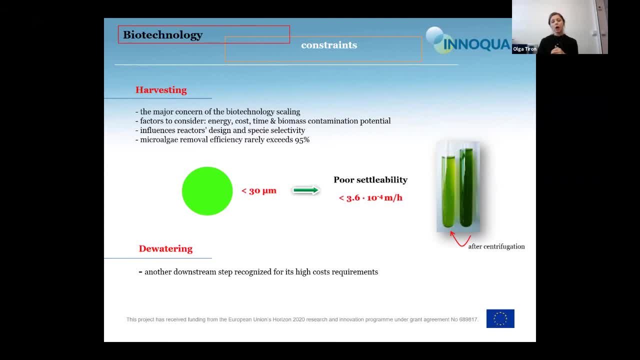 The most commonly used species have a gas cell diameter lower than the first micrometers and the cellular density is similar to that of water. The most frequently applied harvesting methods, such as centrifugation and chemical flocculation, do not ensure efficient harvesting And even two or more harvesting methods. 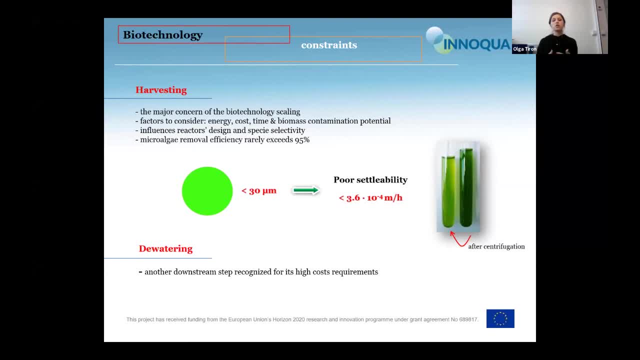 such as centrifugation and chemical flocculation, do not ensure efficient harvesting And even two or more harvesting methods, such as centrifugation and chemical flocculation, more harvesting techniques are applied, the microalgae removal efficiency rarely exceeds 95%. 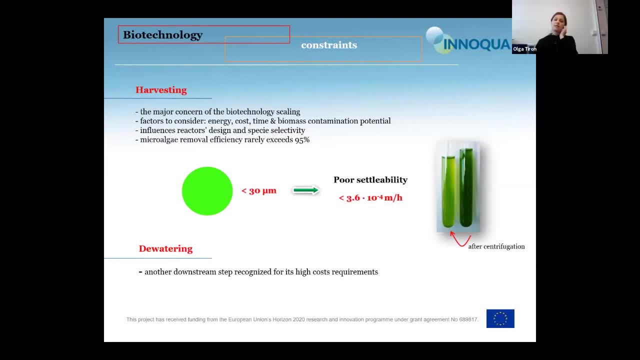 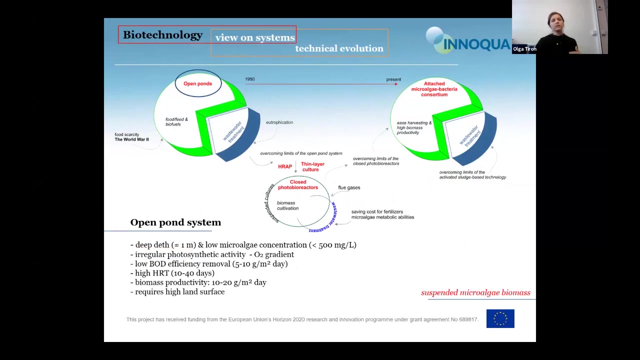 being affected the effluent quality and compromising the system functionality. Dewatering is another downstream step, recognized for its high cost requirements. Proper biomass humidity level must be ensured before biomass extraction phase. Biotechnology scaling represents heavily discussed topic, facing not only economical challenges. 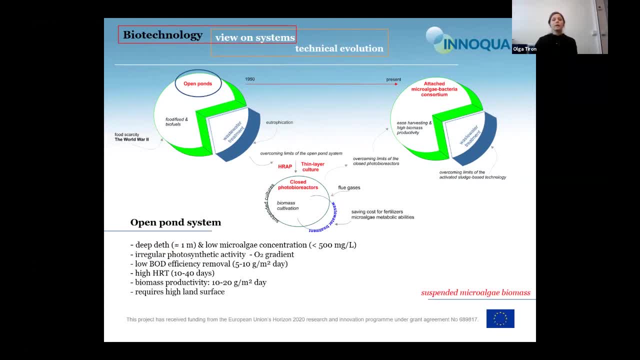 but as also several technical ones At the beginning of the biotechnology development for wastewater treatment. the process occurred mainly in open pond systems characterized by a rather deep depth low microalgae concentration, which increases costs for microalgae harvesting and watering. 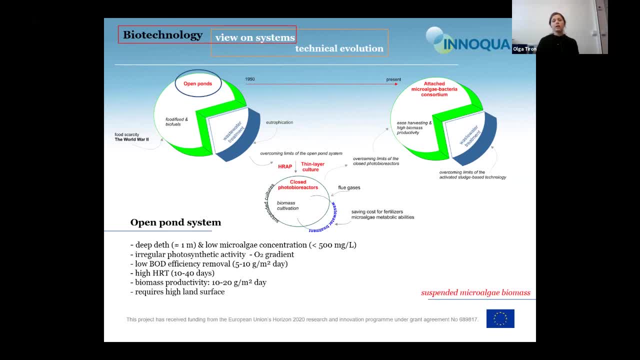 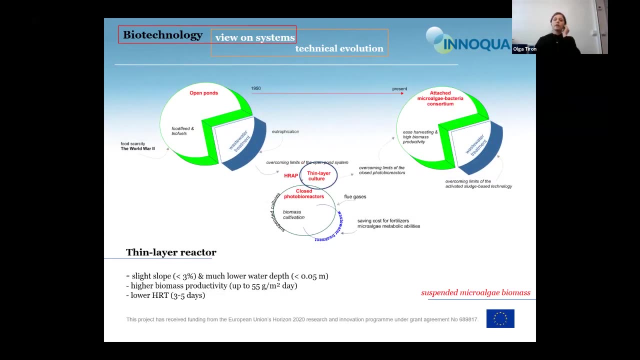 The system also presents irregular photosynthetic activity conducting to the appearance of an oxygen gradient and to a low BOD efficiency removal requiring a high hydraulic rotation time. Starting with 1960, thin layer reactors were proposed in order to overcome open pond limits. 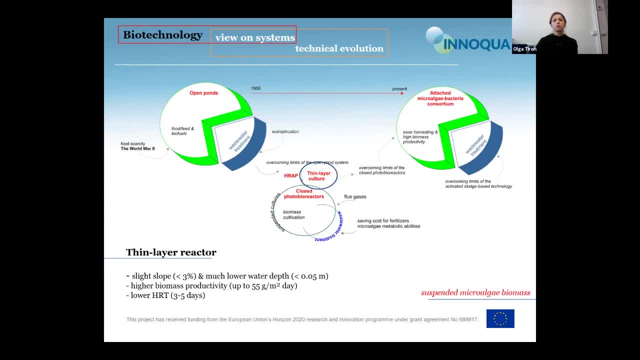 Thin layer reactors are represented by a slight slope in order to avoid biomass settling and much lower water depth, Properties which sustain the increase of a photosynthesis efficiency and biomass productivity, as also the decrease of the hydraulic retention time. Close to wet period, high rate algal ponds were tested for secondary 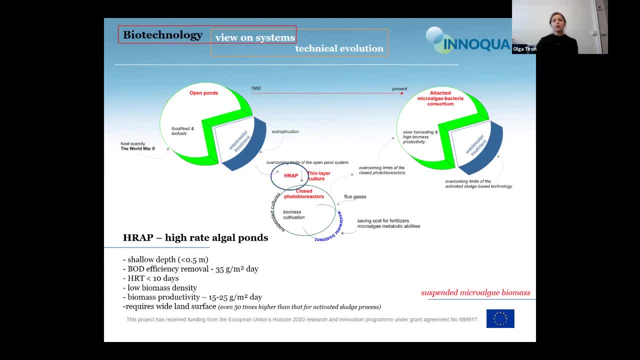 and tertiary wastewater treatment, mainly domestic and agricultural water resources. This type of ponds are characterized by a small, a small depth being provided with mixing system which allows an increase of the photosynthesis activity and organic matter removal efficiency. lower hydraulic retention time. 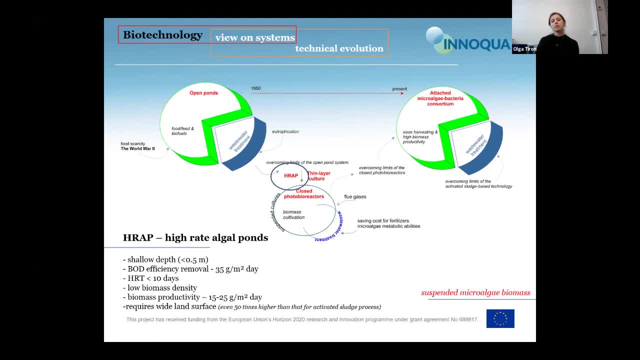 However, they are represented by low biomass density and the biomass productivity and require wide land surface, even 50 times higher than that needed for activated sludge process. Compared to open ponds, photo bioreactors allow better and ease operational control and the higher biomass productivity. 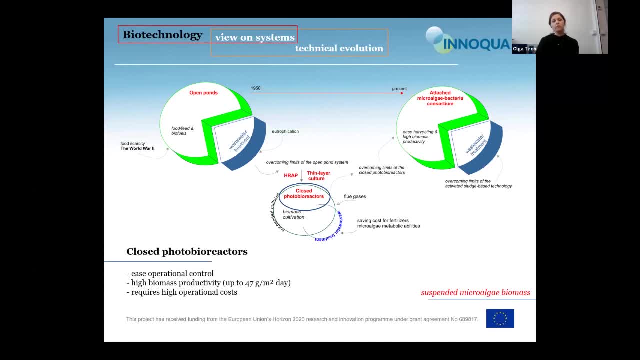 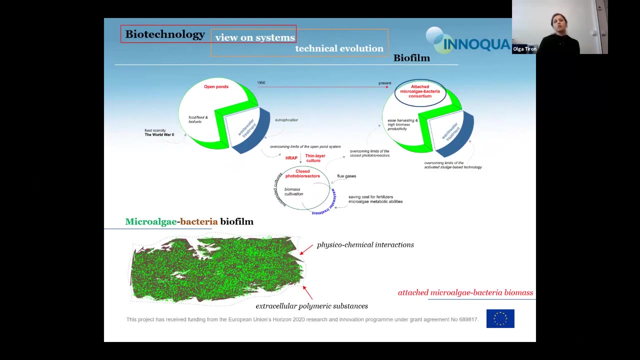 However, they requires high operational costs, especially for mixing, but could be by even 15 times higher than that required for open ponds systems. With about three decades far from the first signs of the microalgae biotechnology development for wastewater treatment, the idea is that you know. 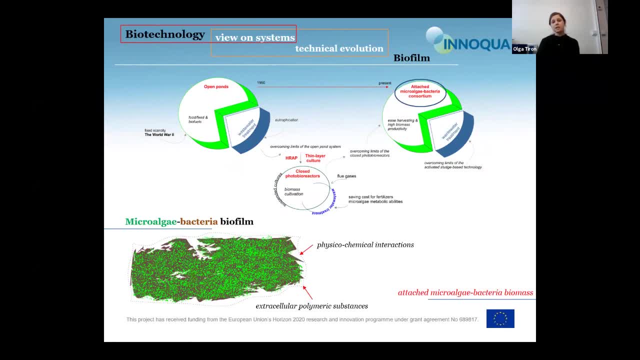 the microalgae biotechnology is a very important part of the development of the system. In addition to the microalgae biotechnology development, the algae-based biofilm reactors hold the last step in line with the microalgae biotechnology development history. 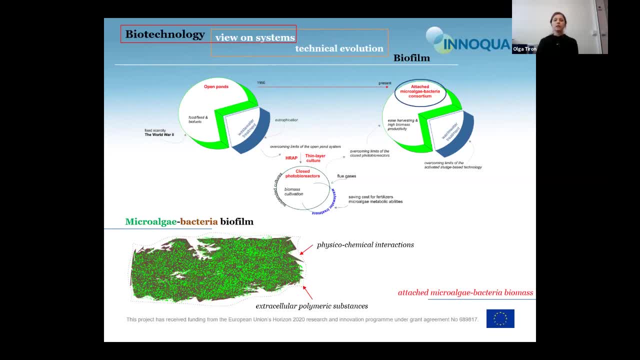 Advancement of this type of system was not so visible as in the case of the suspended microalgae applications, as algae-based biofilm presented many interest in the wastewater treatment processes rather than for commercial biomass culturing. Algae-based biofilm represents a dense 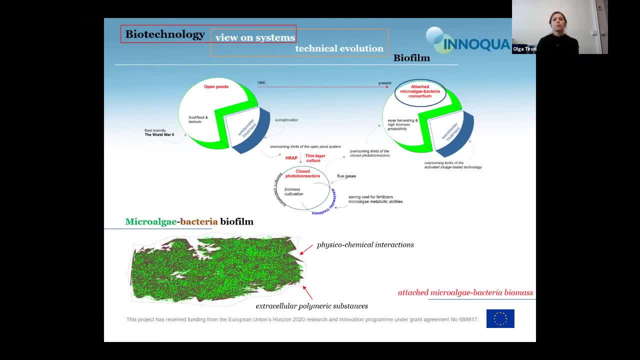 and multilayer biological structure consisting of a mixed population of microalgae and bacteria and developed by a physical, chemical and biological attachment mechanism on the surface of the specific material. What are the strengths which promote the use of the biofilm system instead of the suspended cultures? 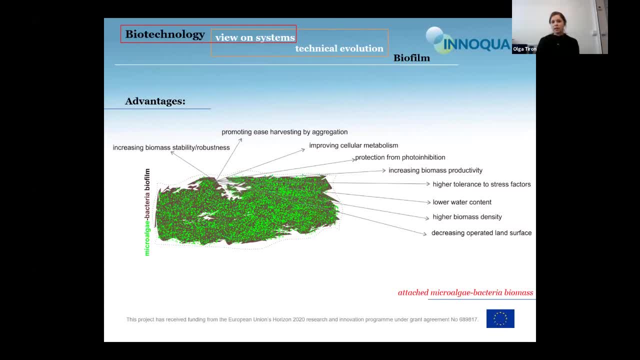 for wastewater treatment. First of all, speaking about harvesting, the attached biomass can be eased harvesting by scrape with no energy input requirements, as also biofilms have higher biomass density, even up to 100 times higher, compared to the performance of the open-point systems. 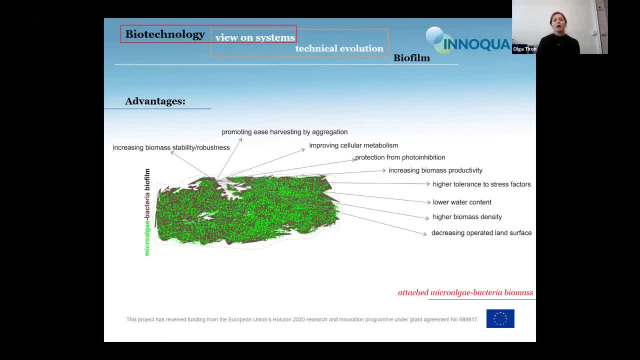 allowing decrease in the operating land surface. The biomass organization allows the decrease of the biomass water content, the scrape biofilm having a humidity level similar by that resulted after centrifugation or after centrifugation, or even this means that allows the exclusion of the harvesting step, while saving energy. 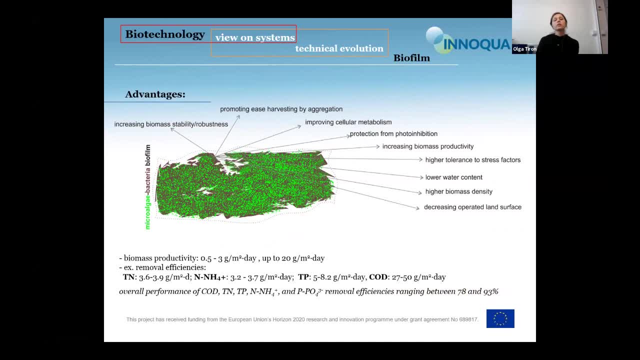 Biofilms have higher biomass productivity. commonly reported performance for algae biofilms ranging between 0.5 and three grams per square meter per day, but could reach even around 20 grams per square meter per day. Biofilm properties sustain higher wastewater treatment efficiency. 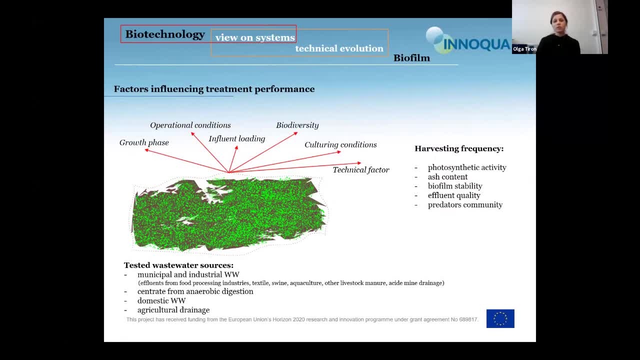 compared to suspended cultures, higher robustness for a wide range of wastewater types being found and can sustain both nitrification and denitrification processes by uneven oxygen distribution. In terms of wastewater treatment performance, the organic matter and nutrients removal efficiencies vary in a wide range, depending 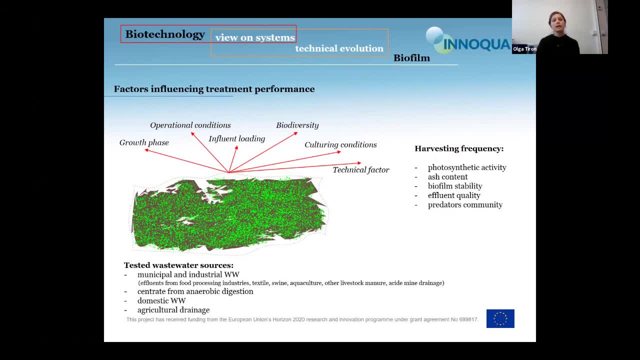 on multiple factors such as the reactor design, scaling involved, microalgae and bacteria species, implant loadings, harvesting frequency. The impact of harvesting frequency must be especially pointed as it influences the photosynthetic activity, influences ash content, biofilm stability, effluent content. 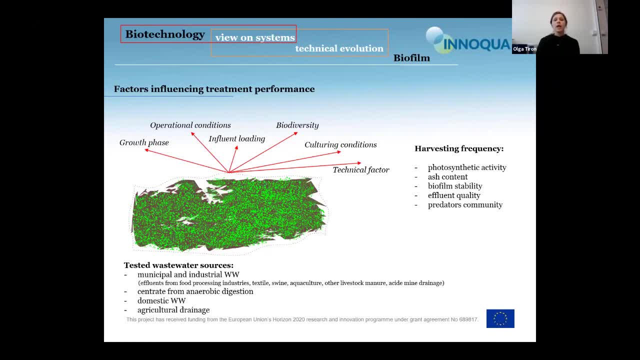 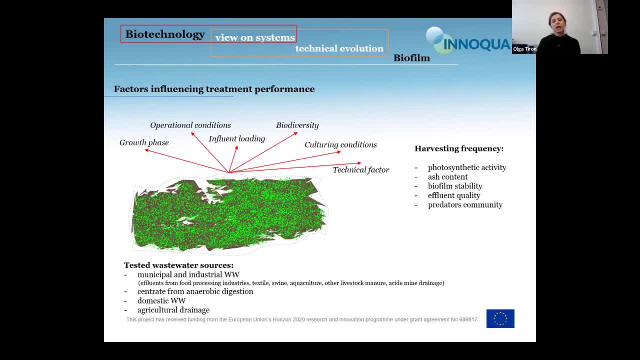 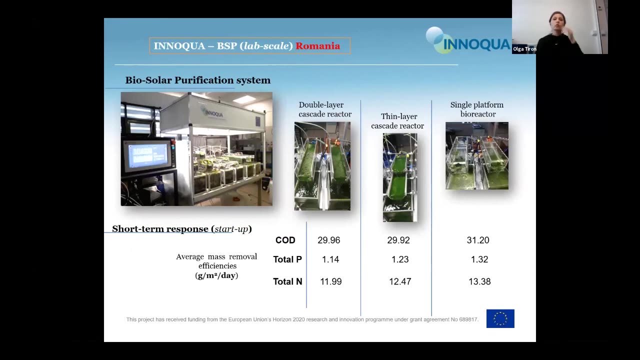 on a wide range of wastewater sources. on a wide range of wastewater sources, but a lack of experience of biofilm large-scale application was noticed to perform outdoor studies accounting less than 10% of found related publications. Farmer's several important achievements will be outlined here: gained 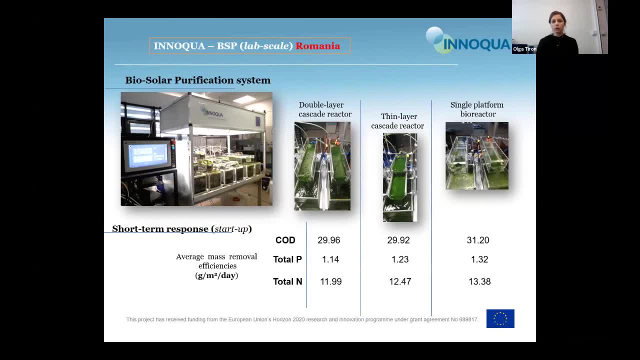 on microalgae bacteria biofilm testing for effluent polishing at laboratory scale and demonstration sites within Inoha project. before pilot scale design and microalgae bacteria biofilm testing in outdoor conditions and microalgae bacteria biofilm testing in outdoor conditions, Lab scale experiments were conducted in order to establish the influence. 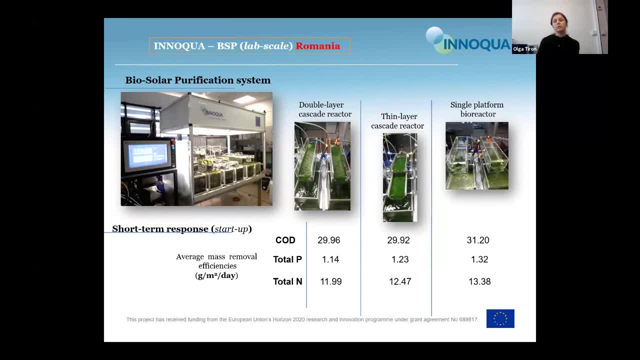 of the several technical and other operational sectors. on treatment performance, The system performance was monitored during the start-up period on three types of reactors: double layer cascade reactor, thin layer cascade reactor and single platform reactor. Under given operational conditions. the results emphasized quite close treatment performance between reactors. 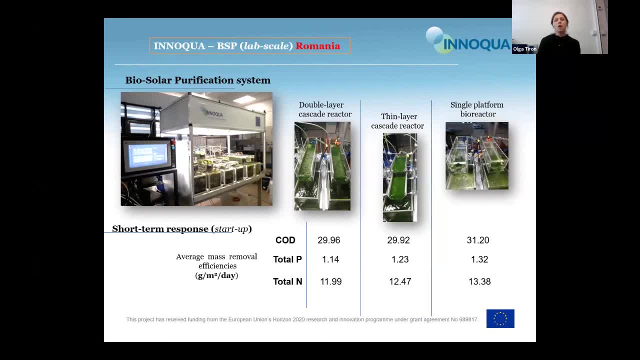 which allowed some fluidity to be achieved. However, the higher the flexibility in choosing the design reactor for pilot scale testing, Long-term assessment of the reactor's performance after the start-up period underlined an increase of organic matter, total phosphorus and total nitrogen removal efficiencies in line. 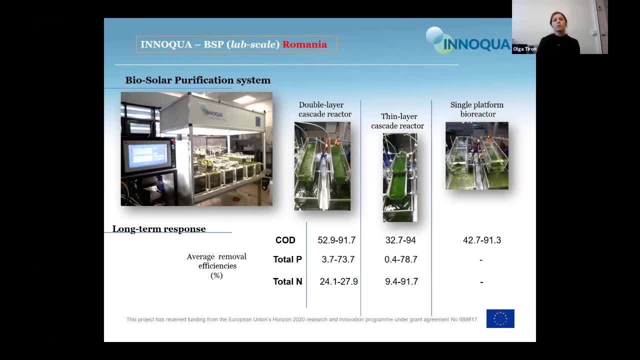 with the increase of the solid retention time. However, for long exponential growth phase of the biofilm affected the pollutants removal efficiency. So this has led to some significant changes and outlining in this way the importance of the harvesting frequency factor on systems performance. 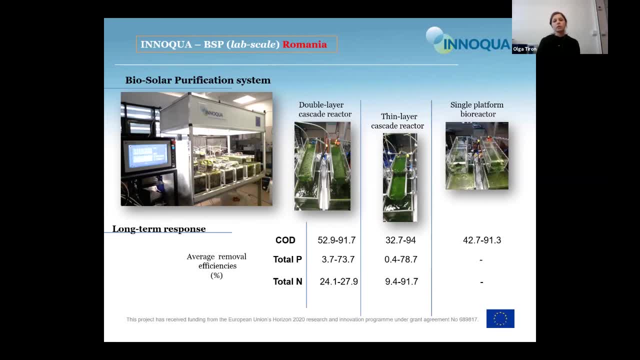 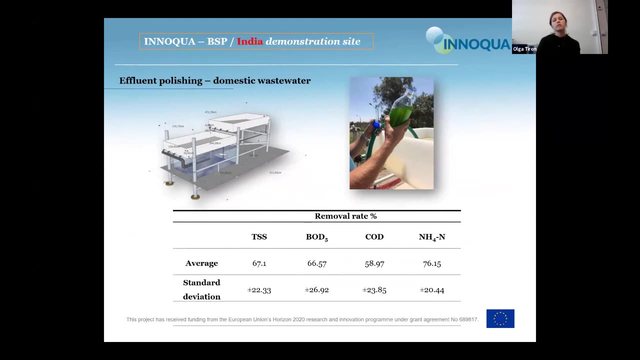 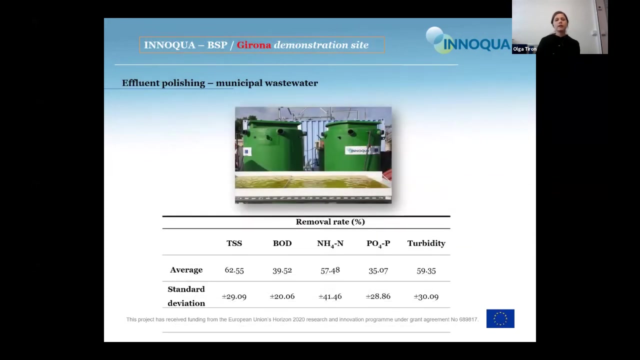 Obtained results were used for outdoor technology. obtained results, in this case at laboratory scale, were used for outdoor technology implementation. As a bet from India used for a plant polishing originated from a domestic wastewater source, the results being outlined in their page table, or As here it is presented as a demonstration. site tested in Girona, which used also the solar pollution treatment step. 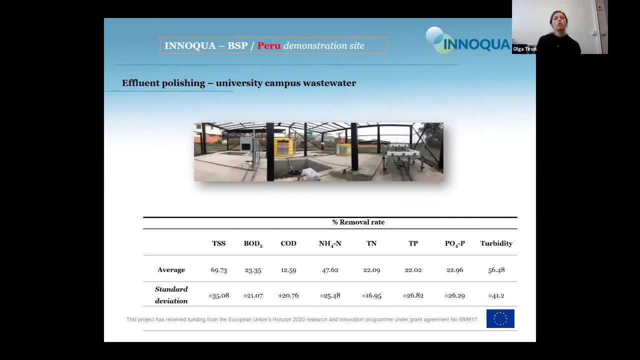 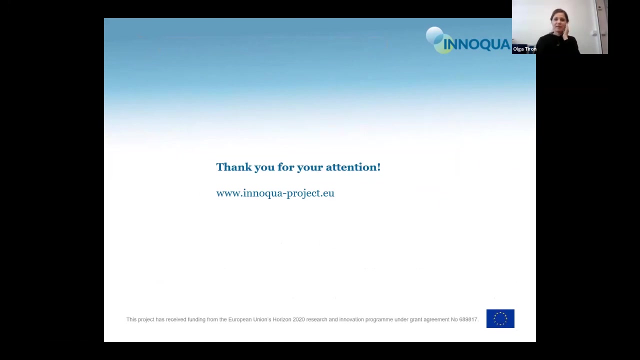 And But from Peru. more detailed information about systems performance related to advancement treatment step using microalgae based biofilms in different geographical locations could be provided as a request. Thank you for your attention and if there are any questions. Thank you, Olga. Looking at the audience now, if I can see some hands. 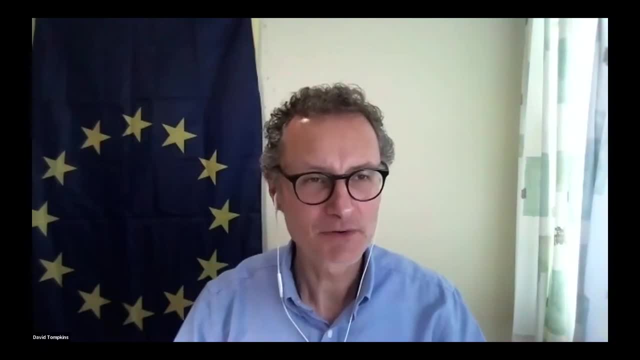 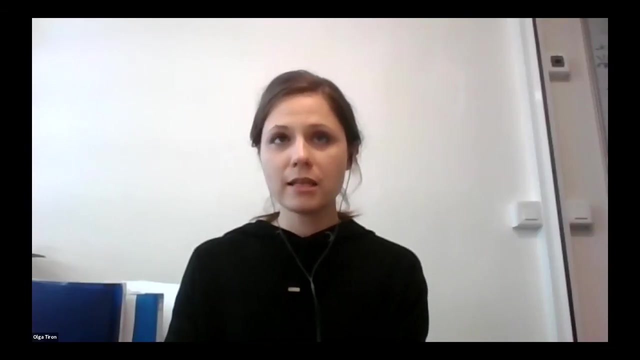 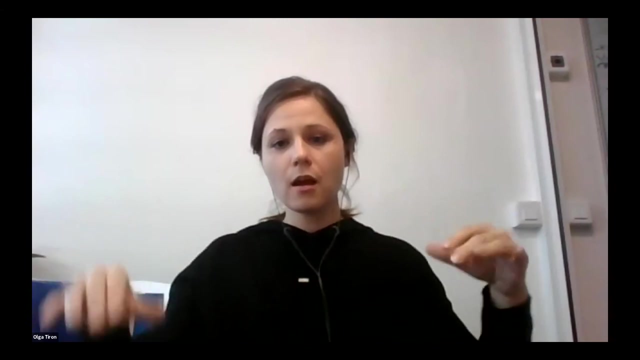 Yes, please, David. A quick question, Olga. Are there any commercial systems using this kind of algae bacterial biofilm at the moment or is that, that approach, relatively new in the market? It's relatively new. There are several pilot scales successfully tested, but only several, mainly at the equatorial regions. maybe lower than 10 pilot scales, because 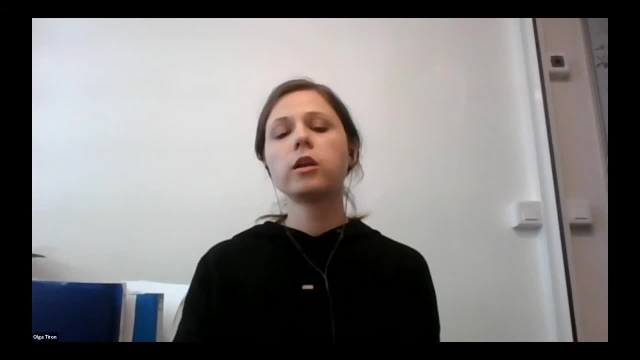 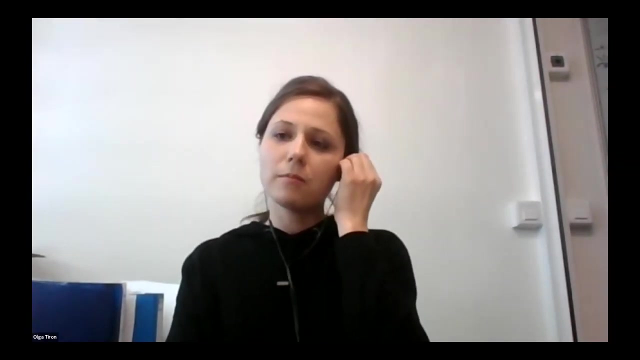 usually it was used closed photobioreactors in order to control all operational factors and was easy to test. Environmental conditions influences very, very much the treatment performance and it is hard to implement at the pilot scale. For this reason, the technology is in developing now. 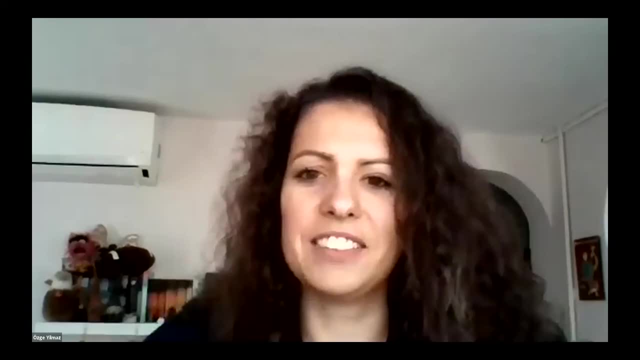 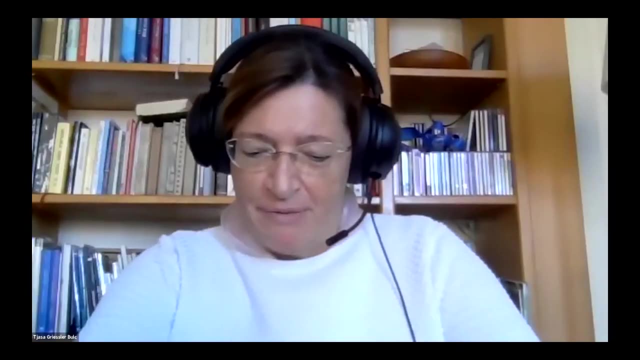 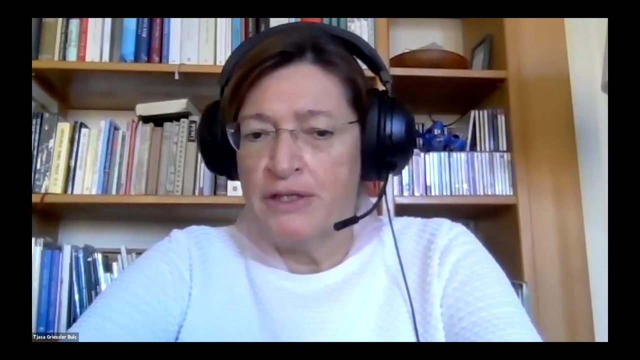 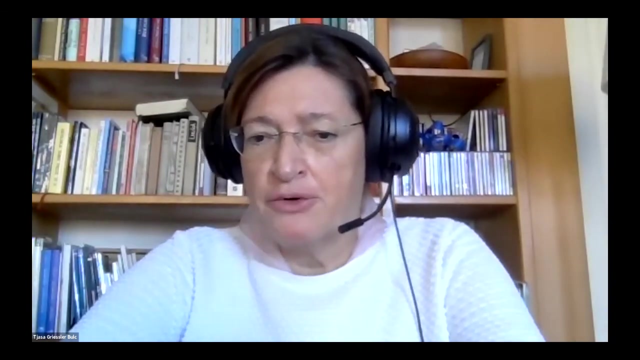 Thank you, I think we have another question. Please go ahead. Yes, thank you very much for a very interesting presentation, And I would like to first pose a question about the ratio between the bacteria and algae community. So how could you control that you don't have too much bacteria or too less algae, or vice versa, so that the symbiosis relationship would be the most efficient one? 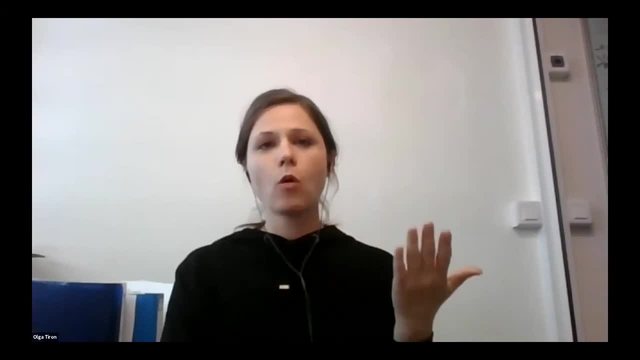 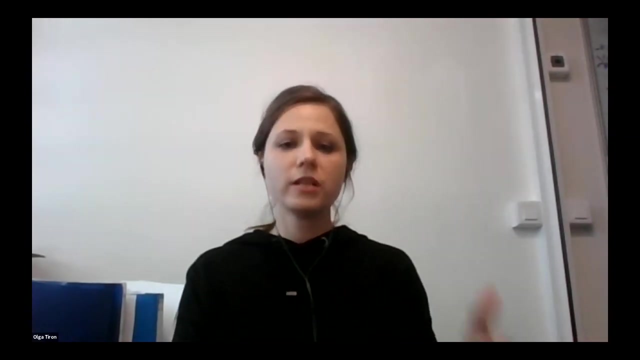 In this case, it depends on what type of waste battery we use. If we use wastewater with lower loadings, lower than 500 milligrams COD per liter, we can make. there are multiple factors that influence these systems, Beginning with influent loading, and also solar irradiance is very important- light irradiance. 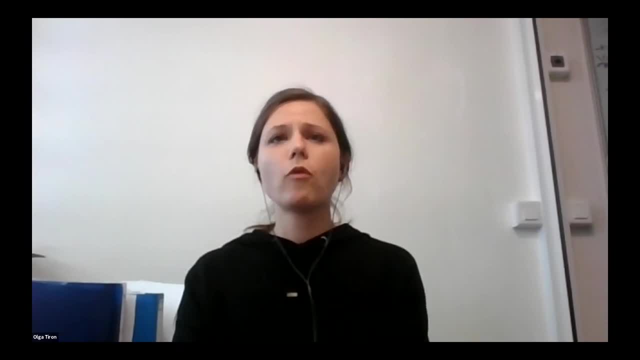 For this reason, every test must be performed- is linked with one type of wastewater, For example. if you need, if you test daily wastewater under optimum light conditions, you can see that maybe the bacteria could overload. the balance between bacteria and microalgae could be. 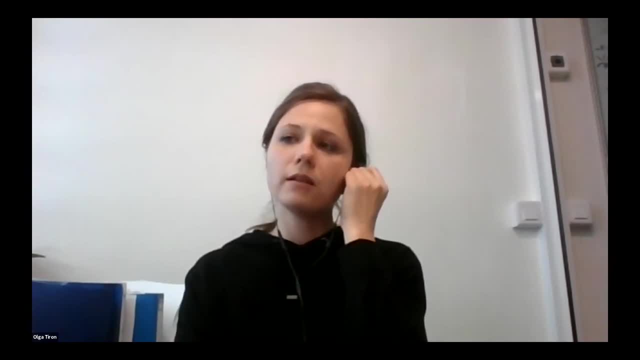 I don't know higher than, and it will be determined. the shade shading effect will be on microalgae. It depends on what type of wastewater is testing and what operational conditions are. Maybe for this reason pilot scale testing is so so few tests performed outside. 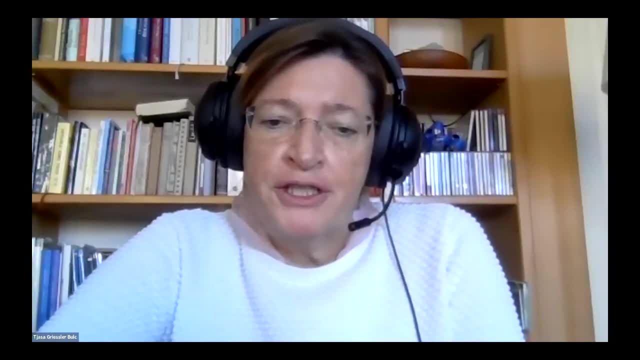 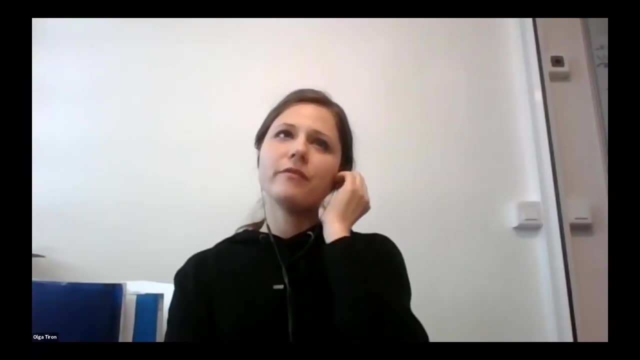 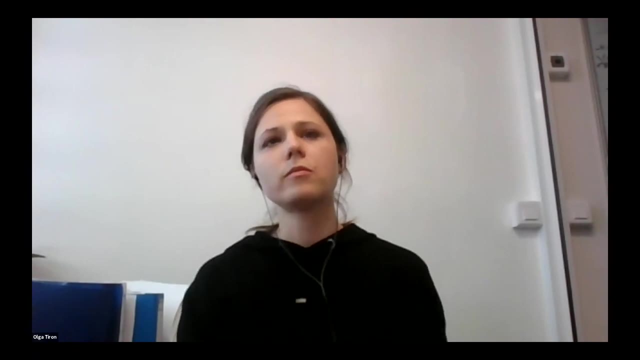 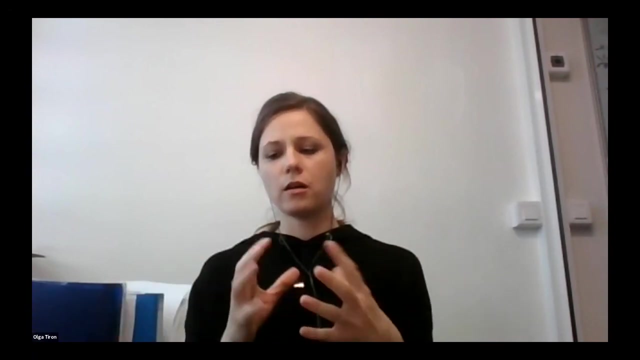 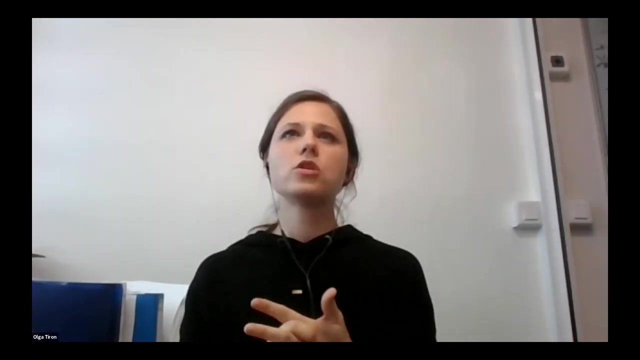 So what kind of ratio you would you suggest for the common communal wastewater like a sewage? There is no information about the ratio because the interaction, the describing of the microalgae bacteria composition is quite new. The In order to research the interactions- how much bacteria, how much microalgae- is quite new methods applied in this field. 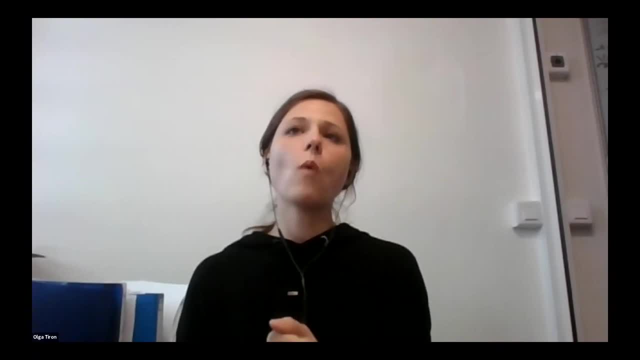 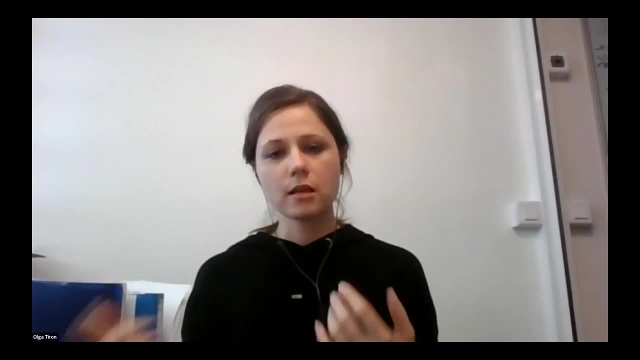 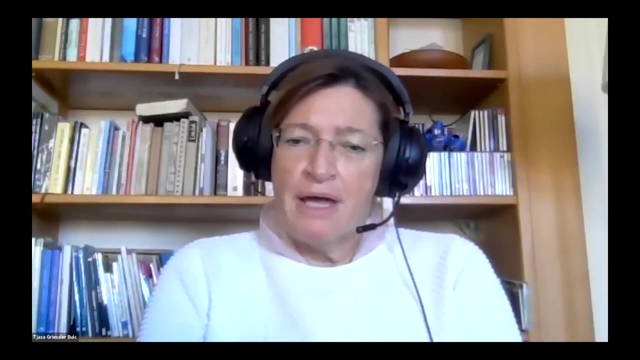 And there is no information on what ratio must be. Also, it depends on other factors such as implant characteristics and other operational conditions. So the answer I mean, as I understand you, the best option would be to test with the pilot scale and then see what the ratio would be the optimal for specific case. 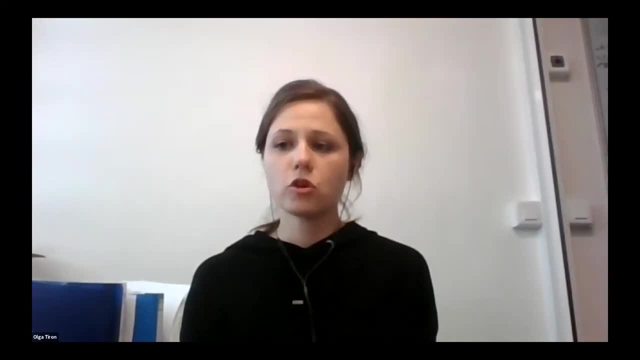 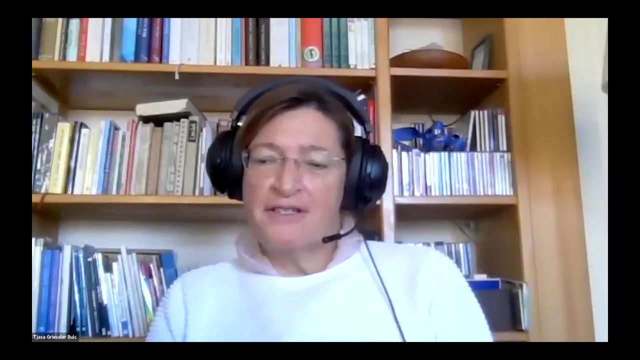 Yes, it's specific for geographical location, for conditions, for what type of microalgae you test. Yeah, of course, for the species. And another question, if I can be quick: What is the best harvest application? What is the best application that you can suggest out of your experiences? For the, maybe the algae pond, which is maybe closed, Which would be the best harvest option, Because this could really be a challenge. Yes, The most applied harvesting is centrifugation, But it consumes a lot of gas. It consumes a lot of energy. 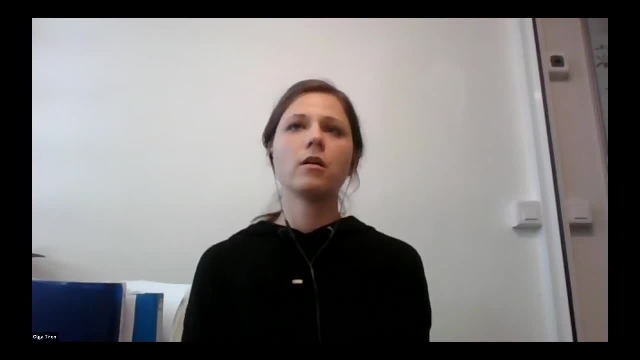 We, besides biofilm, we developed in the institute an alternative biomass structures, granular structures which could be used as suspended biomass, which allow the settlement of microalgae within minutes. But it requires also is undergoing research in this case, And it is an option to cultivate the microalgae even in open ponds systems. 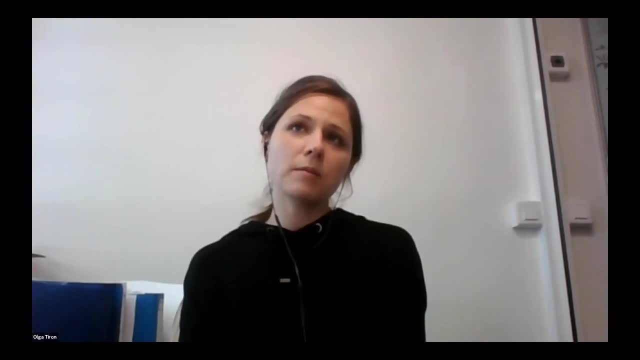 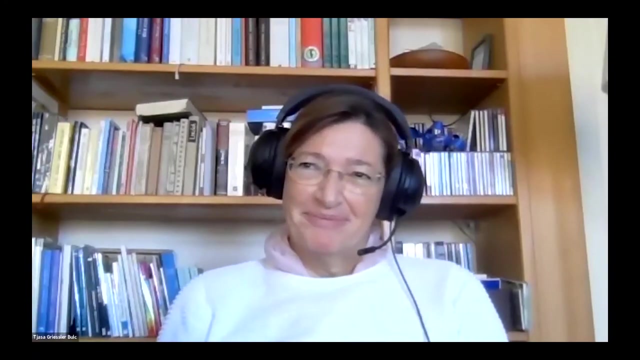 But regarding the used, frequently used applied methods, each method has its disadvantages, such as high energy or biomass contamination with metals due to the flocculation. Yeah, Thank you very much. It depends. it depends. it depends on what type of microalgae have the open ponds systems. 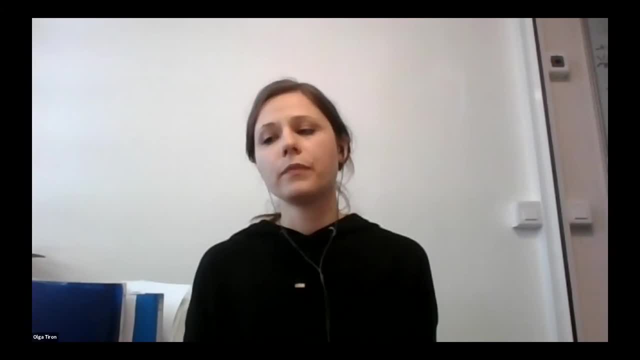 Usually the filamentous microalgae facilitate better, easier sedimentation of the biomass. The presence of the filamentous microalgae it is. it is an option for decreasing the energy costs, But it is also a very important factor in the development of microalgae. 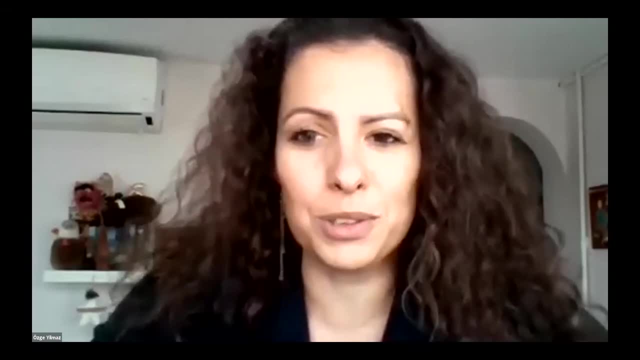 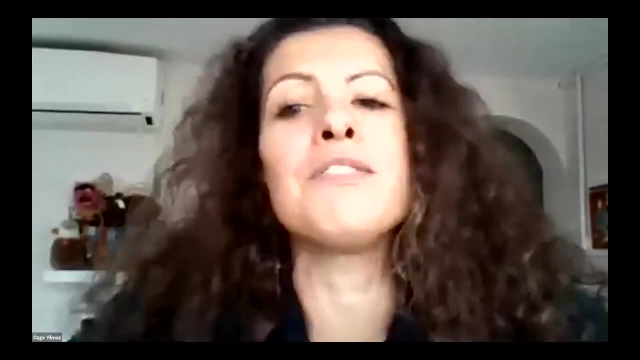 So I'm delighted to introduce you Dr Asman Korkusuz, who is a long time friend. We are both curly, We're here, So Asman is a very busy woman. She is the research and development project coordinator of Optima Engineering. 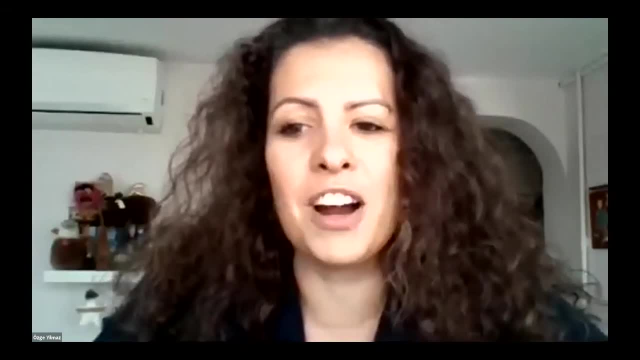 Also the deputy general manager of Optima Environmental Technologies in Turkey. She is also a part-time instructor at Middle East Technical University. She is also a part-time instructor at Middle East Technical University. She is also a part-time instructor at Middle East Technical University. 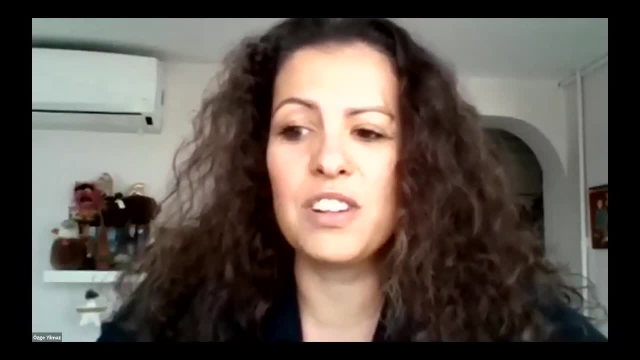 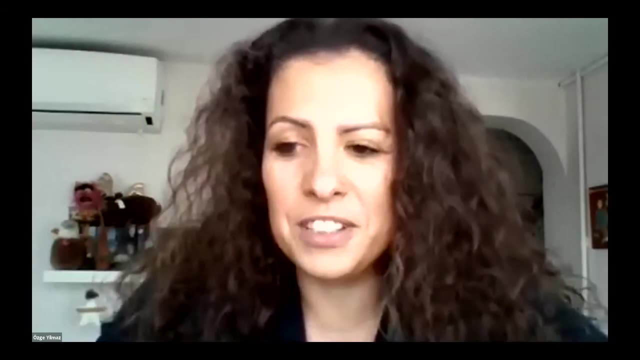 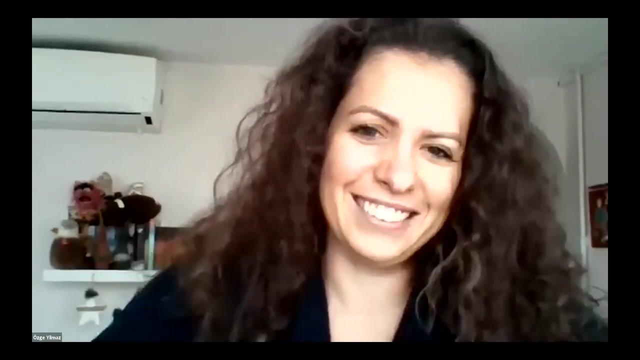 Her areas of interest involve constructed wetlands for wastewater treatment, ecological solutions and waste management. So Asuman will deliver her speech on constructed wetlands for domestic wastewater treatment in Turkey. Asuman, we are ready to listen to you, Thank you. 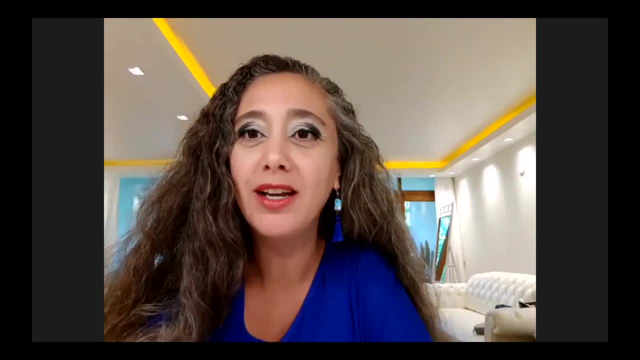 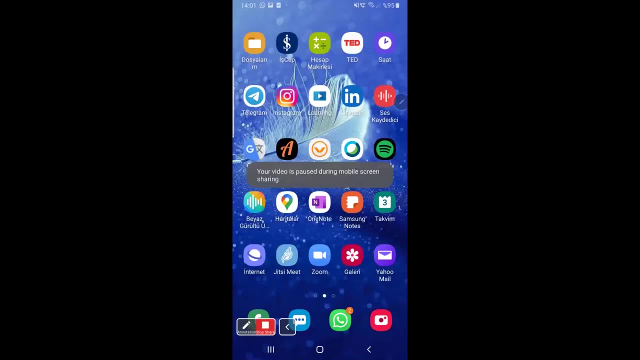 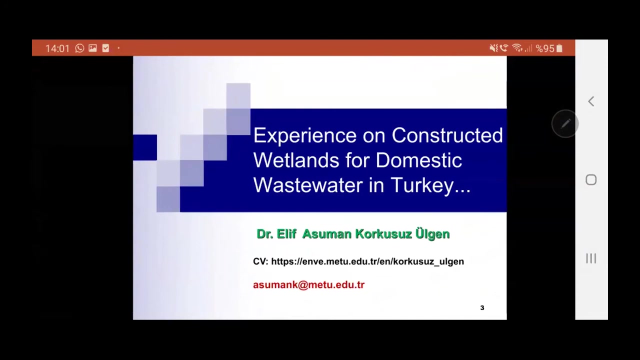 OK, thank you so much for the nice introduction. I am trying to share my presentation screen, OK. OK, can you see it? Yes, we can. OK, great, because I cannot see myself, because I'm connecting to it through my mobile phone. 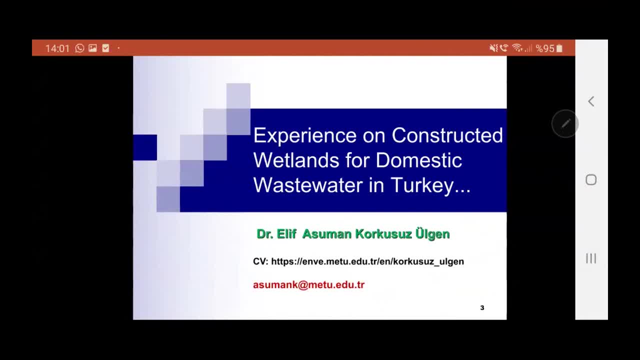 Greetings to everybody from Antalya. I'm sorry. I'm in Antalya in a very nice situation and in a very lovely atmosphere, But tomorrow I will be also traveling to Ankara, So thank you so much for your time. Thank you for the invitation, for the nice webinar. 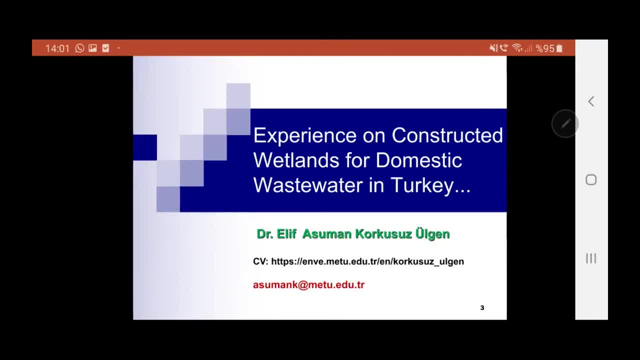 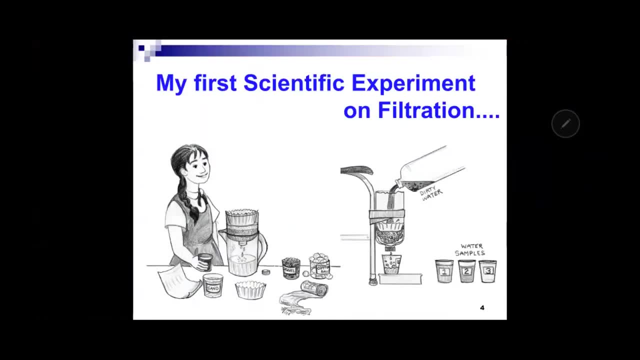 It's really very nice for me to talk about my experience on constructed wetlands for domestic wastewater in Turkey. Yes, it started in when I was in primary school. You know my first scientific experiment was on filtration and I was amazed to just prepare some dirty water and pure it. 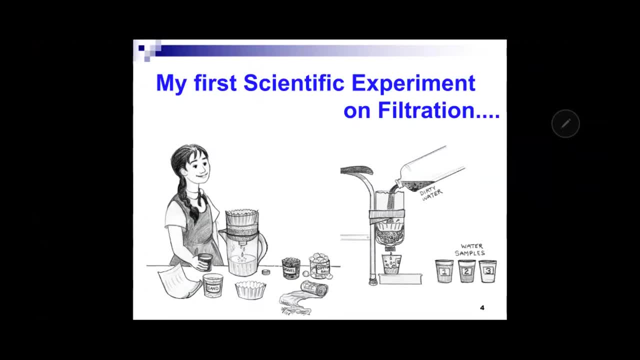 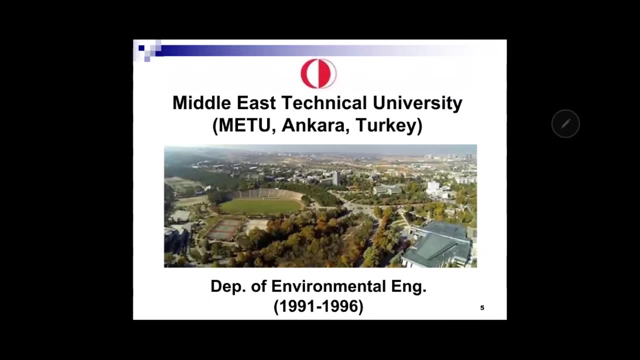 to level off. You know different layers of the substrates, you know so some sand, some gravel and so on, And this was giving me the inspiration to continue with environmental engineering in the future. So when I was studying in environmental engineering at Middle East Technical University in Ankara, usually the context 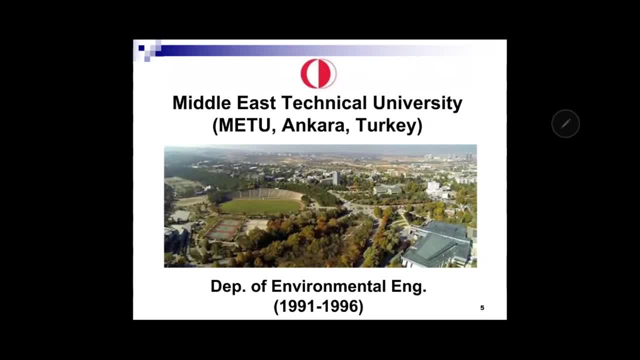 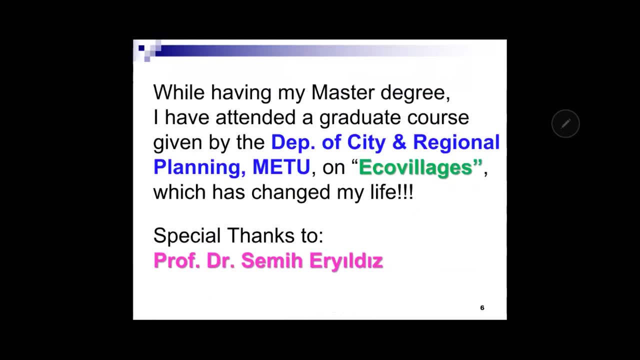 I mean so. the curriculum was based on conventional treatment systems. When I was graduated from this department, I continued again, So with the same department, but I was able to take some other courses, for example from the Department of City and Regional Planning. 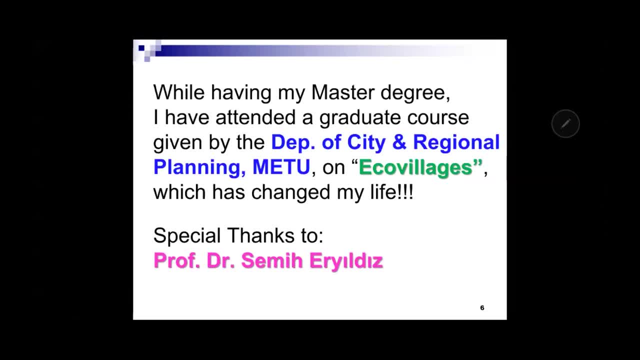 And then there was a course on ecovillages And within this course, Professor Dr Semih Aryildiz. he was mentioning about ecovillages And I was amazed again. So once, once, one more, because he was talking about the greywater treatment system. 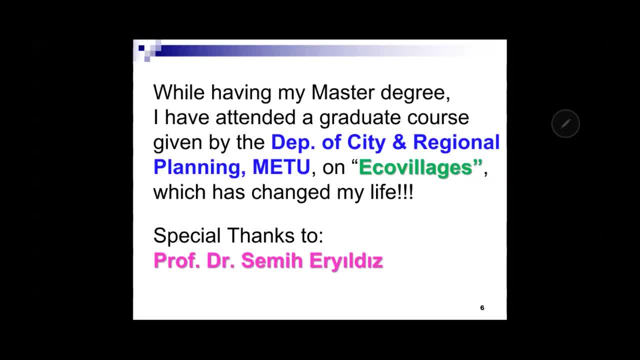 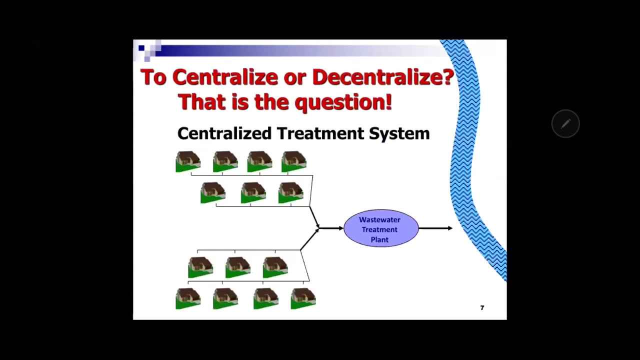 And composting toilets, wetlands and algae treatment, And it was at the time, called like living machines. OK, so we were dreaming really to have some applications also within our university campus. Therefore, I continued to work on this topic And he gave us this idea: to centralize or to 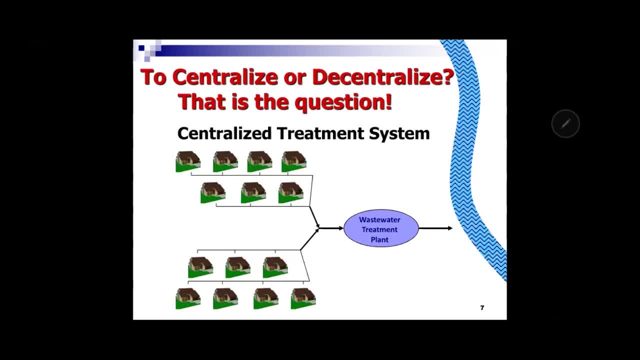 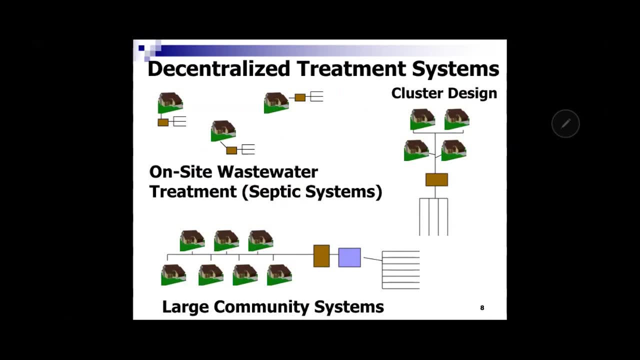 Decentralize? That was the question, And my, my idea was also going to have such kind of courses maybe, But at the time we didn't have such kind of courses also within our university. It was 1997.. And but then I was convincing one of my professors to have some studies on constructed wetlands. 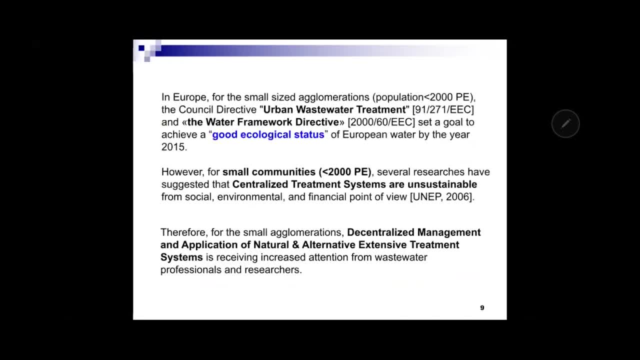 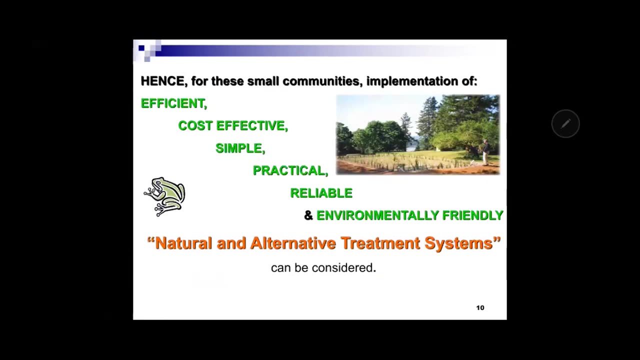 Why not to have a master thesis, for example, For constructed wetlands? And most of you? you were talking about the centralized treatment system, So I will not go to into the detail. The constructed wetlands for the small communities can be also a solution because they are efficient, cost effective, simple, practical, reliable and they're environmental friendly. 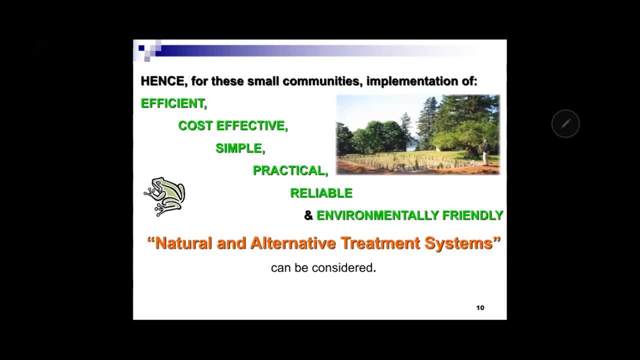 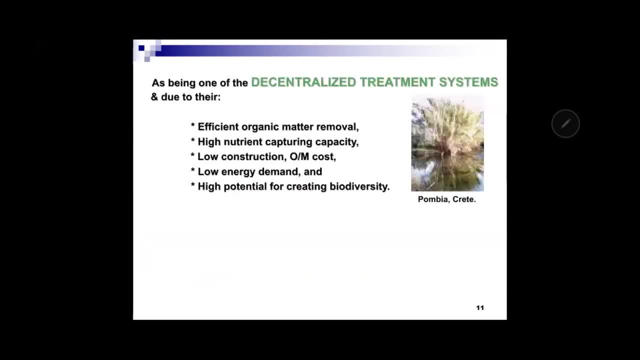 And these are also called as natural and alternative treatment systems- And it's my time, OK, so we were calling them as also ecovillages- And as being one of the decentralized treatment systems and due to their efficient organic matter removal, high nutrient capturing capacity, low construction operational maintenance costs, low energy demand and high potential for creating biodiversity. 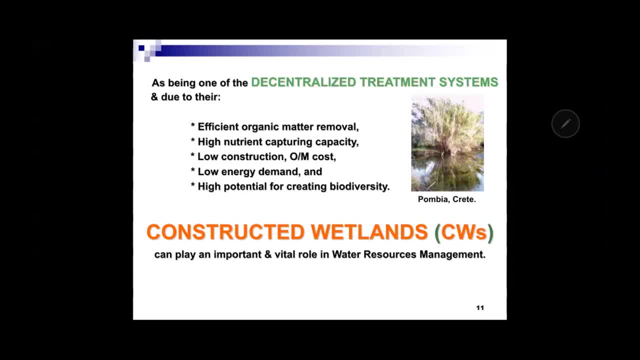 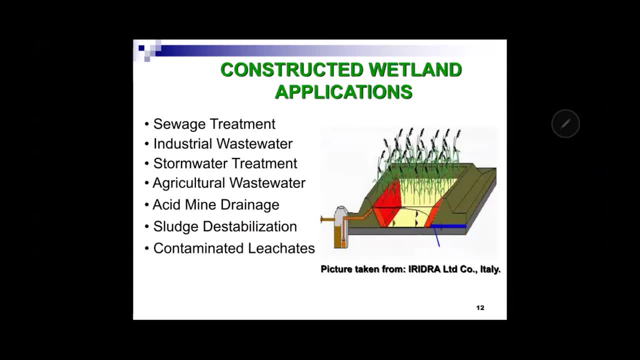 Constructed wetlands can play also an important and vital role in water resources management, especially for developing countries, And we can use the constructed wetlands- applications like this For sewage treatment, for industrial wastewater treatment, stormwater treatment, agricultural wastewater treatment, acid mine drainage, sludge destabilization and contaminated leachates. 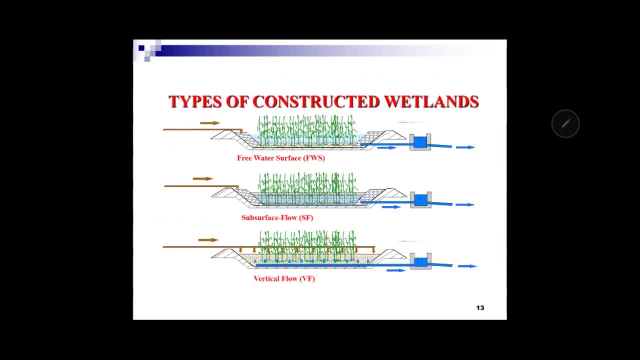 And there are types of constructed wetlands based on the flow of the water. For example, there are some free water, surface flow wetlands, subsurface flow, constructed wetlands and vertical flow wetlands, And there are, of course, a number of different types of constructed wetlands. 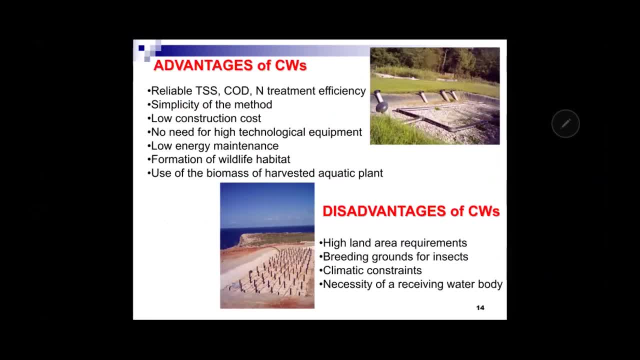 And there are of course, the advantages of the constructed wetlands and, of course, disadvantages. Reliable totally suspended solid COD and nitrogen treatment efficiency, the simplicity of the method, low construction costs, no need for high technological equipment, low energy maintenance, formation of wildlife habitat, use of the biomass of harvested aquatic plants are the advantages of constructed wetlands. 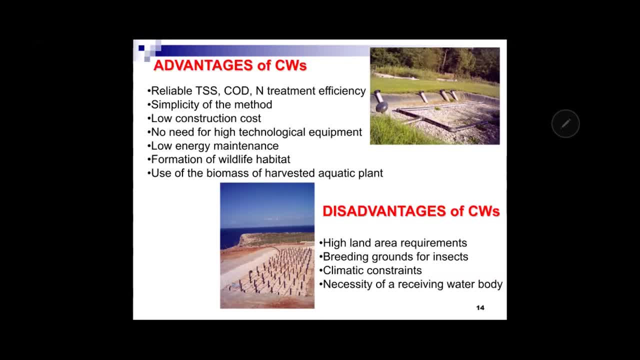 However, there are some disadvantages, as I said before- OK, said before, uh- for example, the highland area requirements for one person, for example. there it starts from a minimum one square meter and it can go up to 10 square meter, and sometimes they can be also the breeding grounds for insects and climatic constraints. 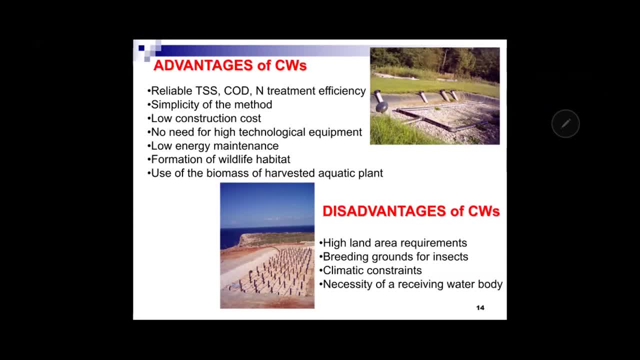 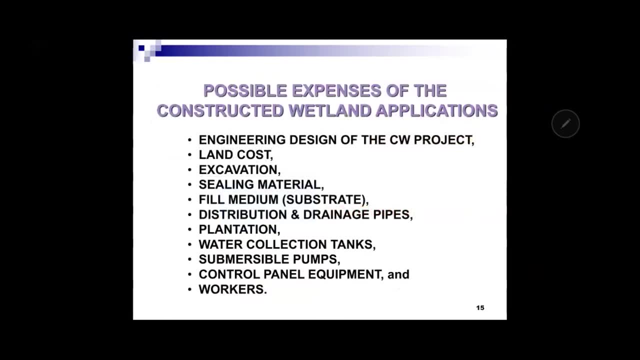 are also there necessity of a receiving water body. as for the treatment plants, this is also needed and there are some possible expenses of the constructed wetland applications, uh, the engineering design of the constructed wetland project, land cost, excavation, ceiling, material, field, medium, uh- we call it also as substrate- distribution and drainage pipes. 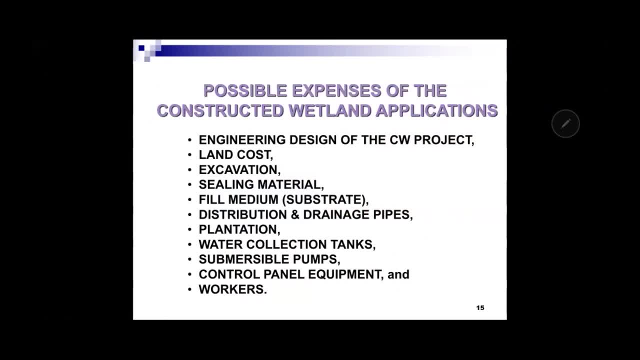 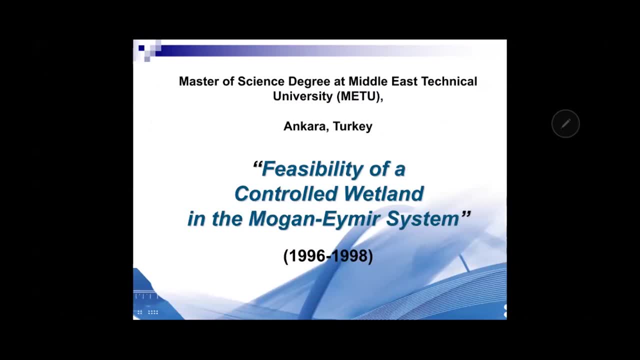 plantation, water collection tanks, submersible pumps, control panel equipment and the workers. of course you can also add the plantation, because i'm so for the plants, and so i decided really to work on such a study. uh, feasibility control: wetland in the mogan and aimer system. it was my master thesis. 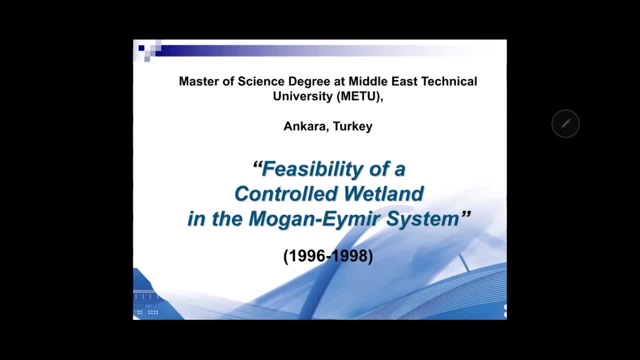 where i was uh simulating, when i was using a model for constructed wetlands and in order to remove the nitrogen and phosphorus efficiency. i mean so the nitrogen and phosphorus levels uh in a lake, in a eutrophicated lake. uh, i was suggesting to the government uh such a system. 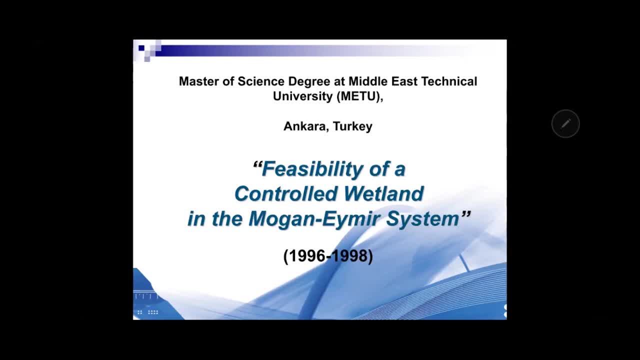 okay. so what will happen, for example, if we can uh just have some uh constructed wetlands uh on the top of the re of, on the top of the rivers, for example, which are feeding the mogan lake in ankara? so when i finished my master thesis, then 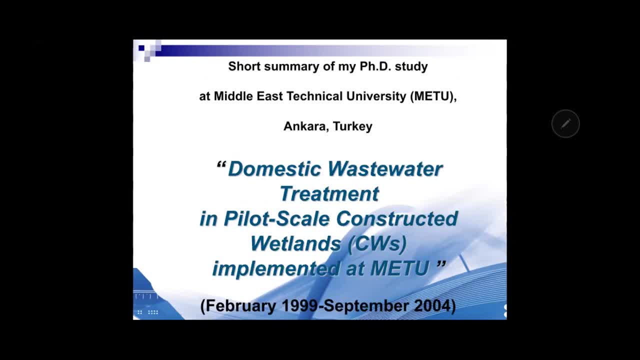 i was very, really, uh, feeling passion also with this constructed wetlands because, uh, very few people were working in turkey at that time also on the constructed wetlands. so my dream was, as i, as also in our master course, to have to apply really a pilot scale constructed wetlands. 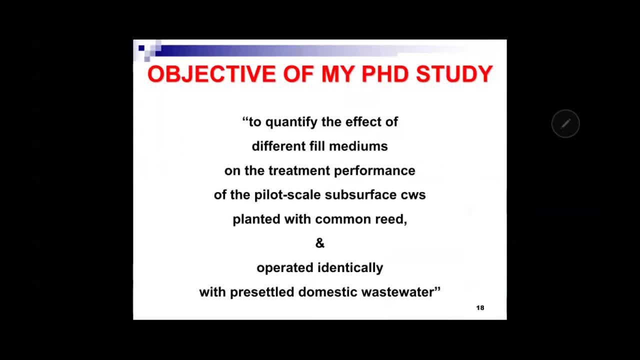 at the university campus. then again, i convinced two of the professors in my university, one from the biology department, one by from the environmental engineering department. by the way, i studied in biotechnology, uh, my phd uh, so uh. the study was to quantify the effects of different 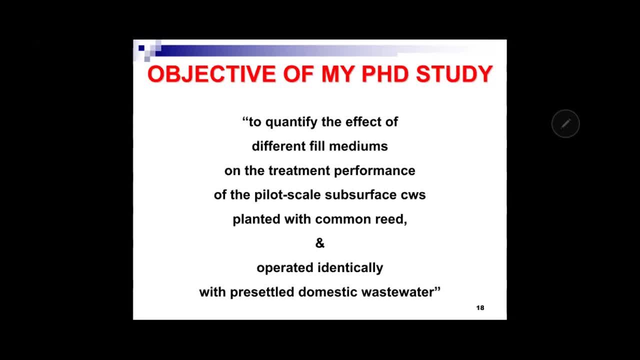 field mediums on the treatment performance of the pilot scale subsurface constructed wetlands which were planted with the common reed and operated identically with pre-settled domestic wastewater. i will just skip it very, very uh fast so there you can use in constructed wetlands uh. 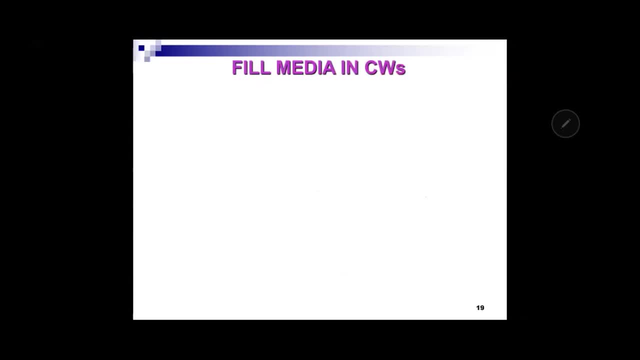 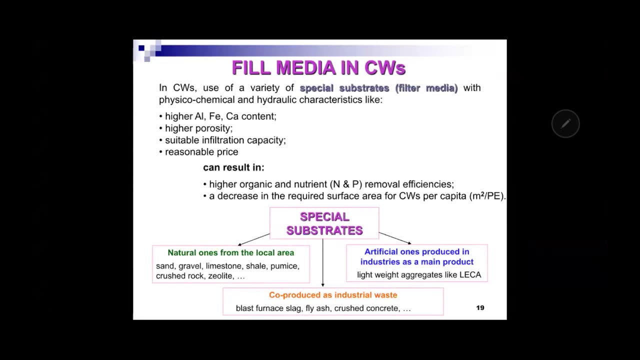 different kind of field media. there are some spatial substrates, for example. one of them is the nature ones and the other one is the artificial ones, and there are also some corporate produced, as in just industrial waste, um, and we are looking for higher aluminium, iron and calcium content, uh, higher porosity, suitable. 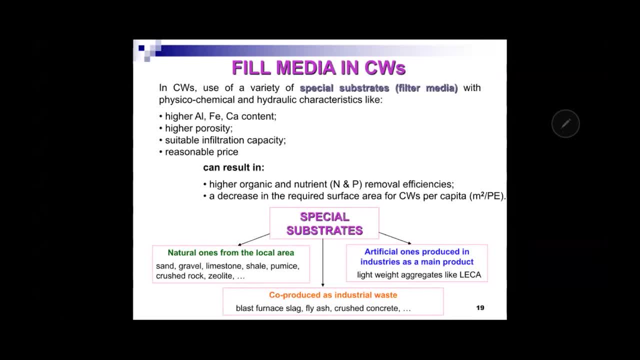 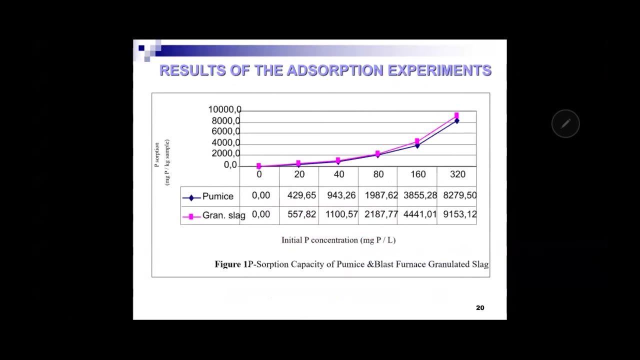 infiltration capacity and reasonable price so that we can have higher organic and nutrient removal efficiencies and a decrease in the required surface area for constructed wetlands per capita is needed. then i was just doing some batch scale experiments in order to compare the efficiencies, the absorption capacities of pumice and blast furnace related slack and this blast furnace related slack from. 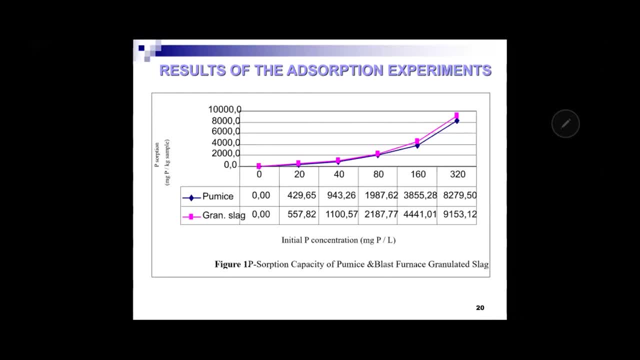 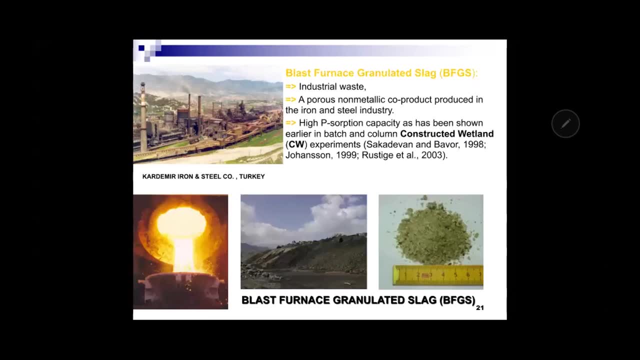 turkey from the black sea region. uh, it was just showing slightly differences and it was uh showing higher uh efficiencies. uh, i was contacting them and uh just asking for a sponsorship because uh, at the time, uh, the the people they were not thinking about uh such kind of projects, and so they they. 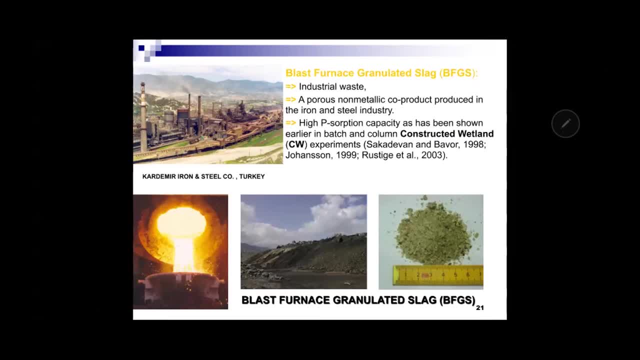 were uh just thinking, uh, it's, it's not their job to do this, but they were just thinking, uh, it's, it's kind of funny, you know. so what are you doing? So, eco-technology, therefore. I couldn't find any funds for my PhD research, but I didn't give up. 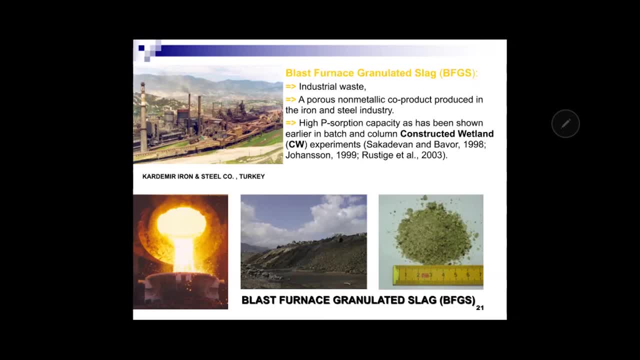 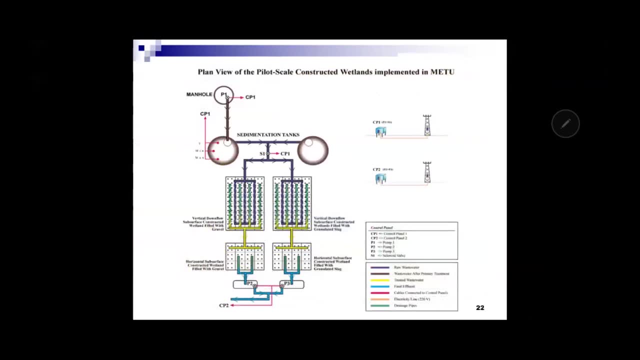 So I continued to contact the people. So, as an industrial waste, the blast furnace granite slag was used also within my system. Of course, we have lots of also experience and also funny memories, And some of them are not so funny memories. 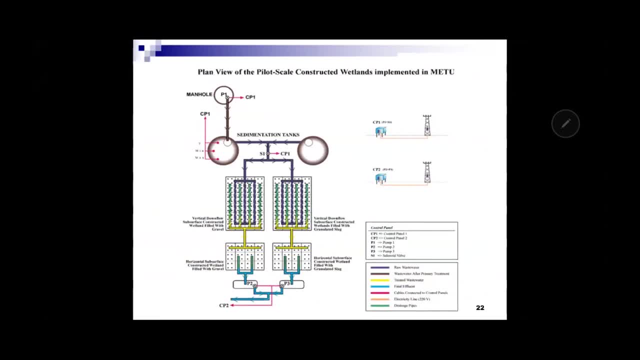 You know, I was going to the field and I was just looking for the manhole and we had to build something in the manhole so that we were able to just pump the wastewater, And I had to find also sedimentation tanks and excavate and blah, blah, blah yeah. 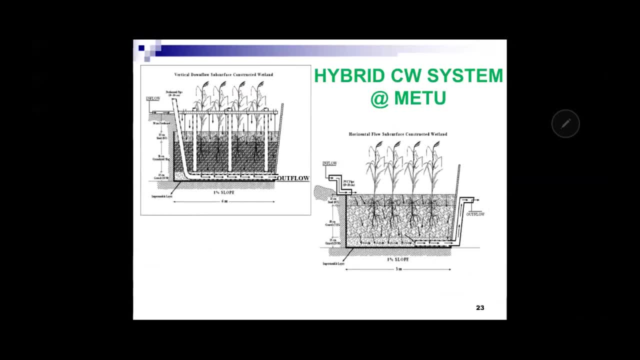 So here are some pictures and some cross sections where I was using mainly two of my own materials. These are two types of the constructed wetland systems, So the first one was the vertical flow one where you can apply the wastewater to the perforated pipes. 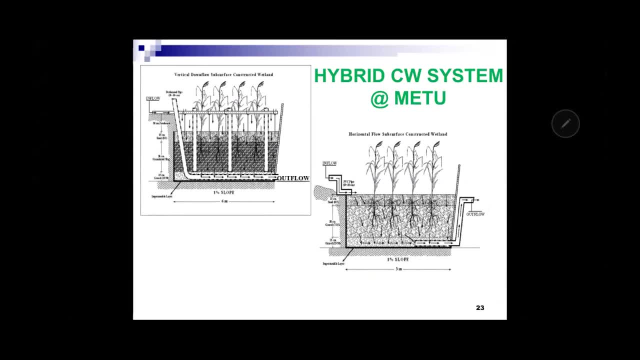 and you have different layers of the substrate And the second space basin- we can call them also as constructed wetlands beds, So it was horizontal flow. Both of them have different treatment ideas. For example, in the first one you can have the nitrification. 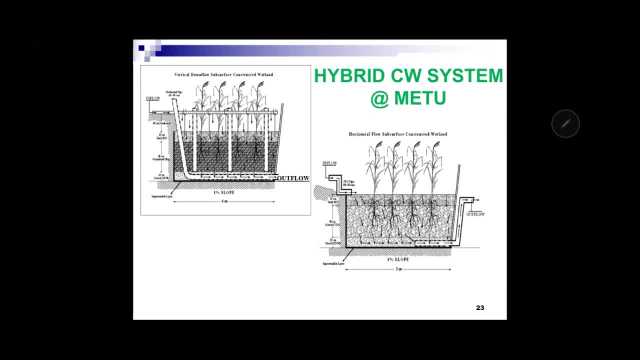 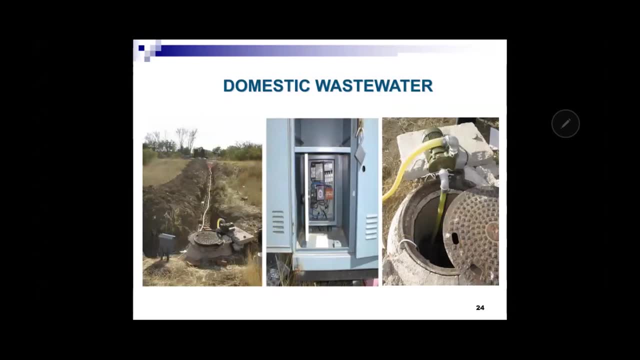 and this. in the second one, you can have the dentification, And here are some pictures from that application. Okay so, but, for example, what happened was the first pump. it was stolen by the gypsies, for example, from the field. 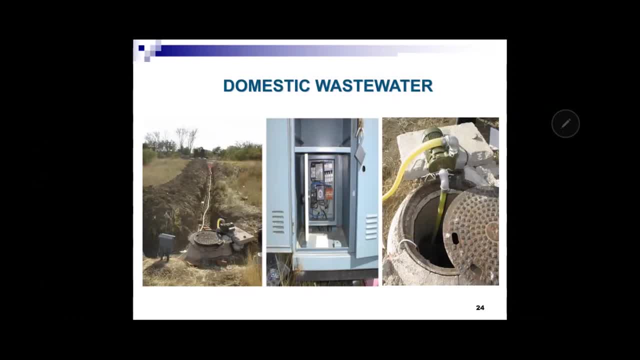 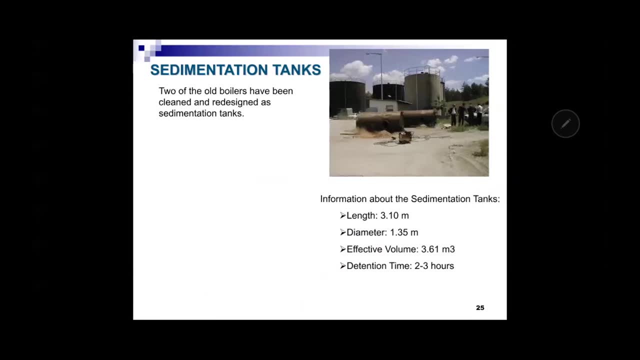 I was crying because it was difficult for me to buy the pump, but then afterwards I had to also find another sponsorship to find this pump And for the sedimentation tanks. I was lucky enough when I was going to the recycling activity area So I found two identical old boilers, you know. 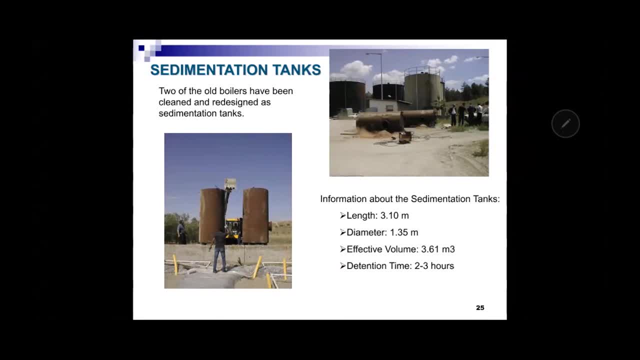 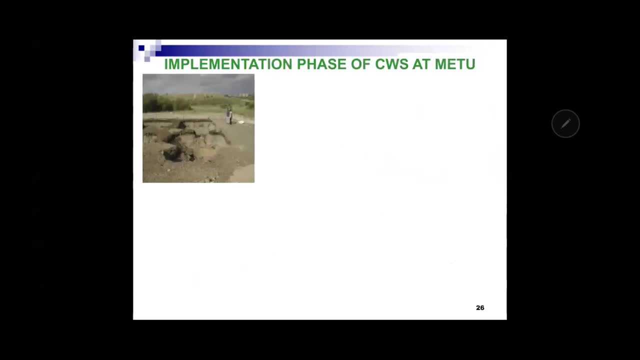 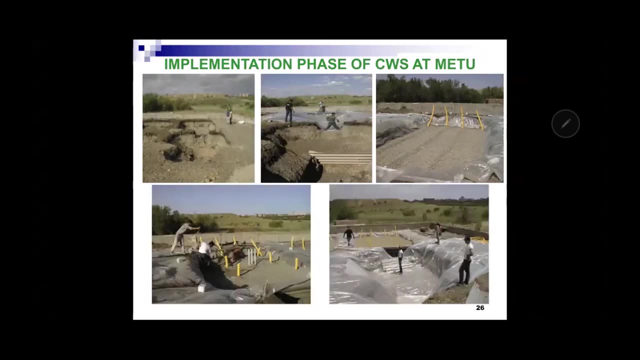 and we cleaned them and we redesigned them as sedimentation tanks, So we were able to put them also into the field. And of course I didn't have workers because I didn't have too much money for paying them. So, my dear friend, they helped me, you know. 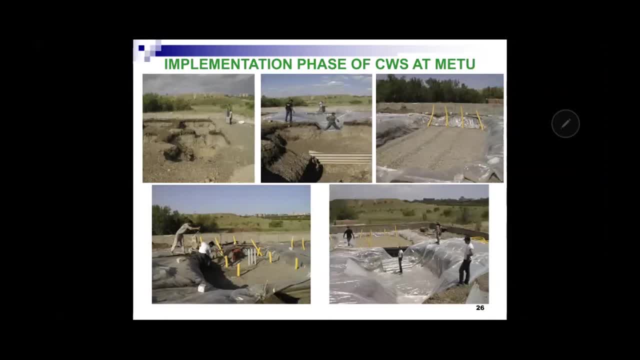 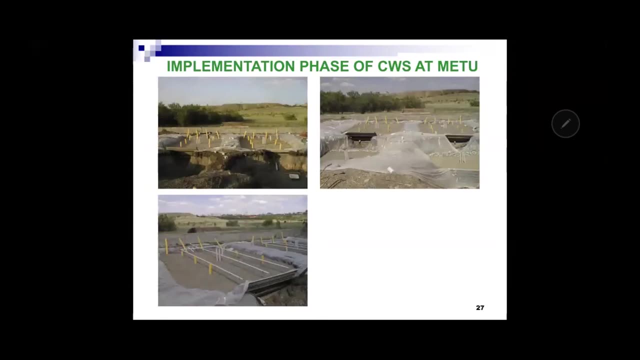 I was asking my assistant friends and the students from the student clubs of my university and we were applying this step-by-step Okay. so within the field. Okay, I'm just going very fast because I don't have very much time, So you see here some of the pictures. 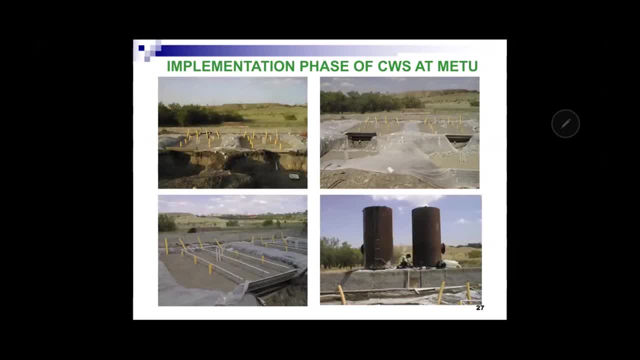 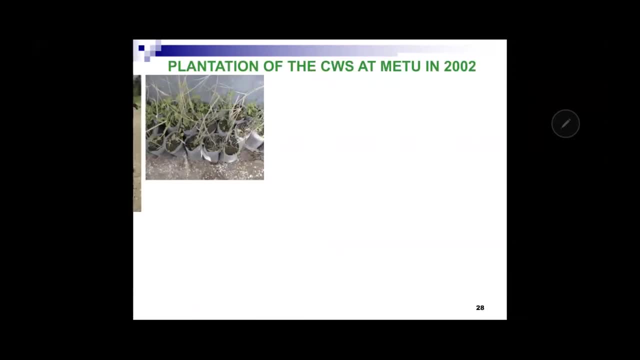 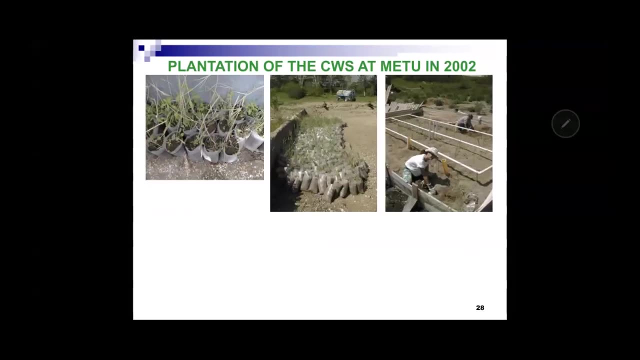 some application of the, also drainage pipes and so on, And I had to lose one year because of this replant. Everybody was saying, okay, it's so easy to plant them, Really, just resist, and so on, But I lost really one year because of the plantation. 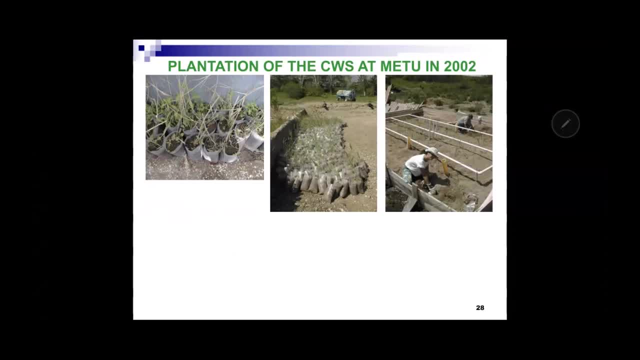 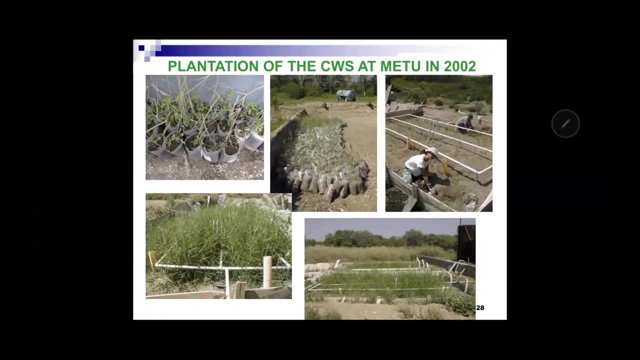 We were planting them and they didn't survive And afterwards I had to really tube them, you know. so, like the tree, baby trees, like the seedlings, and 1000 of them, we had to keep it also in the greenhouse at my university campus. 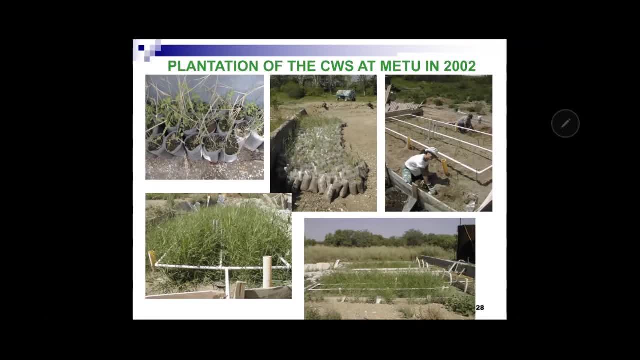 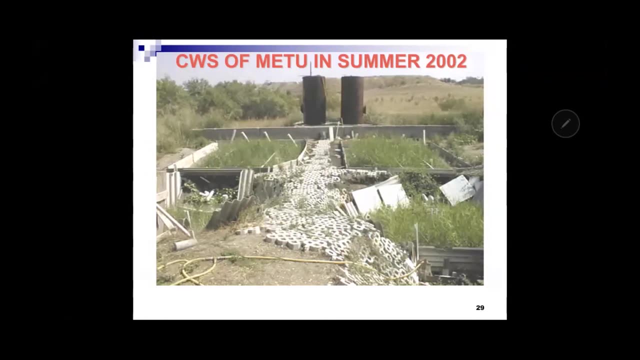 And, but afterwards again. so we were just planting them after a month, after applying the real domestic wastewater, they were happy, So I was able to continue with my research. I was very happy I was going there every day and just giving some wastewater. 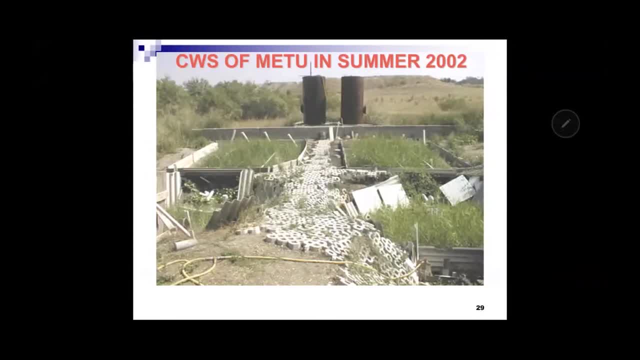 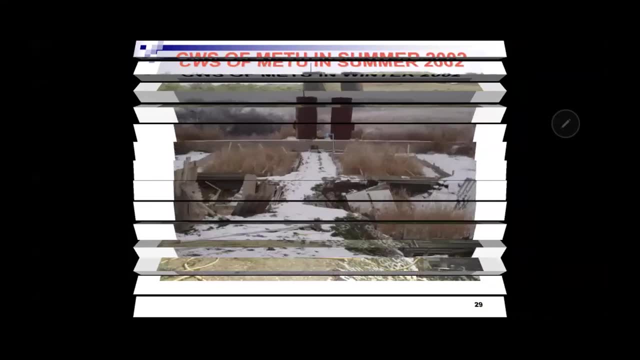 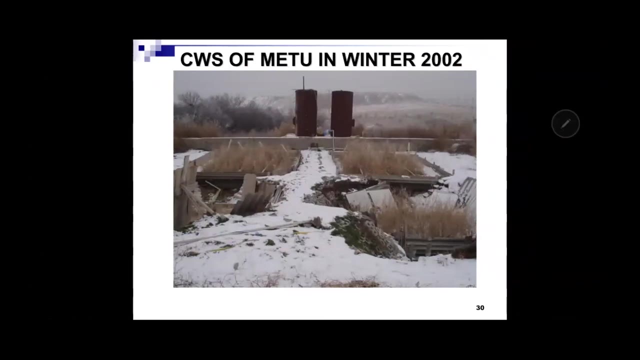 not some wastewater: three cubic meter for each of the beds. I was applying to domestic wastewater after the sedimentation It was because it was totally six cubic meter per day. So it was almost like a little treatment plant for 60 person And it is one of the pioneering studies also. 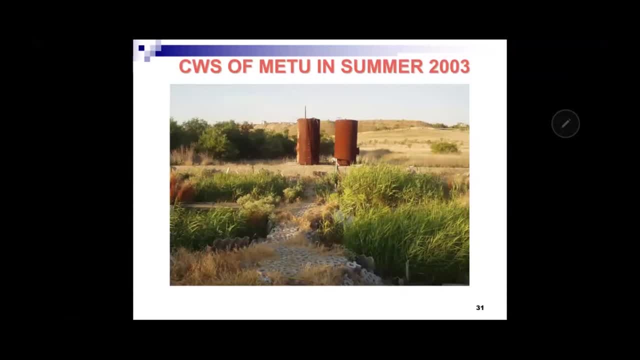 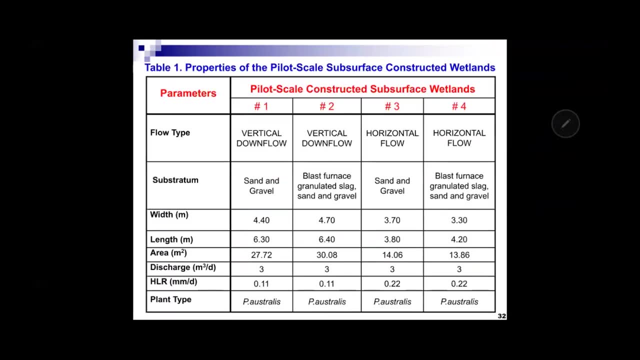 for constructed bedlands in Turkey. Okay, And after one year they were. the plants were really growing and I was applying the wastewater, for example, as a with a hydrocloding rate 0.11,, et cetera. 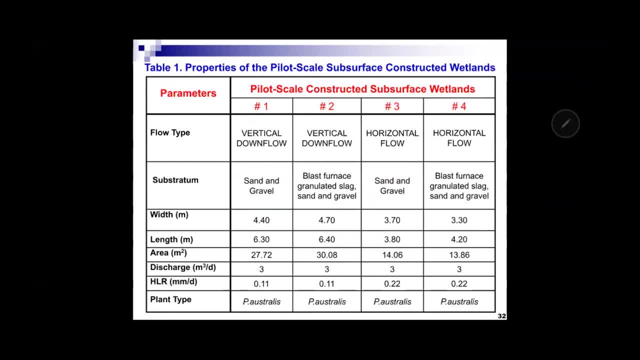 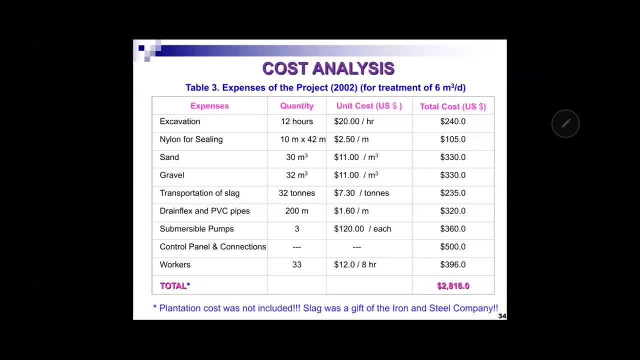 You can maybe have this presentation afterwards if you are interested. And then I was monitoring the constructed wetlands And here is a cost analysis. Of course there are lots of- well, there are lots- of volunteer work, But at that time in 2002,. 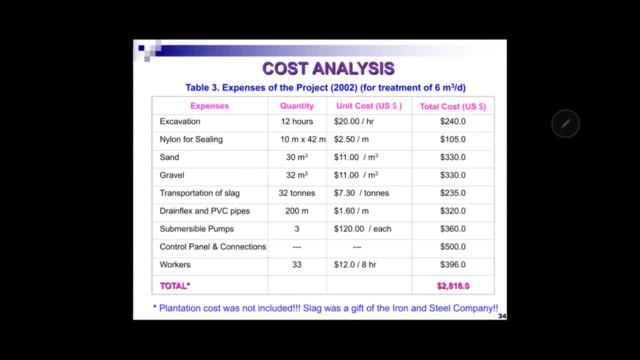 for treatment of totally six cubic meter per day, the domestic wastewater. it was around 3,000 euros, 3,000 US dollars. sorry, But the plantation cost, so the when you want to apply this, for example, in Europe. 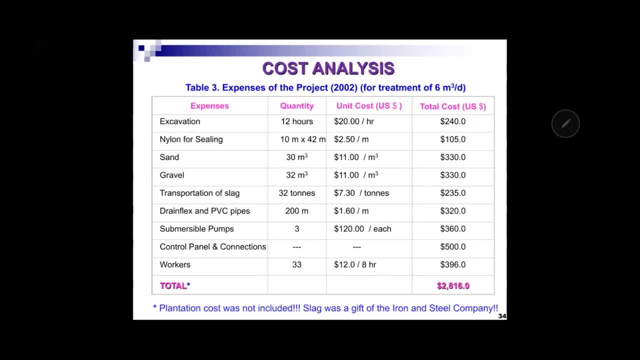 then you have to really pay money also for the plantation, because you need the baby plants And the slag was also it was a gift of the iron steel company. Therefore, maybe it is not the exact amount, but still you can have an idea. 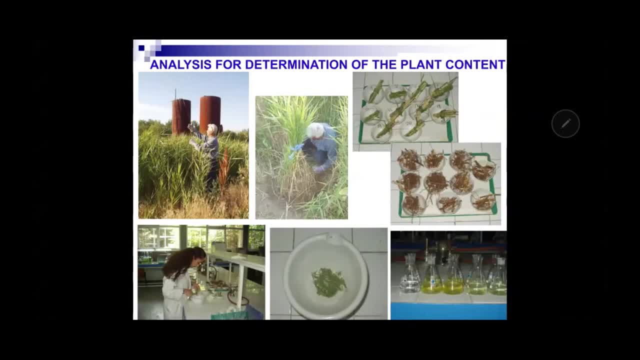 After finishing the monitoring study for one year so that I was able to observe it for four seasons. then this is also my lovely father. He was also helping me And we were removing from the constructed wetlands the plants and the stones. 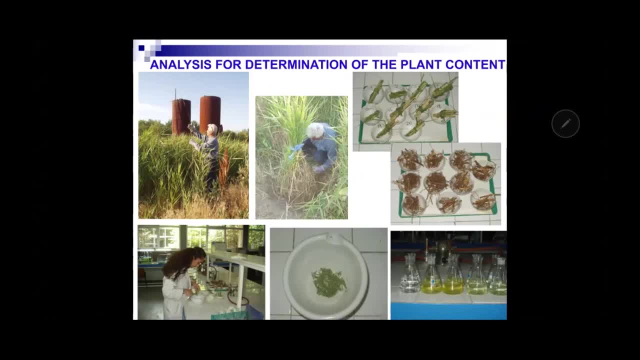 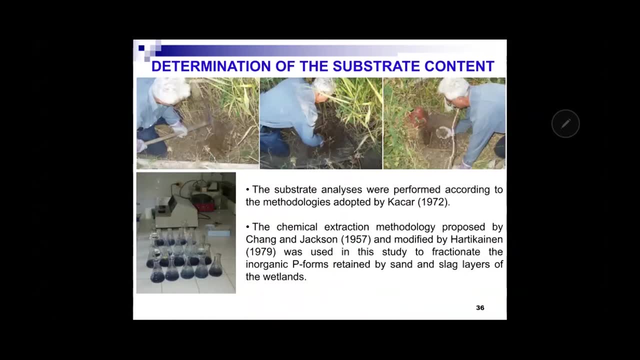 I'm sorry, I was carrying around with me. I was taking out all the alternative substrate so that I was able to have a mass balance study. so in order to understand what was the treatment effect of the plants and also the substrates on the treatment efficiency. 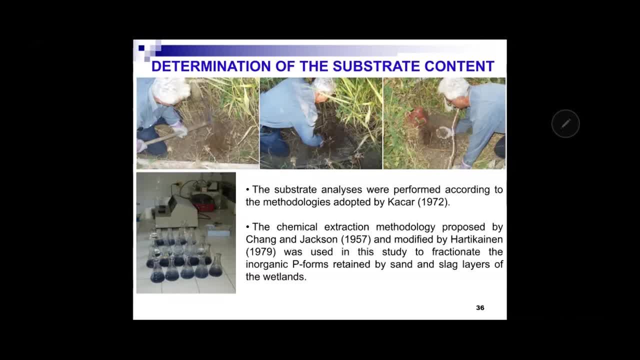 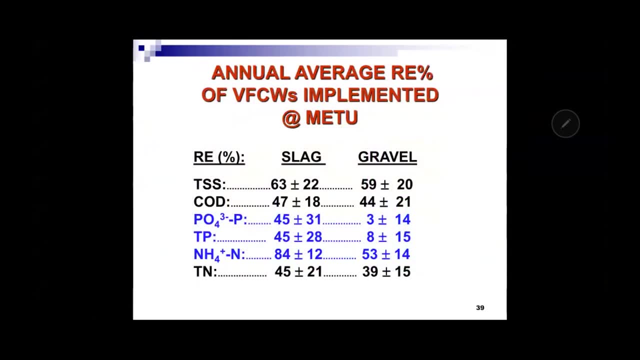 As far as I remember it was only 10%. the effect of the plants on total nitrogen and phosphorus removals. Okay, I'm just going very fast. result for the slag bed and for the gravel bed. okay, so, because I was comparing them. so for the 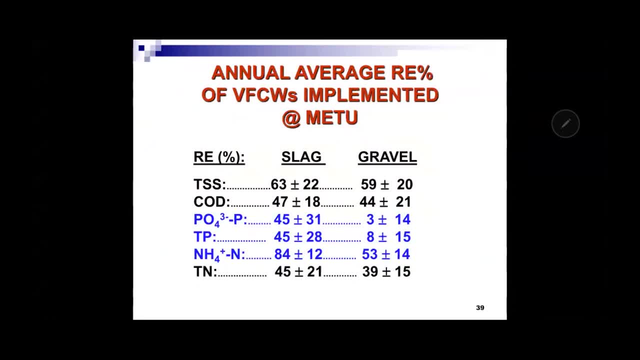 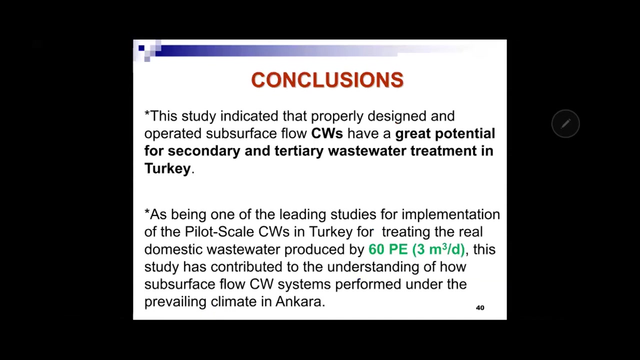 total suspended solids and for COD there was no statistical difference. you know so after just looking for one year. but for phosphate, phosphorus, total phosphorus and ammonium nitrogen, the slag content, of course, as I was expecting, much more efficient in comparison to gravel, and for the total nitrogen there was also no statistical difference. and as a conclusion, I 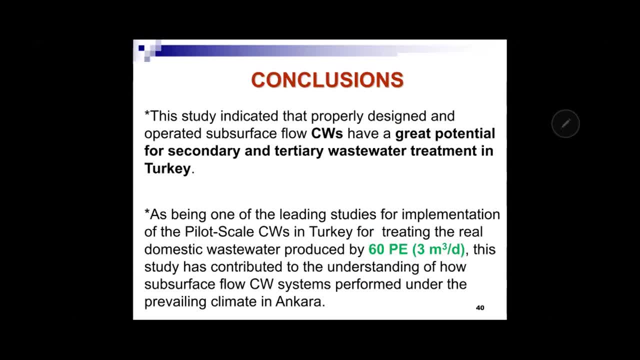 can say for this study. this study indicate indicated that the properly designed and operated subsurface flow constructed with wetlands have a great potential for secondary and tertiary wastewater treatment in Turkey and as being one of the leading studies for implementation of the pilot scale constructed wetlands in Turkey for treating the real domestic wastewater produced. 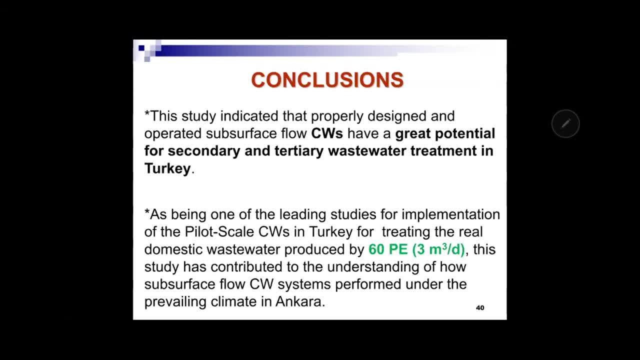 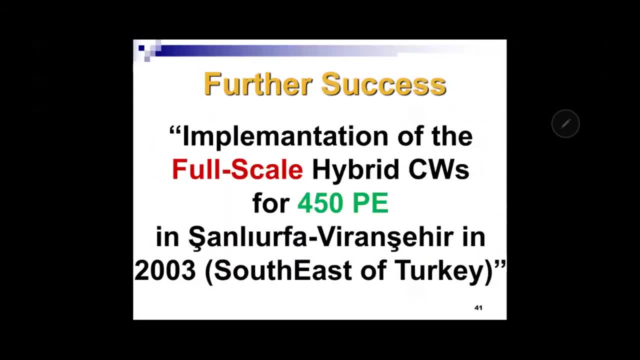 by 60 person. this study has contributed to the success of the study and I can say, for the first time, this study has contributed to the understanding of how subsurface flow constructed wetland systems performed under the prevailing climate. in Ankara and before finishing my PhD, again there was an opportunity to apply a real- I mean so a bigger, full-scale constructed wetlands. 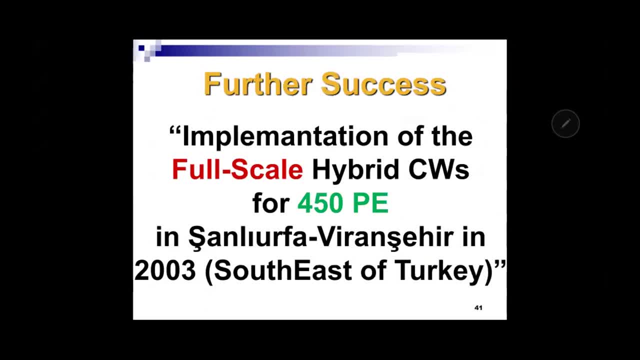 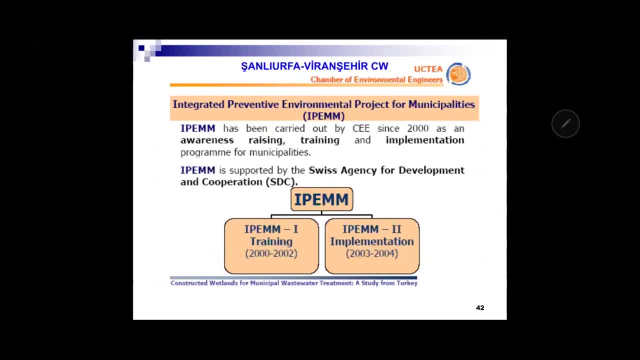 a hybrid constructed wetlands for a 450 person in Shannur, for Biranshehir, in 2003. it was because of a project okay, and the Swiss agency for development and cooperation was supporting the chamber of environmental engineers of Turkey, so we had the opportunity to apply it in the branching in this. 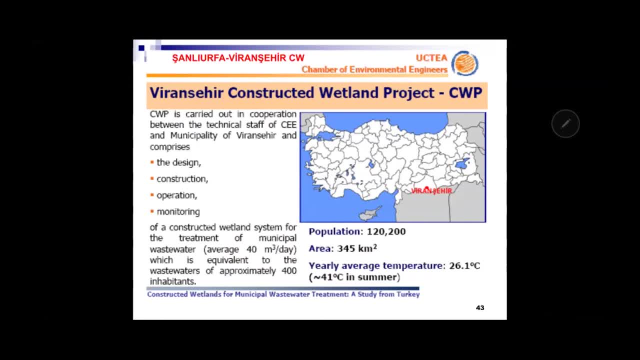 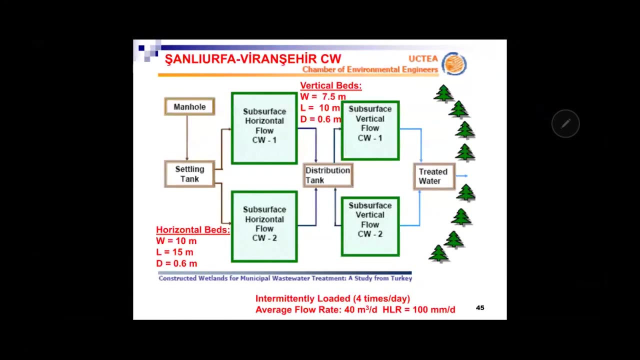 southeastern part of Turkey. okay, so I was able to design the constructed wetlands depending on my experience from my PhD. so again, we were monitoring and here is also the schedule and so the plan of the constructed wetlands. in this case I was using the subsurface horizontal flow constructed with us in the in the first treatment stage. of course, we had 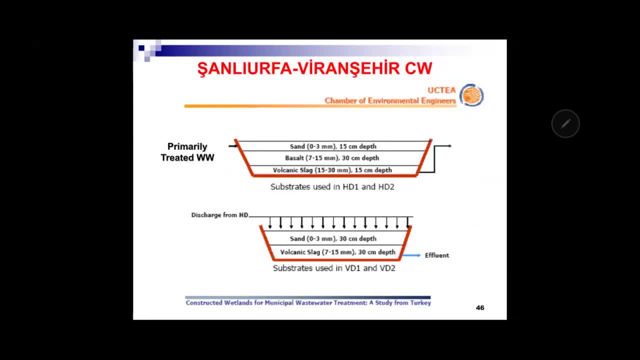 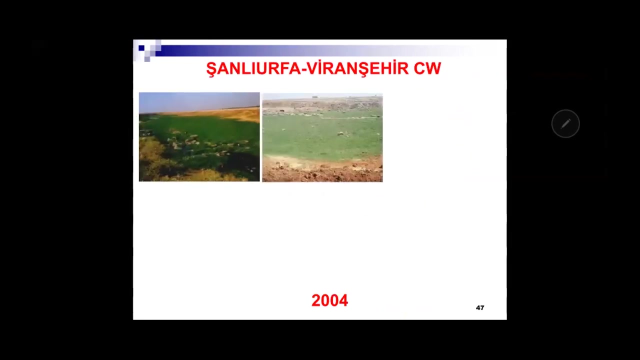 again settling tank and so on, and in that time so there was nearby a volcanic mountain and we had to reduce the volcanic slag and basalt from the, from the system. and then we, when we were applying it, first of all the area was an old municipal solid waste disposal area, okay so, and we had to. 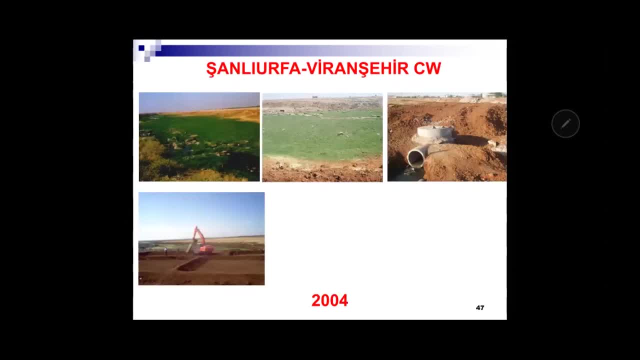 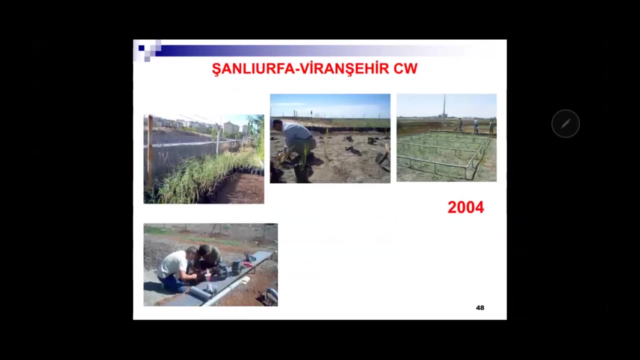 rehabilitate the system and afterwards we were applying also the- the clay impacted clay at the bottom and And again we were planning, but this time we didn't lose one year. So because we had the experience, so we planned again and there was the opening. 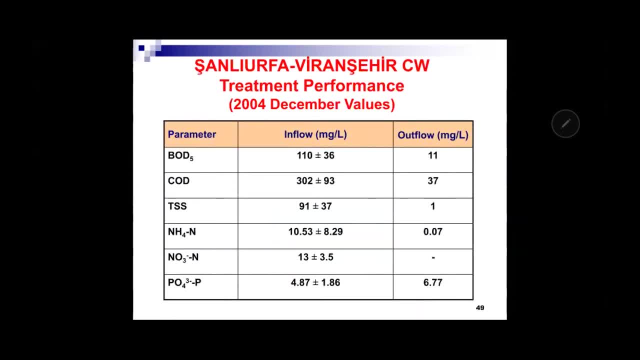 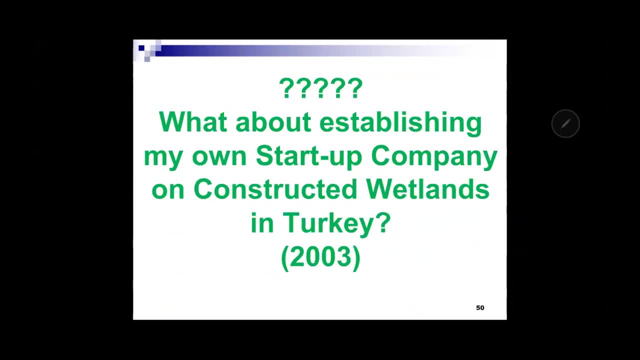 But unfortunately, afterwards there were some problems because of the maintenance and operation. This is also one of the important things we have to keep in mind. I guess- And after finishing my PhD, just before finishing my PhD- I was coming up with the idea. 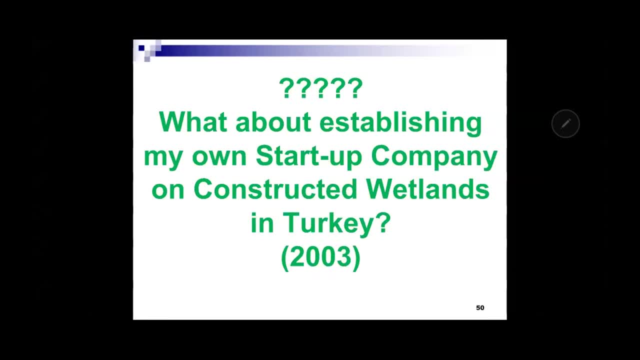 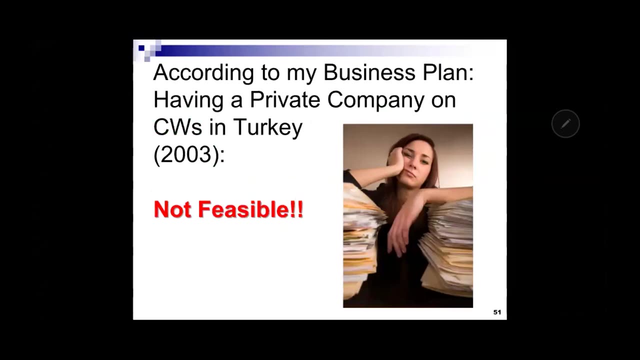 OK, what about establishing my own startup company on constructed wetlands in Turkey? It was in 2003.. And I just had some courses also on how to manage this. But according to my business plan, having a private company on constructed wetlands in Turkey in 2003, it was not feasible. 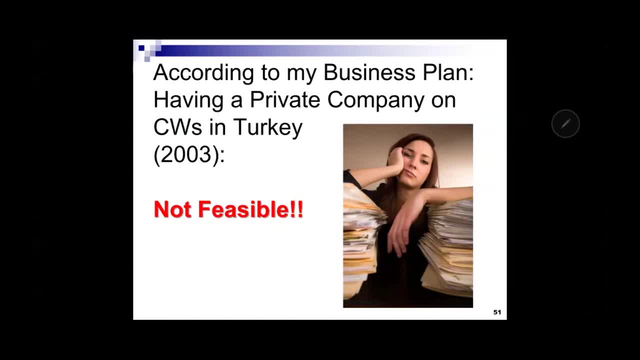 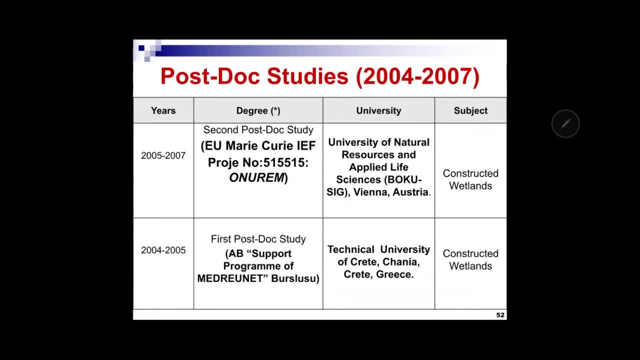 I was very upset, But then I was saying, OK, but I don't want to continue on working on constructed wetlands. So I just had two postdocs. One of them was in Chania in Crete, and the second one was in Vienna as a Marie Curie fellow for two years. 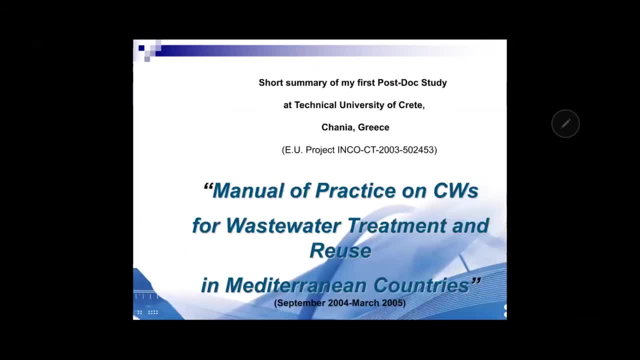 Both of them were on constructed wetlands. I just want to give just short information because I don't have too much time, I guess. So I prepared in Chania in six months a manual of practice on constructed wetlands for wastewater treatment and reuse in Mediterranean countries. 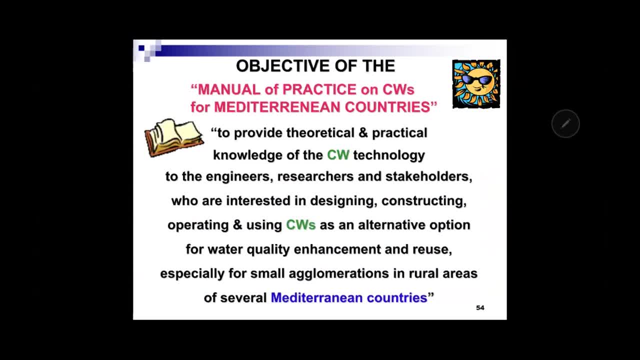 And the objective of the manual was to provide theoretical and theoretical information. I also had to provide practical knowledge of the constructed wetland technology to the engineers, researchers and stakeholders who are interested in designing, constructing, operating and using constructed wetlands as an alternative option for water quality enhancement and reuse, especially for small agglomerations in rural areas of several Mediterranean countries. 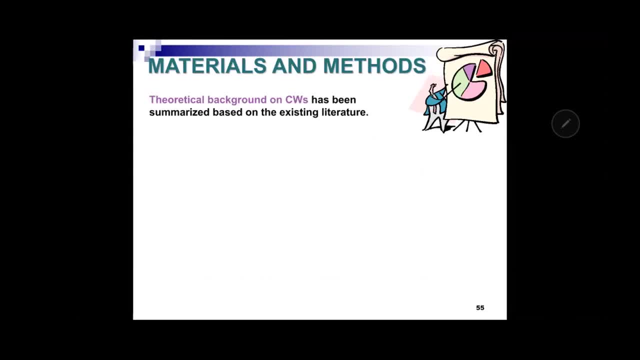 And the theoretical background on constructed wetlands has been summarized based on the existing literature And theoretical background on constructed wetlands has been summarized based on the existing literature, and constructed wetland case studies produced in some of the Mediterranean countries have been reviewed, summarized and evaluated. 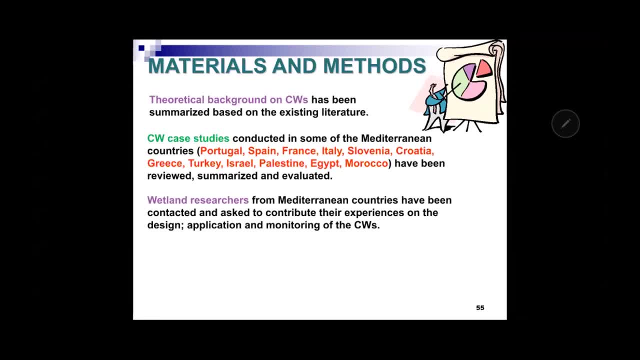 And wetland researchers from Mediterranean countries have been contacted and asked to contribute their experience on the design, application and monitoring of the constructed wetlands, And good practice guidelines have been developed for future constructed wetland applications in the Mediterranean countries. If you wish, you can also find this manual. 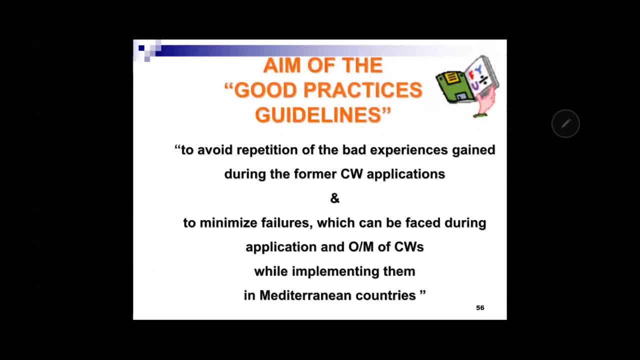 on the website of the ResearchGate OK, and the aim of the good practices guidelines was to avoid repetition of the bad experiences gained during the former constructed wetland applications and to minimize failures which can be faced during application and operation. maintenance of the constructed wetlands while implementing them. 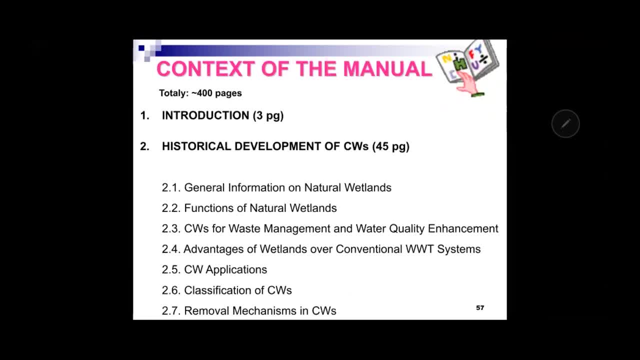 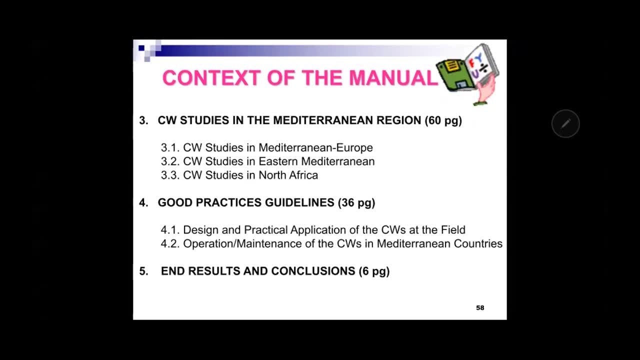 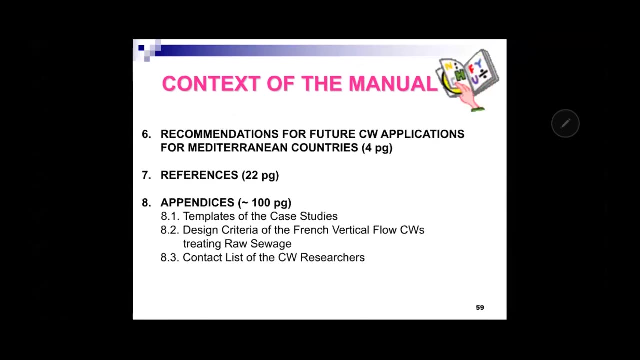 in Mediterranean countries. OK, so the manual was about 400 pages. It had the introduction, Historical development And some of the constructed wetland studies in the Mediterranean region, The good practices, guidelines And end results And some recommendations of course. 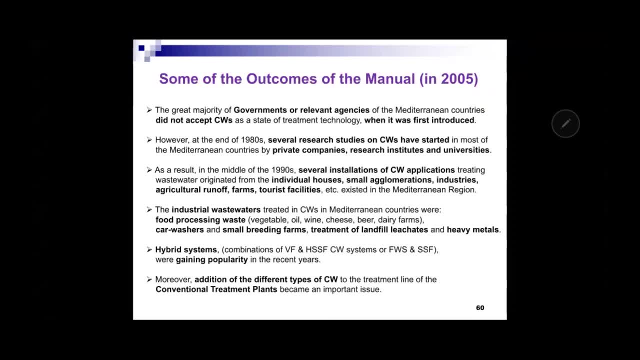 The references and appendices And some of the outcomes of the manual. It was the great majority of the governments or relevant agencies of the Mediterranean countries did not accept constructed wetlands as a state of the treatment technology When it was first introduced. However, at the end of the 1980s, 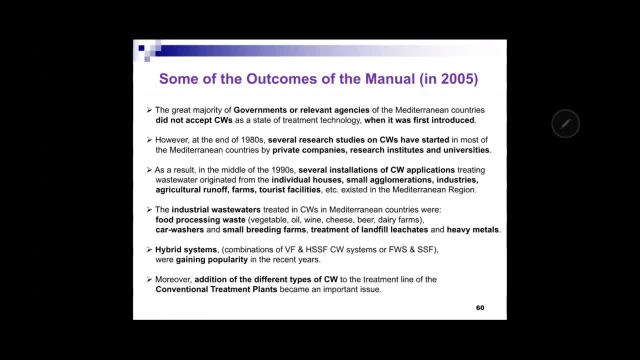 several research studies on constructed wetlands have started in most of the Mediterranean countries by private companies, research institutes and universities And, as a result, in the middle of the 1990s several installations of constructed wetland applications treating wastewater originated from the individual houses, small agglomerations. 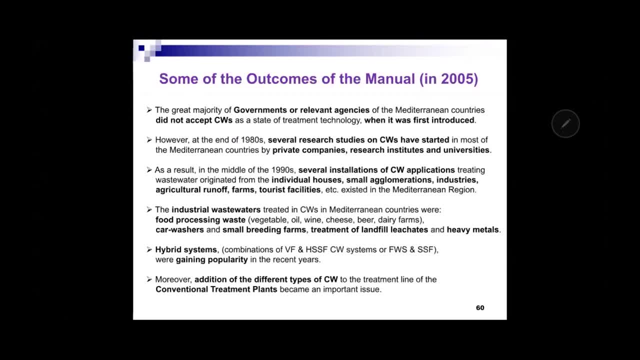 industries, agriculture, runoff farms, touristic facilities existed in the Mediterranean region, And the industrial wastewater treated in constructed wetlands in Mediterranean countries were also different, yes, And the hybrid systems were gaining popularity And, in addition to those, the different kinds. 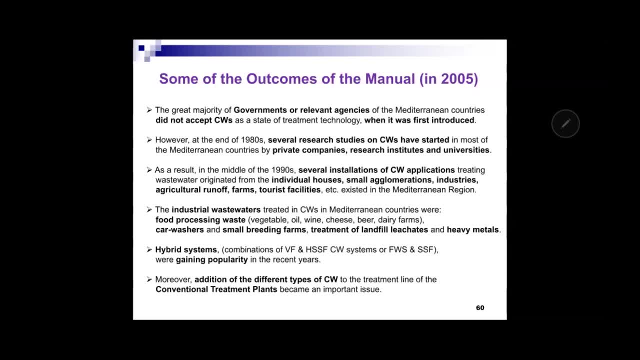 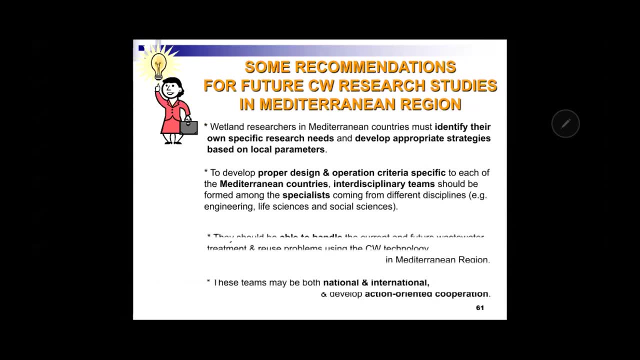 of constructed wetlands to the treatment line of the combination treatment plants become an important issue. OK, and maybe we can discuss it later. I don't know, But As most of the speakers were saying on decentralized treatment systems, the wetland researchers also in those countries. 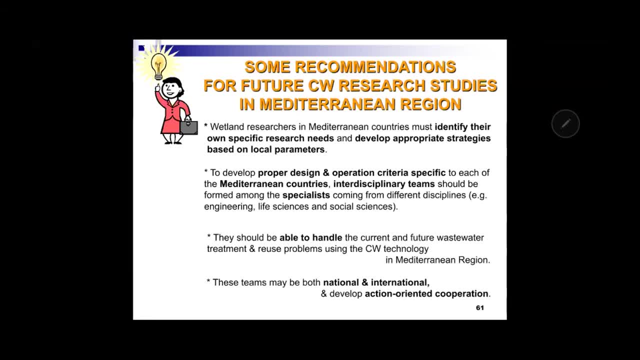 must identify their own specific research needs and develop appropriate strategies based on local parameters, And they have to develop proper design and operation criteria specific to each of the countries, And interdisciplinary teams should be formed among the specialists. OK, They should be able to handle the current and future wastewater. 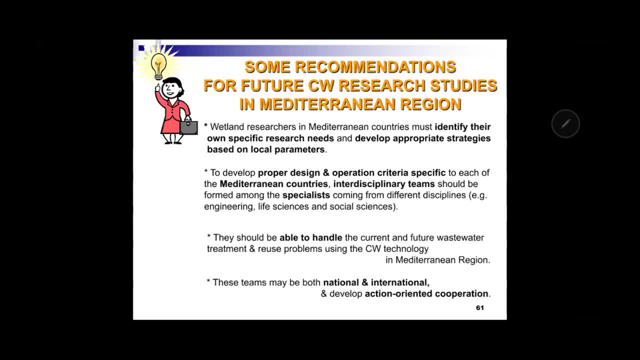 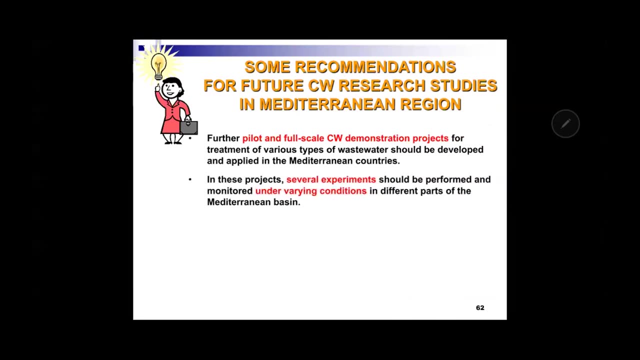 treatment and reuse problems using the constructed wetland technology, And the teams may be both national and international, And they have to develop action-oriented cooperation. I guess I don't have too much time, So maybe we can really discuss them also later on. 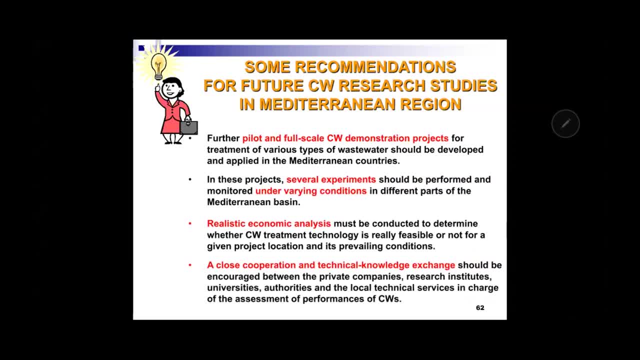 But what I was also suggesting is the pathological and the environmental aspects of the project are very important. The pilot and full-scale constructed wetland demonstration projects are very important, also in the region, And you have to also continue with several experiments under varying real conditions. 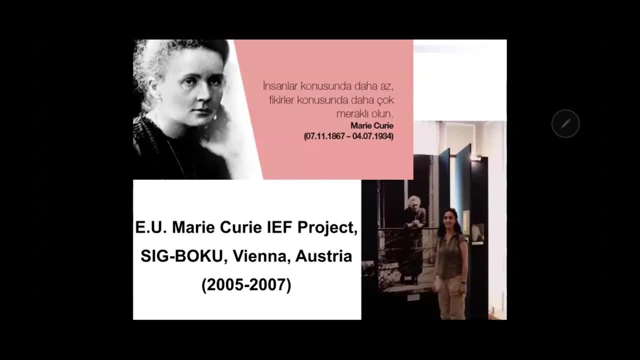 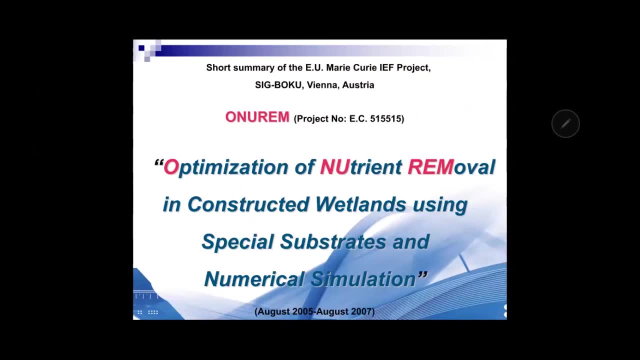 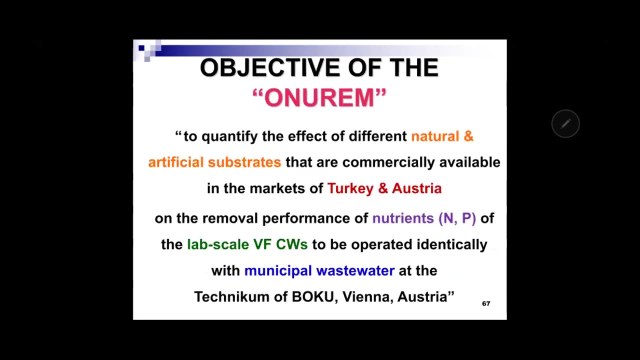 OK. so And last I want to say I continued in Vienna with this study: optimization- It was a European Union project also- Optimization of nutrients removal in constructed wetlands using spatial substrates and numerical solutions. I don't want to say 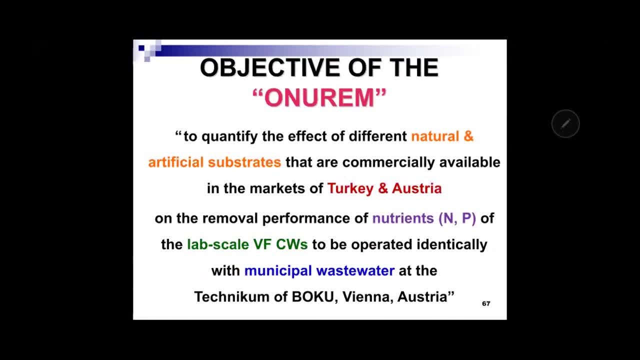 OK, so to end, the objective of the on-ramp was to quantify the effect of different natural and artificial substrates that are commercially available in the markets of Turkey and Austria on the removal performance of nutrients of the large-scale vertical flow of constructed wetlands to be operated identically. 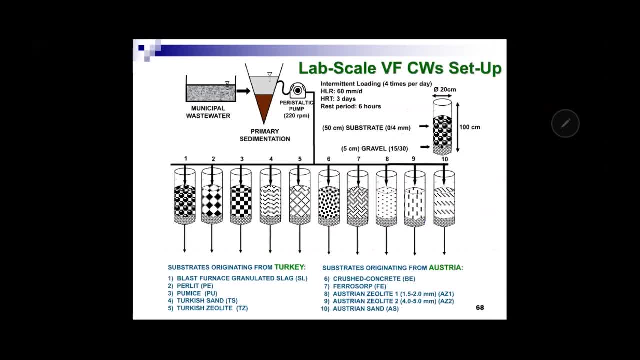 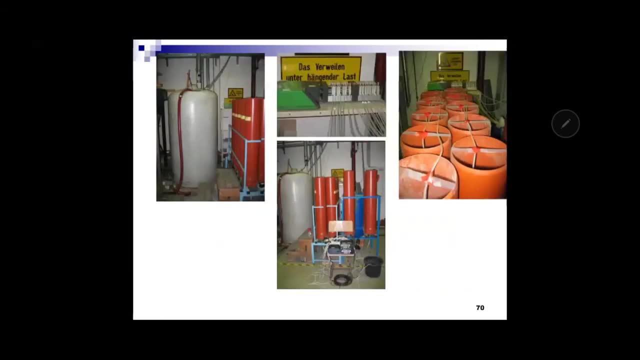 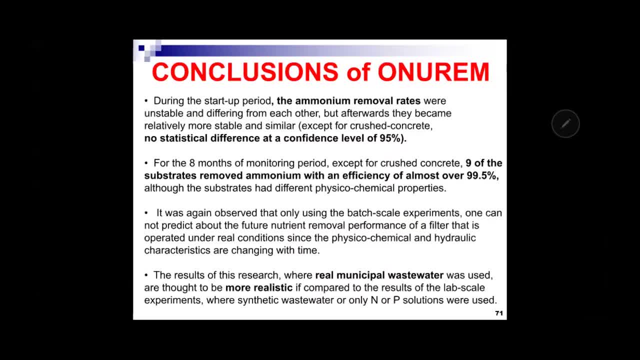 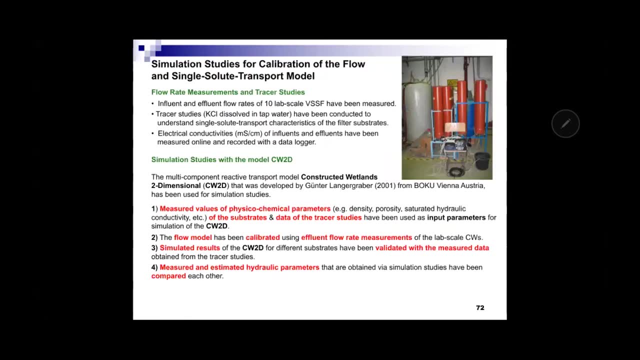 OK, so this was also from the laboratory And this study was also showing us working with real municipal wastewater is very important And also most of the substrates. they were also showing a higher So the and we put also those kind of results. 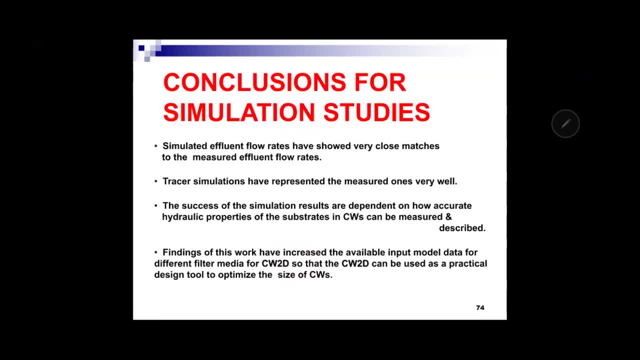 into the multi-component reactive transport model constructed wetlands, two-dimensional. It was developed by from Boku Vienna And we used them also for simulations And the results of that work have increased available input model data for different filter media for constructed wetlands. 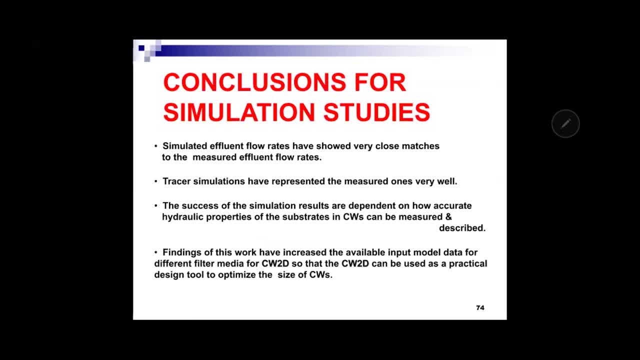 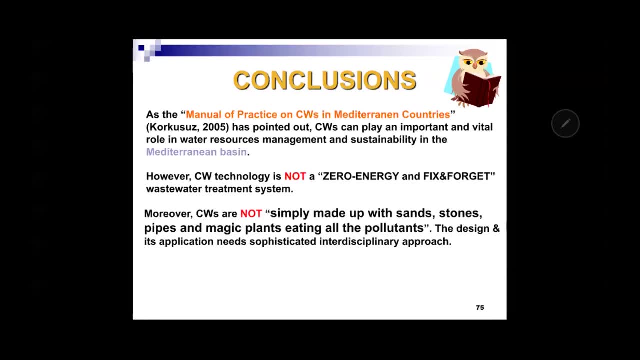 so that the constructed wetlands two-dimensional model can be used as a practical design tool to optimize the size of the constructed wetlands. OK, this is my last slide. It was a bit fast, but, as conclusion, constructed wetlands can really play a very important role. 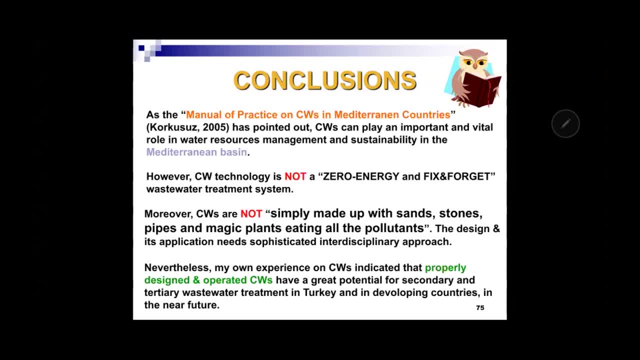 in water resources management and sustainability in our region. However, constructed wetland technology is also not a zero energy and fix and forget wastewater treatment system. Moreover, constructed wetlands are not simply made up with stands, stones, pipes and magic plants eating all the pollutants. The design: 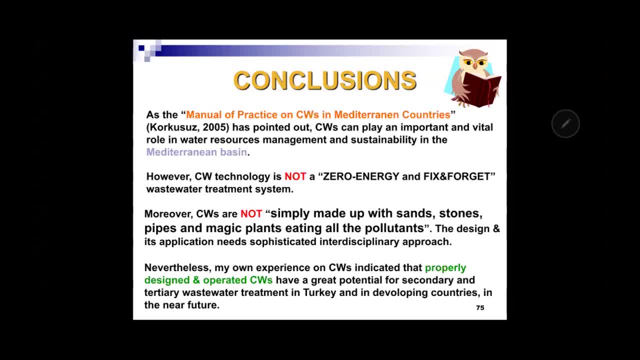 and its application needs sophisticated and interdisciplinary approach. Nevertheless, my own experience on constructed wetlands in Turkey indicated that properly designed and operated constructed wetlands really have great potential for secondary and tertiary wastewater treatment in Turkey and in developing countries in the near future, if, of course, the legislation allows. 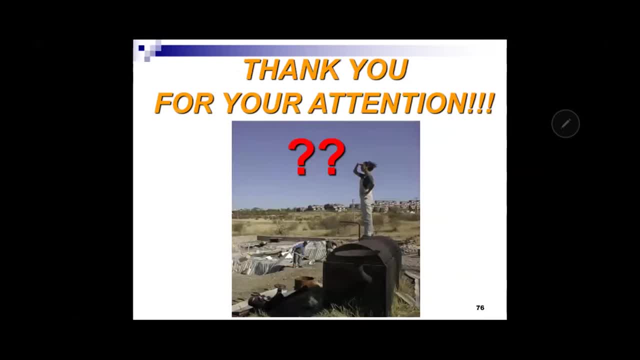 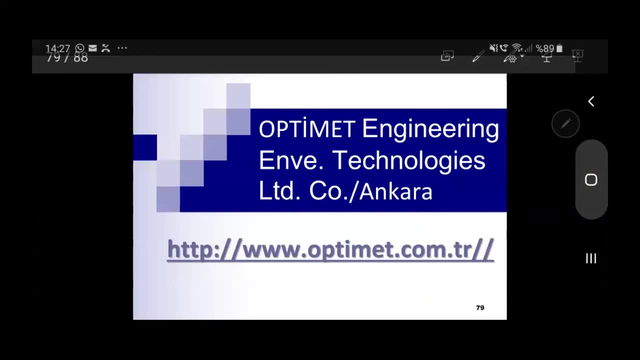 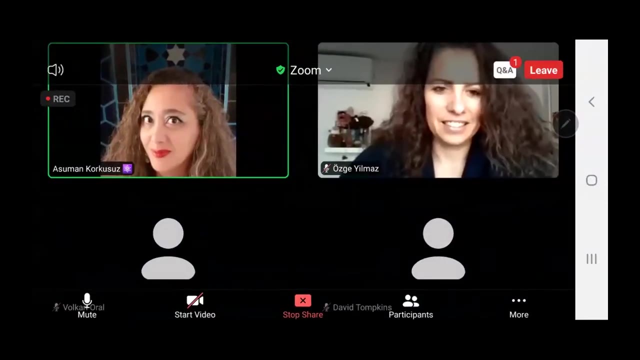 Okay, thank you so much for your attention And if you have any questions, I will be pleased to just listen to your comments and questions. I am struggling. Okay, Yes, great, Yes, Aslan, thank you very much for your presentation. 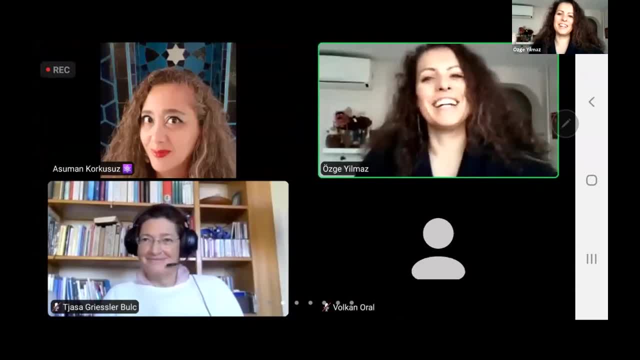 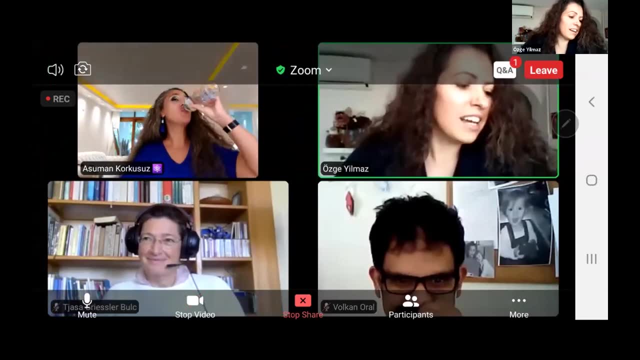 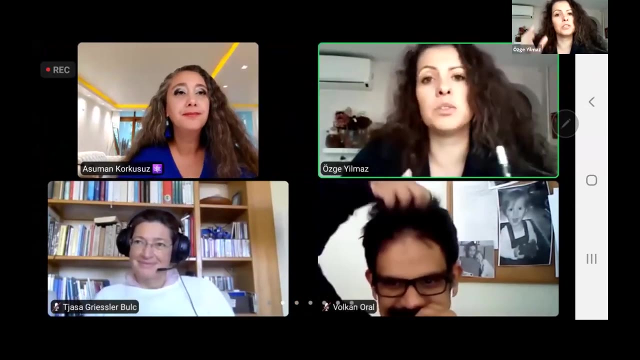 Obviously you have done so much, It's really hard to fit in into 15 minutes. That's quite understandable. Thank you very much. I have a couple of questions in my mind about maintenance of the wetlands, but I think we can leave it to later. I just want to say using blast furnace. 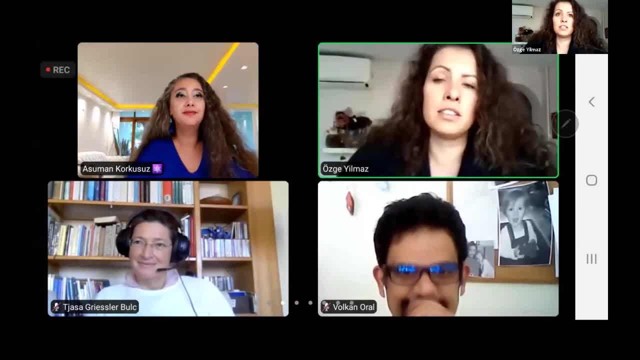 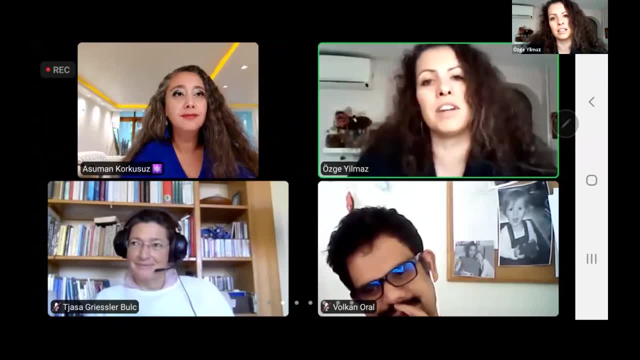 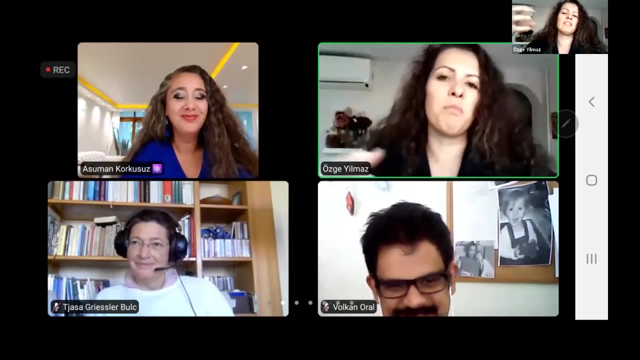 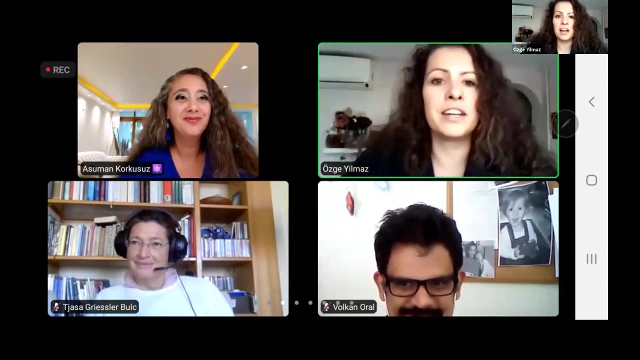 granulated slag or any type of industrial- let's say waste or resource- byproduct in such a system. I think it's a very nice example of a circular economy model that we can, you know, combine industrial waste management into nature-based solutions like this. I think that was very impressive from my side. If you have any, 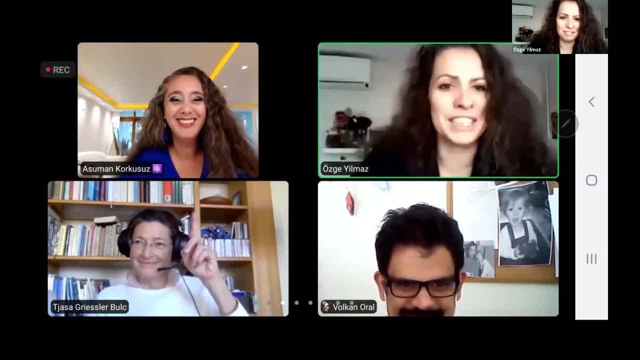 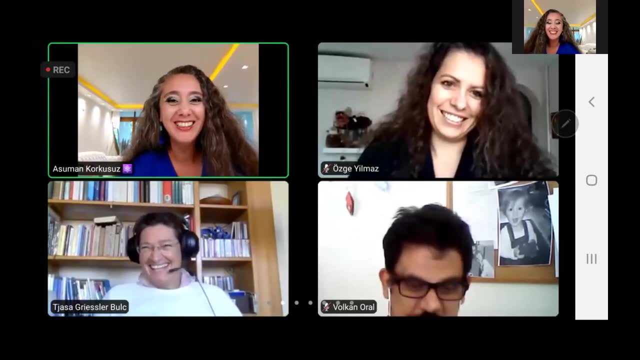 questions. please just go ahead raise your, please. Yes, Hello Aslan. Hi Tiajah, Nice, to see you, my old friend. Yes, So my question would be: you gather so much knowledge and knowledge and knowledge about the? 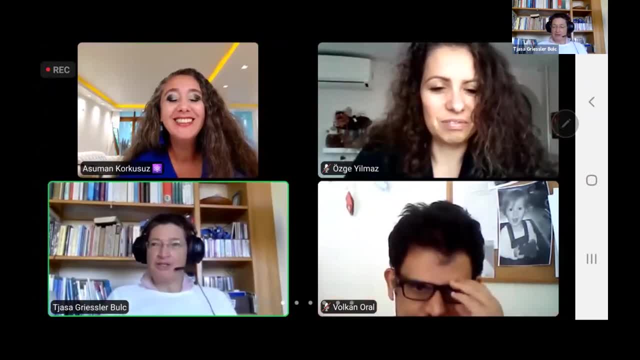 environment. How do you see the future of the environment? and how do you see the future of the environment? I mean, we have so much knowledge, so much experiences, so much enthusiasm, And what is the status quo today in Turkey? How you would. 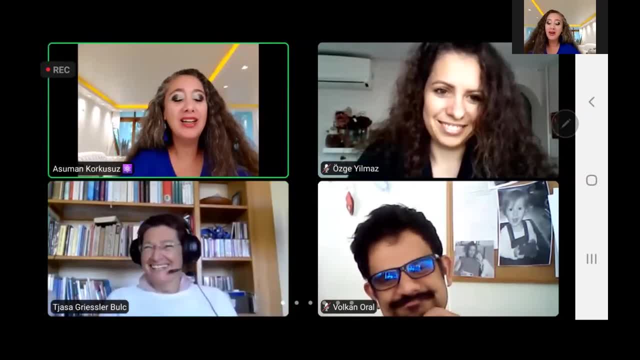 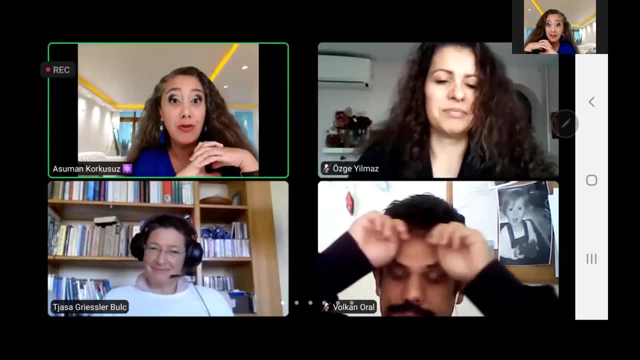 comment on that, Sorry. You know what, after coming back from Vienna I was really feeling very much so energy-critical and I have been to Minister of Environment and I was saying please can we just write to legislation on this topic? And they were saying, OK, 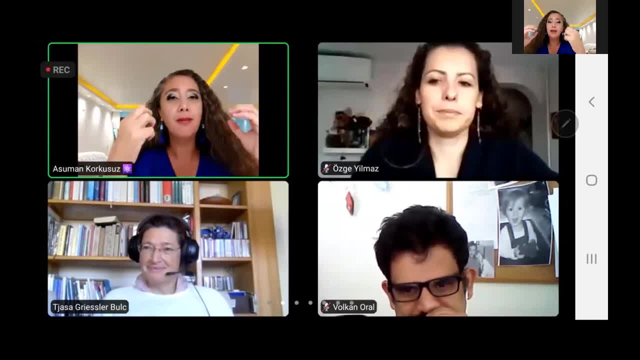 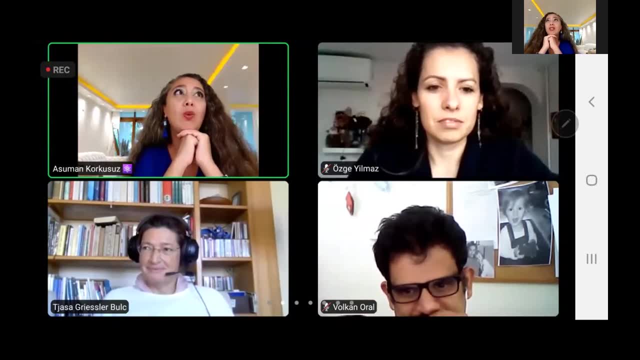 just come and just give us also some lectures, And I was giving some lectures and some recommendations. you know we will use this to help some other people, All right, But I am not gonna left. But anyway, and some recommendations and so on, but afterwards they you know what. so when you have to build your 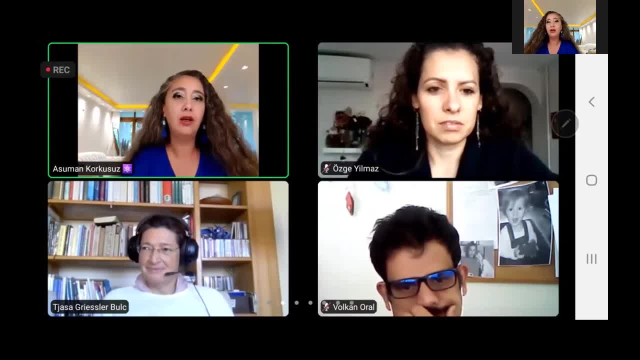 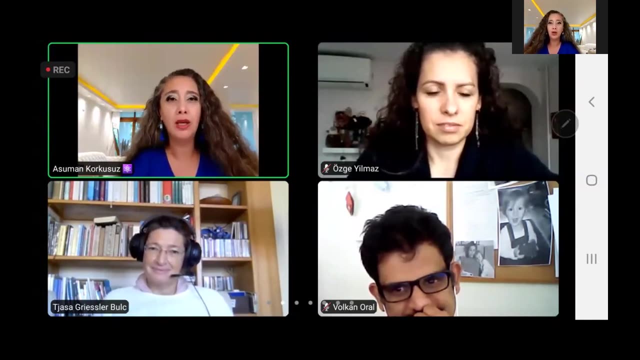 wastewater treatment plants in the cities of Turkey by the governments, I mean by the municipalities. so you, you don't have too much chance also to build your own treatment plant, because the legislation is in in a way not allowing you, you know, and because I saw that it is not feasible. 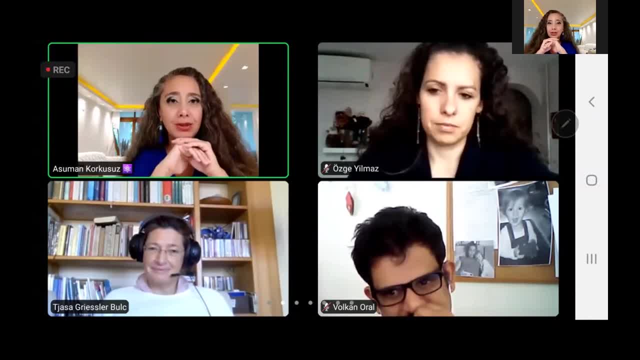 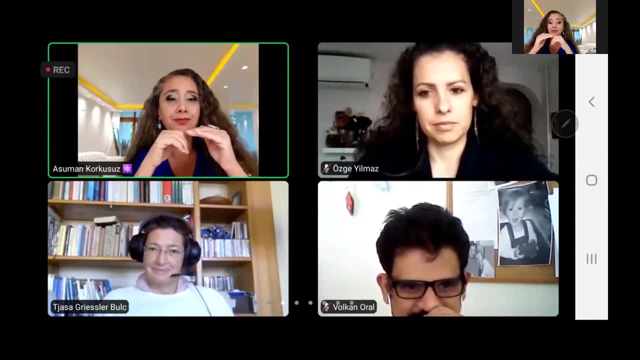 because in comparison also to the other packaging system, treatment system, it is not any more feasible, you know. so it is not any more cost effective. we had also some applications, but the thing is, if the treatment system is becoming a bit so simpler, then really the people are thinking to start in that way and they don't pay too much attention. 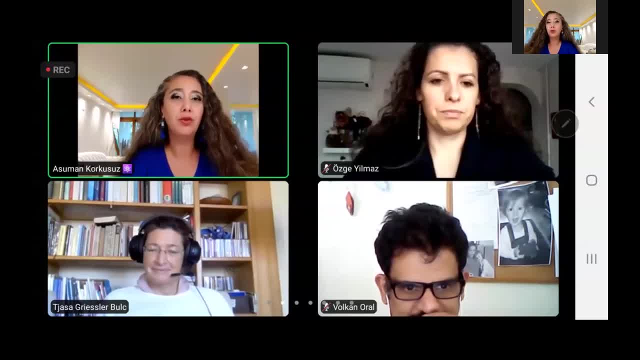 I saw also some of the constructed wetlands, some application afterwards made by the government, but it was not functioning because they they didn't have any idea about it because, therefore, it was my last presentation sliding on. it is not a fixed and forget system, it is not a magic system or it's not so simple. okay, it looks like so simple, but still it is very. 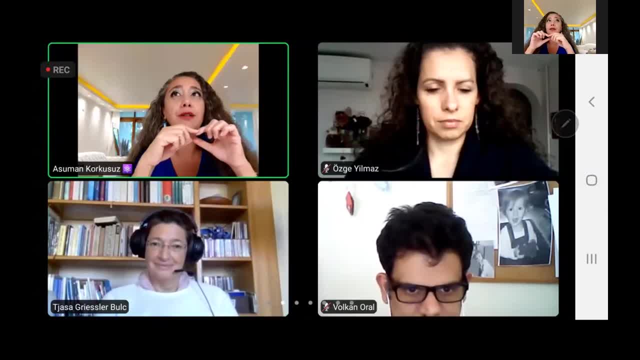 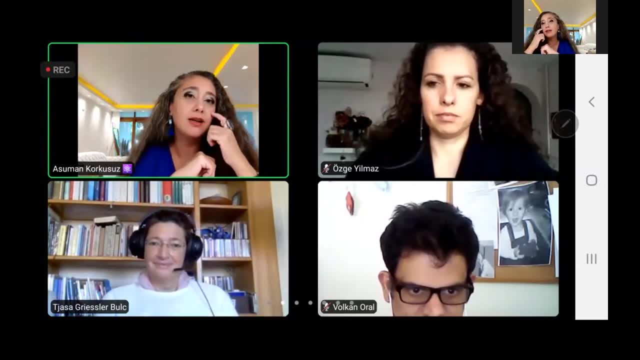 difficult for the, for the people maybe, who are living together, for example like, like in eco villages. it might start again in that way in Europe. as far as I remember, for example in Austria, it was like this: for the communities with, with, with the people of less than two thousand. 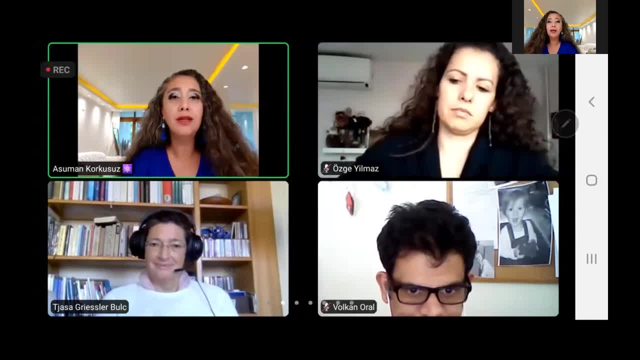 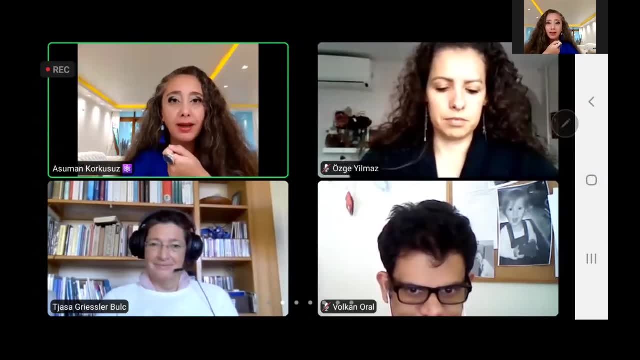 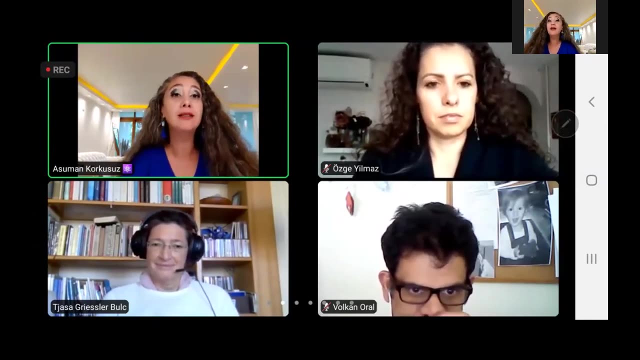 people, the, the communities had to build their own treatment plants by themselves. they had to charge. they had to pay the money you know for for the treatment plant. therefore, the constructed wetlands or such kind of nature-based treatment system were also an option, but in that case in 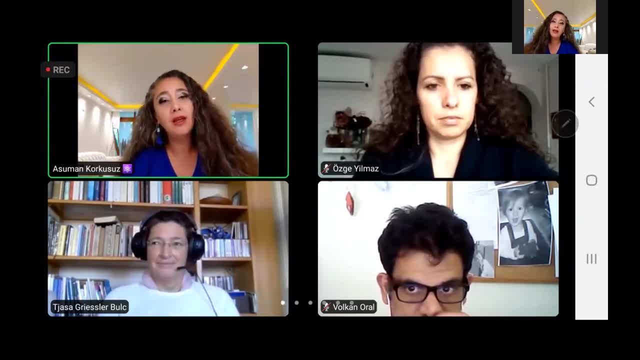 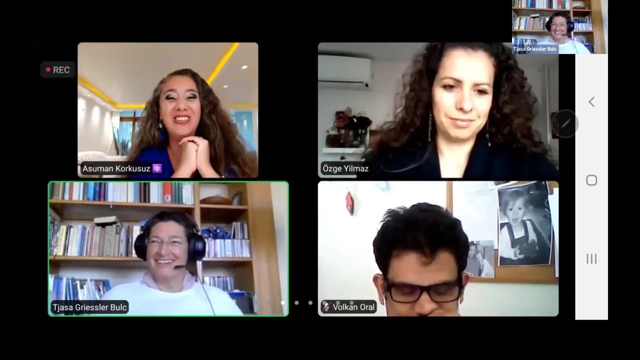 Turkey we still don't have such a thing, usually for septic tanks are used, you know, but little by little. now I guess it is changing. this is my okay, thank you. so yeah, I hope all the best. thank you, thank you, yeah. do we have any other questions more Asma? 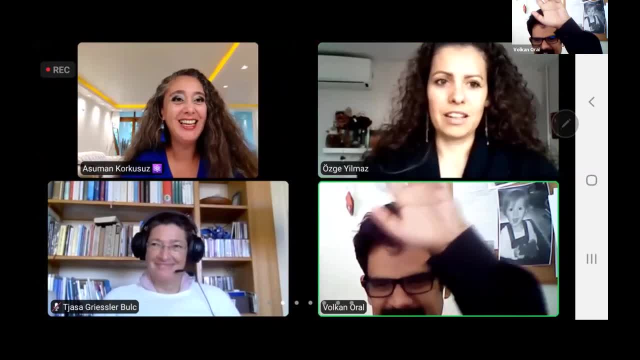 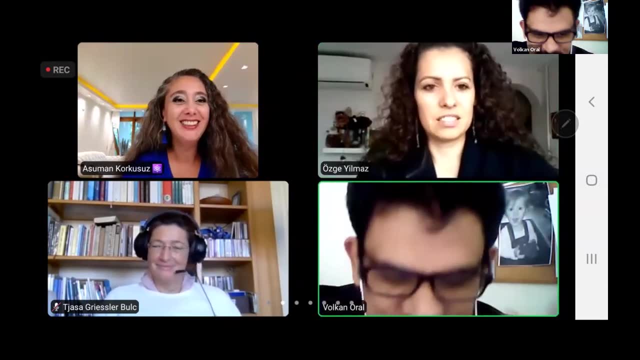 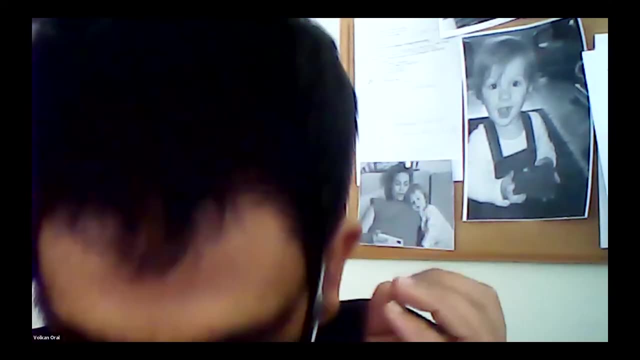 maybe, maybe, hello, can you see me? yes, yes, hello, good to see you. good to see you again, Tiesha. regarding you, by the way, good to see you, Tiesha, again. another my colleague. I'm so honored to be with them, mostly to be here. and one more small comment I don't want to take your 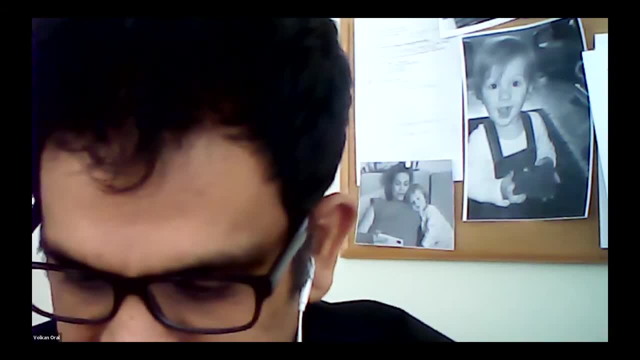 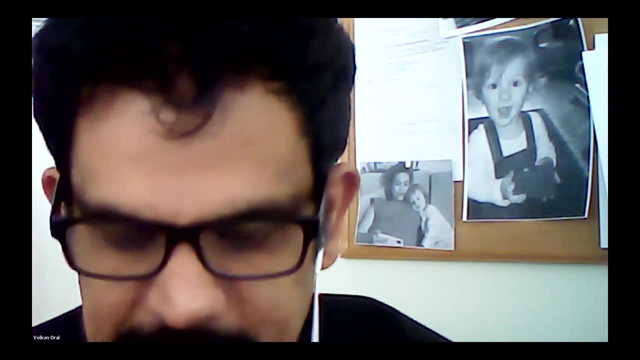 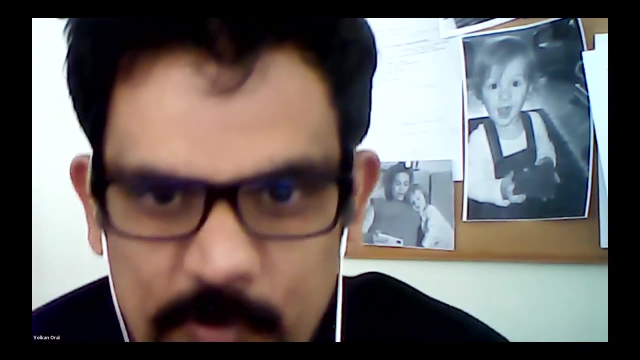 so much time in here. actually, the wastewater treatment legislation you know has been improving in Turkey. but you know, depending on some local conditions and local legislation properties, if you want to apply a new project it's getting some time. for instance, circularities or circular assessment is a kind of a new topic and a couple of days ago or the weeks ago, ministry of environment. 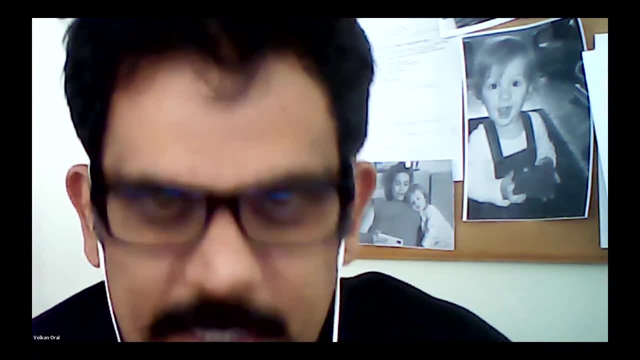 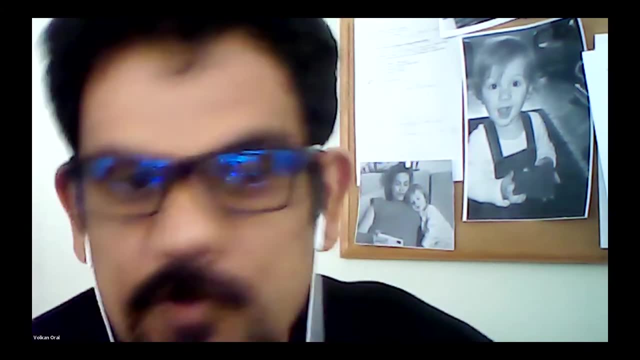 has been, you know, launching a kind of- you know, the auction or the kind of, you know the special topic calls, where on the government levels you can see some improvements, but in the local levels, when you talk the municipalities or the local governments, I mean there are still some, you know. 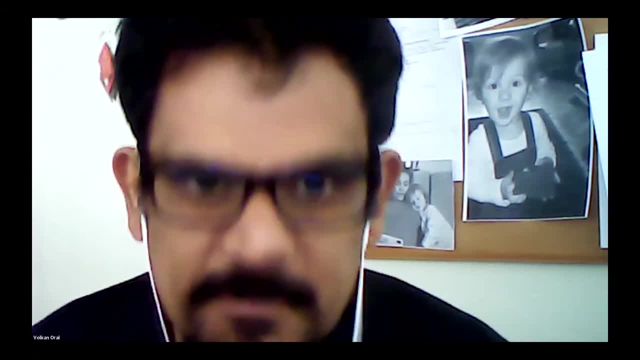 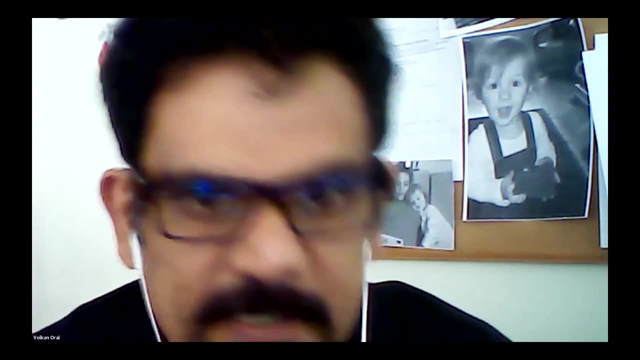 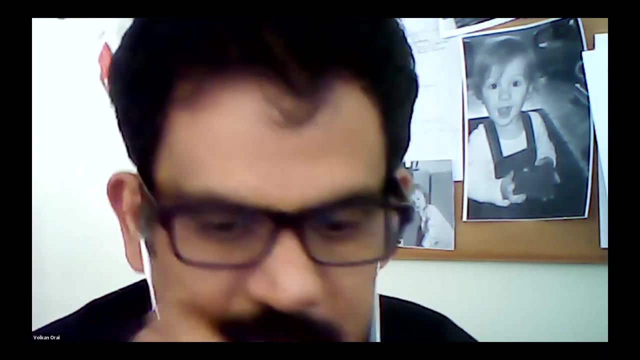 barriers first, you need to go over or you need to pass these barriers. but what I believe, actually you know Asma has also mentioned, and time by time, I think we are in the position to go over these barriers, a kind of project, just like you know the eco dengue or you know the, you know, I mean, I think. 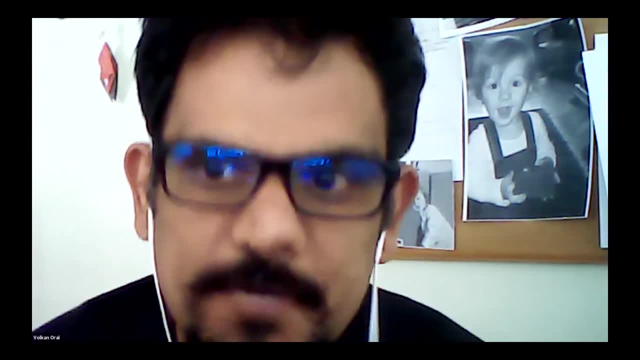 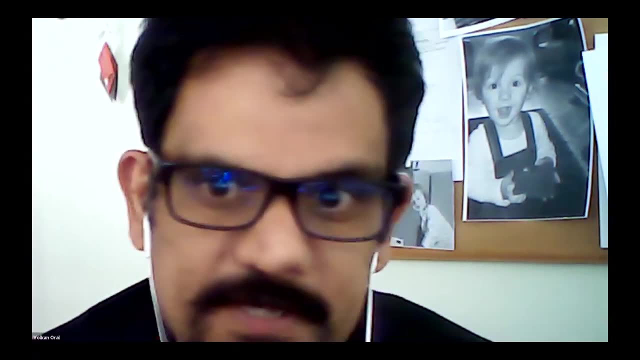 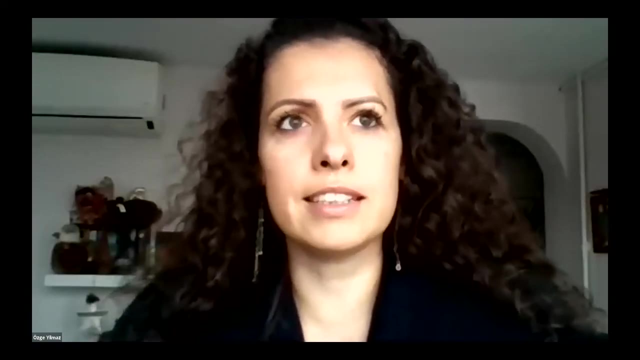 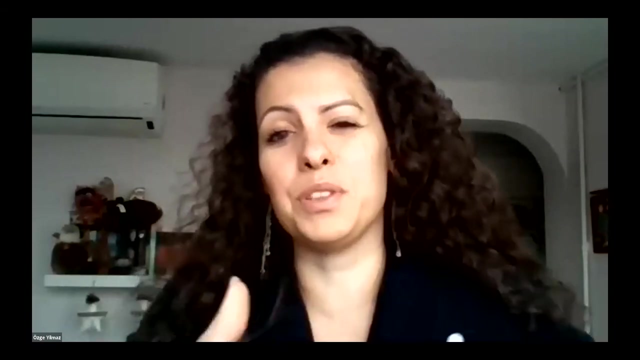 we are in the position to go over these barriers and I think we have much more opportunities, also from our cost section. allow us to pass these opportunities, to apply these. you know the barrier. this is what I believe. thank you, welcome. thank you, I also think. I think success stories are very important to push this kind of 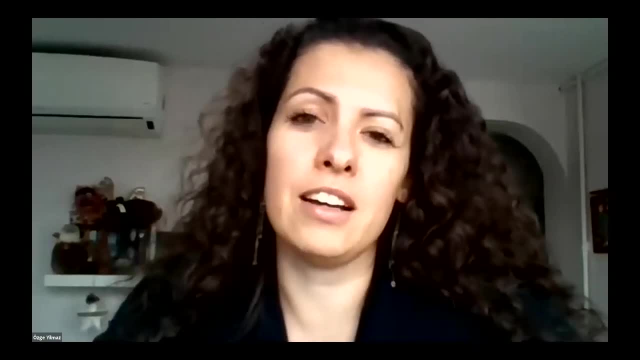 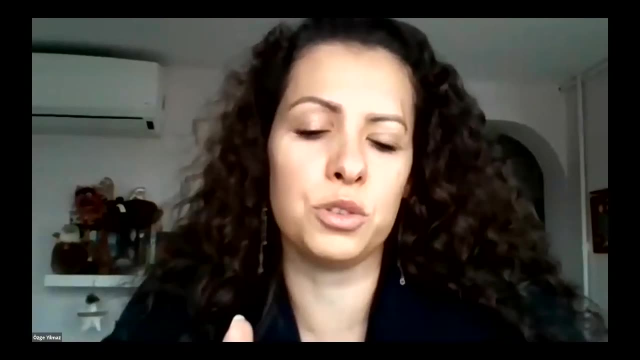 agenda forward in terms of the decision-making processes, especially if they are as slow as the current one. so I think it's good to have this type of funding from European Commission, from R&D funds, to showcase what you can do, and this is one of the things that that in a car project. 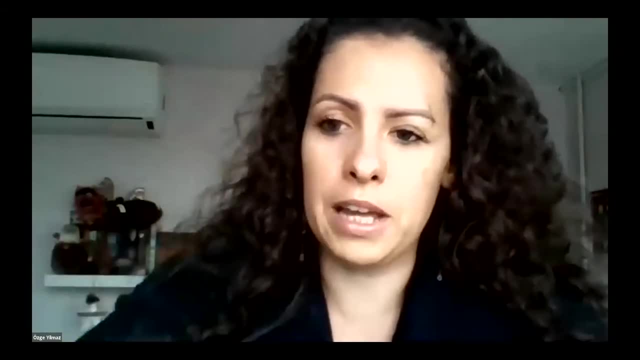 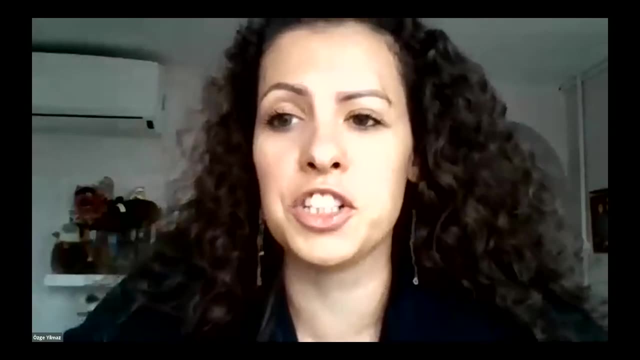 tried to do all around the globe, to be honest. so I don't know if we have any questions. I can see no hands, so I think we can move on with the Eli's presentation. so Eli Cohen is our final speaker. he is the founder and CEO of Ayala Aqua and 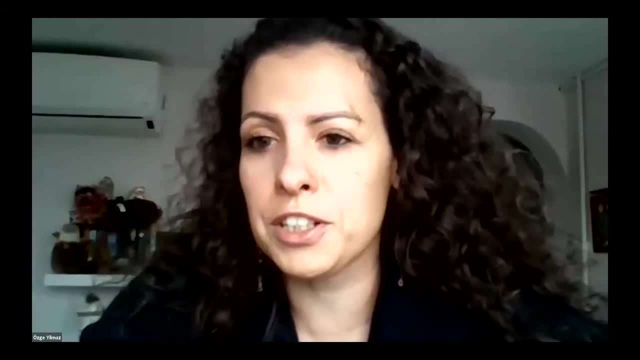 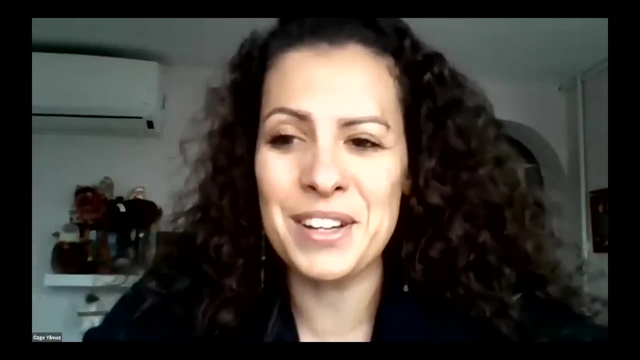 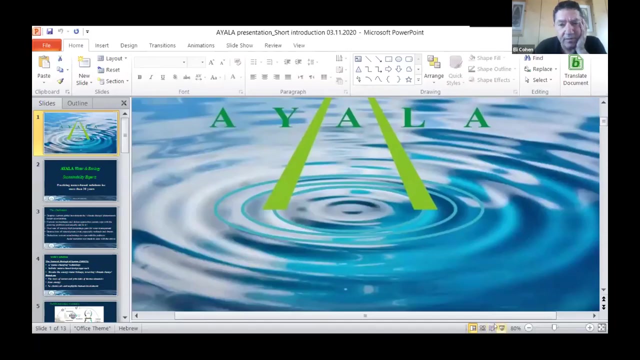 ecology in Tel Aviv, Israel. the company specializes in holistic planning for rural and urban wastewater management and purification of water and soil. so, Eli, we are eager to listen to your presentation on intensifying natural processes to treat wastewater. thank you, hi everybody, and hi Asuman, it was great hearing you after many years not seeing you, and it was it took. 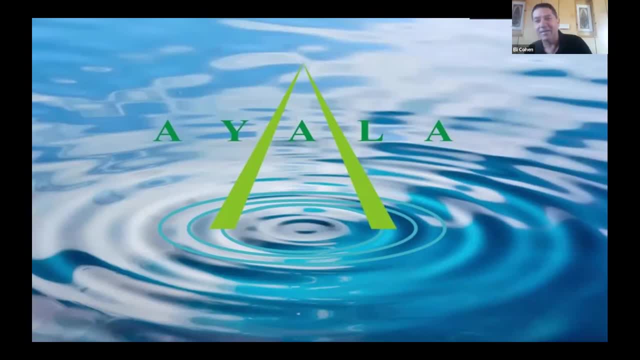 me many years back hearing your experiences and and struggling. it was amazing. thank you for that. I spoke to David just a few weeks ago and he asked me to share my experiences in this field, and these fields go back 30 years ago, and I want to talk about nature-based solution. 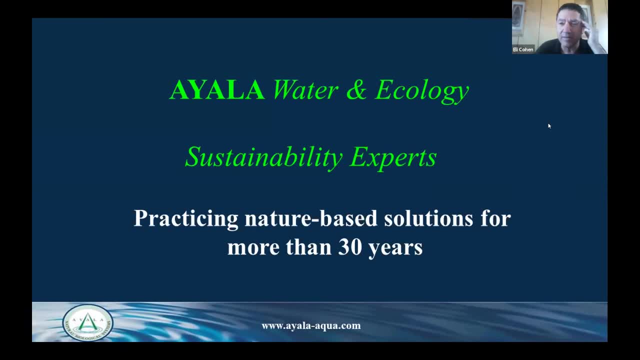 it's not something that can. people still think that it's something that kind of in the air. you know it's not. it's a habit, it's something of the future, but it's not. it's here. it's possible and we we have to do that. actually, we don't have any other choice. it's something that, if you want to, 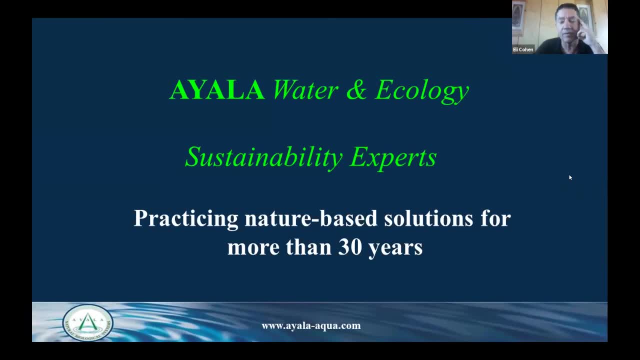 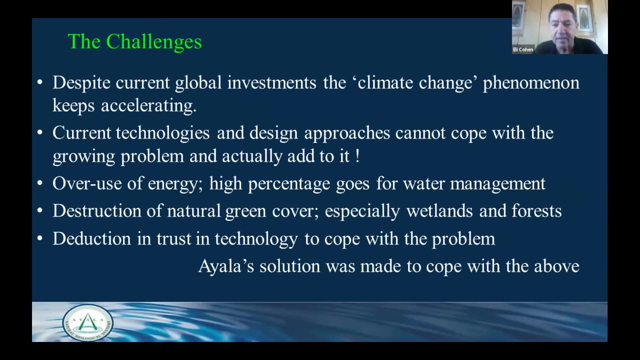 do we lose this? we lose the humidity planning should remain here, but we have humanity. much might might disappear because we're talking about climate change, and the only way to fight climate change is actually by changing our ways. changing our ways mean using less energy, meaning the and. 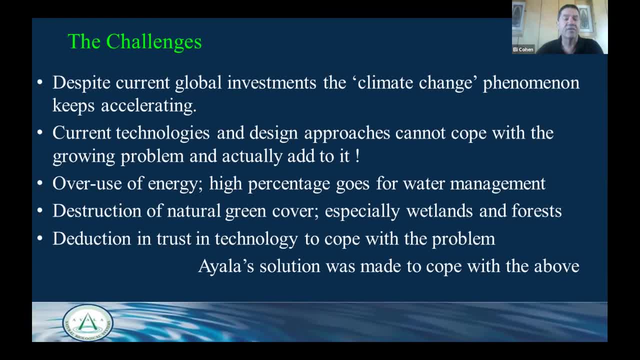 less destruction of the, the green cover of earth, which we're doing all the time. we're using enormous quantity of energy and this balance between uh, energy and water, this nexus is, keep keep on hanging around and it's a spiral. it never ends. we treat more water, we use more energy and we we never have, don't have a. 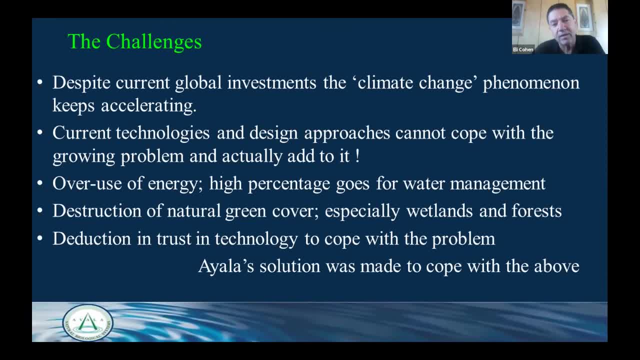 chance to to uh, to change this, this balance, or or again, the balance that we used to have in the past, and by using the natural base approach. this is the only way to do it, using no energy, no chemicals and and using only uh, only nature. god, god, god bless us. there's a lot of laws of the thermodynamics and 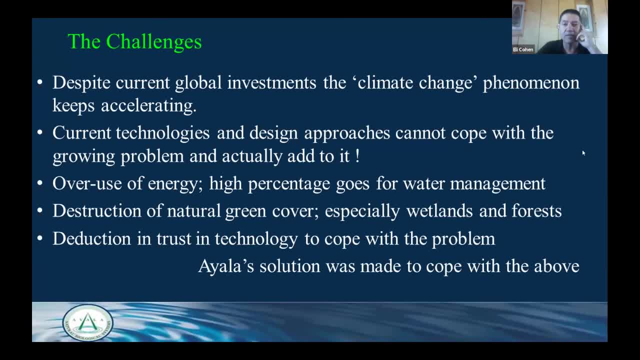 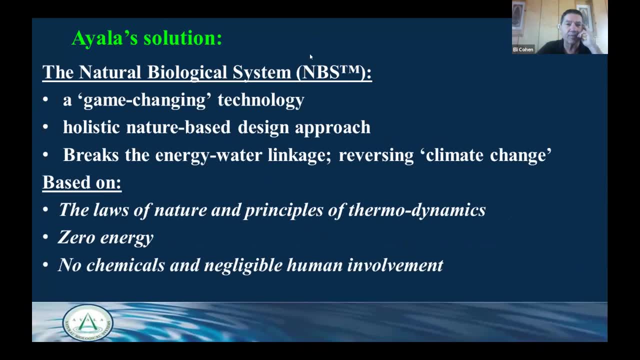 and nature if we can use and do amazing, amazing work around us, and i want to show you some examples of how it's worked. but before that, our solution: we call it the nbs. it's for many years already we call it the natural biological system and today people use it as a natural, nature-based solution. 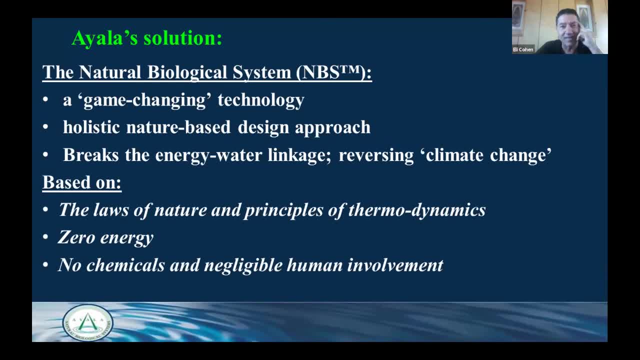 which actually it's uh, it's okay with us, it's a, it's a trademark, but it's uh, we, we, we are happy that it's actually take its place and it's a. we see it as a game-changing technology and it's true. people ask how it's being accepted by the regulators. it's still hard everywhere in the world. 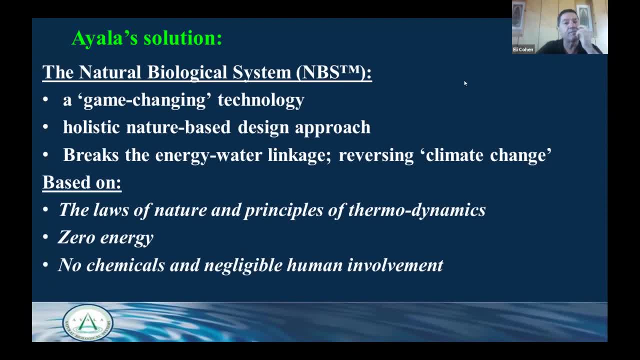 not only in my country, in in turkey, everywhere, because because there's a lot of interest involved in it and the big companies don't want it to happen. because it changed the game, the, the, the. it's a game changer and you ended to penetrate. it's take time, take time, but, but, but the conditions. 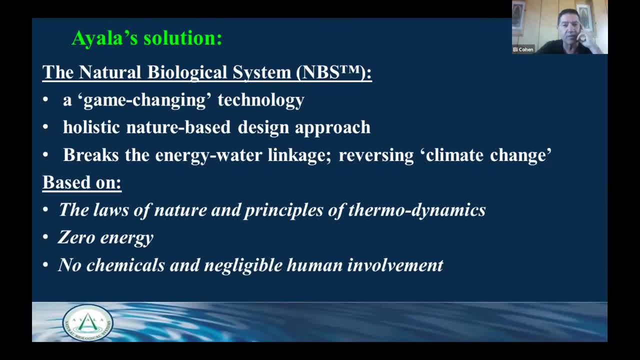 now are for us. so we need to uh, use it and and go ahead and just show the cases and then and move ahead fast and uh and the. our approach is also holistic. it's not only about treating water, it's about approaching the entire watershed. i'll show you some, some, some, some examples and then. 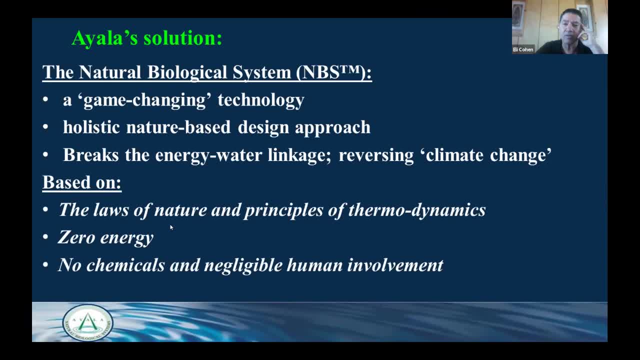 you understand what i'm talking about and again, like i said before, it's about uh, it's about a law of natures: thermodynamics, zero energy in the system itself and no chemicals and negligible human involvement, because systems are usually tend to fail when it's come to. 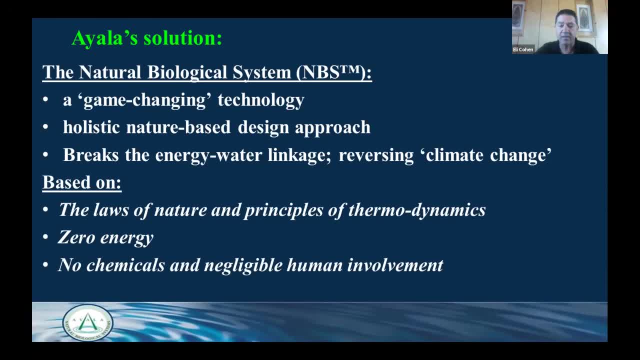 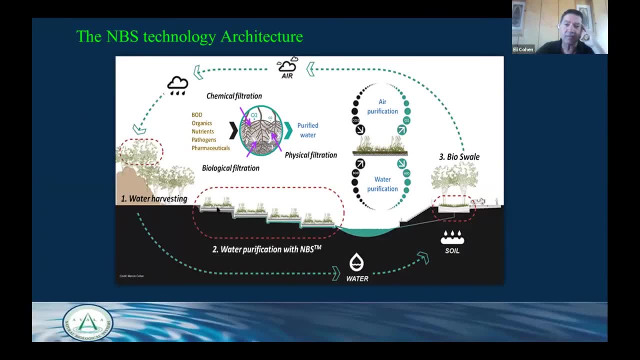 maintenance and we try to avoid it. let nature do its plates all and then, in general, this is the picture of how it works. we can see this: the system we use, the gravity, we're using the, the root zone over here, we where we're having this chemical, biological and physical filtration happening all together, all in natural way. 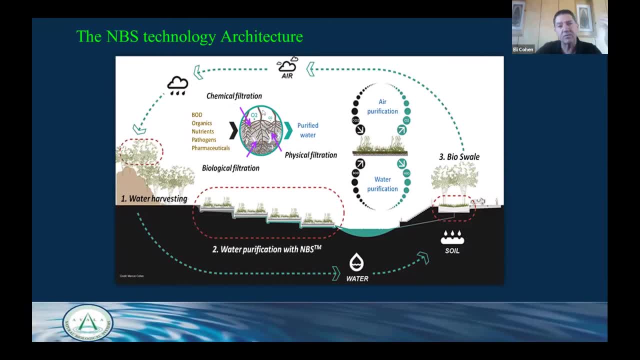 very effective. we all know how it's work. plants introduce oxygens at the root zone, exudates all together, the, the, the, the volume of of activity in this, this area, is thousand times more than in a database class, for example. very effective, very efficient and everything is. 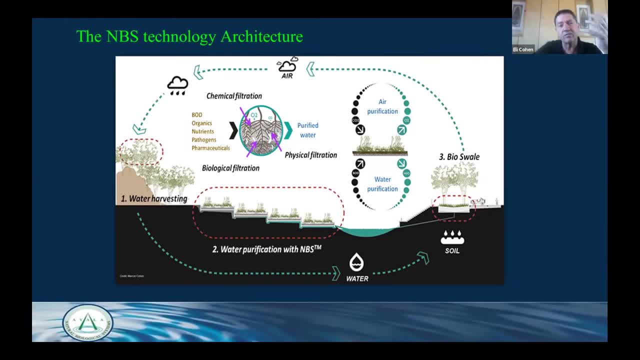 regrettable. you just need to to play with right, right with rightly, with the, with the, with the plants. i'm talking about the hydrology, which is very important. talking about the plants, talk about the, the substrates, the gravel, talking about the additives that we're adding, natural ones, all. 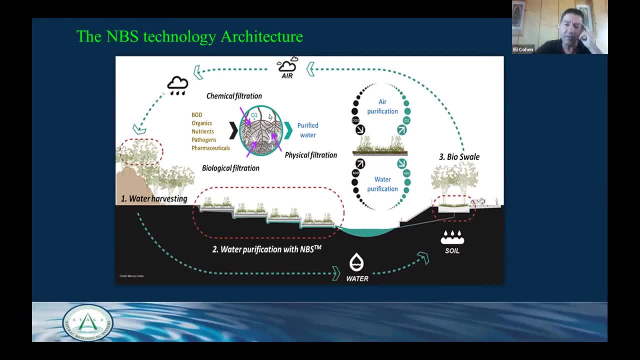 together create a very powerful, very powerful system and the root zone and the and the and that can do anything we want. we just need to design it properly. and it's also about water harvesting, stormwater harvesting, treating them, recharging the aquifers. it's about preventing floods. it's about 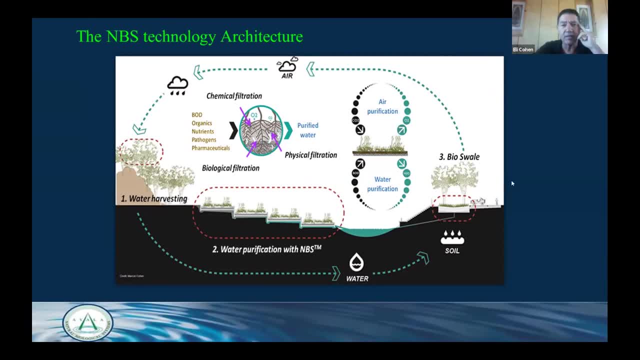 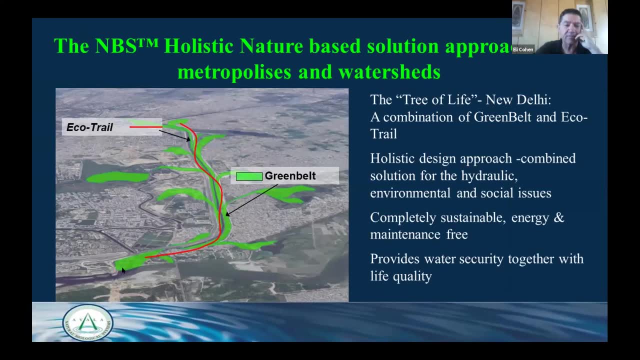 the, the, the temperatures in the in the urban area. let's see example. this is something that we designed for the city of of uh of uh, delhi- actually it's a state of delhi, new delhi in india. this is the yamuna river, you know the name goes to the gangas and this is a big drain running into the. 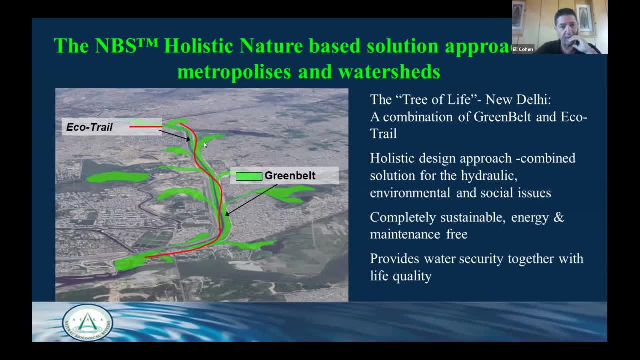 into the river. we got a mandate to treat the sewage coming out from all this area. it's a big area. it's about eight kilometers length of this stretch and it's a about eight million people living in this area. eight million people and we and they don't have. 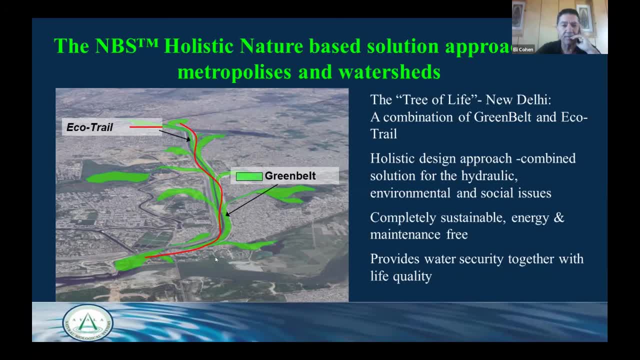 a solution. all the sewage running freely down here, filling the yamuna, which is very dirty. they don't have the aquifer being pumped to this. it's very low. no, no, no, no sources of clean water. uh, temperatures goes up. they're facing floods every, every monsoon time, because the nothing stopped the rain water from running down. 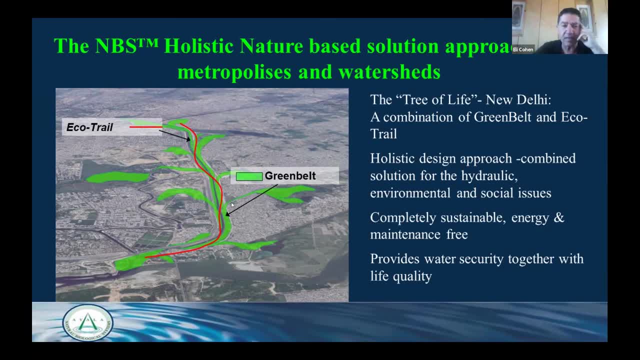 and people just living here in hell, and we designed a system that uh, give give answers actually to all the problems at once. we created the tree of life and actually we treat the sewage on site, at close to source, and we as part of the landscape, using gravity, only gravity. 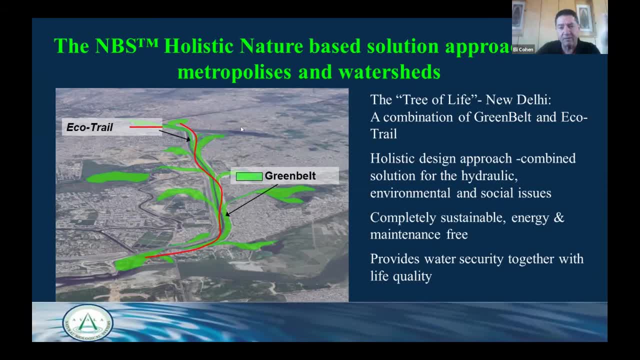 and we reduced the, the conveying system, dramatically, almost to zero and no centralized, all, of course, decentralized, we creating actually a beautiful park over here. people actually can walk from the yamuna to their home through a park without even thinking about uh, uh and not having, not having to go. 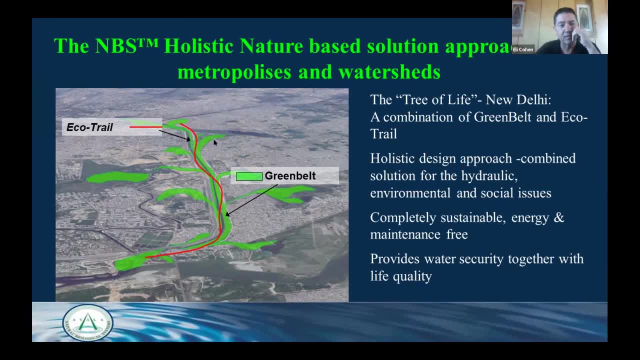 through any street or a highway that they can, and people are being killed every day there by numbers. and then, and opening this green corridor over here, we call it the echo trail and the green belt, and it's it's uh. in the same time it's a. 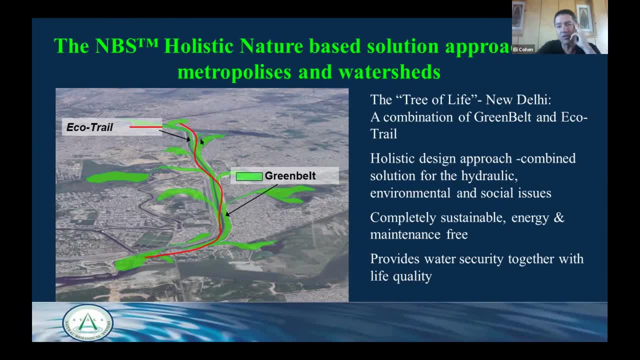 holding rain water. treat them storm water. treat them on site, recharging the the aquifer with a clean water. create the sewage water in this area, on this stretch, we calculated can treat 250 million liter a day, which is a huge quantity of water: 200, 200, 250, 000 cubic meter, if you're. 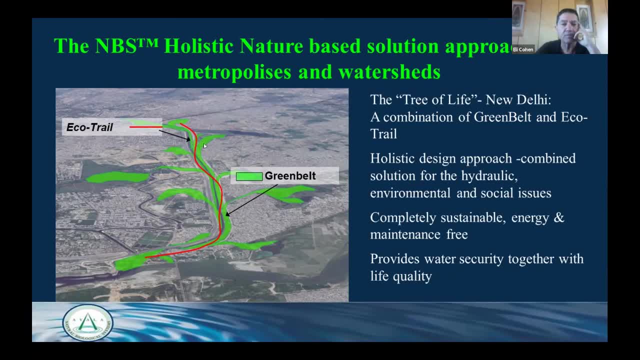 wanting to in cubic meter, and it's of course. it's because don't use any energy, it's reduced the the temperatures and it's a. it's a very powerful carbon, uh food, carbon, uh food production, carbon absorption. and just keep in mind that wetlands are much more effective. effective than than. 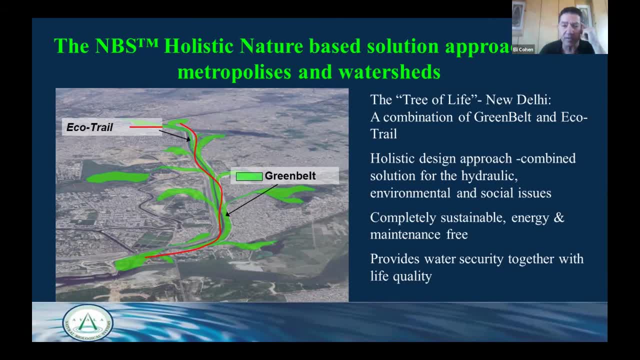 forest in, in harvesting carbon from the air almost 100 times more effective, which is very, very important to remember. so if we, if we fabricate the city with many systems like that, things about the change and it's all a part of your landscape. we call it the active landscape. 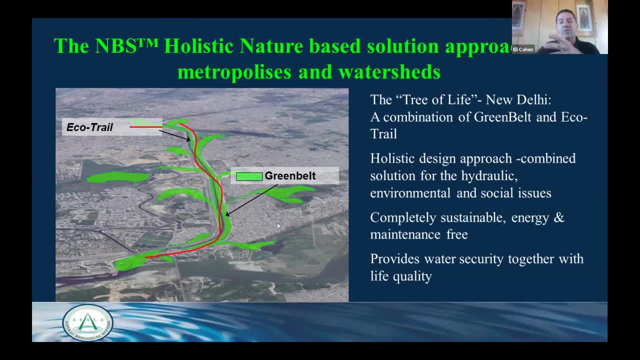 so actually you don't actually change the city, you add to it. you change, don't change people life. you add to it and it's, and it's a and it's much faster to build and it's it's much easier to build, it, it's a much cheaper in the end of the day and the water quality you get is very, very. 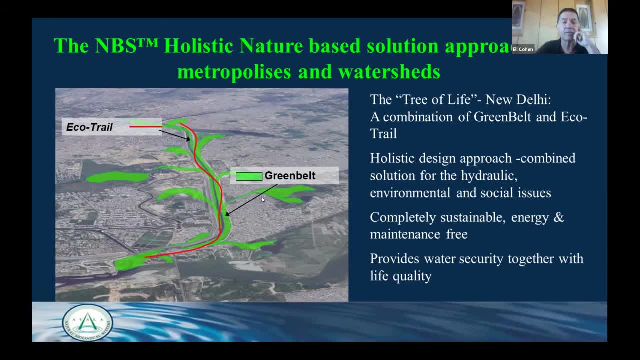 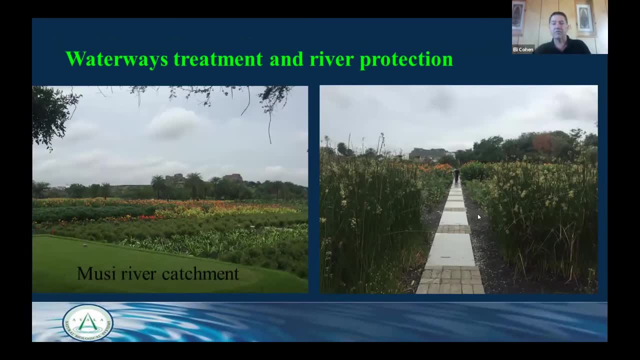 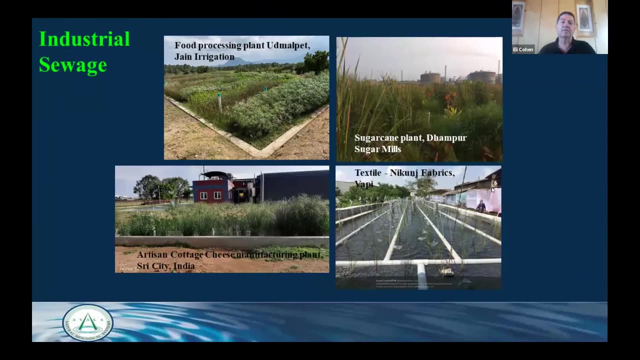 high and stable. it's very, very important to keep in mind- and this is how things looks after being built. look at this: beautiful parts in the part of your landscape and- and we- but it's not only about domestic, it's also by industrial. i think we have many examples. 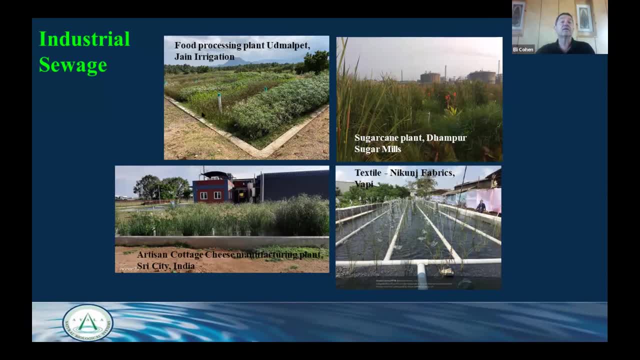 that just didn't go. i just bought a few. uh, this is a food, food production uh factory, uh down in south of southern part of a big company southern of india, in tamil nadu, working for five years beautifully, very hard, water, sugar, sugar cane plant very hard, one of the hardest in the world to treat. 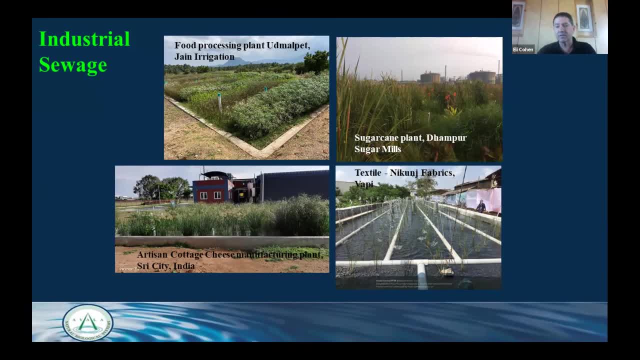 talking about 250 000 cod milligram of cod. uh. dairy factory for for cheese? uh, this is one for, for, uh, this is a one for a textile company in north of of mumbai and it's- uh, it's all working for many years, very efficient, and we save them a fortune. so that and why the investors go for it. 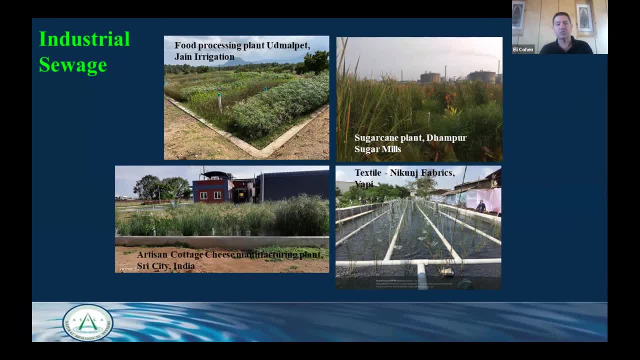 have to, they force them and this is the most economical solution that you can think about, and the quality is getting better and better through the years, and we're having experience with so many others in industries: cosmetic, pharmaceutical, even radioactive elements. we harvest and then we treat uh. now let's go to the domestic uh, i think. welcome. you spoke about the. 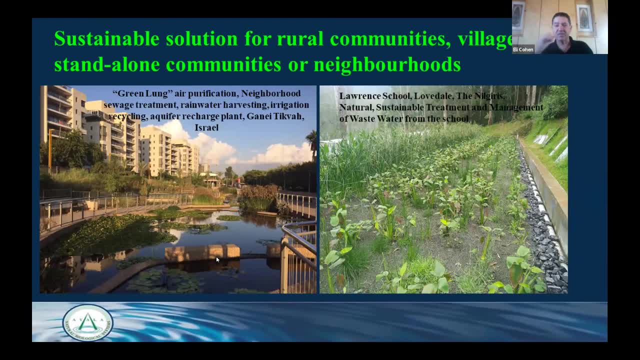 the, the, the, what's called the green green city, something like that. we are doing it. we are doing it and also actually daily going to be. look like this, take some time, but in the end of the day, something like this: you take, you take the sewage from this, this neighborhood, you do it over here. 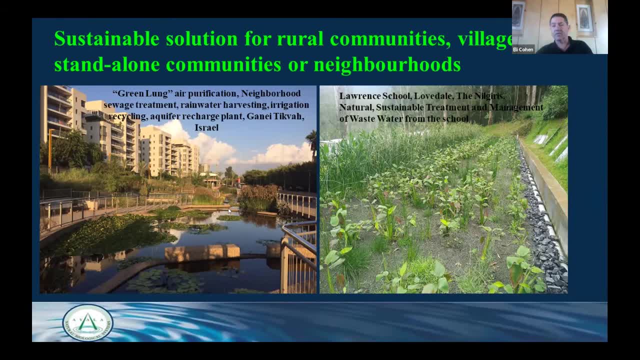 and this, this is a gardens, and then you use it, the ornamental form, very clean water, and in the end of the day it's go for irrigating the entire area over here. this is another. this is, this is a one is in israel, in new tel aviv. this is uh in the mountains, 2500 meters in. uh in india, in the. 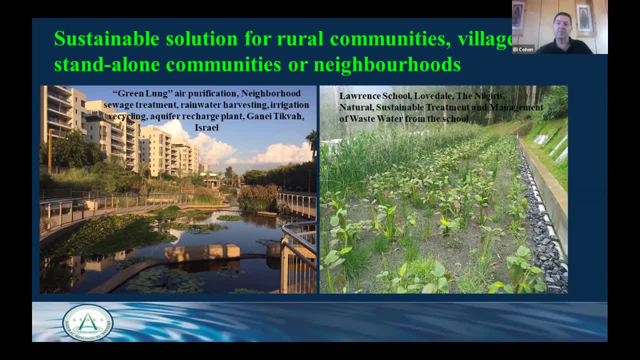 southern part. beautiful, very old school. they build only two systems for a big one and now they're building another two. very happy, and it's a trading and they're talking about the thousands of children. so it's a very high, high class school. so it's working very, very efficiently and they're 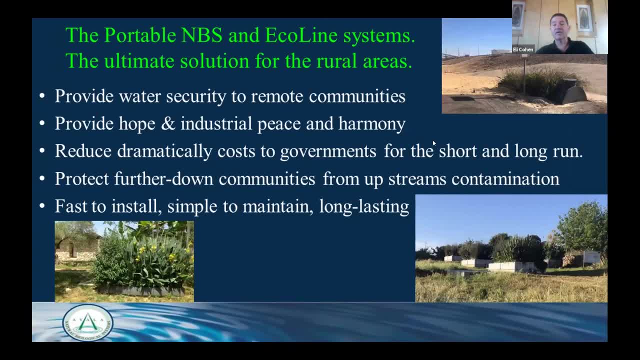 very happy with it. uh, we having, uh, of course, the much more. but i want to show you the, the many people talk about the, the on-site solutions, and i want to show you something that we develop. we call it the portable system and the echo line and the one. 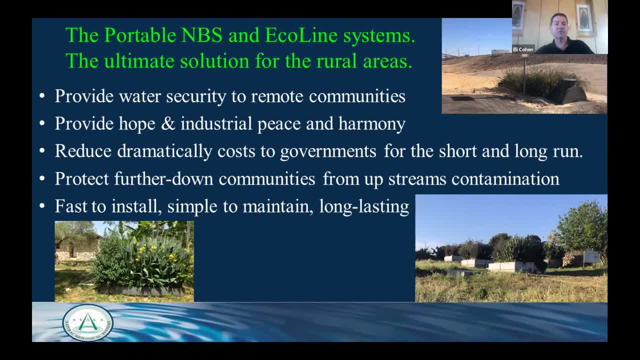 it's a small system- goes for the private house one, we call it the echo line one, through the equivalent two, three, four and up to the portable nbs, which is actually containers. special containers come to the site being a, being a, pulled up, put on the side on the platform that you prepared in advance, and it just you, you. 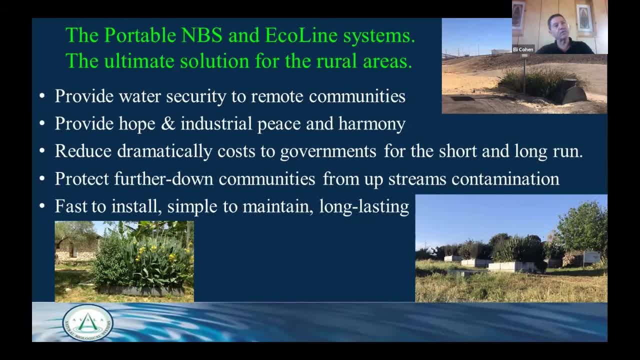 treat water? uh, we, we develop it in in request to um people that ask for to supply good water to villages, many, many villages all around the world. i'm talking about millions of them not not having a good water anymore. all the water sources that is used to have are contaminated now, so we are 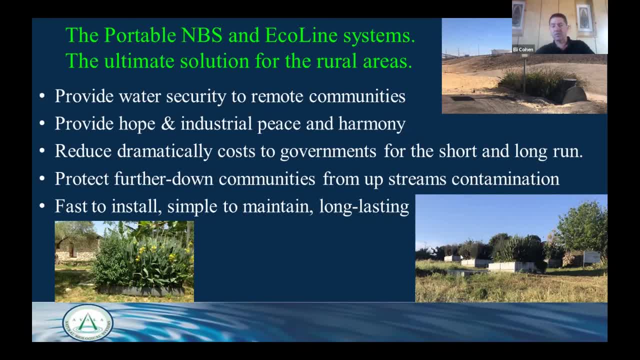 treating this sewage, this soil, this water from this source by natural way again, no man, no chemicals, no energy, it's all by gravity, and you have clean water coming out and in the end, in the end of the day, uh, now we developed another element that you can add to the outlet so we can treat something like 10, 15 or 20 percent of. 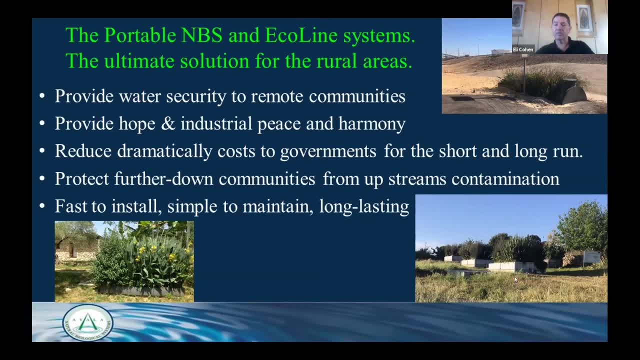 the water to a quality of drinking water and drink quality by using special elements that actually like a magnetic biological magnet, that that harvest the pathogenic element from the water and you have a zero, zero equality in the outlet and the rest of the water goes being used for irrigation, whatever you want to, and we have this. 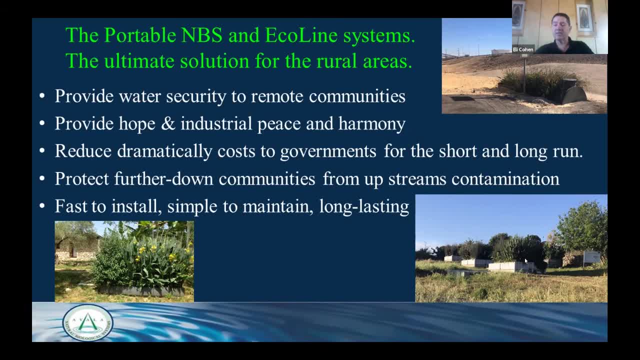 in different sizes, different, and it's again completely sustainable, energy free, chemical free and it can last many years forward and and all it also can create your sewage afterward and protect your aquifers. and then this is the bigger one. it's up to 40 cubic meter per day. it's quite big. 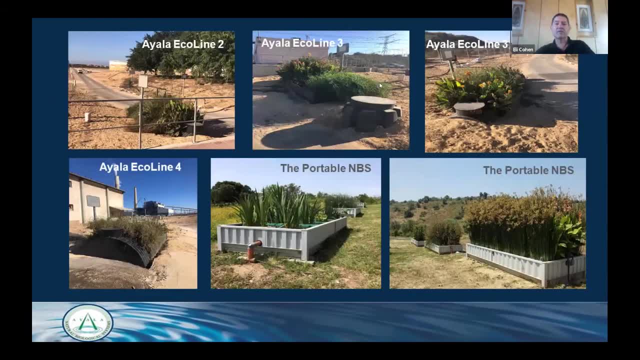 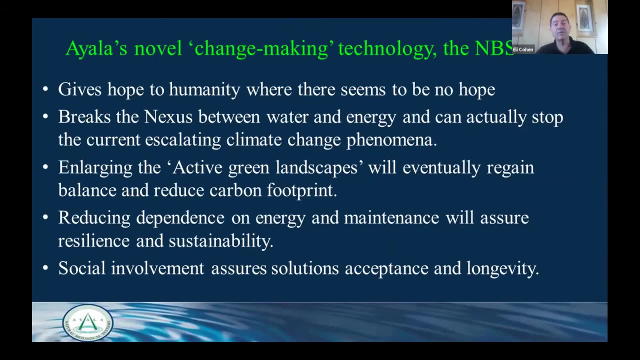 but you have the smaller sizes, you can see them over here: the ecoline three, the two, the portable, in different sides, different places and and it's all uh, it's all uh doing the job uh very efficiently. just to summarize: uh, uh, i mean this is, this is a must. it's not any more kind of a like a. 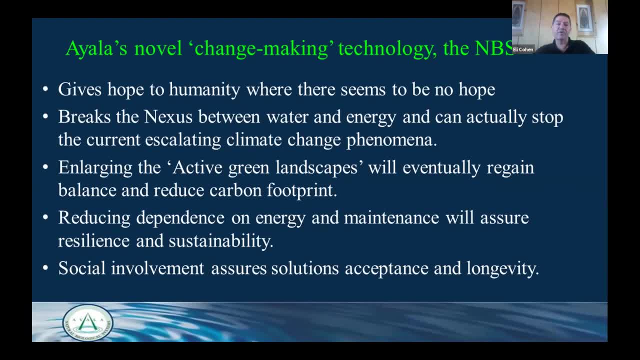 please, uh, fashion it's it's about. it's about changing the, the, the rules over here, the thing that the game and the game rules over here, and and we have to do that. it's a must because, uh, because we cannot keep on using energy as we used before. 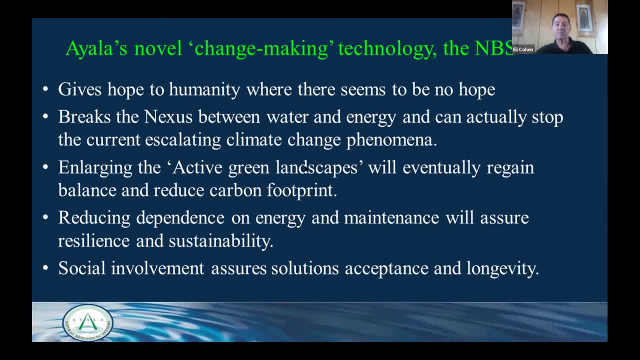 and, of course, uh, we people are looking for something to be also social system that will be part of our life, not something that we have to, that we have to put a lot a part of. we don't have noisiness like smell or the or or a noise just part of our lives, just existing near our place. 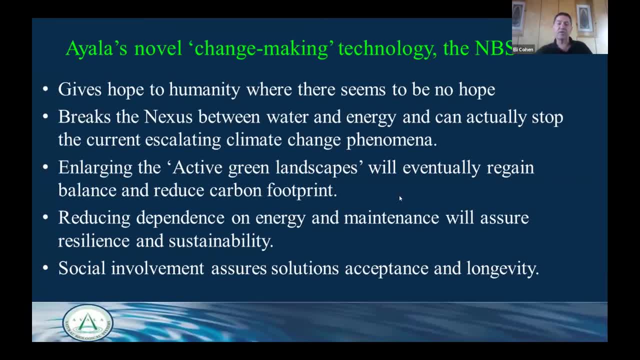 and this is uh. again, i'm saying: this is the future and and you are in the field and i'm happy that, uh, i, i was, i happened to meet david and speak to him in order to show the potential, and i will be. it would be lovely to keep in touch with all of you and just to push it forward, if you have any. 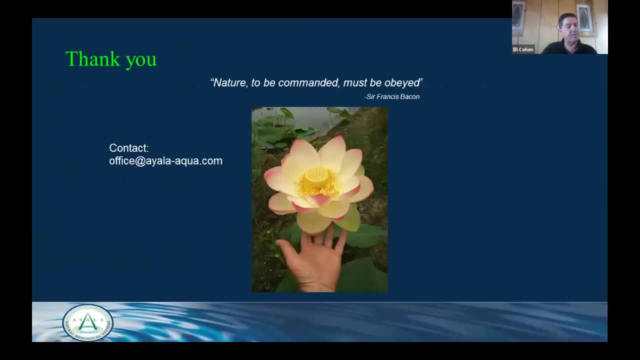 questions. please, please, do it. i'm checking the audience for questions, but in the meantime, eli, this was a very impressive presentation. thank you very much. so the the changes that happened. to see them, it's very eye-opening, uh, to be honest. and also i think you had a very good point about, you know, cutting the. 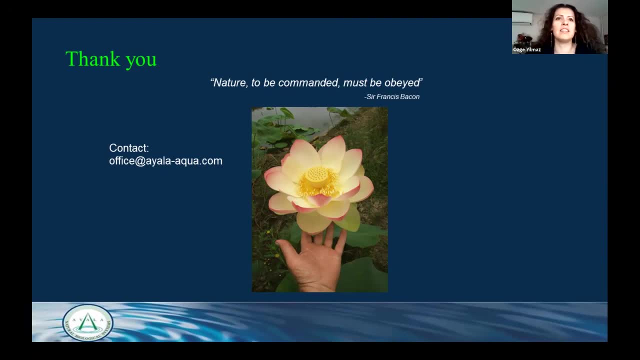 the, the, the dependence on the water and energy, the energy water nexus. uh, it's very important uh within the framework mbs. of course you know we have to be very careful about uh mbs. of course we are concentrating more today on water management, but we should always be aware. 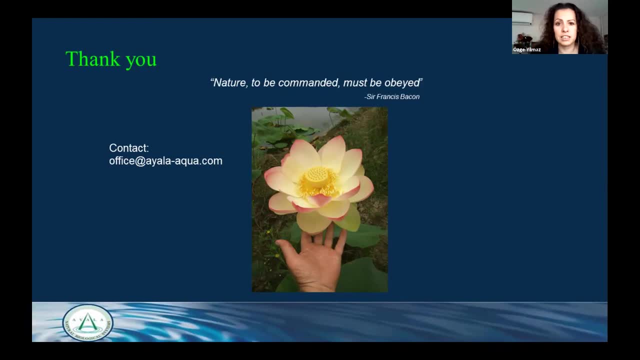 that mbs can be great tools for climate adaptation for the cities and rural communities. i think this was also mentioned a couple of times in previous presentations. uh, thank you very much. i'm just looking at the audience again for any questions. yes, welcome john. please, uh, shalom. 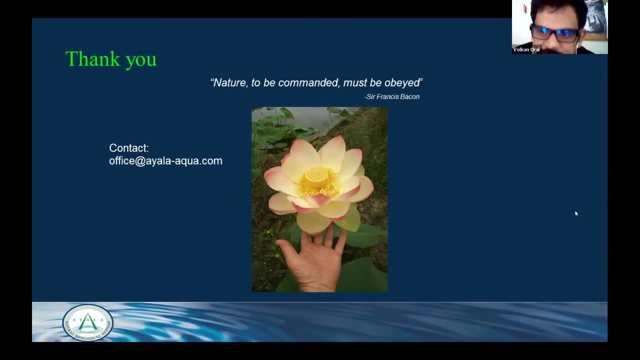 good to hear your presentation, uh eli. thank you for the presentation. i have a question. i spent some years in israel while i was doing my postdoc in sedeboke and during my postdoc uh studies. i'm talking about just seven and eight years ago. 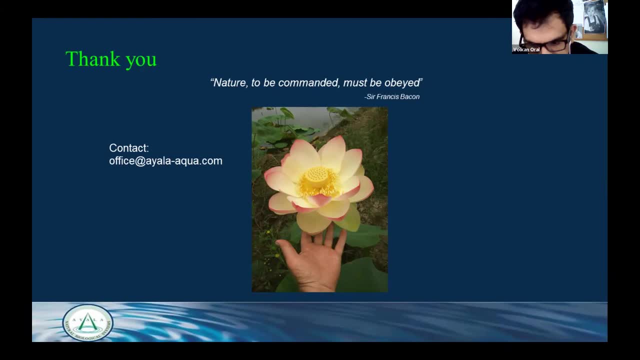 i have also seen some you know um green zone applications that you presented uh in israel and during this time- i mean these- these applications were a kind of a new or novel approach- was taking in the country. um, what is the current station right now, or i'm talking about 10 years after uh more going on? how shall the country can? 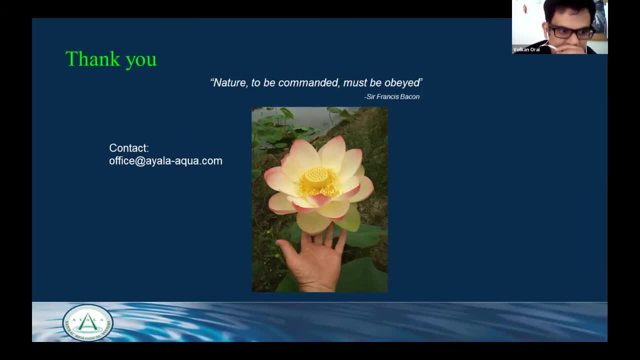 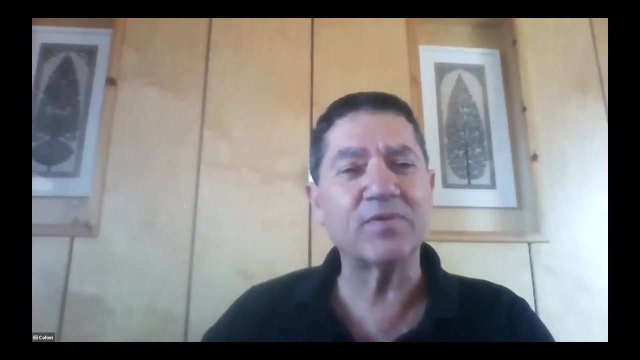 adapt these nature-based solutions that way, and what is the you know, the legal status or any kind of uh governmental application? it's a good question, actually it's strange, but it's getting more, harder and harder to implement it because of you know, since we started doing it in the 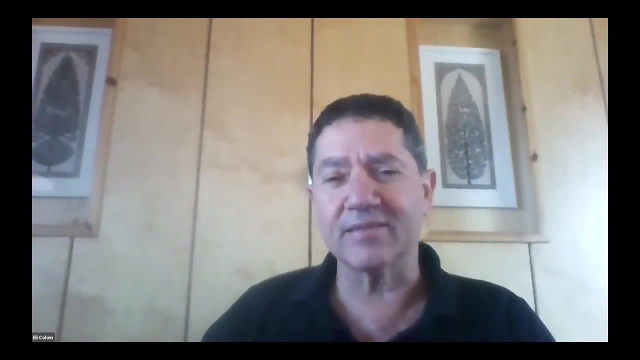 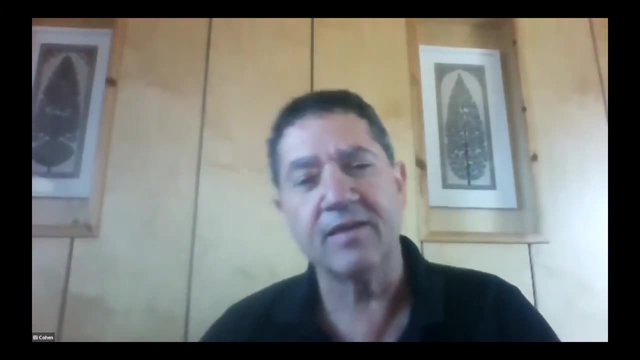 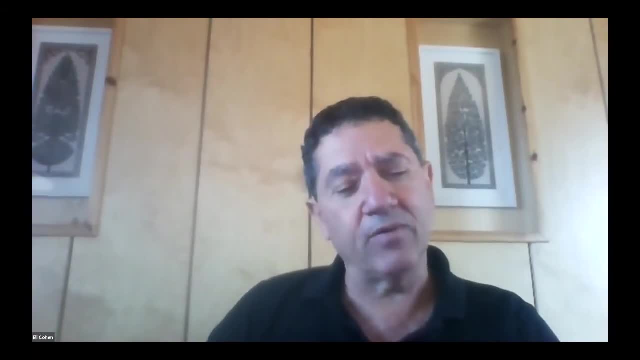 today they're positioned by the, the water company. they don't want it to happen because actually we, we're actually penetrating into the market and you think about it. if you do this one, there's no need for conveying system, piping, pumping, etc. it's a different ball game. 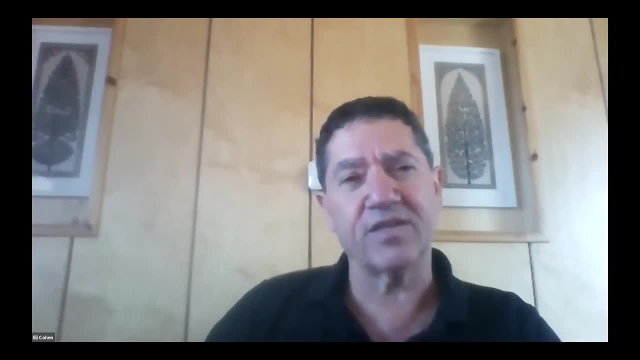 so it's a. it's a it's not easy, but but i can feel a change now and and we're doing now, we're doing mainly in israel, we're doing mainly industries, because they don't have a choice, and we do it at the inside, the industries. we're doing it for remote villages, we're doing our rivers, we're doing. 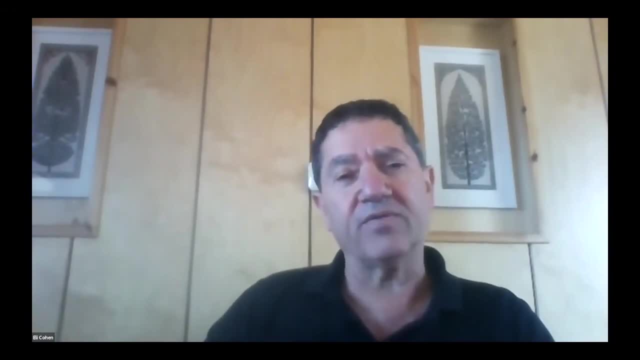 protecting the rivers from incoming sewage along the rivers, on the, on the, on the edge of it and in different places. and we're doing lakes in different places and we found our niche, but but we're pushing forward the, the urban one, and i i believe that the, that there is an open eye, especially now, after this, with this. 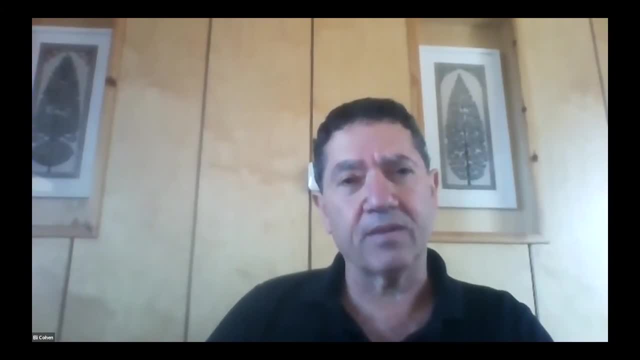 corona stuff. people understand that there's a limit to the technology with all the, all the respect. this smaller, this small virus uh kind of paralyzed the world and there's. so we, there is a limit to what we can do with technology, so we need to to to, we need to uh, give more place to nature. 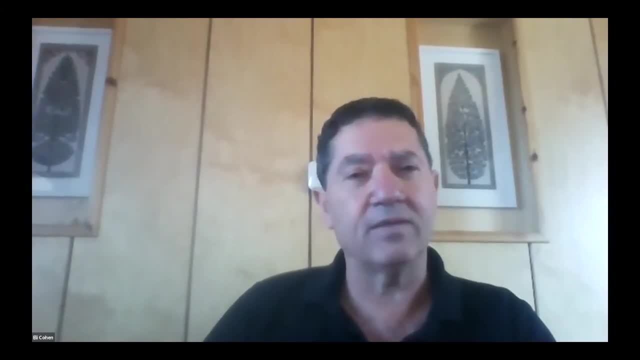 and and still not not affecting our life lifestyle. we don't. there's no, there is no uh, there is no uh, any uh. it's. it's not going one against other, so it can live together. so i think there is a change in the air for your question. uh, as far as i know, there are some keywords located in the south side. 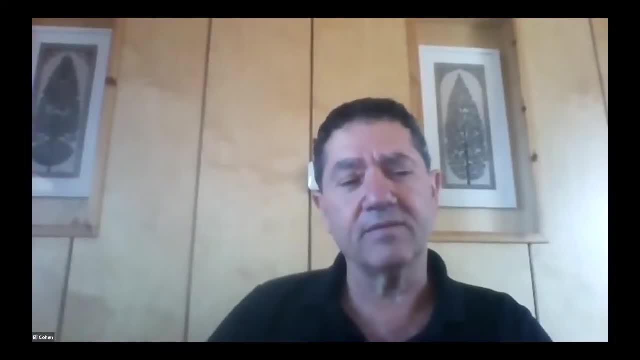 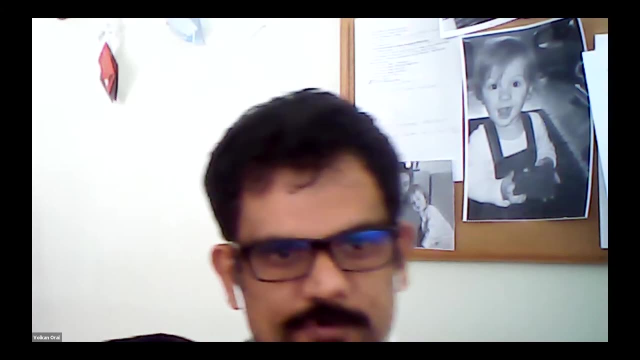 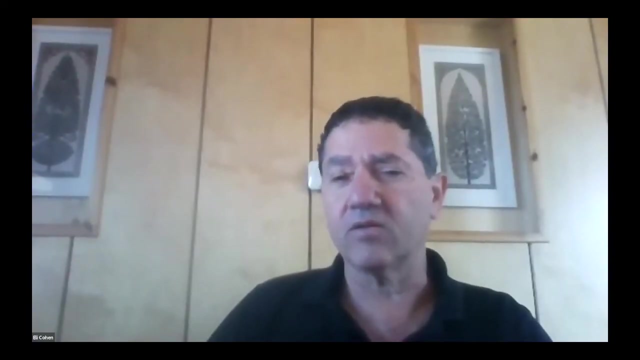 of the country in. you know, yeah, yeah, yeah, yeah, this is my system, so it's beautiful, yeah, and they're applying, they started applying these types of technologies. but yeah, i mean, you can see some, you know initiatives, not only you know the only. no, no, you're right. you're right, we've done a lot of 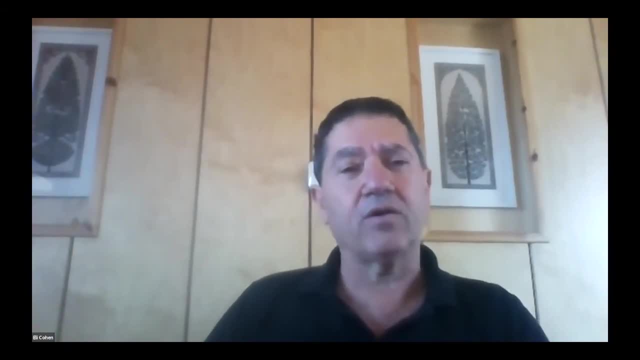 things. we've done a lot of things. we're working, working beautifully. it was also we were used to be part of the course in the past, as someone remembered it, and it was published in the in the post across the uh group for years ago, almost 15 years ago already. yeah, we have done a lot of. 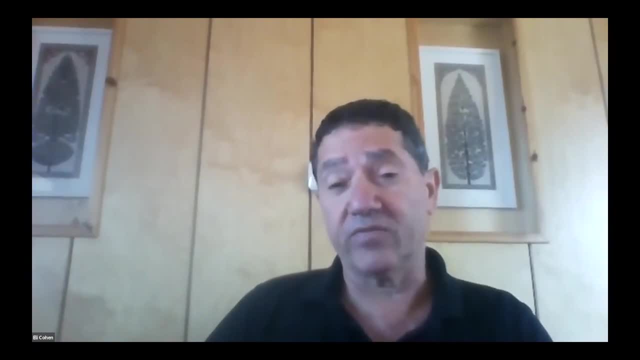 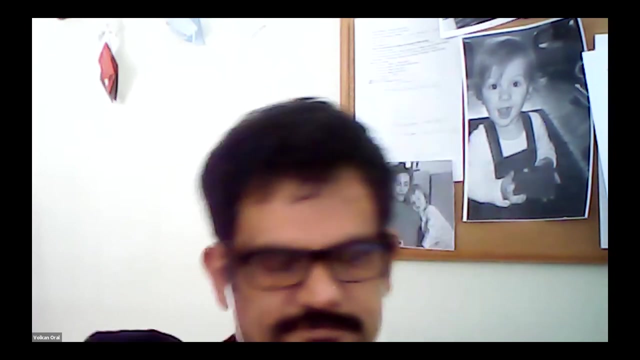 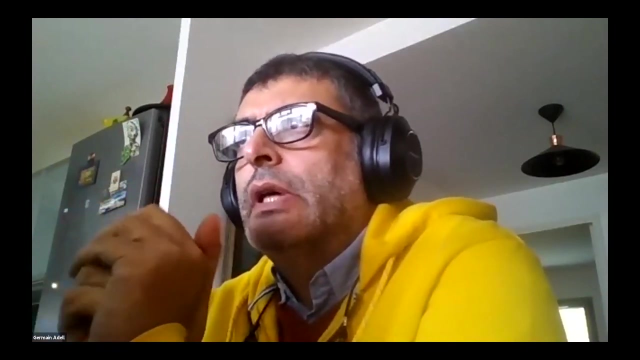 work, and it's working today, getting better and better and it's actually we've done more than 200 systems already, but it's still nothing compared to the, to the, to the need. i'm talking about israel also outside. we've done quite a lot, okay, thank you. thank you, i. i also have a question is about your portable system. can you tell us a? 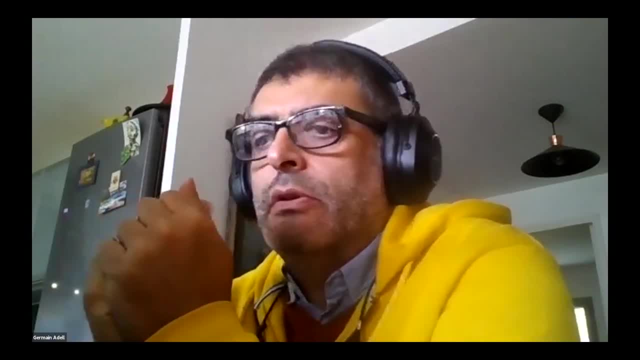 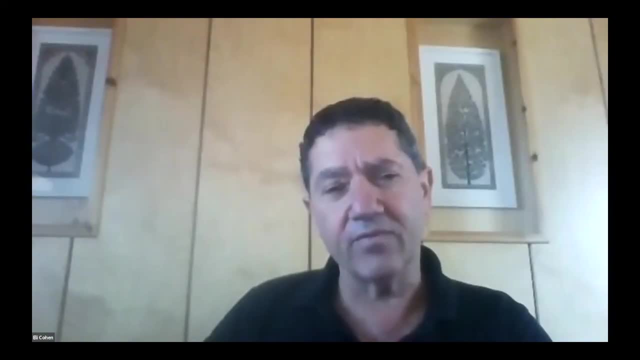 little bit more, eventually showing some other pictures, or which is the size, or how you deal with it. with the portability of a system like that, i give it a give it a background. i was approached by some volunteer, an ngo, years ago, asked me if i can. he can treat water for in villages and 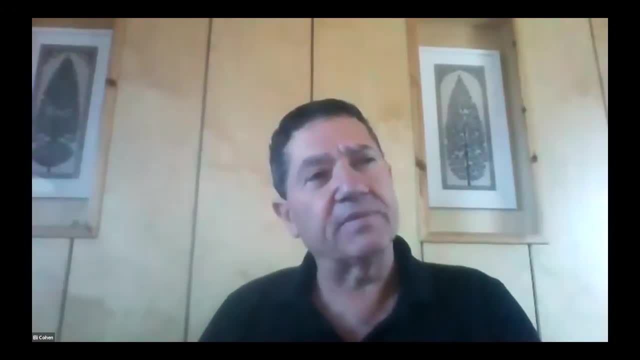 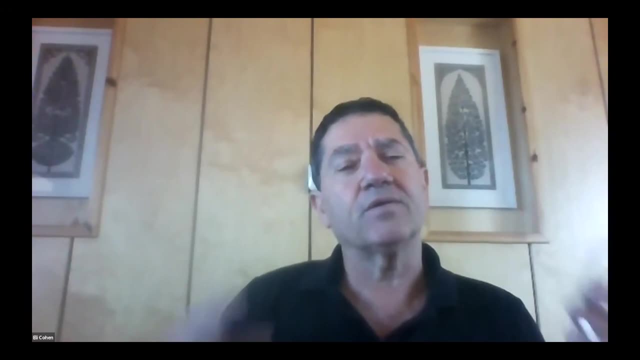 in africa, for example, and i said no, no, no problem, of course, but then i have something that said: to send people to every village in the world to build a system, it's impossible. then i was thinking about building something that you can send over and i i was thinking about the container. this is. 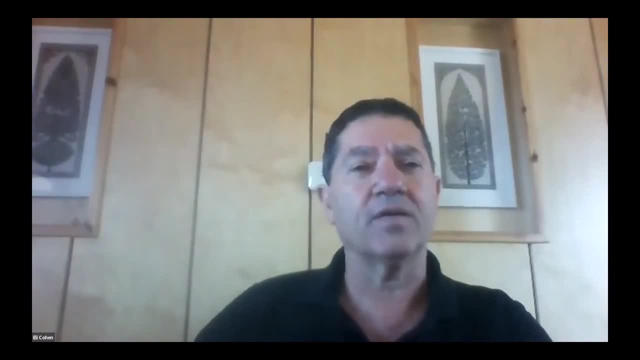 something that can reach today almost any, any place in the any any corner in the of in the world. so we took this platform and we built on this the set system. of course it's built in a special way. it's a got a special height, especially the. the hydrology inside is a well designed 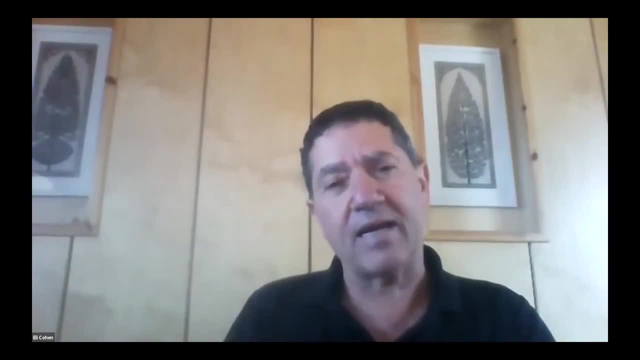 the hydrology inside is a well designed, it's a well designed, et cetera, and it's. it's being sent in the container with substrate all over the inside with all the hydrology systems inside. you just take it to the size and pull it out, and talking about 20, 20 feet containers and the 40 feet containers as well, we 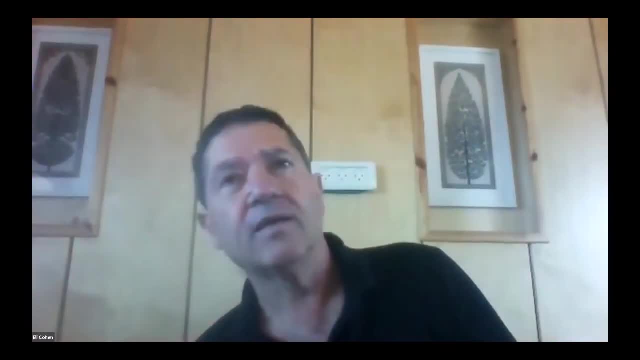 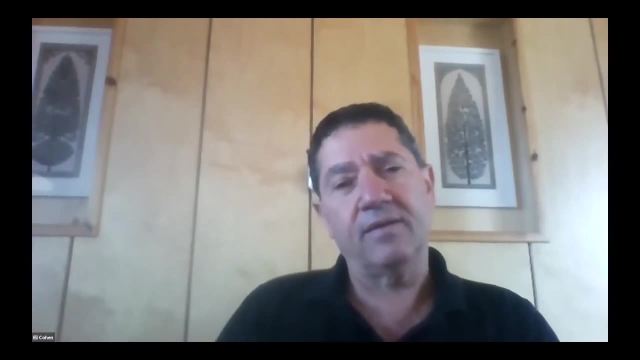 have the different variation: the most, the most uh uh, the most uh um. popular one is the 20 feet and it's reached the. it's a six meter and that's the two and a half to 2.4 meter width and the. The height of it is something like 85 centimeters. 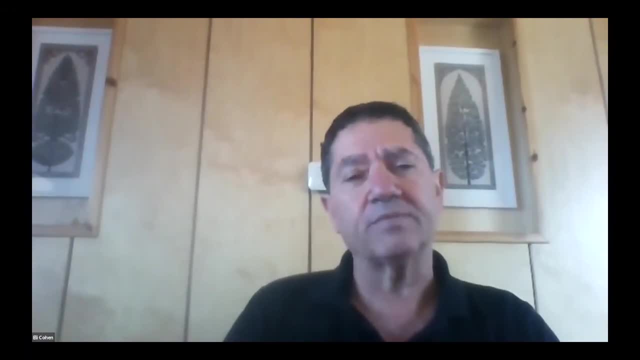 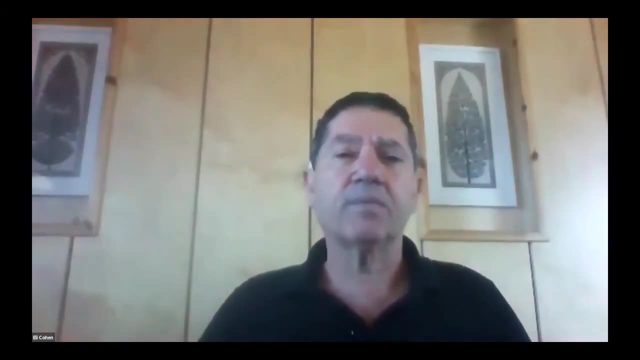 Each pond. all together it's got something like 40 square meters And it can treat between 4 to 40 cubic meters per day, depending on what's coming in, If it's just a semi-contaminated river or lake. 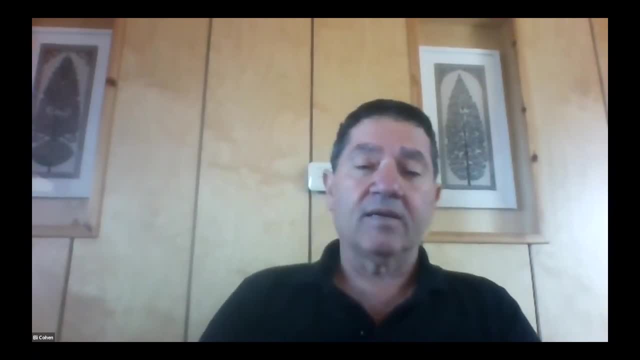 it can be up to 40 cubic meters a day, which is something like can reach also almost 400 people or 600 people supply of water, even more than that. So it's very efficient and it lasts long. And there is like, as someone talked about the pump, that was stolen. 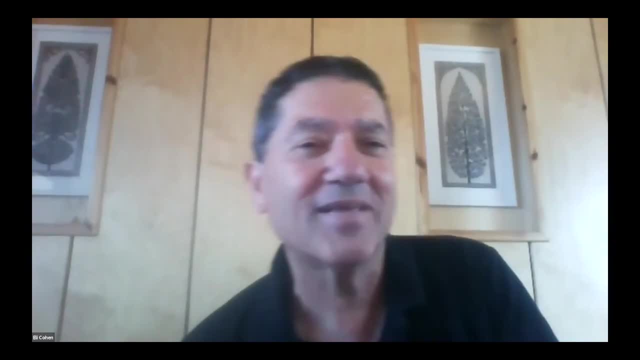 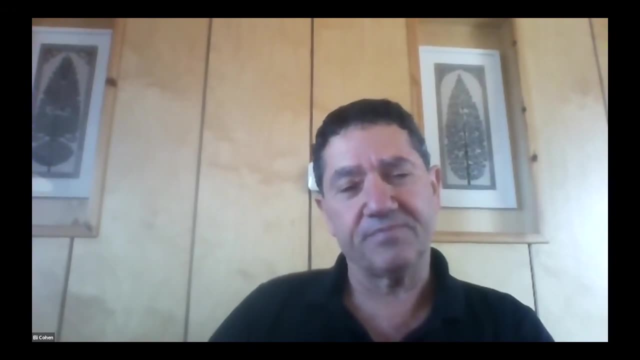 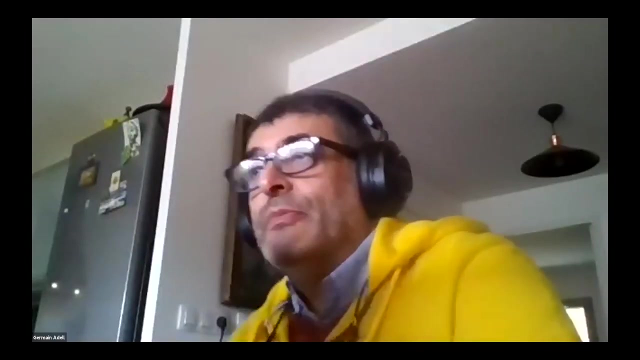 we don't have any pump to steal, It's just there. Nobody will take anything. So this is the idea. Do it simple. That's it. I hope I answered your question, Jeremiah. Well, yes, but I'm still. I would like to see more information. 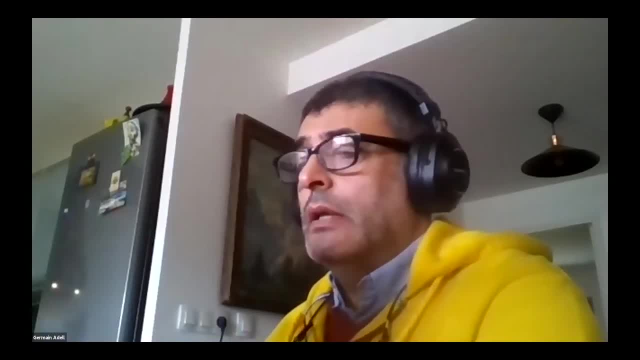 I was curious. I was looking at your website and I couldn't find. for the moment I couldn't find some. No, no, no, you're all right, I mean I'll send you, send me, send me. 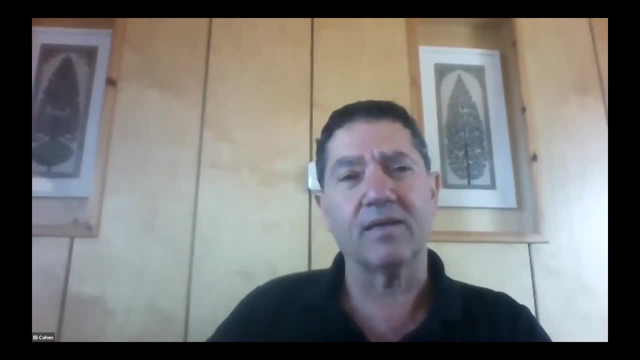 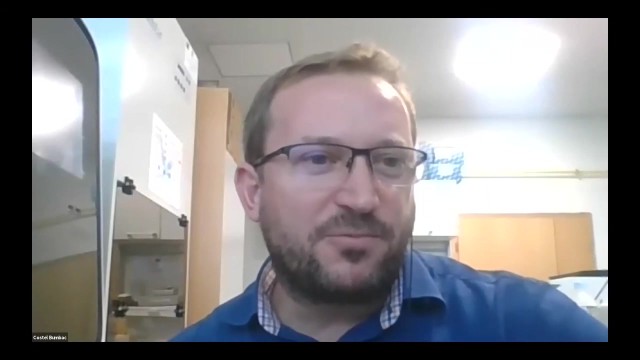 I mean I can send it to all the group. You can send me the, send me the mails and I'll send you Email. okay, Yeah, Sure, You're welcome, Costan. Yes, What would be the lowest temperature limit for the system to perform? without the punishing treatment performance. Well, ever you have plants, the system will function. The water never, never freeze in the in the old zone. So you think about it and we have an article about it. You can send it to you that we all, because we have approaches from all. 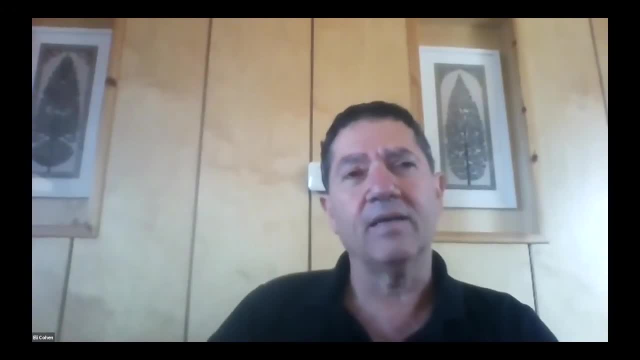 over the world, north of China, north of North America, et cetera, And the people ask about temperature. Well, if, if the, the, the, the centralizes SDP working, functioning in the open, open system, why this one won't work? this is actually closed. 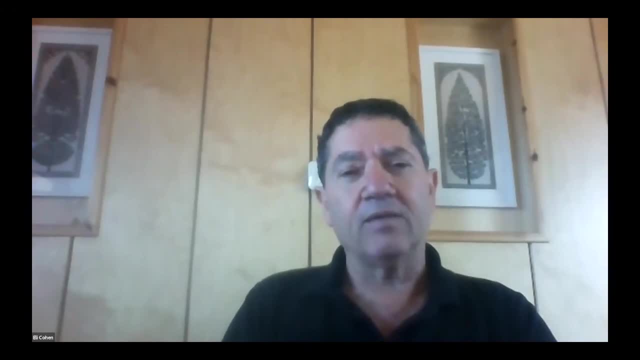 system. the subsurface flow Don't have any open water. water coming in is a higher temperature. There is almost no loss of of temperature in the system itself And when the breakup of the of the contaminants you have a. 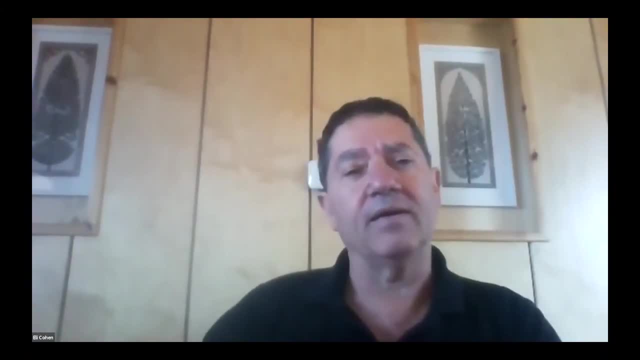 it's actually the exothermic reaction, So you have a energy and heat being released. It's never freeze, It's working very efficiently And the population of microorganisms work in any temperature. You just need to give it a because it's not in thermodynamic. 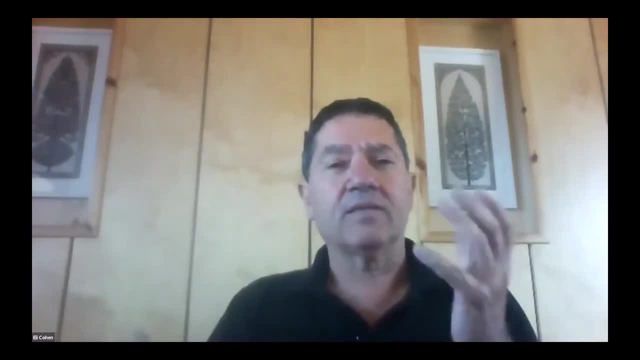 It's not only about temperature. It's about temperature, It's about the pressure, It's about the, the, the, the concentration of different kinds of, of, of uh, microorganisms, say, quantities, et cetera. 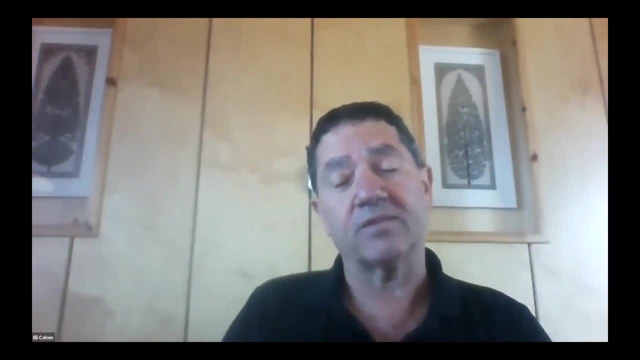 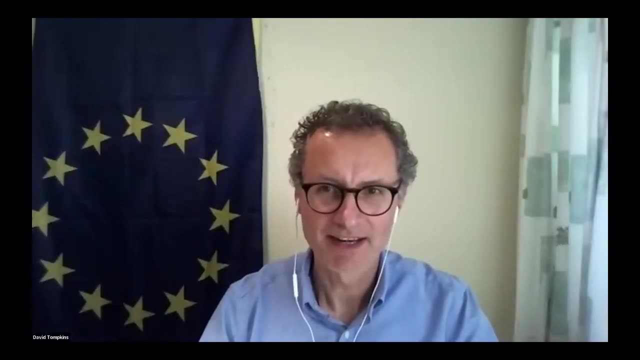 So it's all together create a very powerful and efficient and stable system. Yes, please, David. Yeah, it's a. it's a question I shared with the panelists behind the scenes, but it's. it relates to the the promise of algal technologies. 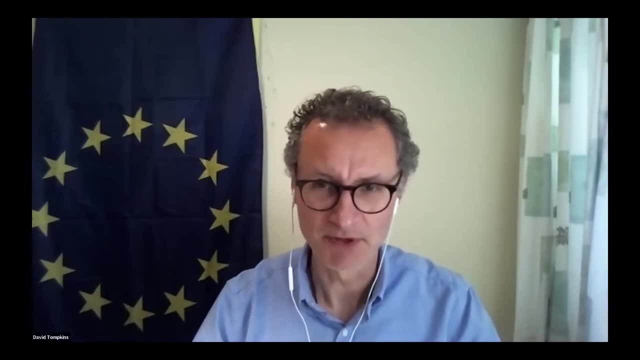 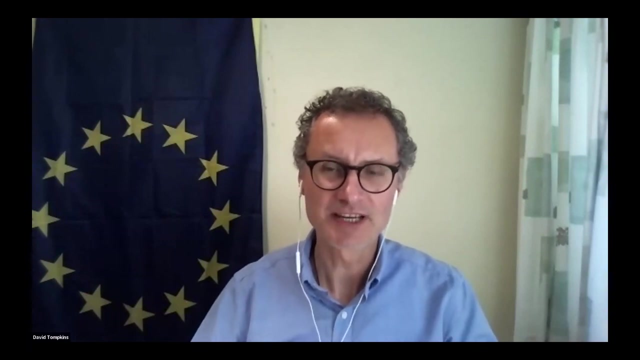 Um, I'm not an expert on algae, but my perception as a non-expert is that the promise is always five years, 10 years, only in certain situations with a high, high insulation. Um, so there's lots of capability, but I'm not seeing that capability coming. 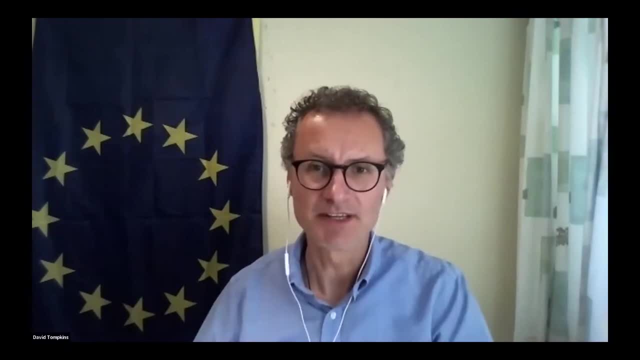 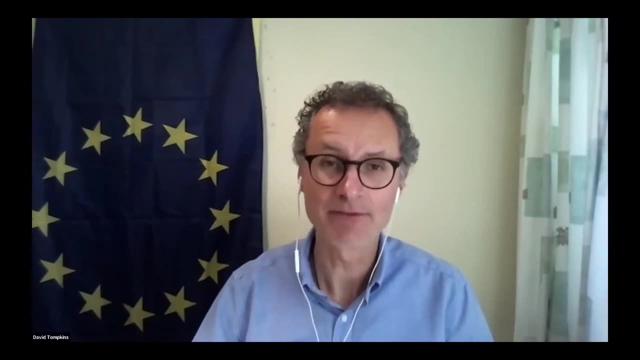 through to market ready solutions. So I just wondered if any of the panelists would like to comment on on that particular question. will will algae meet their promise or do you think they have already met their promise in certain situations that we just need to to raise the awareness of? 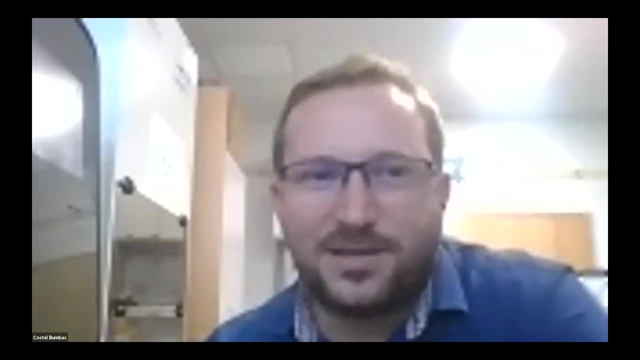 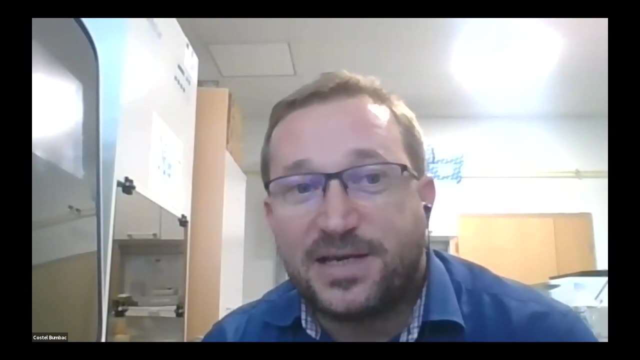 I think the the micrology based wastewater treatment technology uh has a good future Uh. however, um, it has to be uh stated that uh, you cannot talk about using micrology uh for wastewater treatment. 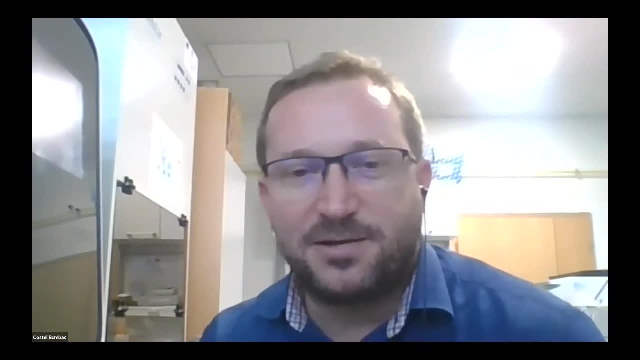 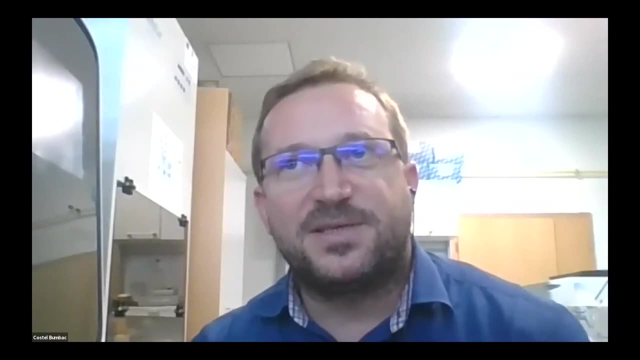 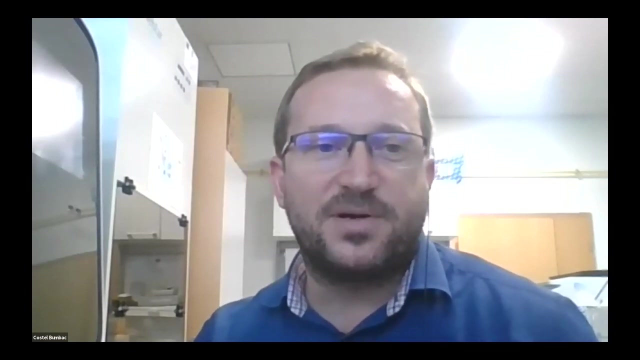 You can only say that you are using micrology and bacteria for wastewater Treatment. You cannot separate the two. because this is uh one of the main reason I think uh, the progress of the micrology based technology is progressing hard, because everybody is looking 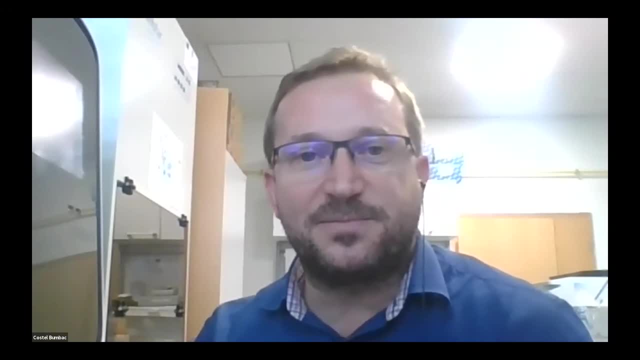 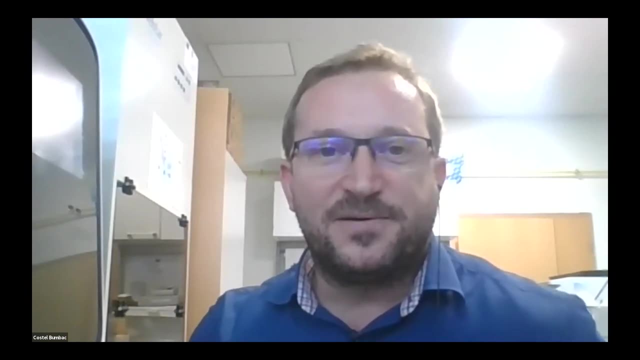 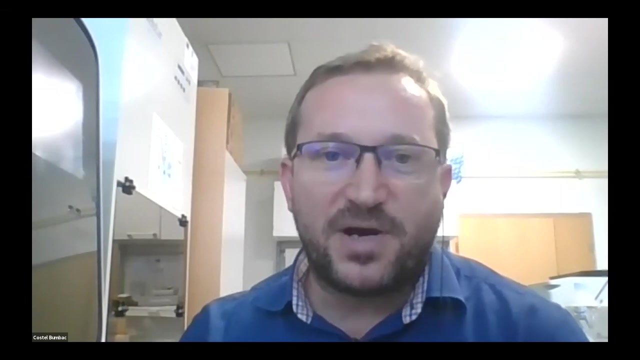 at the development of the micrology based technology for wastewater treatment, as uh they are used in the cultivation of micrology uh in uh algal ponds. So the future Is uh either a biofilm or a granular shape activated algae meaning uh. these are the main. 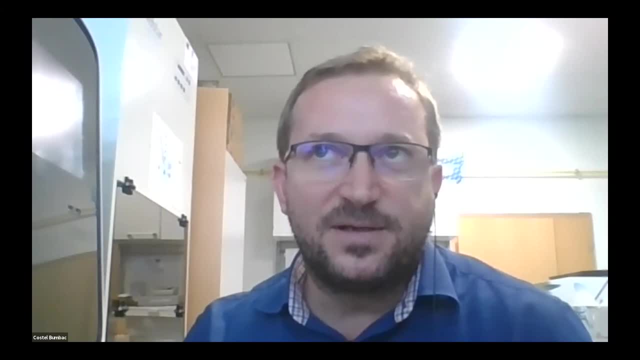 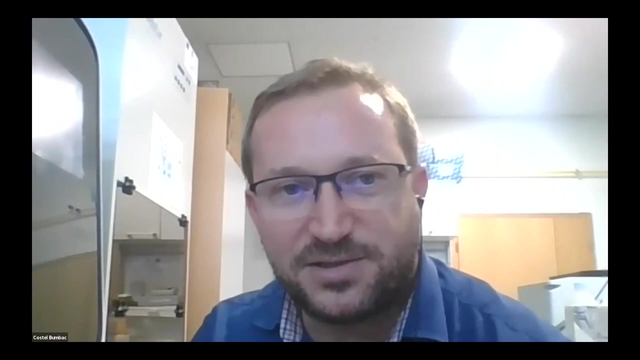 solutions that offer the possibility of uh avoiding expensive harvesting techniques, meaning that the biofilm uh, if it detaches from the platforms, you can easily separate, or the granules have a very, very uh high settling Velocity, similar to the granular activated sludge, which means that within one minute you get 99.99% of the 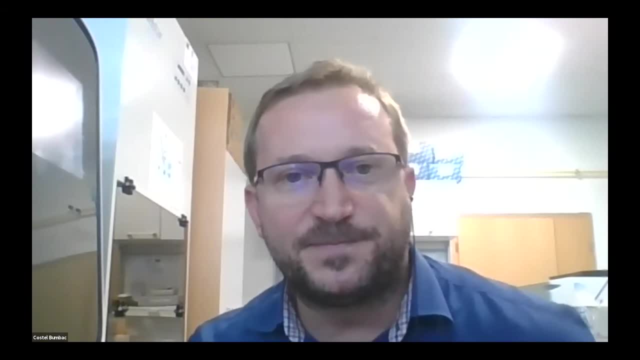 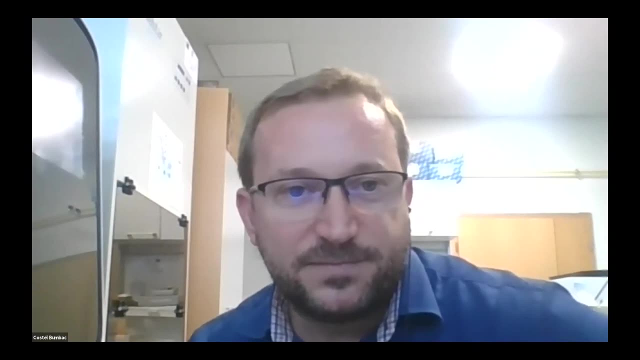 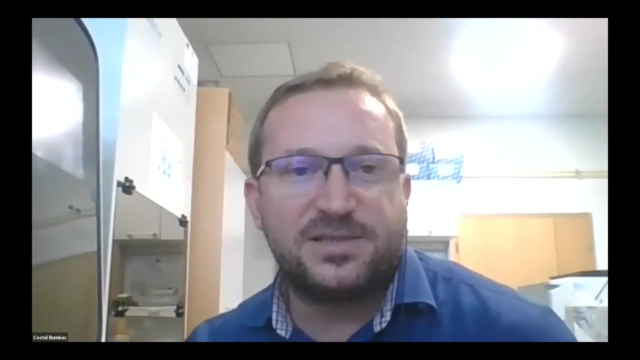 micrology, uh settled within the system And we do have a project ongoing, which just started one month ago, which is called the ground recovery, uh, meaning granular activated algae recovery, which is which is a process for uh. 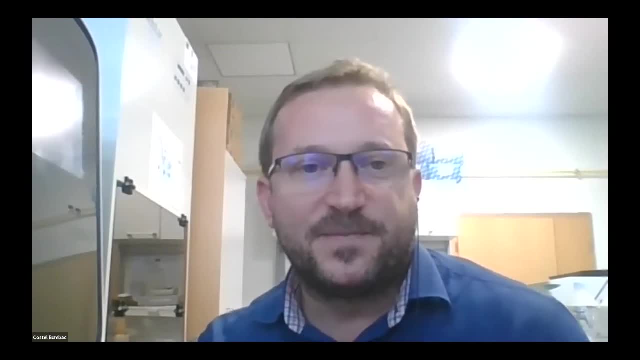 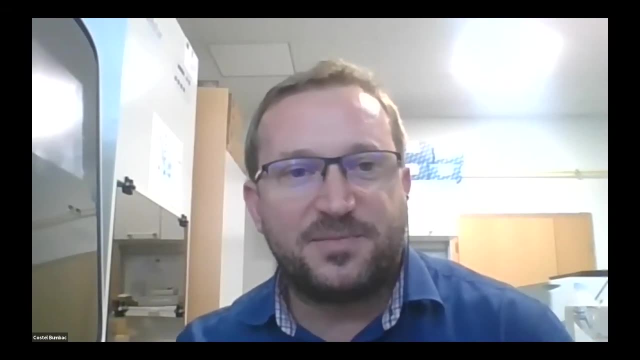 uh main wastewater treatment. uh meaning using the micrology based granular activated algae as uh the main treatment option for wastewater, mainly municipal and with the possibility of recovering the resources from the residual biomass, which should be of greater value than the one of activated sludge alone. 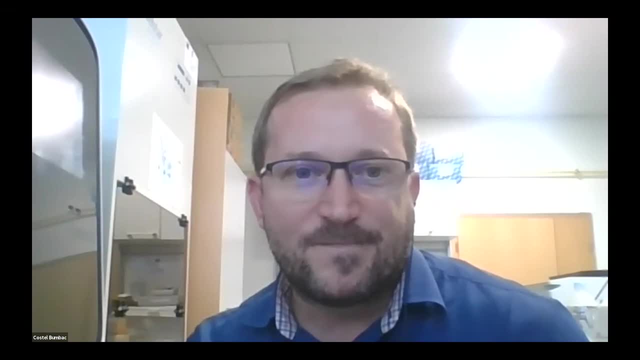 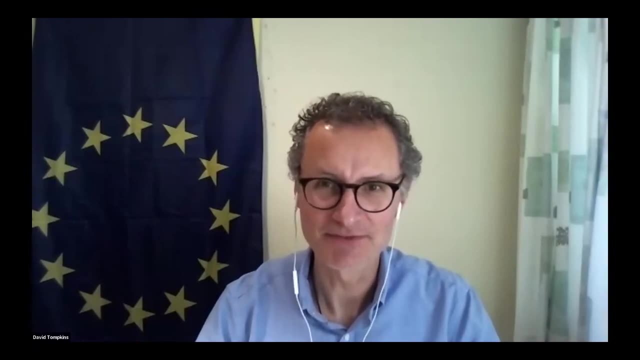 Thank you, Costelle, I'm, I'm, I'm going to, I'll, I'll, I'll. abuse the privilege, Ezki, if I might, and and ask a bit of a, a cheeky follow-up question. 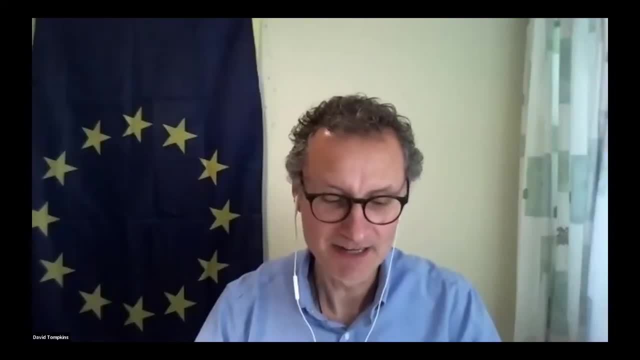 Both- both for you, Costelle, and also for Eli, because, Eli, your presentation was extremely inspiring, just to show us how these things can be implemented and that they work. So the question really is, why aren't we doing it? And so the follow-up from Costelle is. 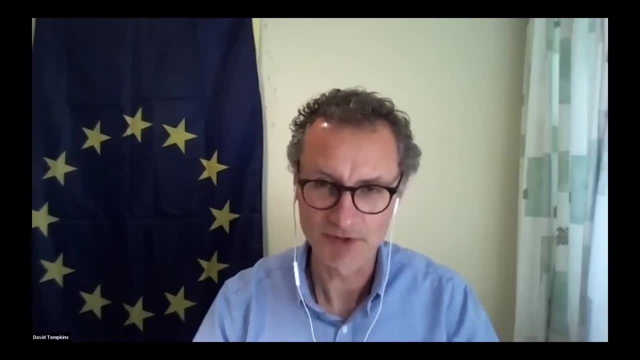 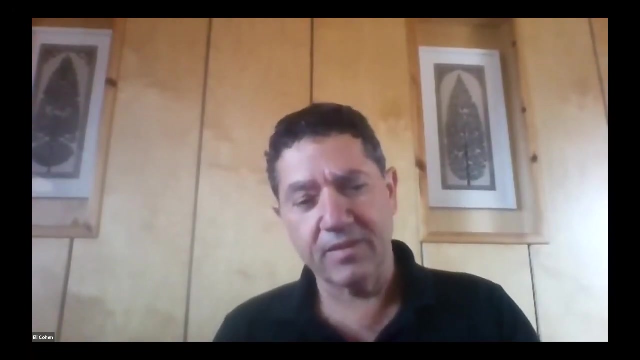 are these kind of algae systems- the other systems we're talking about- just unnecessarily complicated? we know how to treat wastewater using nature-based systems. should we not just be focusing on implementation and further uptake of the existing straightforward wetland type systems? well, i'll tell you a question. algae is very important component of the system, but for myself, 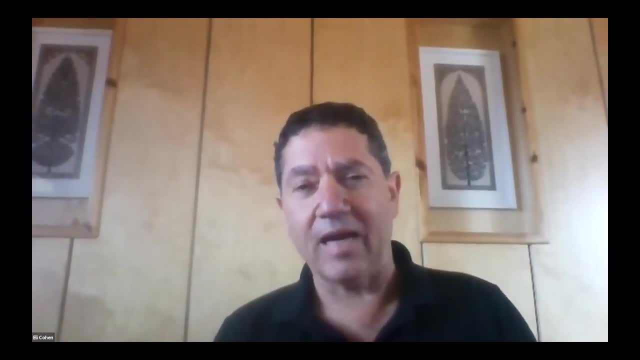 i am against monoculture, i believe in a hybrid system and and the polyculture. and to depend on only one, on organism to do the work for you, you know it's very, very dangerous and it's also need a lot of energy. think about if you want to grow your garden only with the, with the, with the. 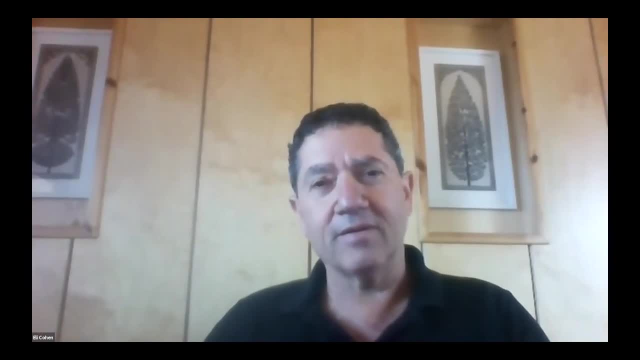 roses. you know how much energy you need to put into it to keep on harvesting the the other one. so i think that algae will come there anyway, will be there anyway. one way, if you want it or not, you can leave some open places in the system for algae for specific things, if you know that it can. 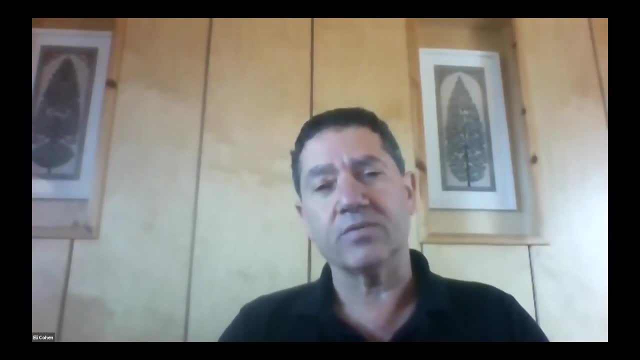 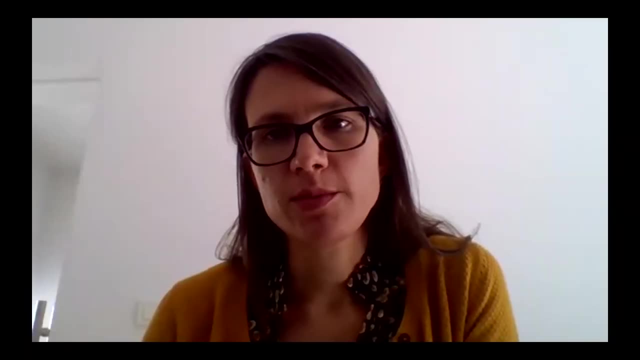 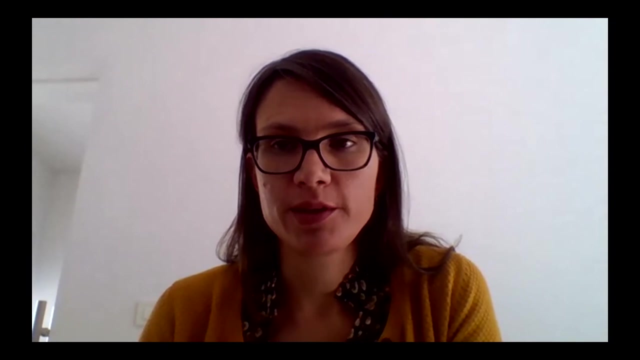 do something specific, but not only to build the system, only on this one. this is my important, thank you, may i also comment the algae topic? so i think that this, um high-rate algae ponds and similar systems that based on algae, should also um be looked as a perspective. 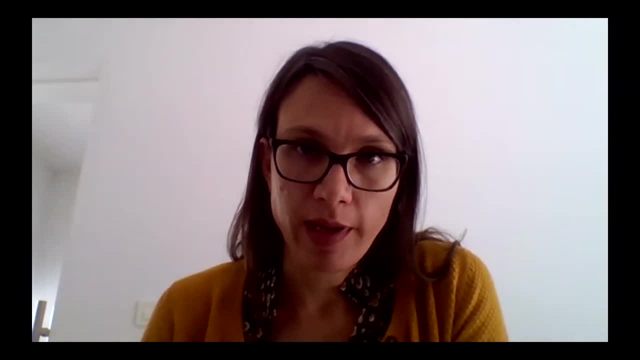 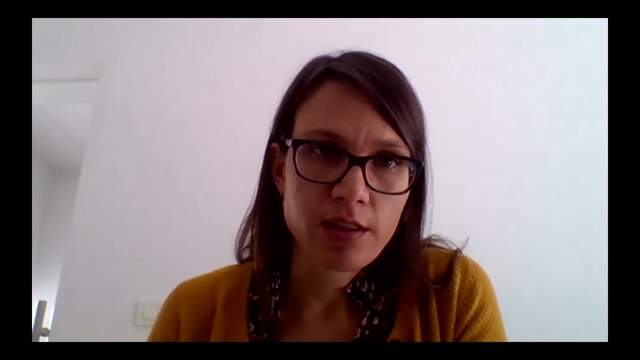 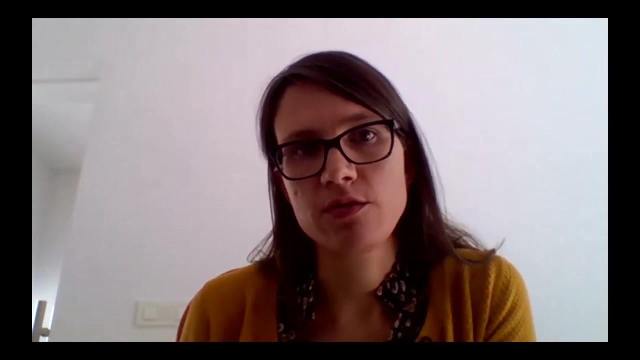 um, not only as a wastewater treatment plant, but as a system that produces algae as a product. so if you can sell this algae as something as a bioproduct that you gained from wastewater, then it has a future. i think i know that there are also horizon projects that are working on. 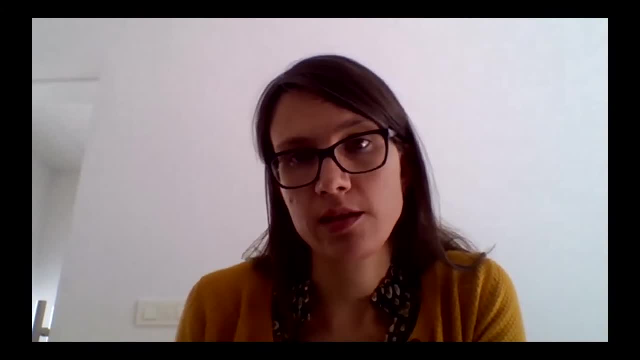 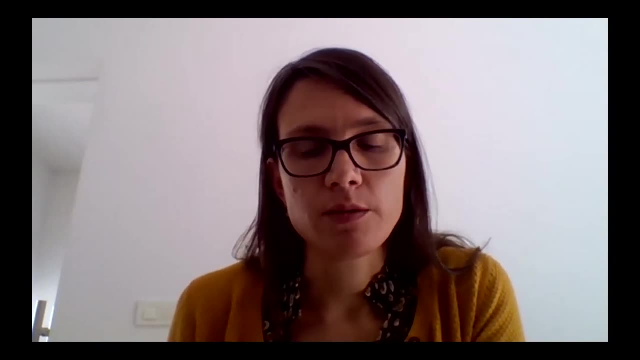 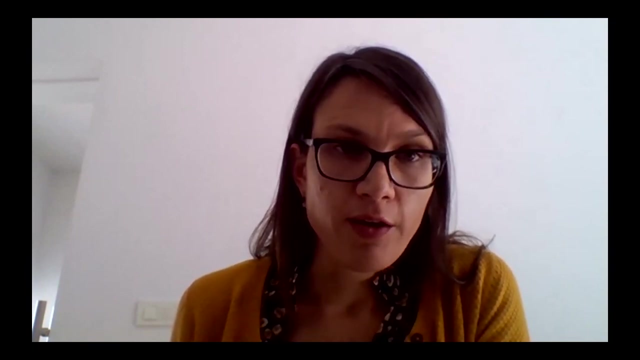 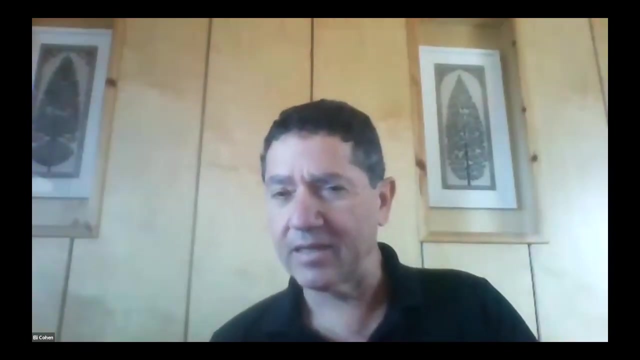 production algae, biomass and then producing bioplastic from the polymers that are stored in the algae. so these are, then some products with high added value, and this can then also maybe um cover the energy expenses that you have with breeding the algae. i have to say you're very much right. i mean to believe all. i was involved in these. 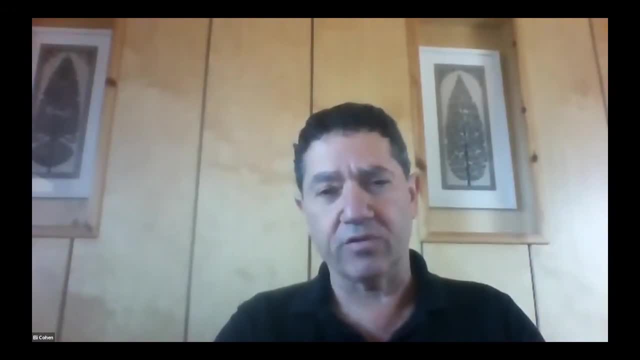 farms that used to go algae because they were looking for the biofuel. the price of of oil was very high at that time so the oil from the biofuel from Algae was the top interest in that time. But now, but maybe if you have other uses for the algae, 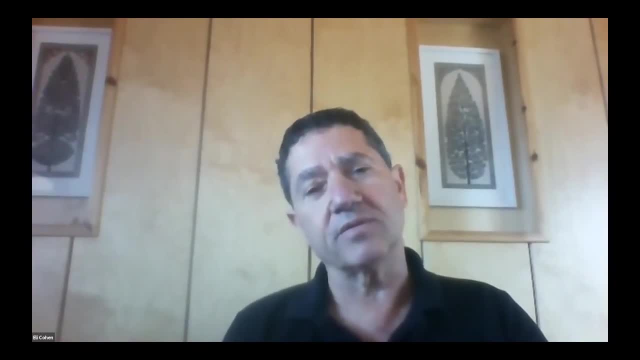 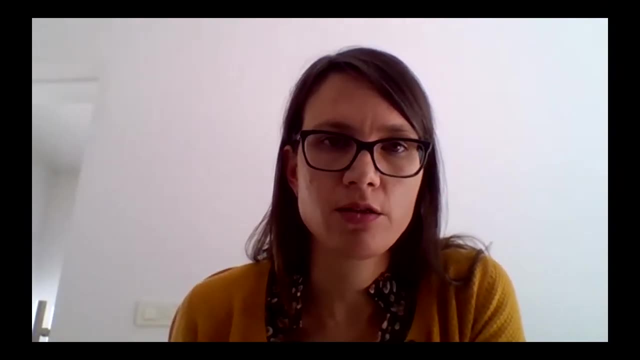 of course, you're right, It can be a by-product of it- drinking water, you're right- Or as a bio-stimulants in agriculture for better growth of plants. This is also research that is going on and to produce these phycocyanins. 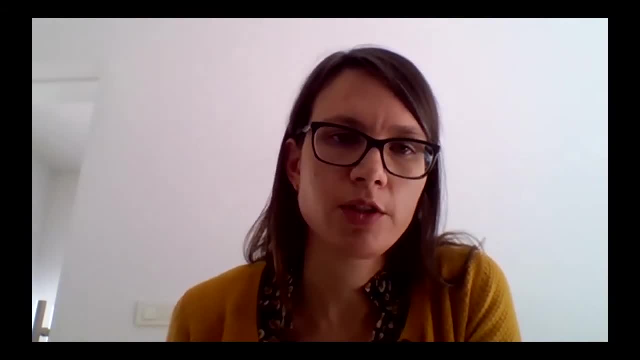 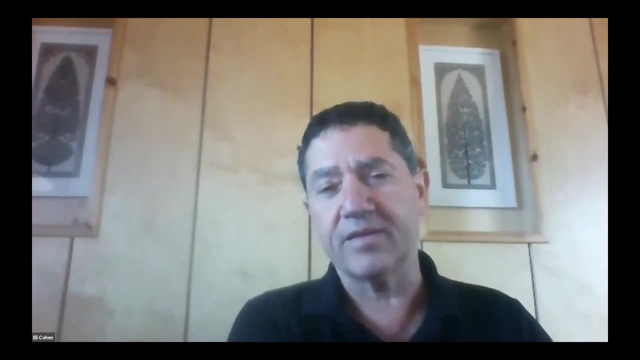 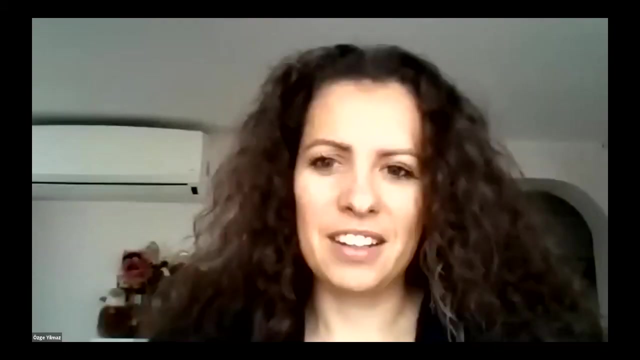 the colors, the pigments from the algae products? You're right. then you don't have to invest in feeding the algae actually. Yeah, they do the job. Yeah, you're right, It's a win-win game. Thank you for this question and answers. 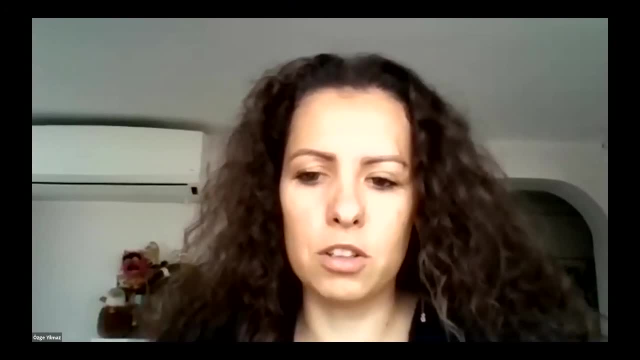 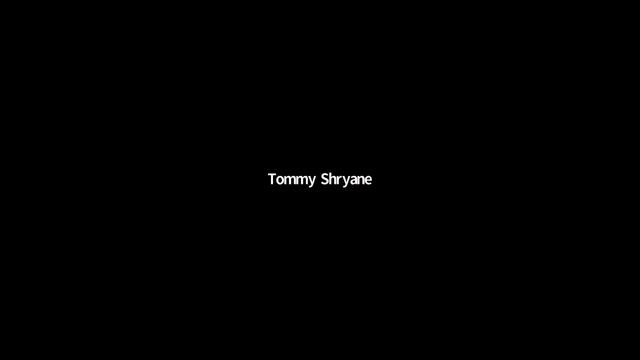 I would like to ask Tommy if you have some questions, because maybe you raised hands and I didn't realize. No, thank you. Thank you very much. My camera's not working. this is my IT setup, Sorry. Sorry for not noticing it. 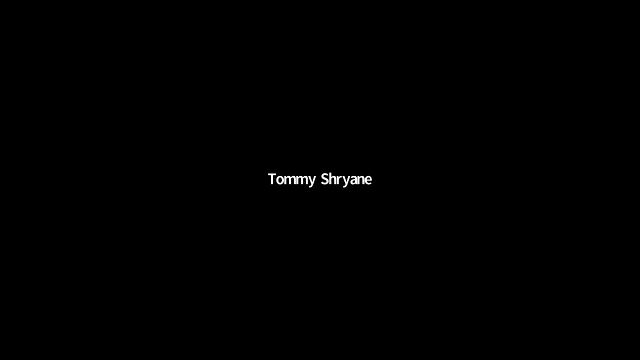 Sorry for the delay. Please go ahead. It's quite all right. Thank you very much for the invite and for the presentations. They're very interesting. I work with Irish Water. We're a new utility in Ireland, So I just want to know: Eli, how did you? 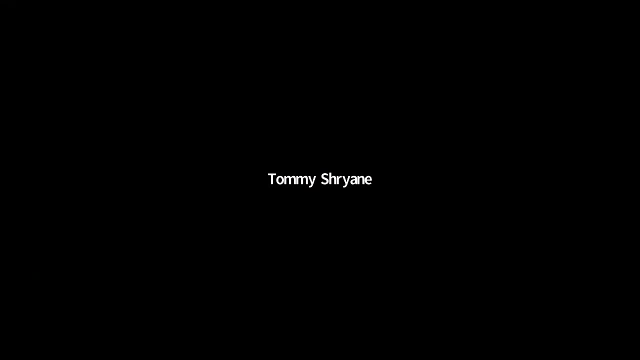 get your buy-in for the decentralized sewage treatment system for individuals. Was it through licensing or legislation And did you kind of, was it a partnership approach? And just how were they managed then and maintained? Talking about the system, you ask: how did I get into it? 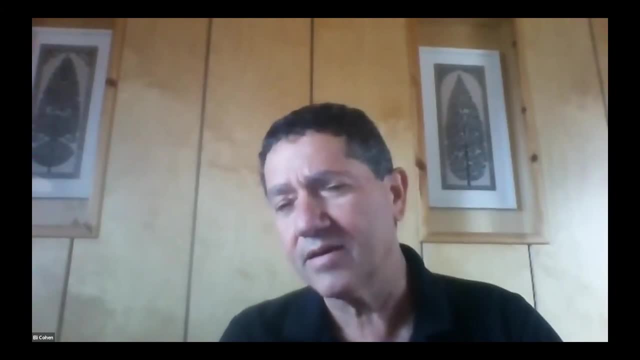 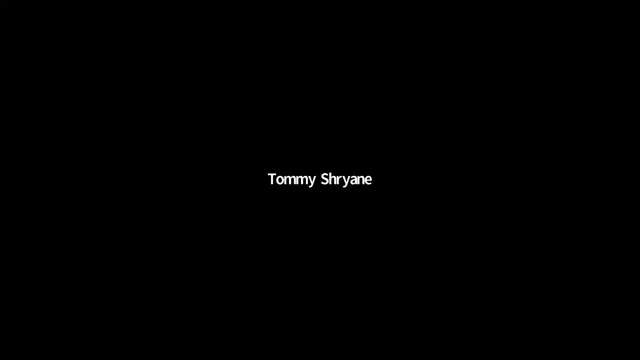 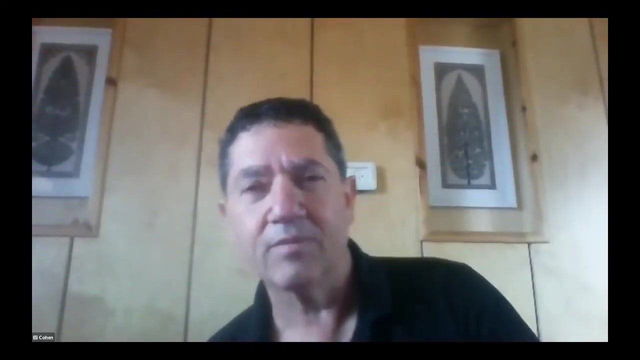 or how do I move it forward, kind of thing. Yeah, how did you get buy-in from the different operators? So you showed a number of examples there from industries. What was there? I think it's well. my background is the physics and thermodynamics. 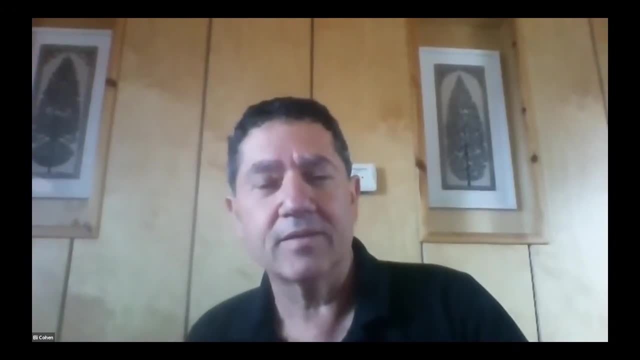 I was working. I was a, I did my. I was working in this high-tech company leading the R&D over there, And I bought my farm in the Galilee in Israel And suddenly I figured out that I want to be a farmer actually. 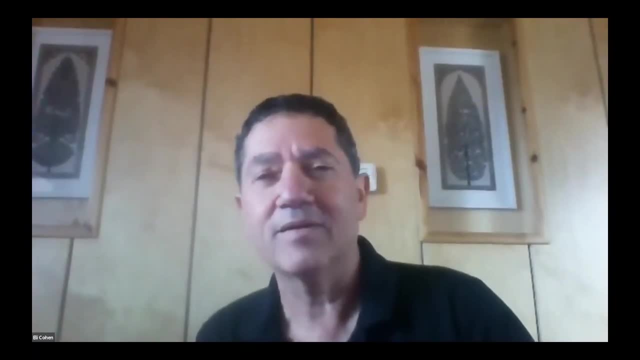 I just I left everything and started doing farming And I didn't know what I'm getting into. But luckily I got somehow very fast into aquatic plants And I started working with water. I used to export plants to Europe, to Japan in the time. 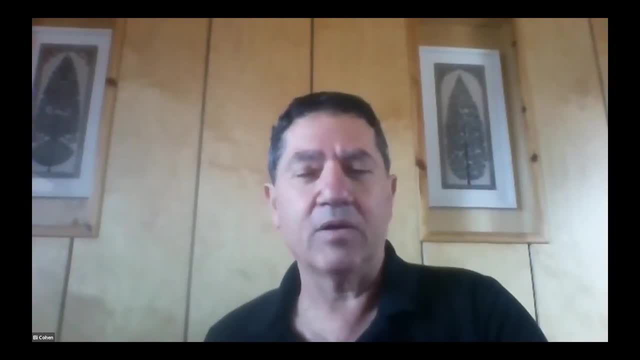 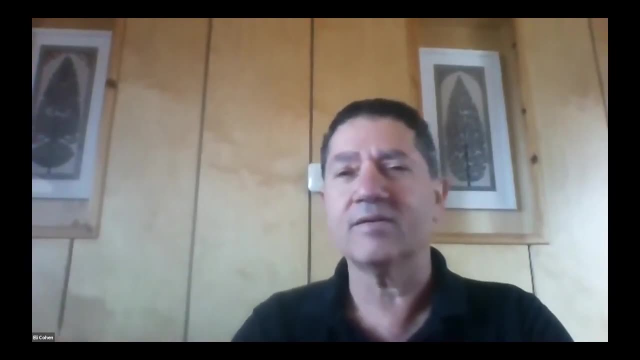 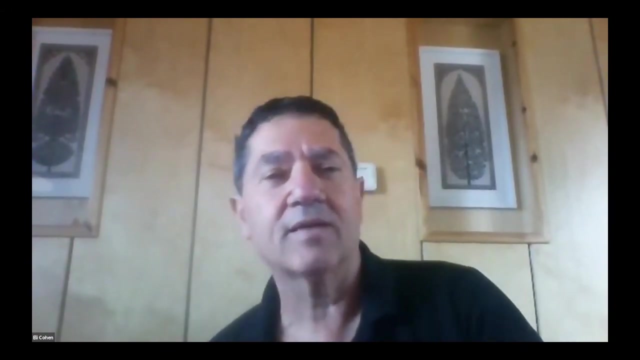 We were one of the biggest growers of aquatic plants, but talking about 25 years ago. But by working with water you understand very fast that actually whatever you learn or you hear from other people in Europe, other places don't catch, Because in every ecological area it's different condition. 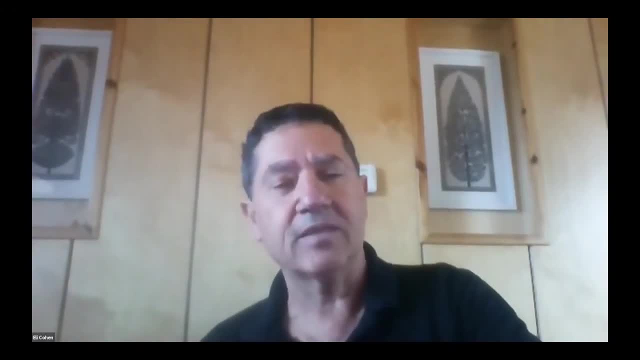 You have to adapt and you have to change and you have to tailor the solution for each place. So a lot of knowledge start to build up. And also I found out that the whatever I learned, I learned. I learned a lot. 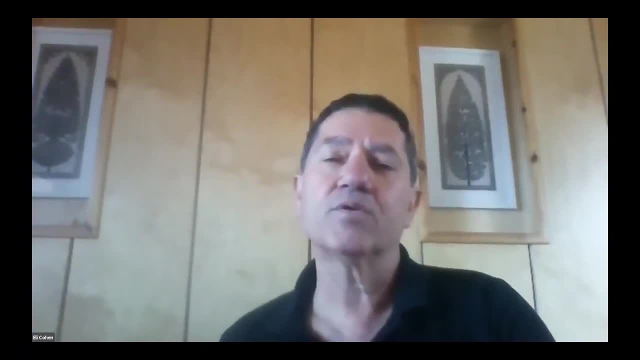 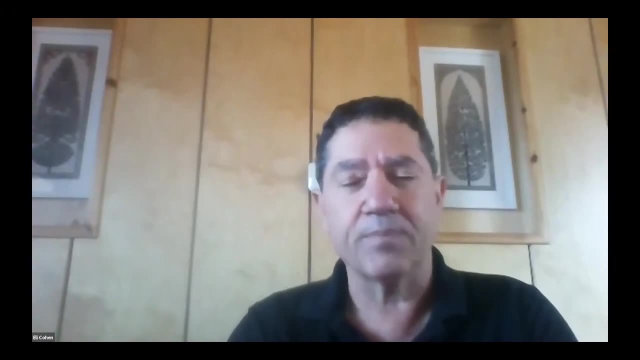 I learned in thermodynamics and physics play a very important role in what I'm doing, So it's intuitively. I learned many things. I did it, I tried it And then I found out that the power of nature is. it's amazing. 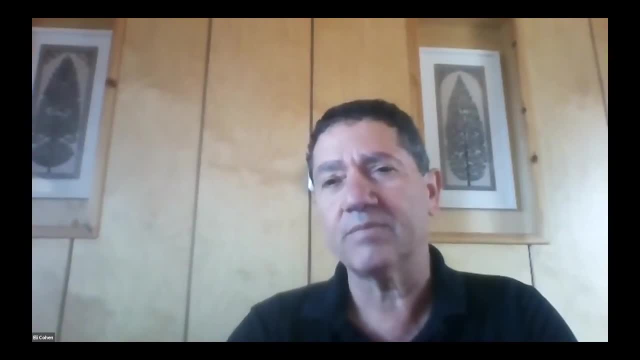 It can do anything, And today I'm not afraid to touch anything because I know that it's going to work. You just need to tailor it in the right way. I mean, it's a combination of it's, like someone said before. 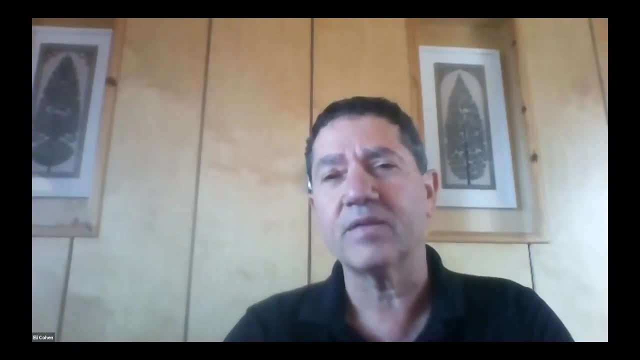 it's not simple, but it's not. It's a need to do it right. I mean, if you don't do it right, then you first of all, it's club, Later on you have many other problems. So you need to tailor the system in the right way to start with. 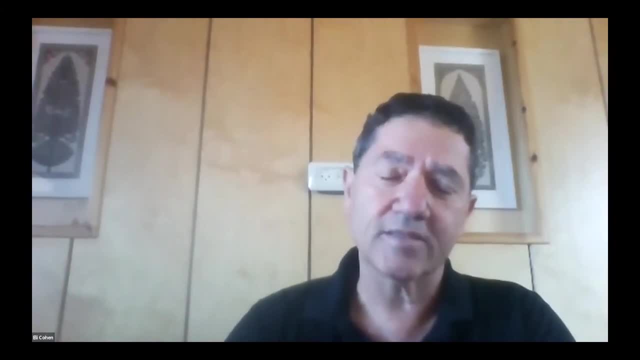 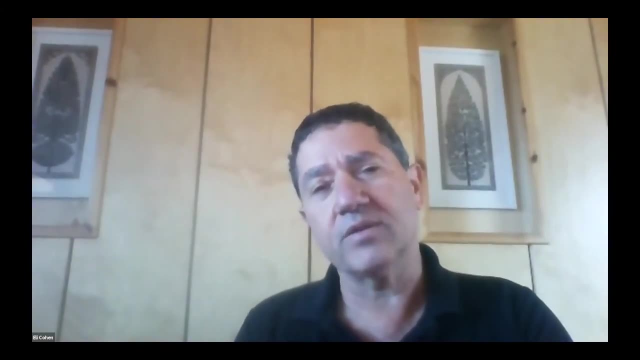 And you need experience, But it's something that you can learn. Just need to be on the field and touch, put your fingers in And after a while, you start feeling it, And this is the way to do it, I mean, and more people will do it. change will be here. 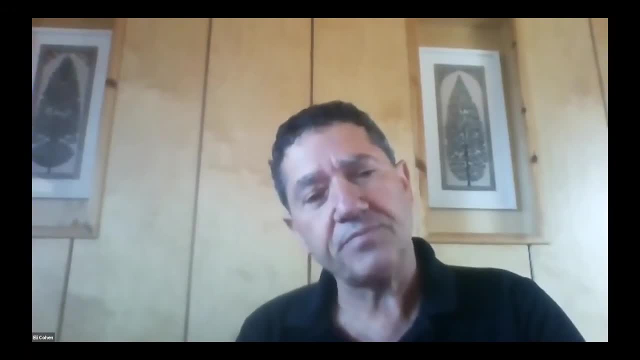 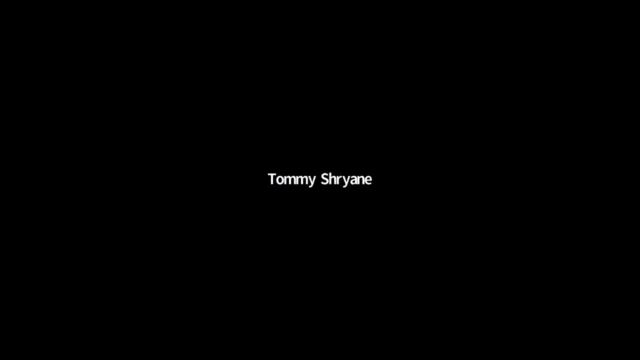 I hope I answered the question. Yeah, no, thank you. That was good, Your demonstration project in India. Just I'm wondering how you got the various companies and industries- dairy companies and textiles and sugarcane. How did they buy into your vision of creating the green tree of life? 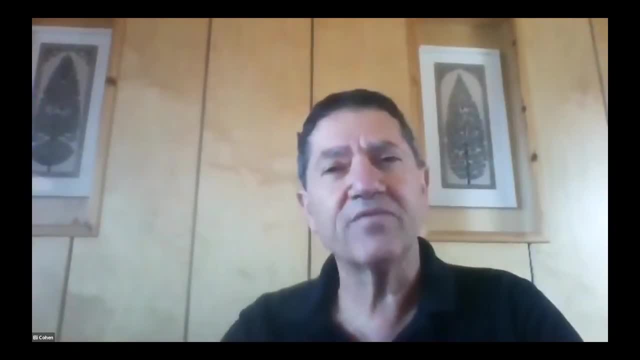 Well, I found that people, on average, love the idea, Really Love the idea, And they want, they really willing to buy it. But later on, when it's come to, I know, to actually implement it a lot of, when they reaching the government and the latest et cetera, start, questions start coming up. 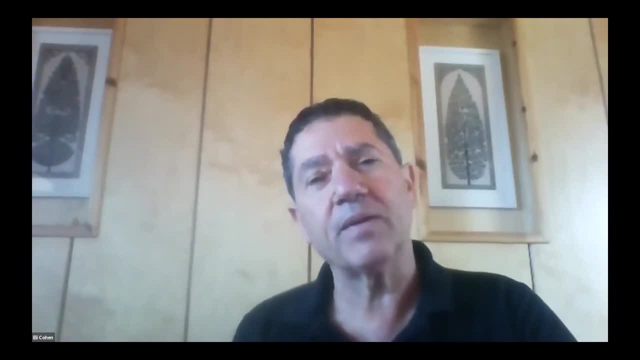 And then the story actually starts. But only the people who really believe and trust you go ahead with it. Of course, when the numbers goes up you have more people that actually willing to try And but it was hard at the beginning, Very hard. 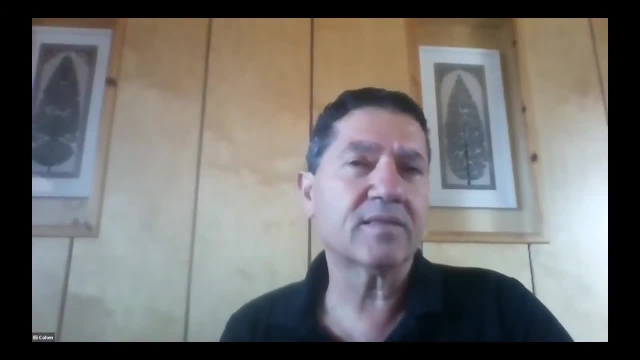 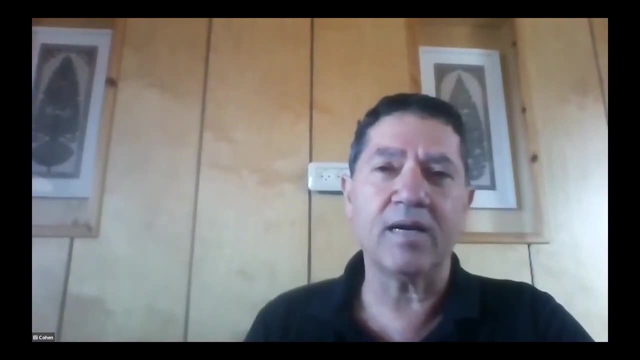 I mean to get into it and to make it Change, But but I feel that it's over there and that you can do it by, you know, by publication and the PR. actually, about India, I didn't put the one whoopie in publication and PR. 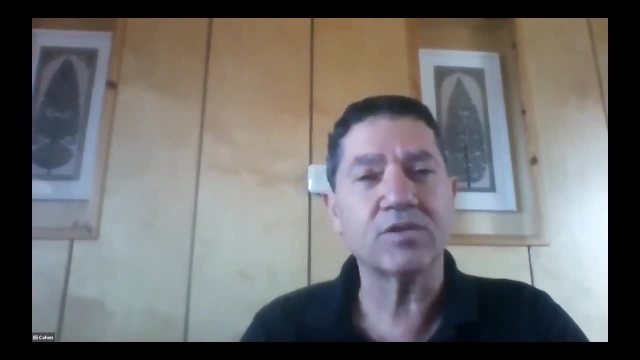 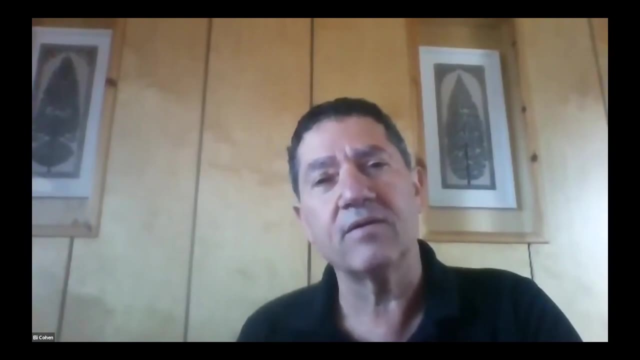 I don't know how, but people just heard about it and came to us and I get the talks here and there and people just like the idea and they invited me in And it's and it's kind of growing there. today We're working all over India- and we're just doing it before- and also in South America and Peru and Chile and other places. 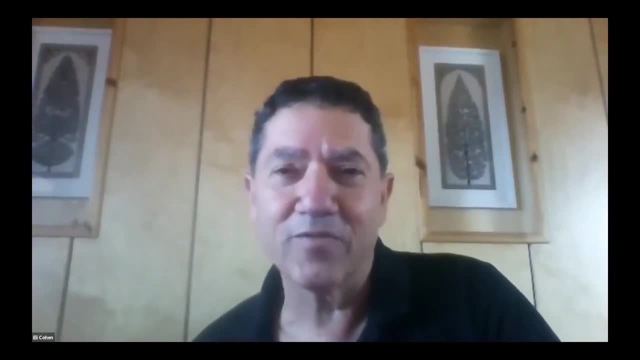 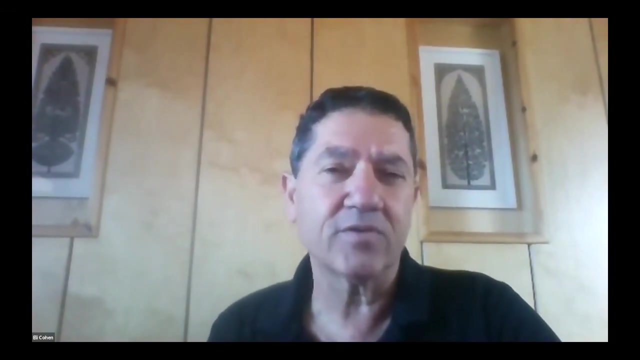 Now we're doing nothing. The corner, But this is different story, Just really kind of here. But it's OK, It's time, time to time out to do other things over here. But yeah, but it's a, it's a, it's something that you need to believe in it. 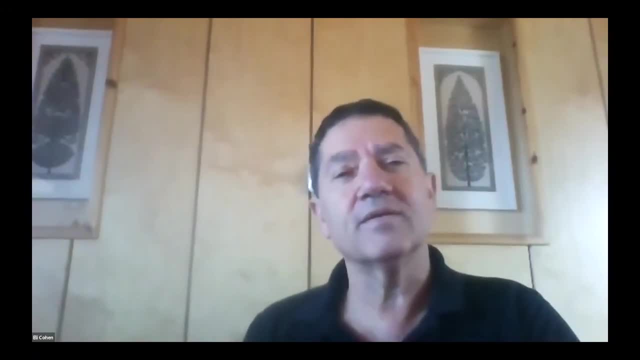 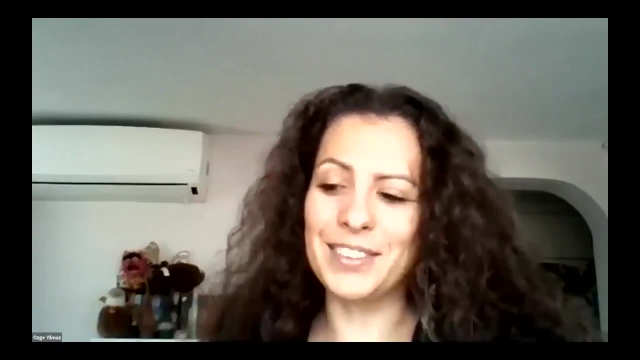 First of all, you need to believe in it, Trust yourself and to go on, And you have a lot of obstacles on the way, But keep on moving If you really want to do it and make a change. So thank you for your patience. 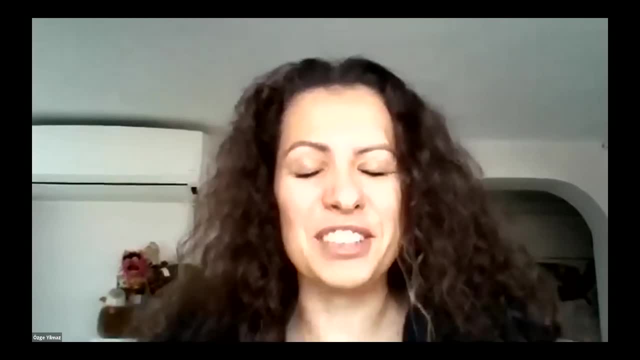 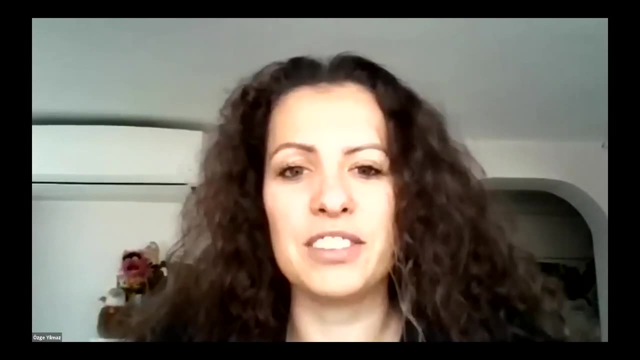 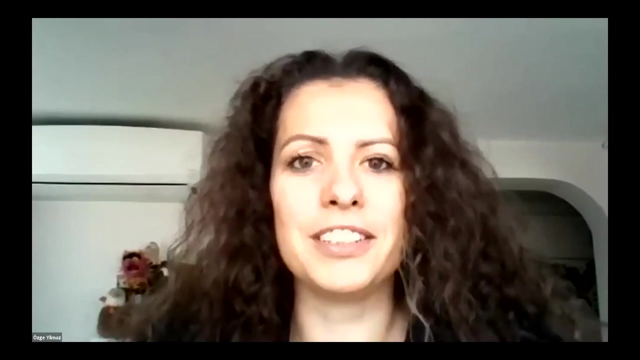 It's been a wonderful event, Even if it was online, But still it was very informative, Very impressive, All of the presentations. I would like to thank all of the organizers, David's, Costa and Christoph, and also all of our speakers, for being here today. 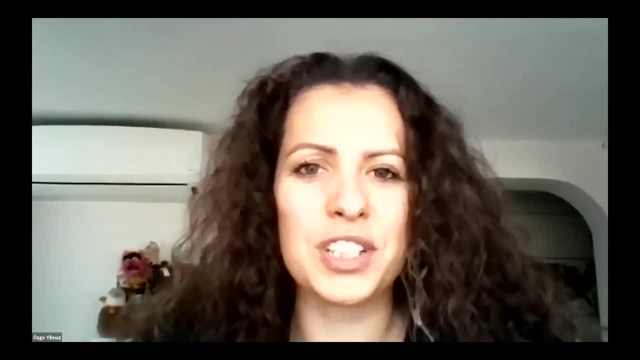 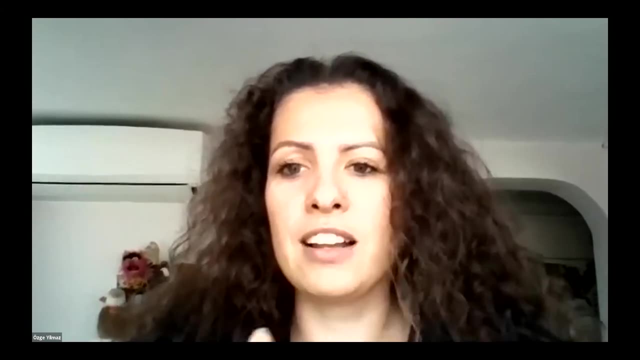 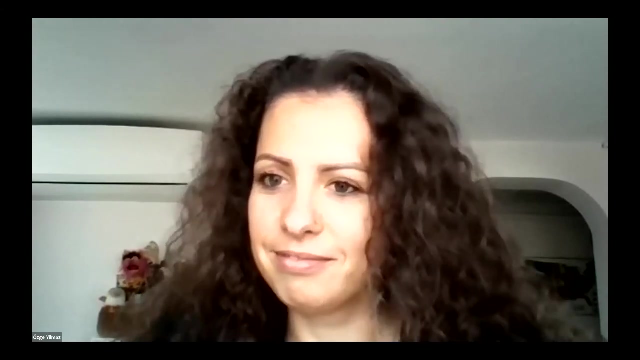 Just answering all these questions Being so interactive. Thank you to all the participants. I don't know if costal or German. Would you like to have questions? Yeah Yeah, We have some closing words for the conference From my side. 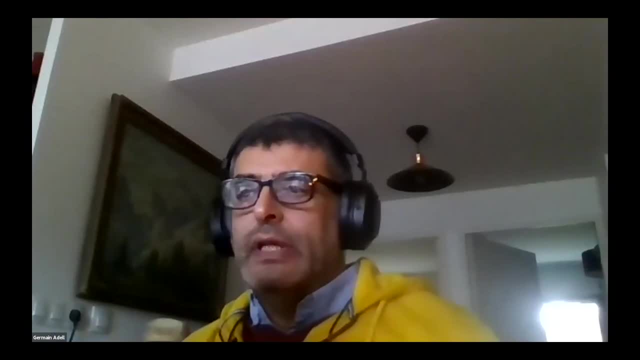 Thank you From my side. Yes, indeed, It was very, very interesting, And it's nice to see people working in similar direction that we are doing, And so we are not alone, And I think I would really like to keep in touch with all of you. 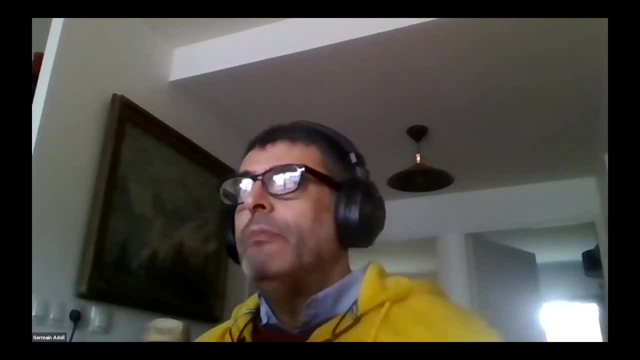 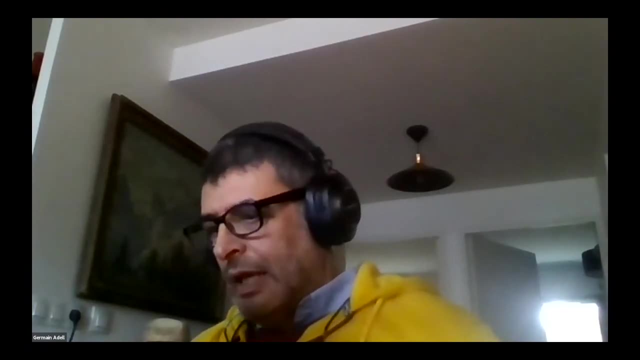 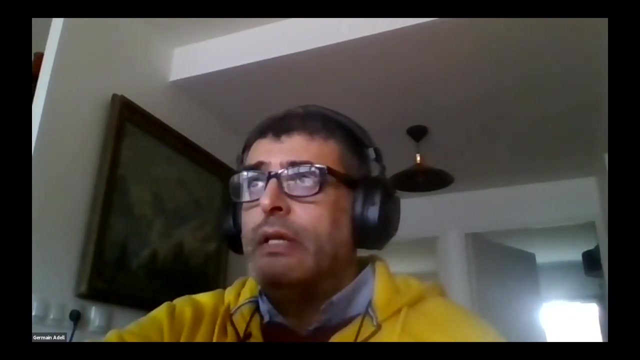 So if, as you said, if we have the emails of everyone and other contacts, I would be very happy to have you in my agenda And, of course, share more information and future possibilities of working together, Because this is: we don't stop working.